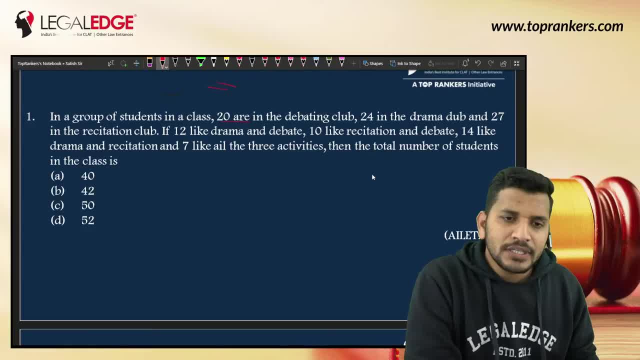 Right in a group of students in a class, 20 are in debating competition a club 24, drama, dub And drama and 27 in the recitation club Right. all these are in the club Now: 12 like drama and debate, 10 like recitation and debate, 14 like drama and recitation and 7 like all are three activities. 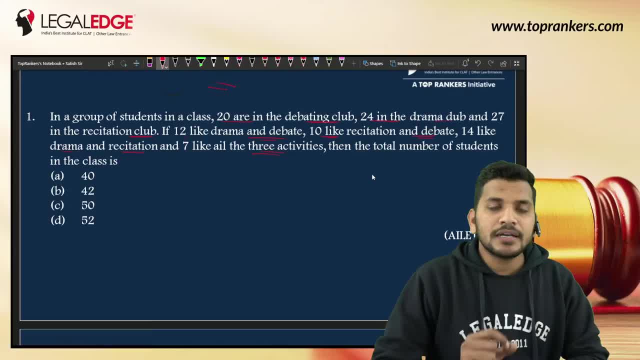 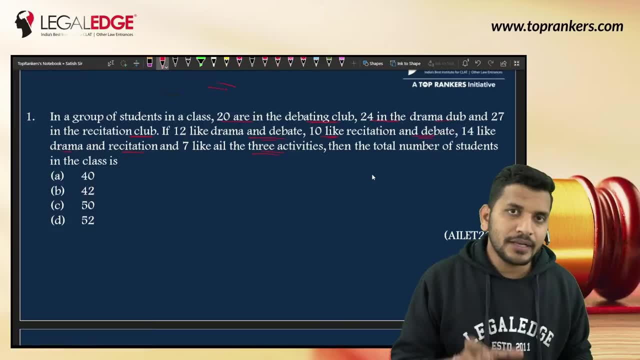 What to do with 7, do all three activities whenever this type of question comes. all only right. So in this type we do it with Venn diagram, and here we will make three Venn diagrams, right? So how will we start? first of all, 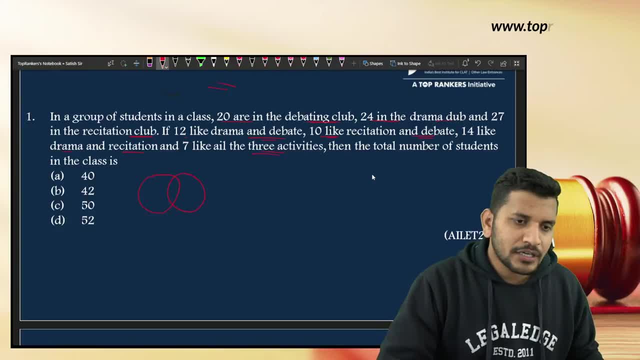 I will tell you. I will make a diagram of three Venn diagrams and start here. Okay, So in a group, 20 are in debating club. So what will happen in this column? Debating will happen, Right. How many are there in this total? 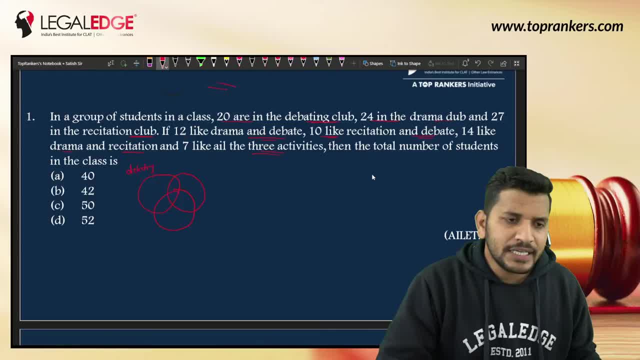 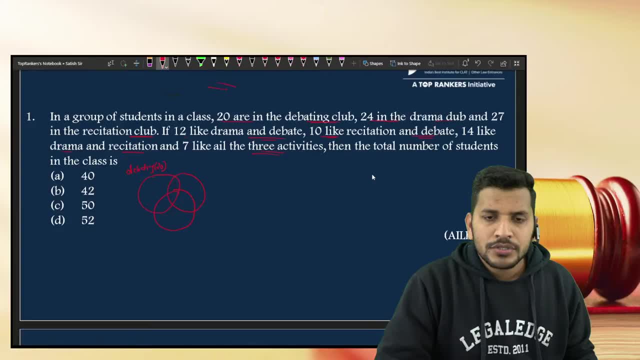 20 are there? 20 are there. 20 are in debating club, 24 in drama Drama. is this one suppose? How many are there in drama guys? 24 are there, Understand carefully. And 27 are in recitation. 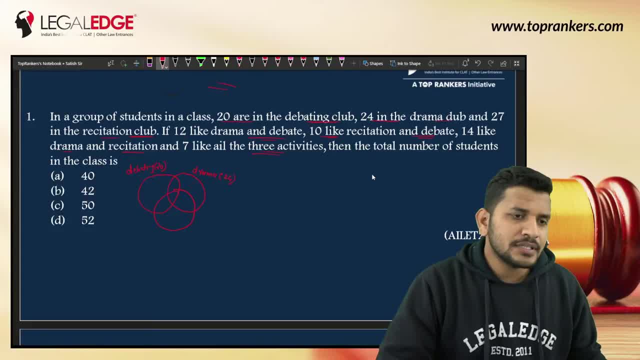 This is it. How many are there in this? 27.. So we have made this. How many are there in this? How many are there in this? No, Right, We have made this. Let's read the next question. 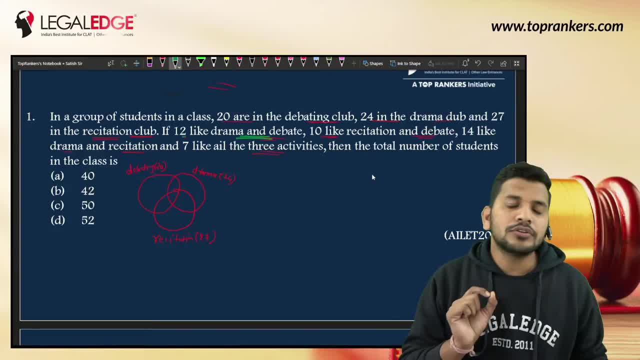 If 12 like drama and debate, Okay, guys, This question says 12 like drama and debate. What does it mean? This one is about debate and this one is about drama. Is it talking about this portion or this portion? Understand carefully here. 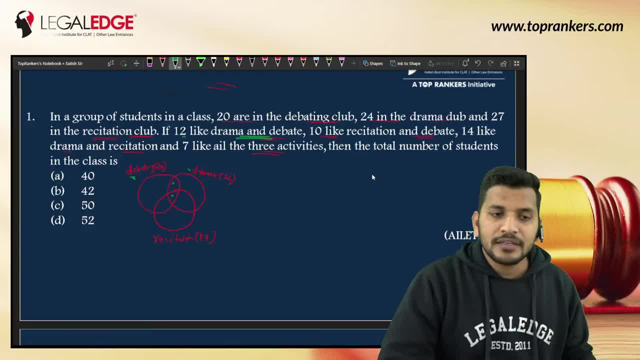 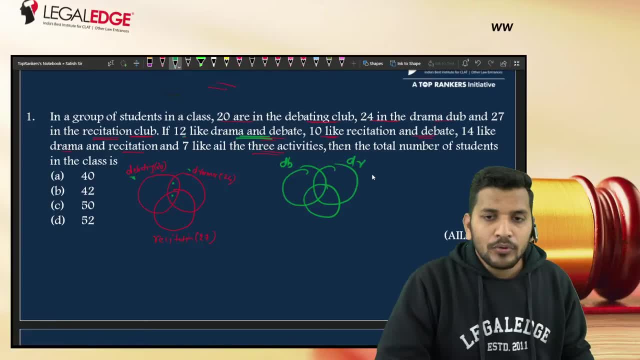 So, if drama and debate comes in this way at any time, It comes in this way by saying this is drama and this is debate, This is debate and this is drama Right Now. what is it saying? Twenty seven, Sorry. 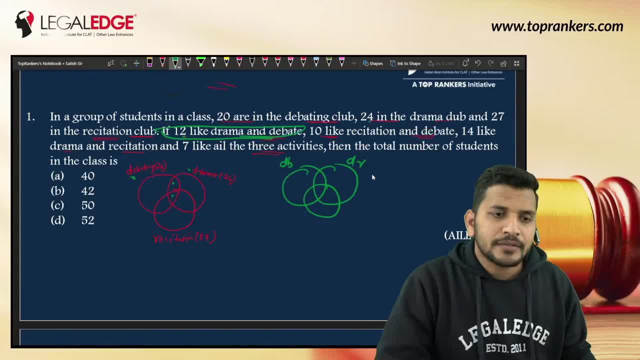 12 will like drama and debate. This is it: 12 will like drama and debate. So if 12 will like drama and debate, So you are talking about this whole thing. Who are you talking about guys? You are talking about this whole portion. 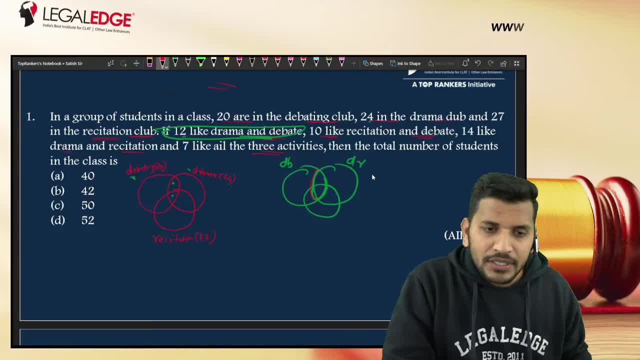 Not this portion and not this portion Because he did not put only. If he would have said: 12 will like only drama and debate, 12 will like only drama and debate, Then only this portion is talked about. If he would have said: 12 like drama and debate only. 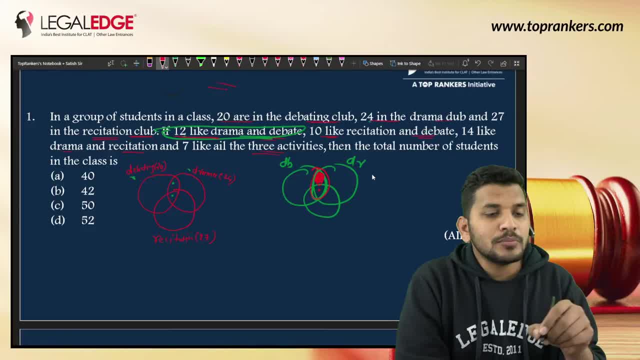 Then only this portion is talked about, But in the question it is said that 12 like drama and debate. So this whole portion is being talked about. So it is being talked about up to here. So it is fine. 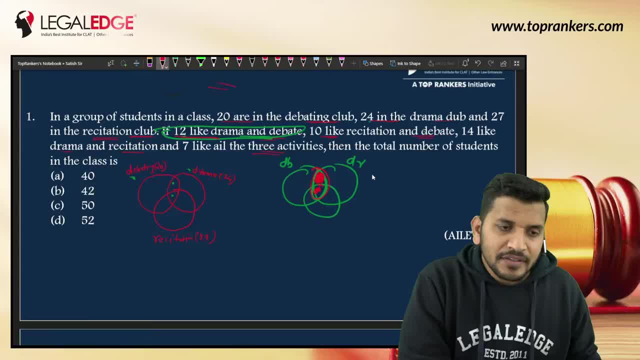 They will make us in this way. Here they will write 12.. This is the way to ask questions. Here we will write 12 and say 10, like recitation and debate. Right, Which is recitation and debate. This is complete again. 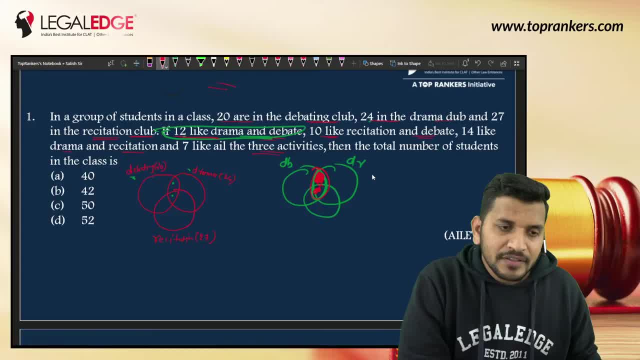 How much is it? 10 is here. How much is it? It is 10 here. We will write 10 here, 14 like drama and recitation. So drama and recitation will come here, And how much is it 14.. 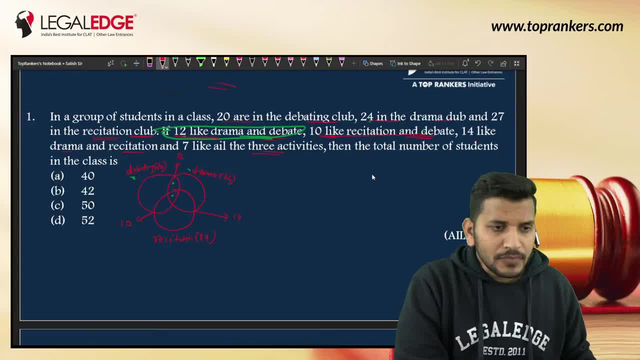 Ok, guys, After this, what we have to do? 7 like all the 3 activities. So 7 is liking all the 3 activities, So all the 3 activities will come here. We have to fill 7 here, Right? 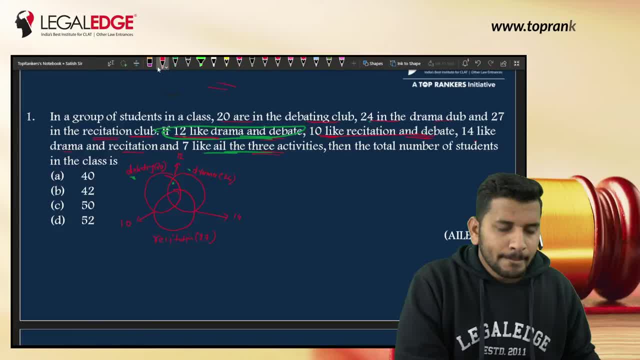 This is 7.. 7 like all the 3 activities. So I have written 7 here. Ok, Wait for 2 seconds. Some take. issue is coming Right Why they are taken. So you write the name and only take 1 option. 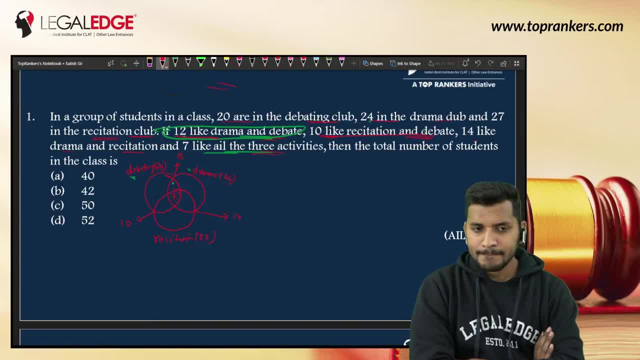 Right, Ok, Like this. Yeah, Okay, guys, so let's start. so what has been said? that debating has 20, let me tell you from the starting: debating has total 20,. drama has 24, recitation has 27,. but question: 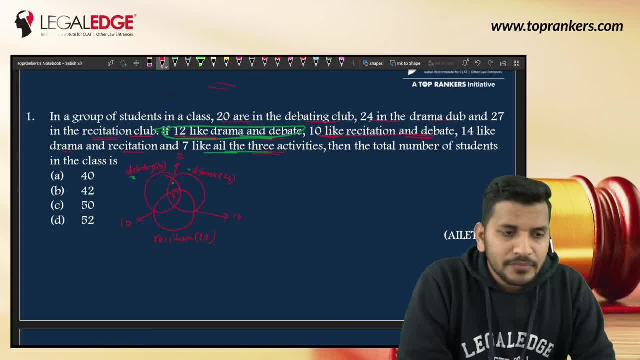 said, debating and drama has 12, and here drama and recitation has 14, and debate and recitation has 10, but all the three has 7,. all the three has. I am so sorry. now see what we do how. 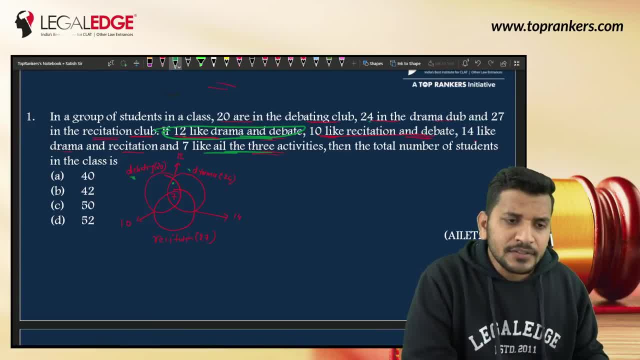 we find values. now the question is easy: case 12, this is 12, from 12, we will do 7 minus, we will get this value. from 12, we will do 7 minus, we will get this value. oh. 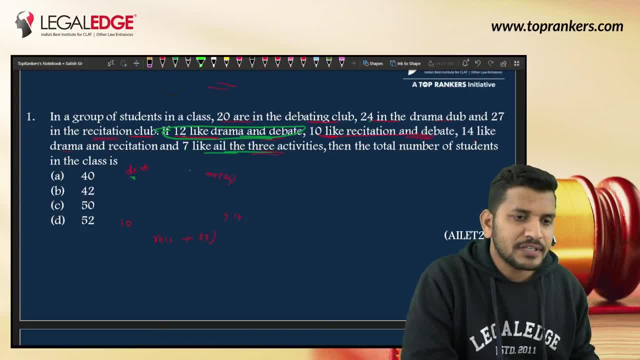 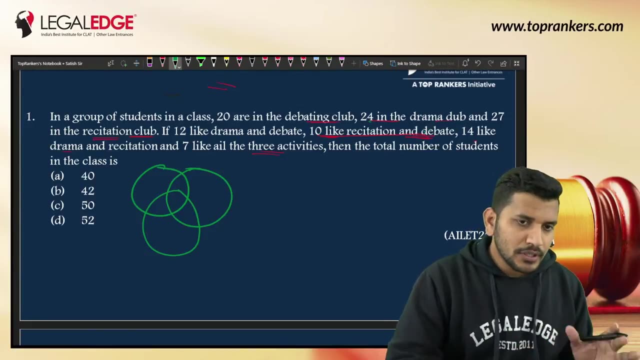 man, wait, it is gone, let's write again. no problem, it is gone, right, so we have all the values here. the question was easy. the question is easy. this is very easy. all the questions is easy. the question is easy if you know the concept of Venn diagram, if 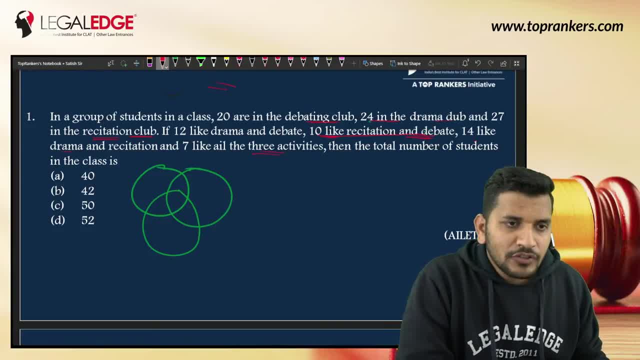 you know the concept of Venn diagram, then there is no big deal right here. I will fill the values. 20 are in the debating club, so 28 debate has been done. debate: how many are there in this? 20, 24 in drama guys. 24, 27 in recitation. these are 27,. all are there色. in drama, rings in drama, rings in drama. okay, so let's pull the public out of here. we'll become jacked on board. we'll move on in this tile. Geniele, minister, put it in the picture does not show any allegorical information. don't guess in this picture. 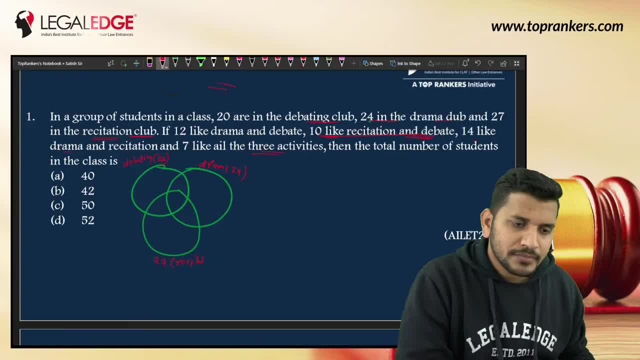 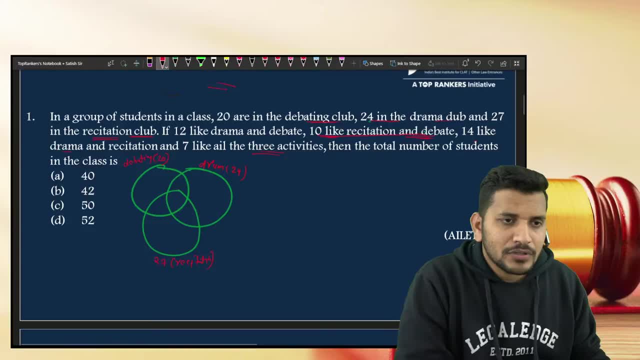 recitation: man, okay, 12 like drama and debate here. drama and debate, how many likes do you guys have to do? 12 likes. I will change the pen for a second. black color may not be visible, ok. white color will be visible, ok. so what is said? 12 like drama and debate. 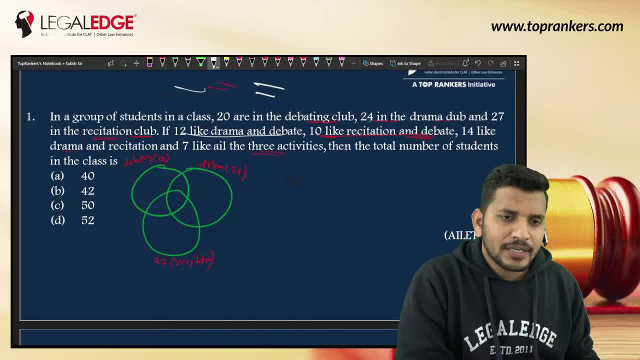 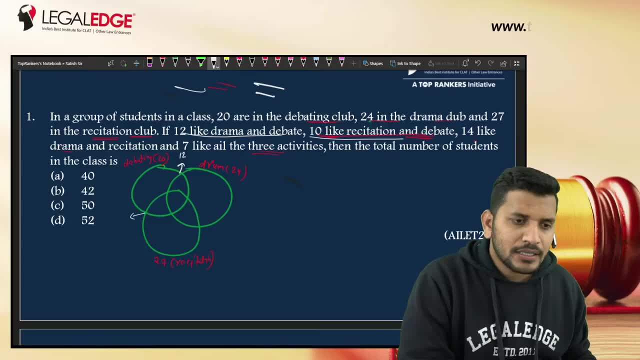 drama and debate: 12 likes. this value will be 12 and after that 10 like recitation and debate. how many likes do you have to do? 10 likes and 14 like drama and recitation. drama and recitation: have to do 14 likes. ok. 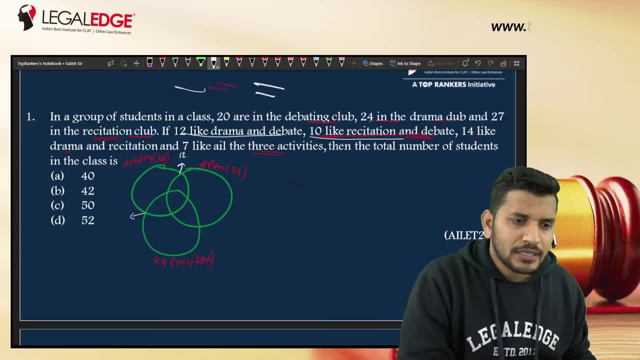 and 7, like all the 3, 7, like all the 3. ok, so, guys, from 12 we will minus 7. so this value will be how much? 5, 12 minus 7, because this one is complete 12, this one is complete 12, this one. 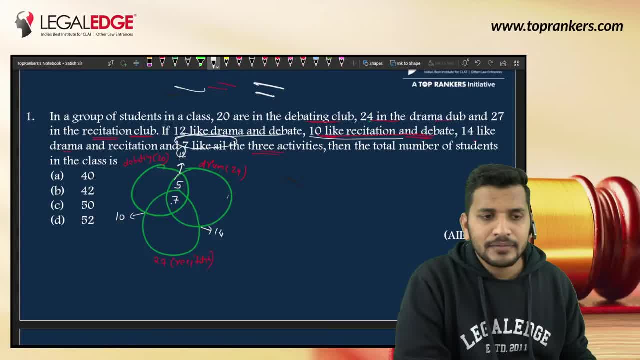 so from 12, I did 7 minus 5. now this 14 will be 12 minus 7. from 14, we will minus 7, so this will be 7. from 10, we will minus 7, so this will be 3. right now, let's take out more values. 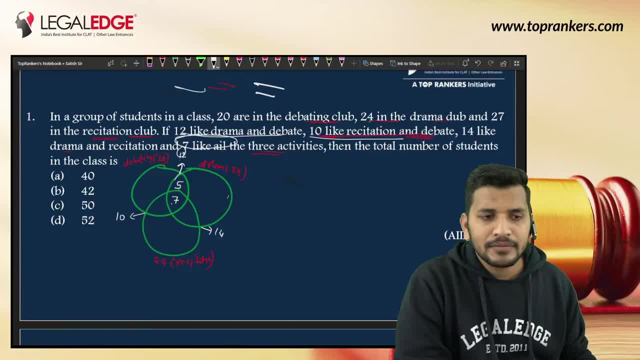 how will we take out the values of this circle? this is total 24. this big circle, this whole big circle is 24. so 7, 7, 14, 14, 5. how much is 19 right? 19, 24, 19, how much will be here, guys? 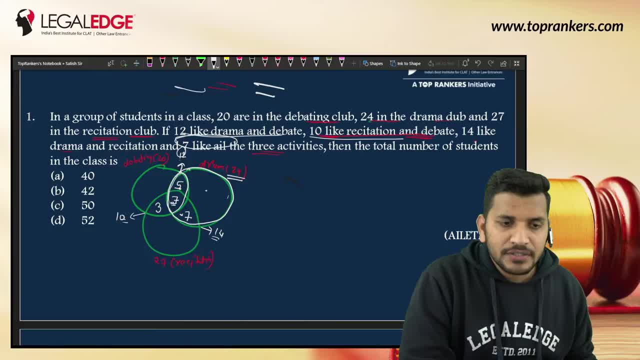 in 24, we will minus 19, so this will be the value. 5 will be ok and here we will see what will happen here. this is total 27, so here we will see what is the total: 7, 7, 14, 15, 16, 17. 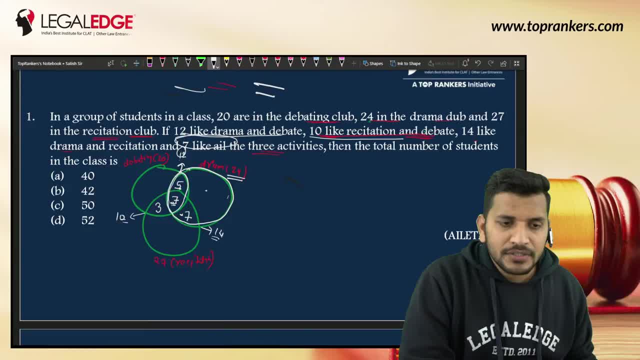 from 17. this will go, so this will be 10, right, and here the total is 20, so this is 15, so this will be 5. so what? it is saying? that then the total number of students in class is 5, 5, 10, 5, 15. 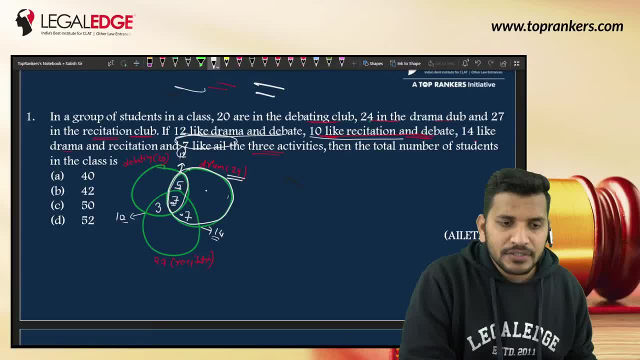 15 and 7, 3, 10, 25, 30, 30. something is wrong, guys. something is wrong in a group. 20 like debating club, so 20 like debating club. 24 in drama. 24 in drama- ok. 27 in registration. 12 like drama and debate. 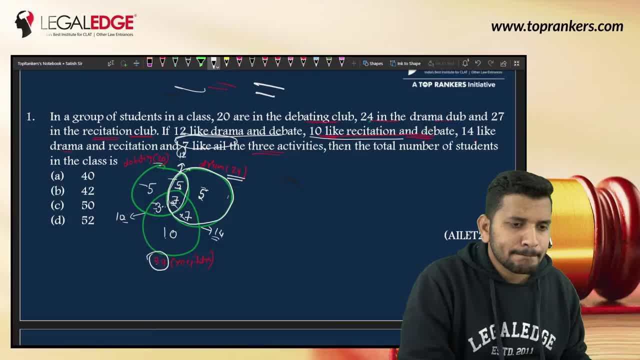 12 like drama and debate, right. so 12 or 7 like are the 3. so 12 minus 7. this is correct. this one is also correct. then 10 like registration and debate: registration and debate: who is doing 10 like? so 10. so 10 minus this will be 3. 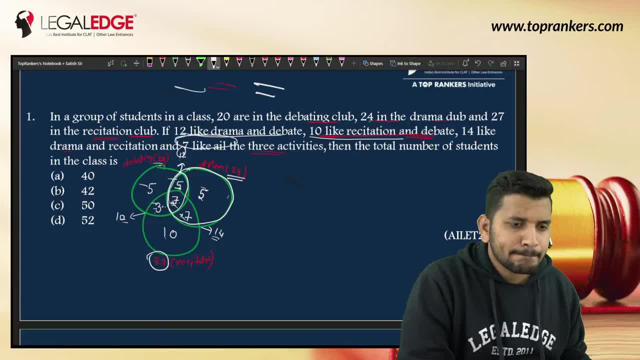 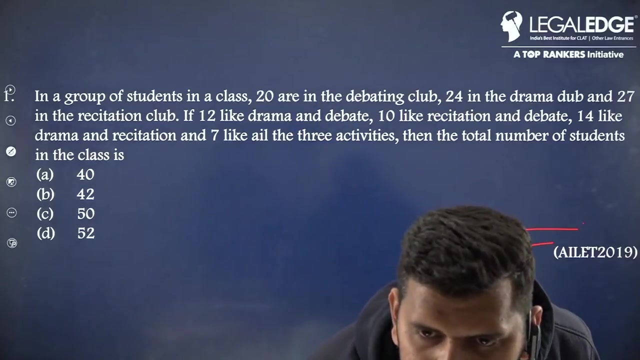 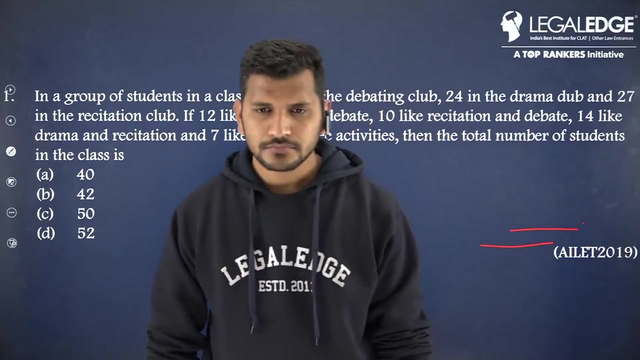 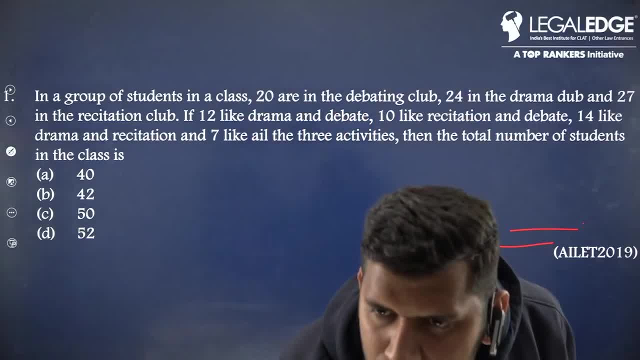 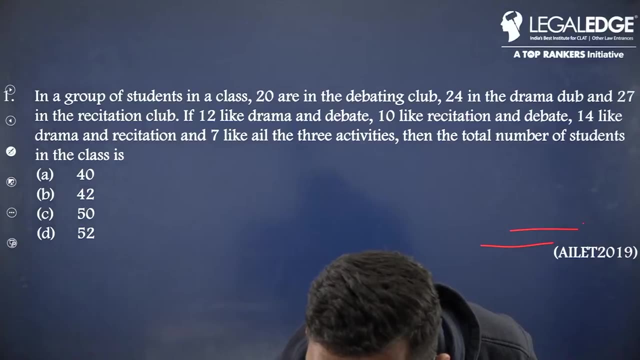 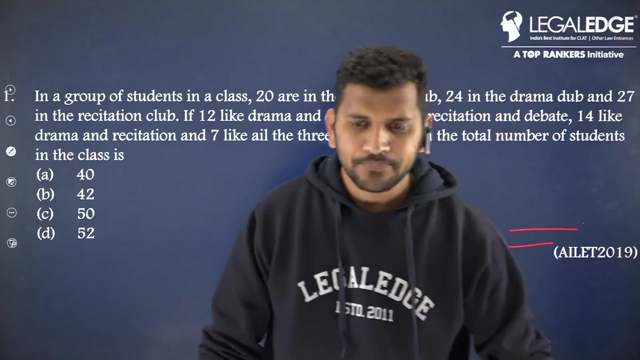 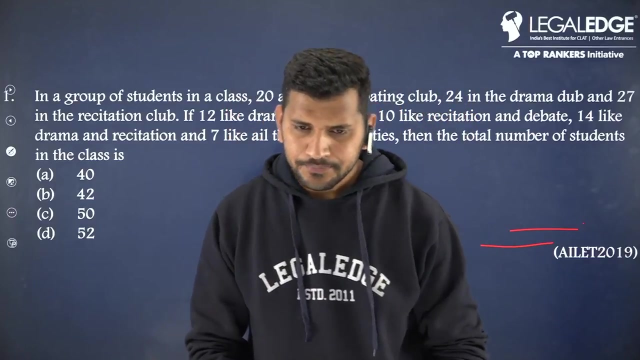 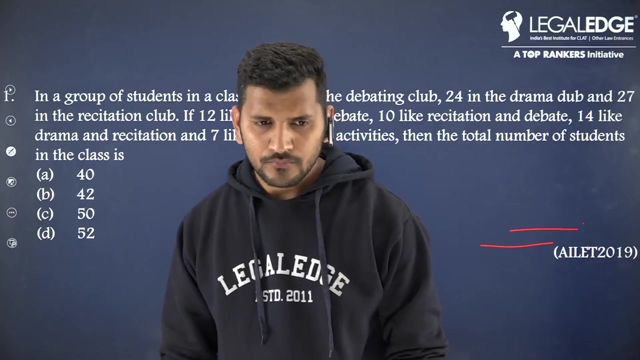 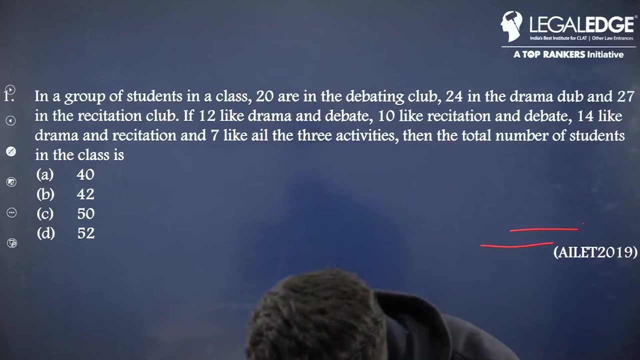 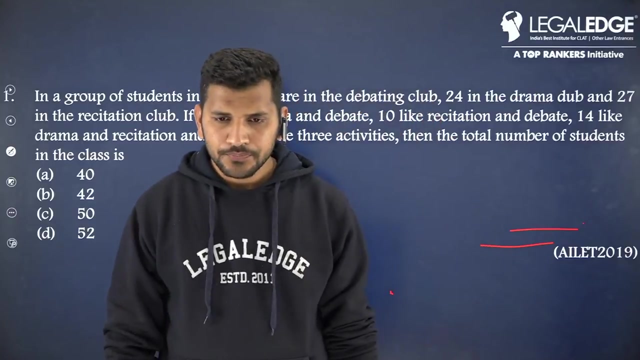 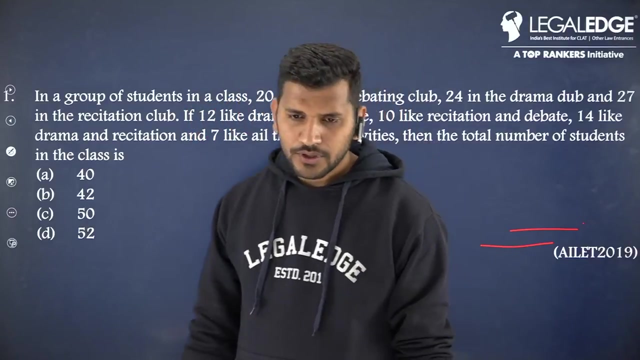 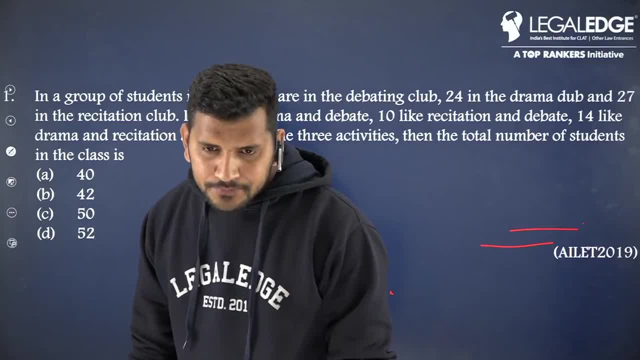 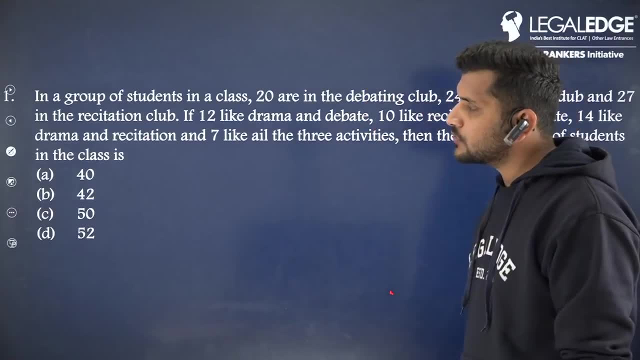 That's why, Now it will be clear. Good evening, Aparjita. The logo. Hello. So, guys, this question came to us in Elite 2019.. And we have to solve this question Right Now. how much time does it take to solve this question? 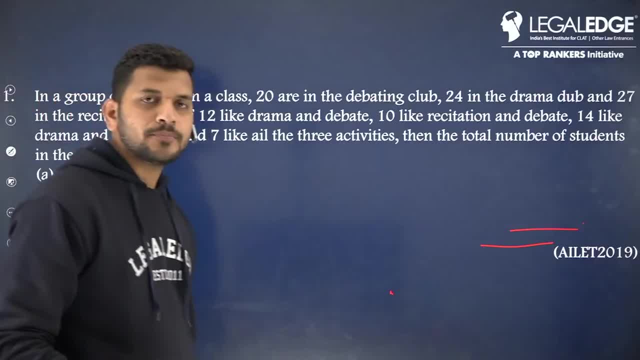 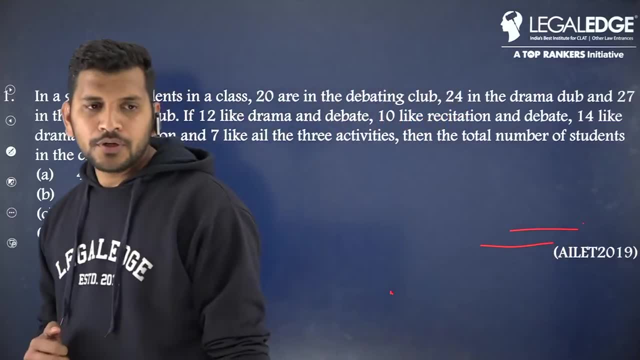 See, it doesn't take much time. We do it very fast. if you have practice, Let's see. That's why I always tell you that you should practice, Right, Okay, uncle Abhijeet, Hi, Hello, So we have to practice. 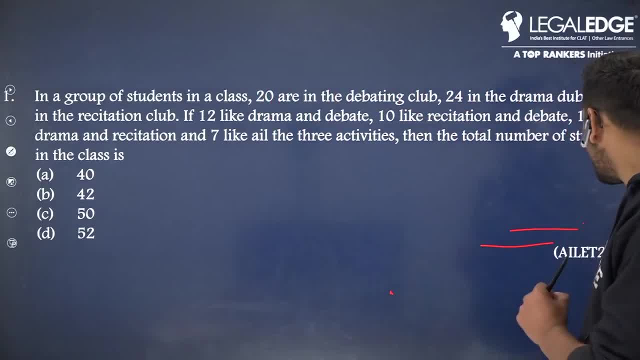 It won't work without practice. That's why we have to practice a lot. Now. this question came to us in Elite 2019.. What is this question? In a group of students in a class, 20 are in the debating club, 24 in the drama club. 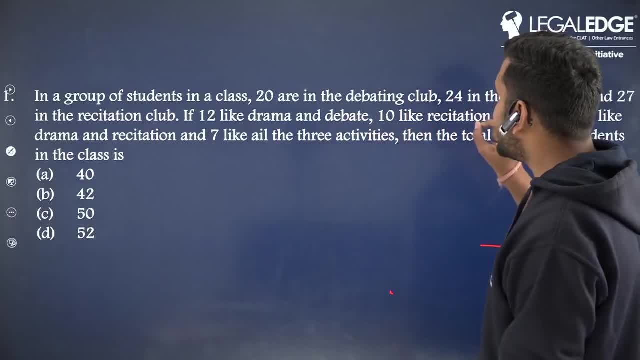 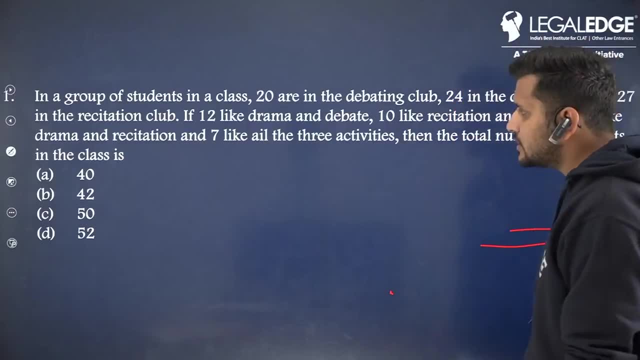 and 27 are the recitation club. If 12 like drama and debate, 10 like recitation and debate, 14 like drama and recitation and 7 like all the three activities, Then the number of students. You must be thinking that, sir, the question is very big. 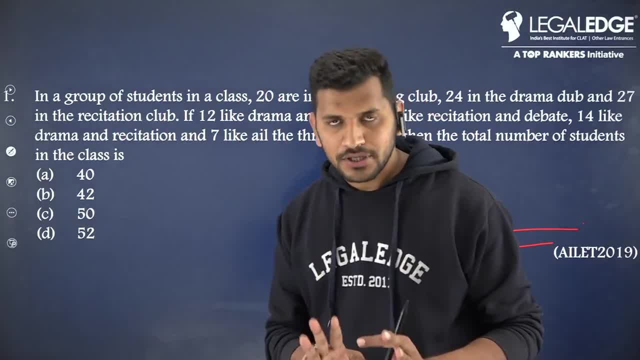 It will take more time. It won't take this question time. Okay, See what to do in this. We have to solve it with a Venn diagram. You must have understood this much, So I make a Venn diagram here. 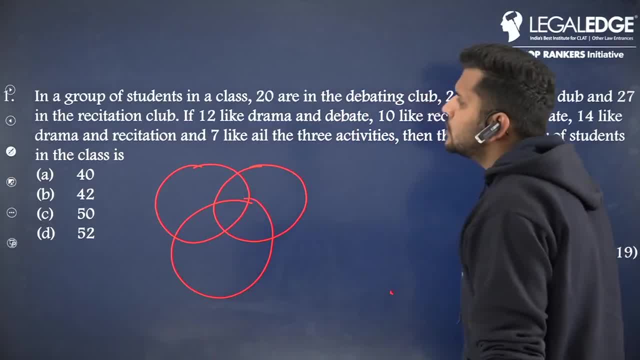 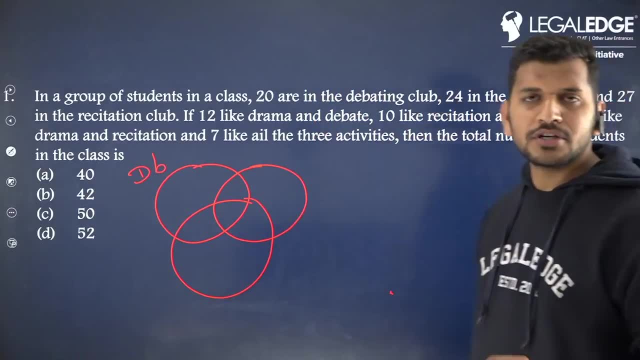 Okay, We make a Venn diagram here. So what did I say earlier? There is a debating club, So I made a debating club. DB means debating club. Always write it in short form. Right, You will write it in short form. 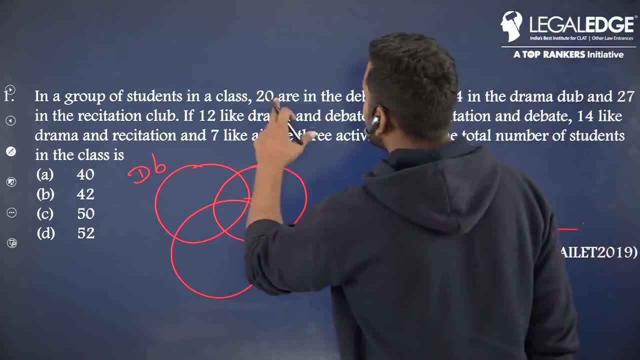 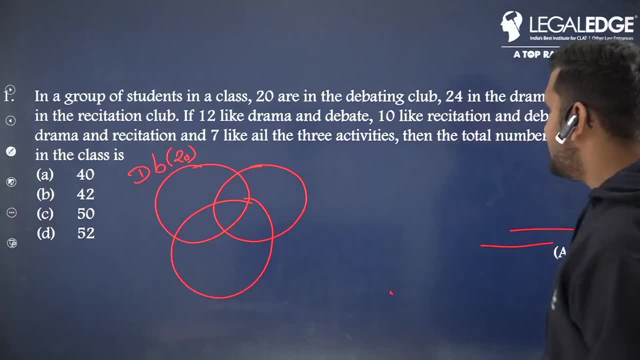 DB means debating club, And how much is there in this? 20 are in the debating club. So how many students are there in this? Total students are 20 in the debating club, 24 in the drama club. Now, suppose this is the drama. 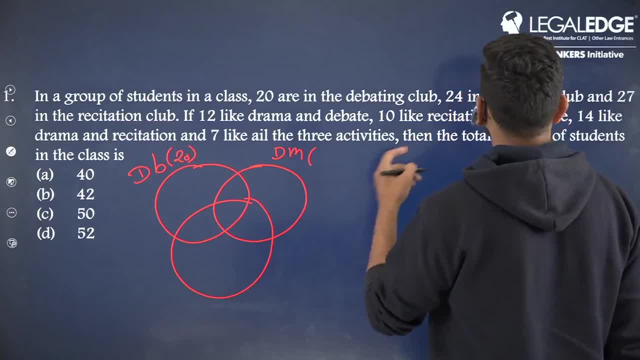 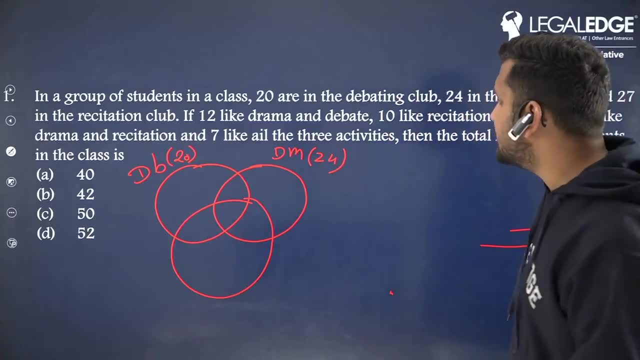 Right, I have written the drama as DM. And how many are there in the drama club? 24 are there in this And 27 in the recitation club. Right, What is 27?? There are 27 in the recitation. 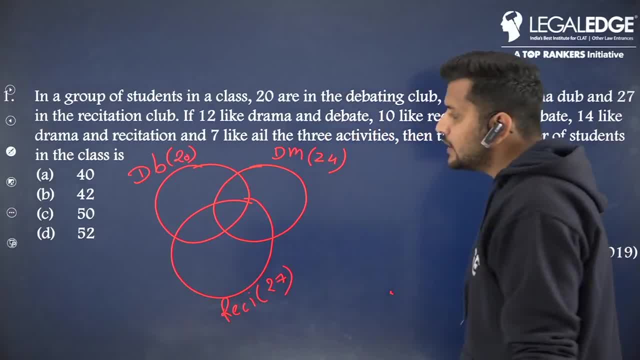 Right, How many are there in this? There are 27 in the recitation. This is the total number. Total number Because this whole circle, You can see this circle, This circle tells you the drama, This one tells you the debating. 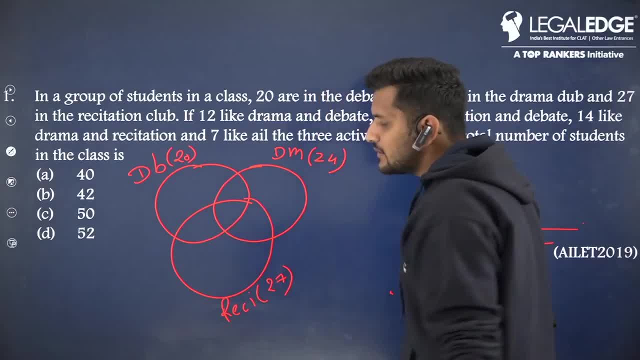 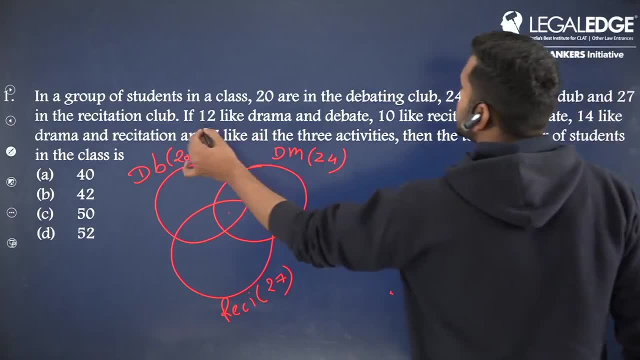 This one tells you the recitation. Understand it. This whole circle tells you The mid one has this value. This tells us about all It is saying. It says that if the 12 like drama and debate, What does 12 like? 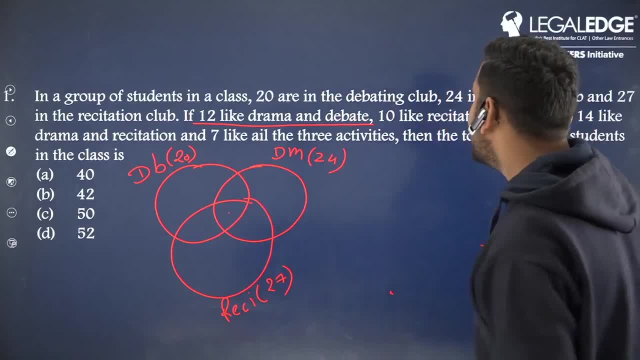 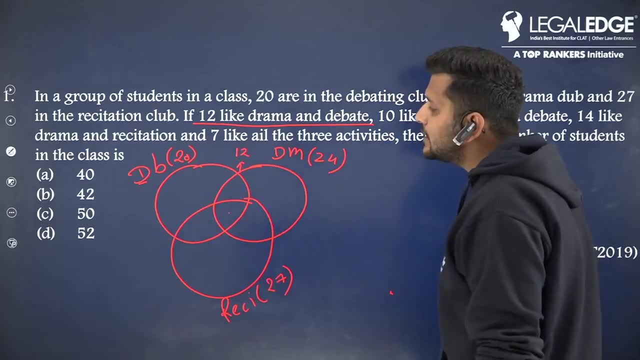 Drama and debate. So 12: drama and debate. This has been about debate, This has been about drama, So 12: like Here I have written 12.. For the drama and debate, This whole circle will be for debate. 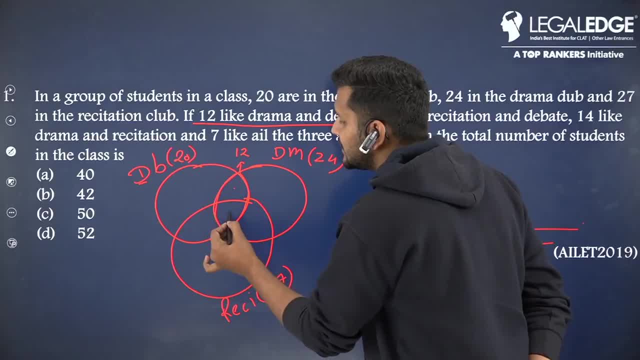 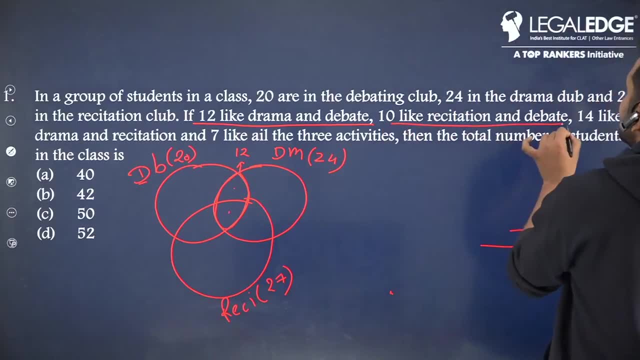 This whole circle will be 12, not this one or this one. this whole circle will tell you 12.. Let's move ahead. 10 like recitation and debate. What does 10 like? Recitation and debate? This is recitation and debate, so this value is 10.. 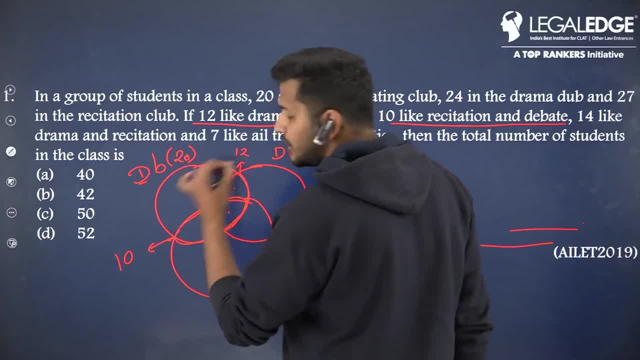 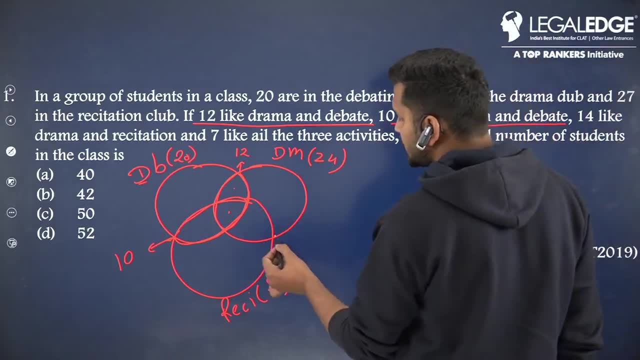 This whole circle will go till here. This circle will go till here. you will call this 10 like. After this, 14 like drama and recitation. this drama, this recitation, this 14 value will come here And the question says 7 like all the 3 activities. 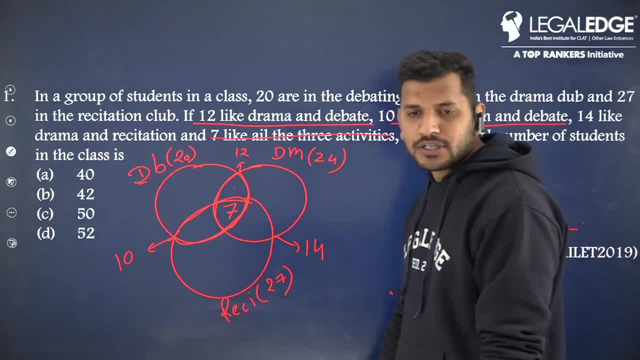 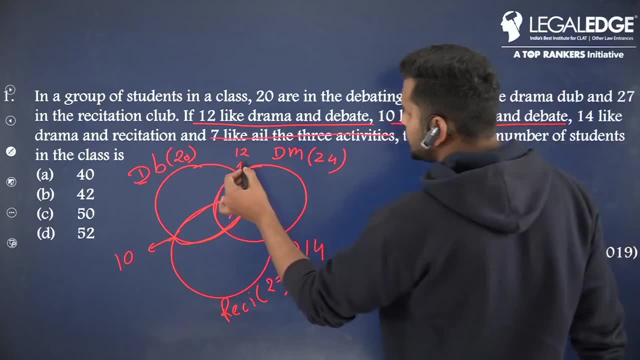 so 7, like all the 3 activities. so we will put 7 here. So this is our Venn diagram. it was a 3 Venn diagram question. now it is very easy to do what to do. See here: this value is 12, so out of 12,, if we minus 7,, how much will it be? 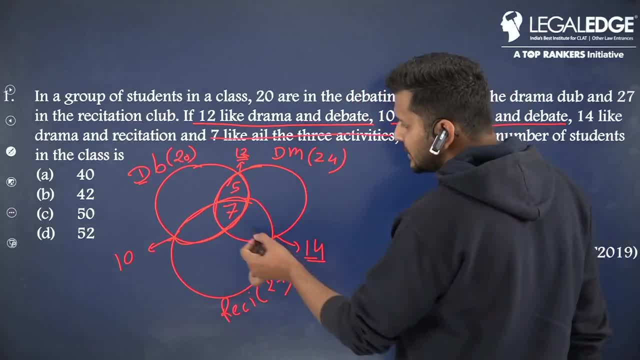 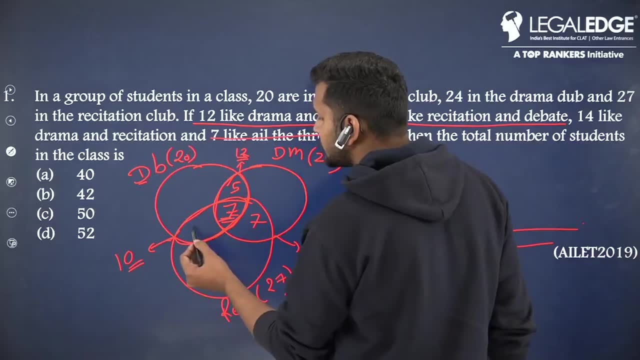 It will become 5, absolutely right. But here, 14 value is given out of 14, if we minus 7,, how much will it be? It will become 7, absolutely right. Here, guys, 10 value is given out of 10, if we minus 7, how much will it be? 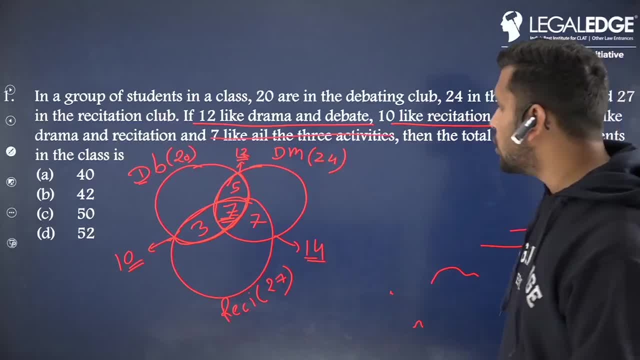 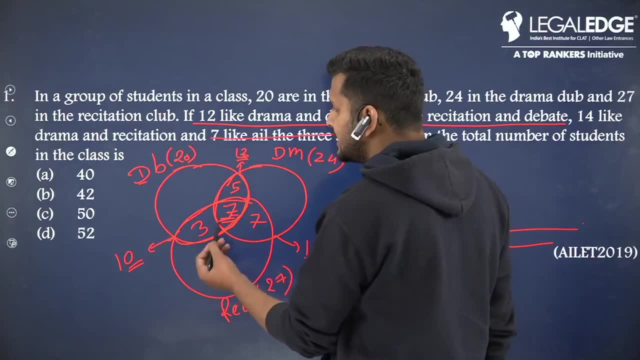 It will become 3, our values have come like this And now we have to remove this debate one. so this whole circle is made up of 20.. How much is the whole circle, guys? It is made up of 20, so out of 20, we will minus 3 plus 7, 10 plus 5, 15.. 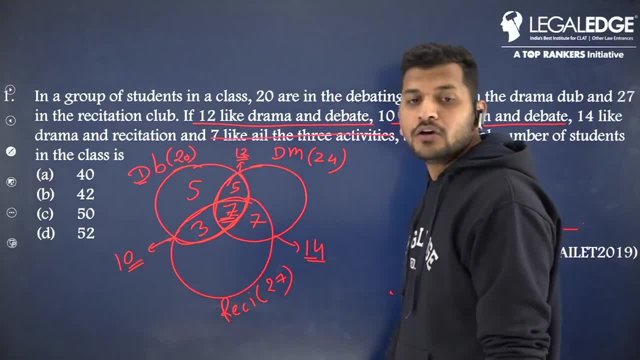 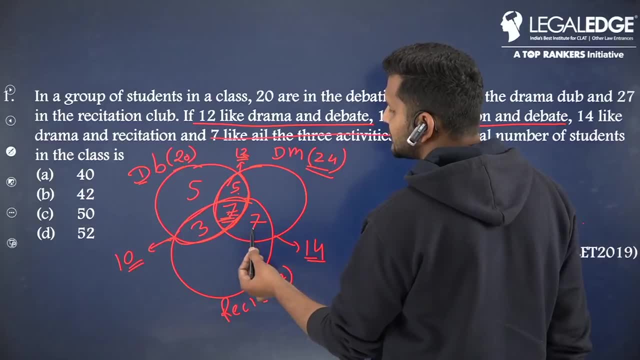 So 20 minus 15, how much will it be? It will become 5 here. okay, After this, see here this 24, from this 24, we will minus this one: 5 plus 7.. 7 plus 7, how much will it be? 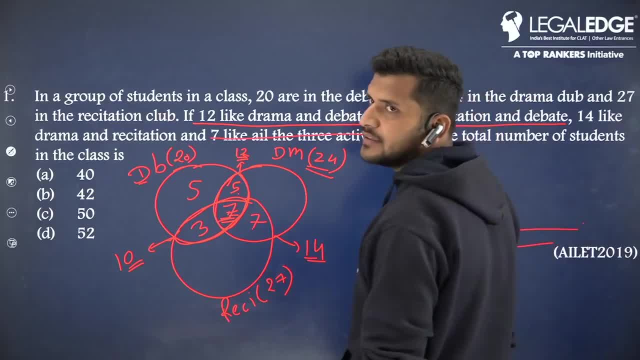 12 plus 7,, how much will it be? 19.. So from 24, we will minus 19. Here it will become 5.. And after this- see here also- we can remove the value. here also, How much will it be? 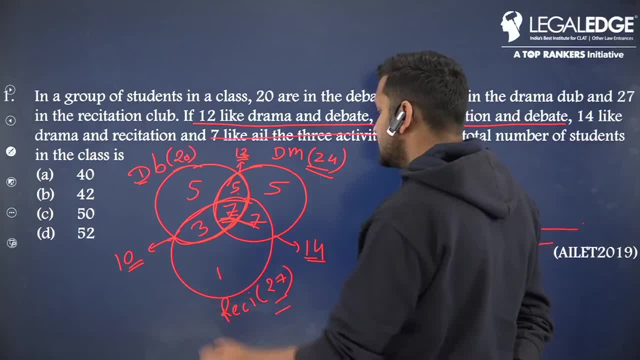 From 27,. how much will it be 7 plus 7,? how much will it be 14,, 16,, 17,, 18.. 18 minus 14, 15,, 16,, 17.. So it will become 10, right. 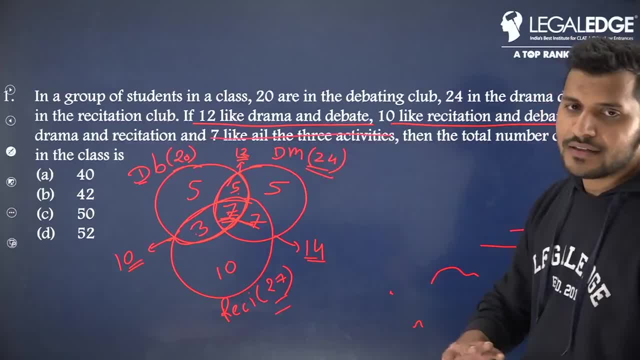 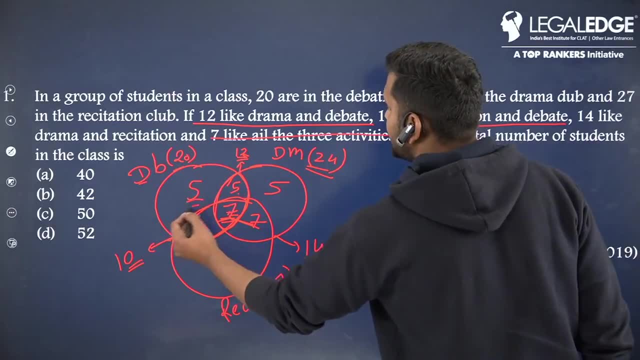 Now it is saying that the number of total number of students. what was the total number of students in the class In the student diagram? the total number of the total number of students, What is the total number of students? See 5 plus 5,, 10 plus 5, 15.. 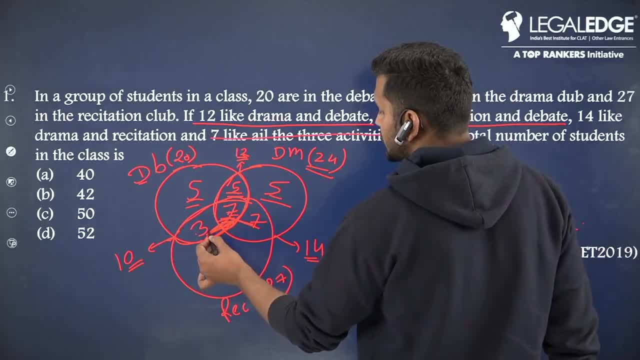 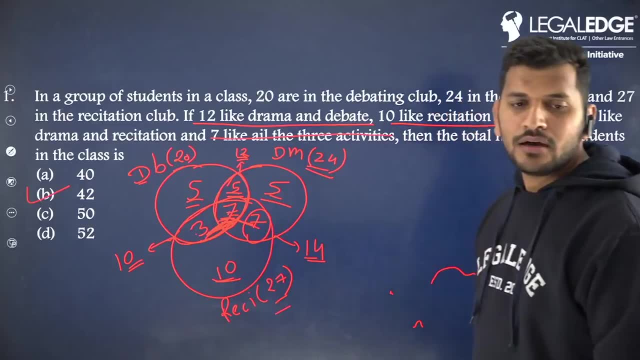 15 and 3 plus 7, 10 will become 25.. 25, 35.. 35 plus 7, 42.. So how much will be the answer to this? 42 will be the answer to this question. 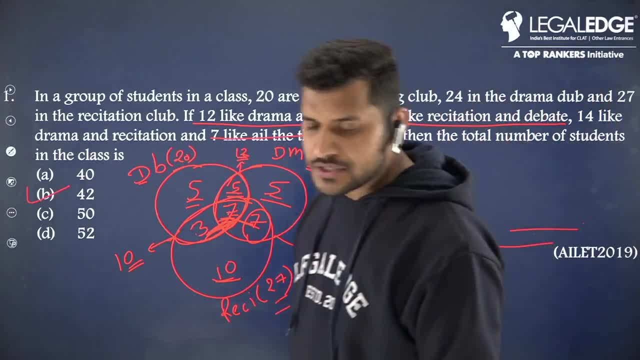 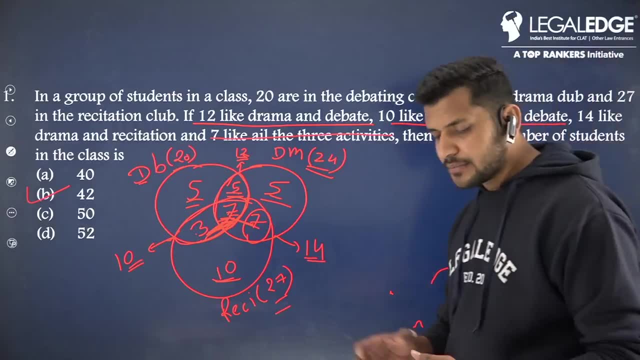 Is it clear to all of you? Good evening. Yes, Vanshika, option B is coming very good. So, guys, option B is also coming here, So it does not take time to explain to you. I took so much time to explain. 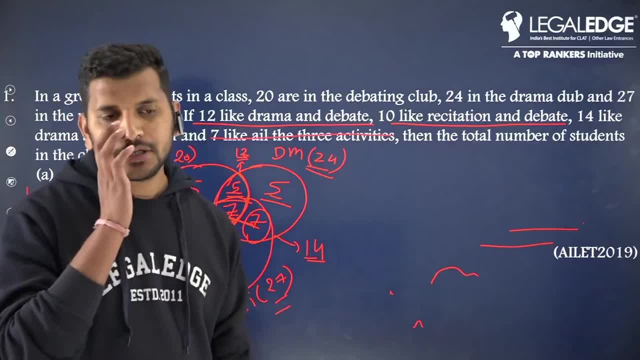 But when you do it in the exam it should not take so much time. there We solve it with a lot of speed. We do not write it completely, We write it in short form. Guys, let's move towards the next question. 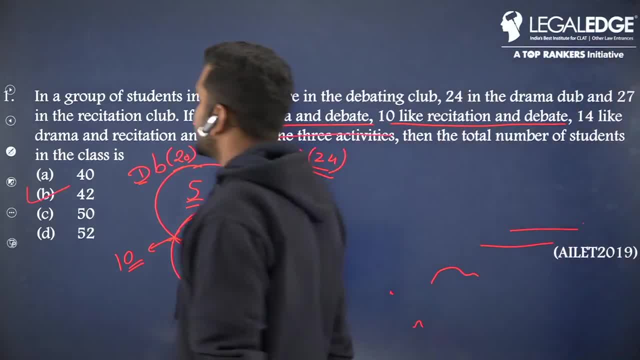 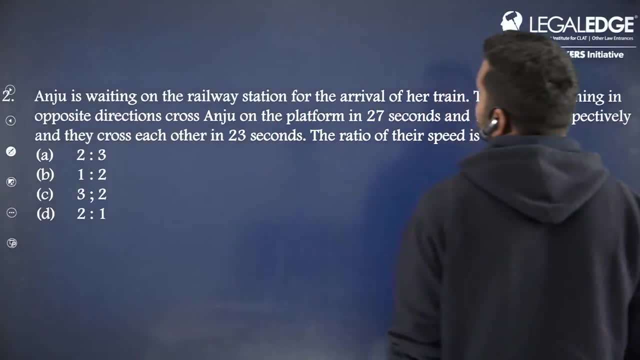 Okay, This question must have been done. Okay, This is second. Anu is waiting on the railway station for the arrival of a train. Anju is waiting on the railway station for the arrival of a train. Two trains running in the afternoon. 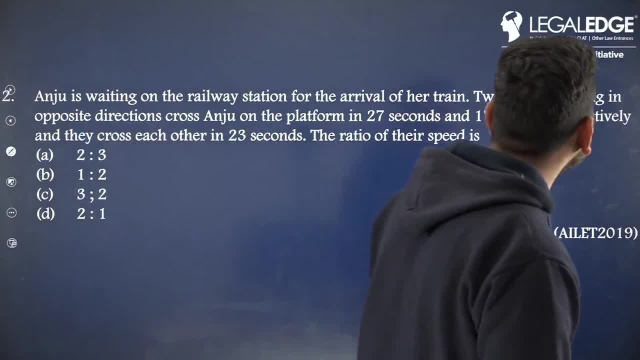 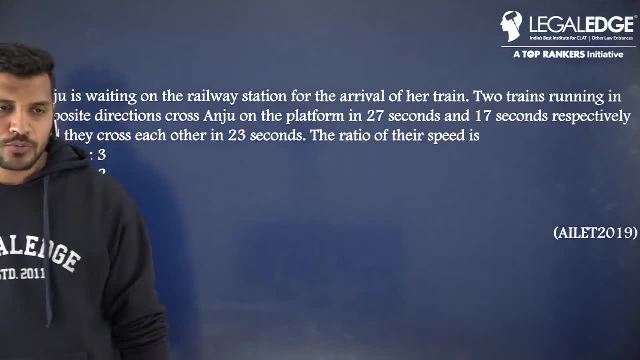 They run opposite direction, Cross Anju on the platform in 27 seconds and 17 seconds respectively, And they cross each other in 23 seconds. The ratio of their speed? Guys, we have to tell the ratio of their speed. The question is good. 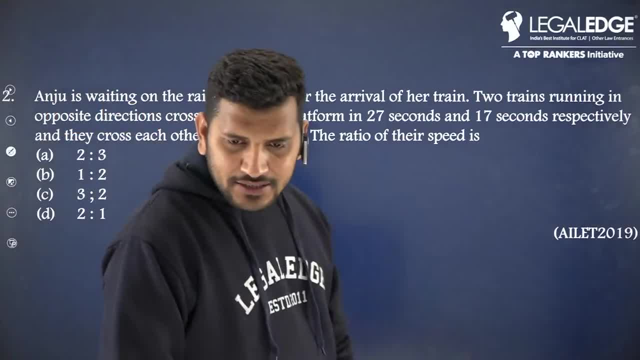 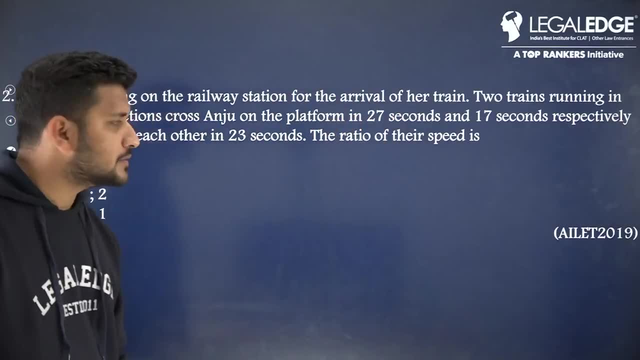 Give answer to it quickly. I am waiting for you. Scientists, Mr comrade. Yes, scientists. Okay. Okay, this was the answer. Okay, this is a good question. What does the question want to say? Anju is waiting for the arrival of an Orbit on the railway station. 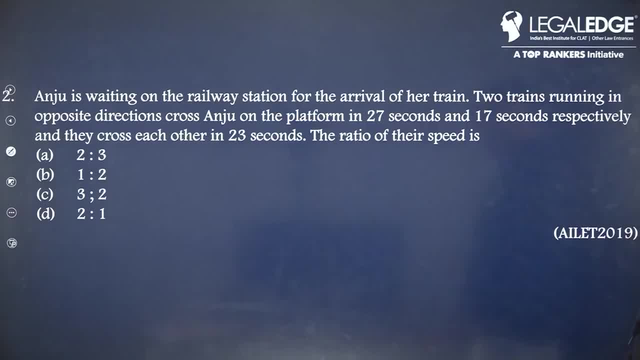 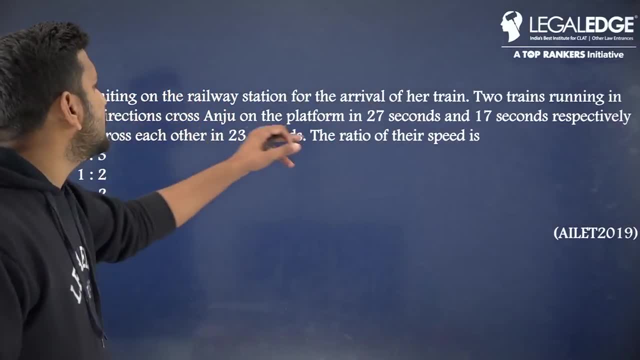 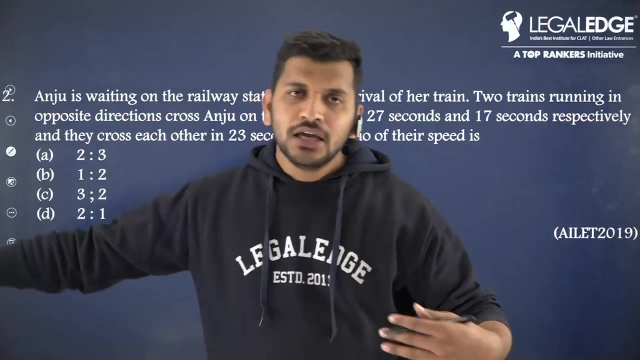 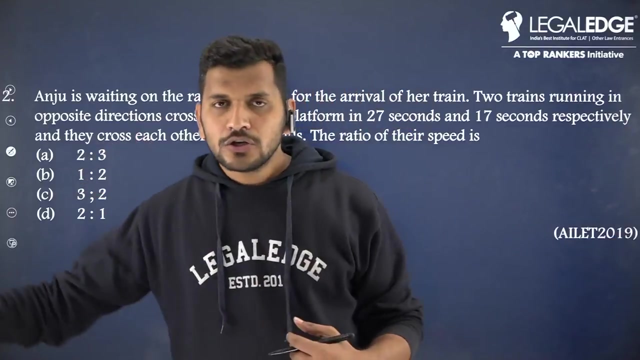 Waiting on the railway station for the arrival of the train. Two trains running in the opposite direction cross Anju. Suppose I am standing here. one train comes from this side and crosses me. I am standing on the platform. one train comes from this side and crosses me. 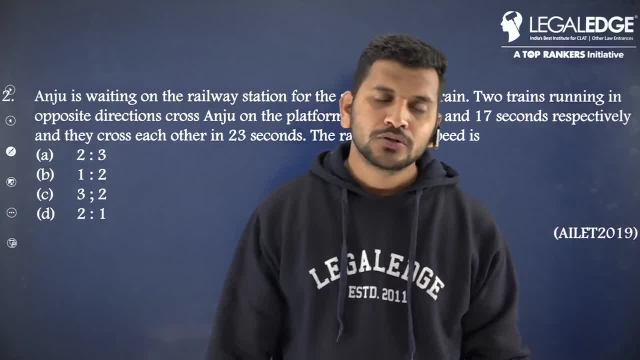 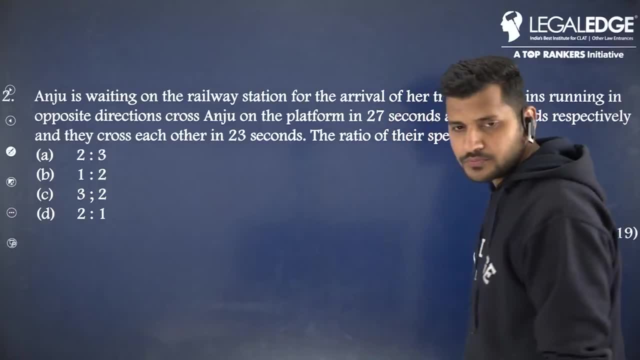 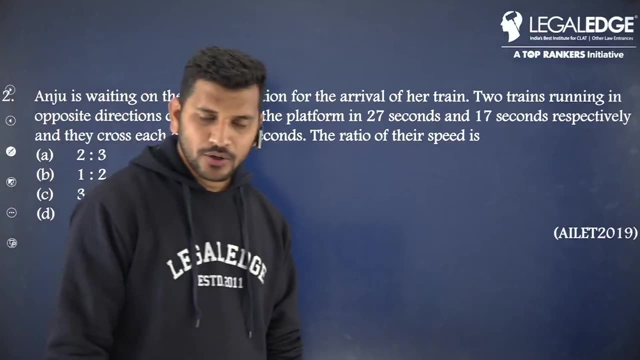 Two trains cross me and cross each other. So this is the question. It was a good question. Here you have to find the speed ratio. Will anyone tell the speed ratio? Everything is going well in life. I think you can't see the question. 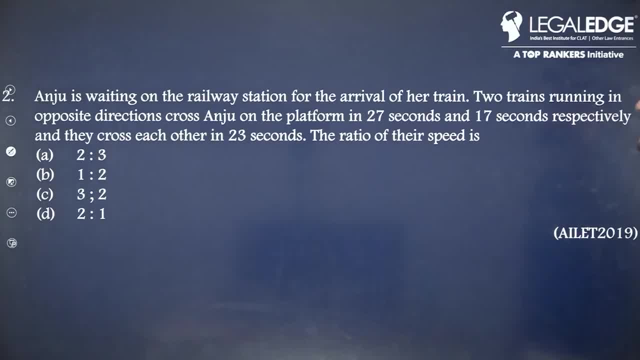 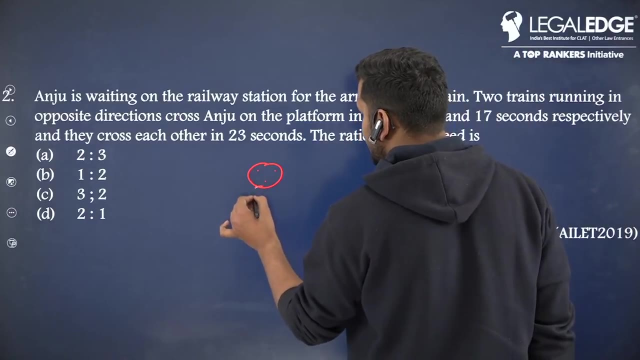 Now you will see the whole question. So how to solve this type of question? Let's start. Suppose Anju is waiting at the railway station. I will make this Anju Here. Anju is waiting at the railway station. Right, this is Anju. 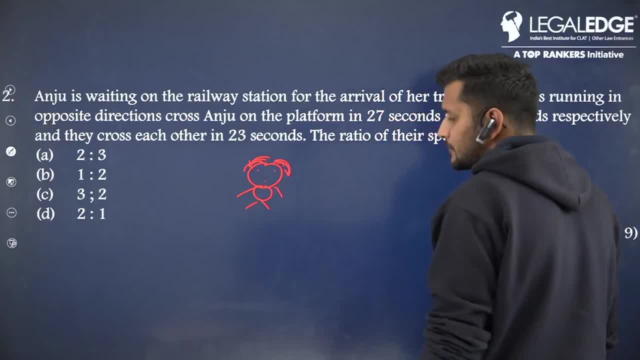 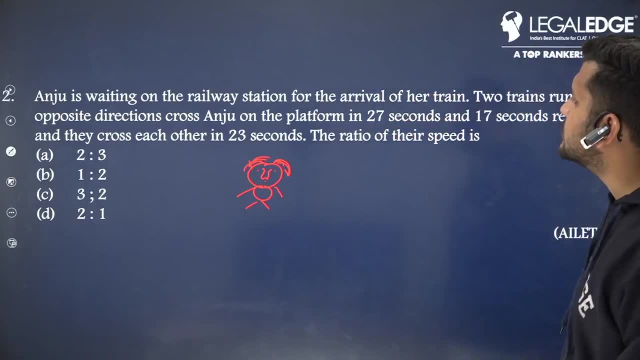 Anju was waiting here. Let's make it better. What was Anju doing here? She was waiting at the railway station. Two trains crossed her. Two trains running in the opposite direction cross Anju. One train was coming from this direction. 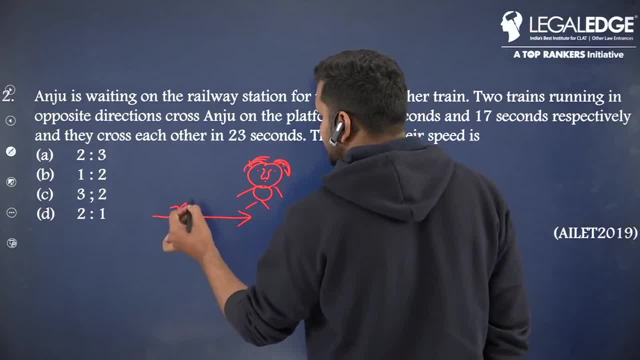 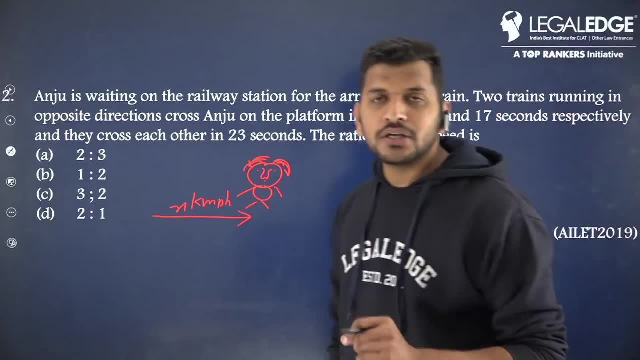 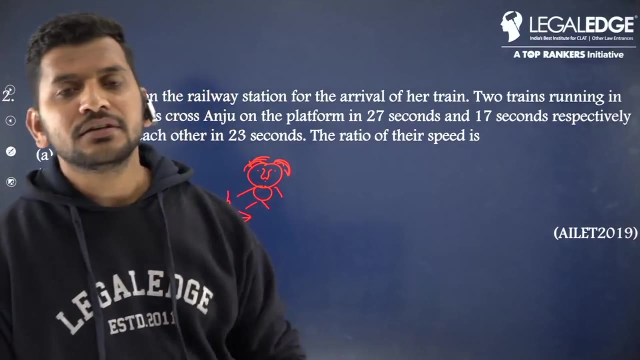 One train was coming from this direction. The speed of this train was x km per hour. Right, It was coming from this direction. Whenever you get the question about the train, Whenever you get the question about the train, If any train crosses a person, a pole or a tree, 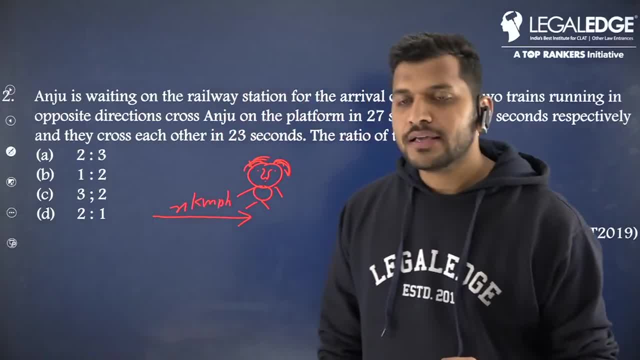 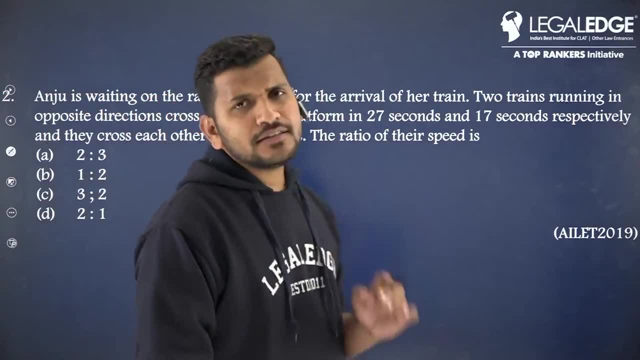 Then how much distance will it travel? It will equalize its length. Suppose the length of the train is 200 meters. I am giving an example. One train's length is 200 meters If it has crossed any person, a pole or tree. 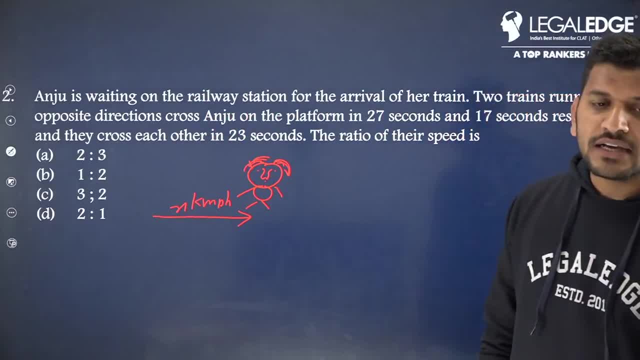 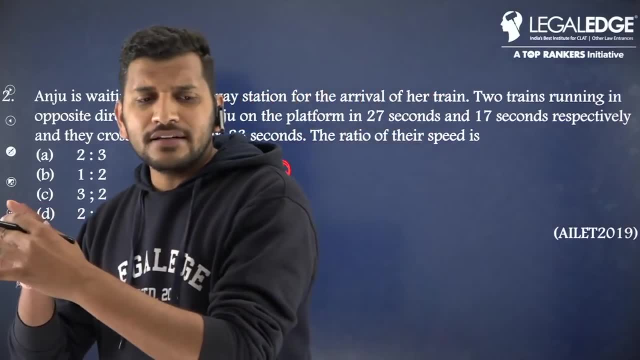 if any person, a pole or tree has crossed a train. If any person, a pole or tree has crossed a train, Then how much distance will it travel? You will say 200 meter long train crosses a man in 20 seconds. It means the distance has travelled 200 m. 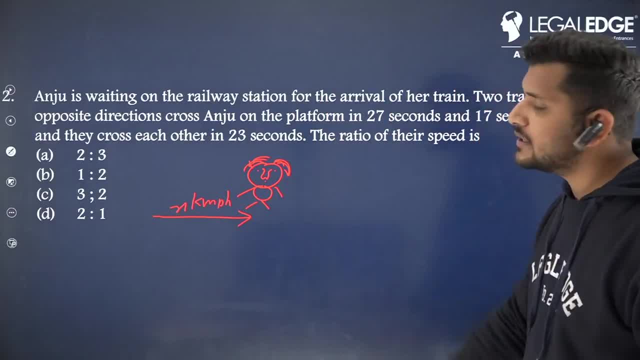 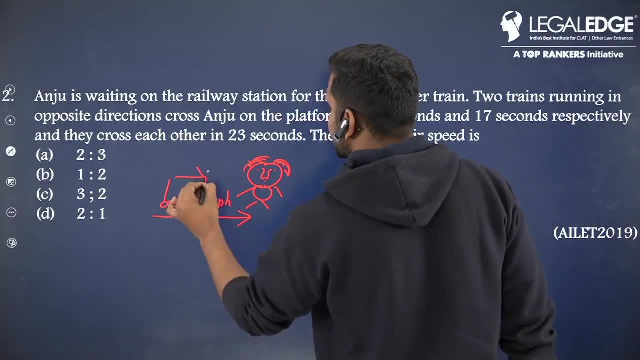 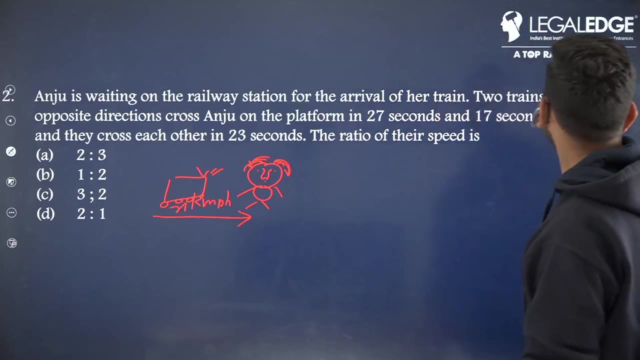 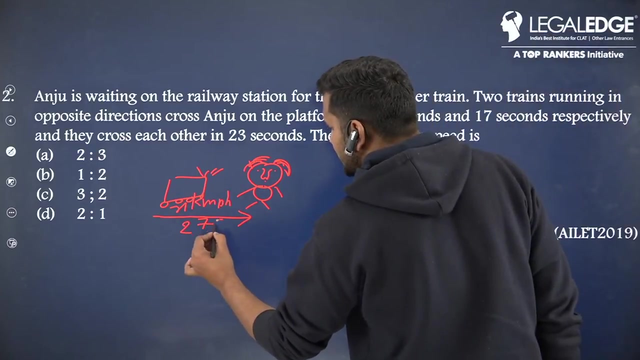 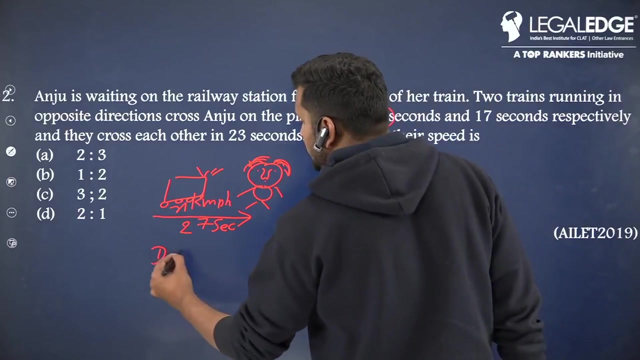 It will travel the equal of its length. So for you, I want to know the distance. Suppose this train was coming, It was coming from this direction with the speed of x km per hour. This is the train. The train is coming like this, with the speed of x kmph. it has crossed this Anju. how many seconds did it cross? it was said in the question, two trains running in opposite direction. the platform it has crossed in 27 seconds. this train has crossed Anju in 27 seconds. so how much distance did it travel? guys, we will see. we know distance is equal to speed into time. the speed of the train was x and how much time it took, 27,. so how much distance did this train travel? 27 seconds? 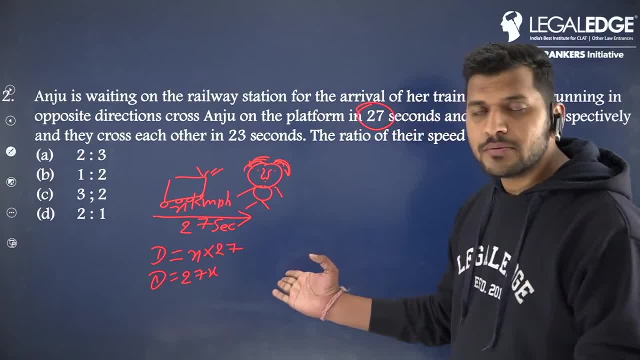 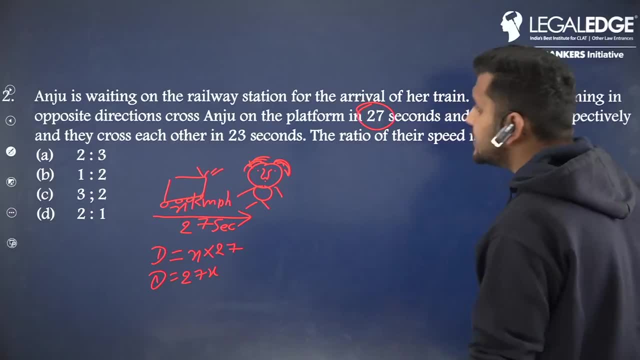 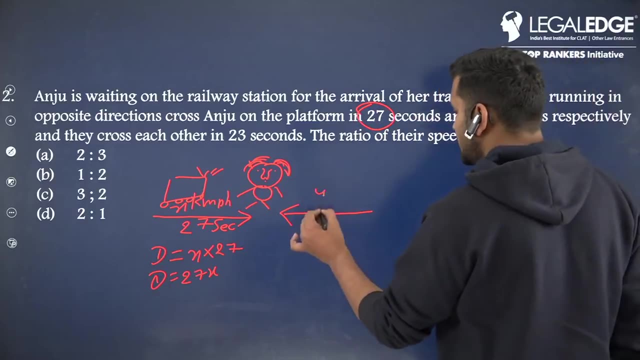 x distance travel. right, it must have traveled this much distance and this is what I told you. when the train crosses the person, then the distance is equal to the length of itself: 27x. okay, this thing is clear to us, sir. when the train from this side, if this train has crossed this Anju, and the speed of this train was y kmph, right, and how many seconds did it cross? it has crossed in 17 seconds. so, when this train has crossed this person, how many seconds? 17 seconds, so it has crossed this person. 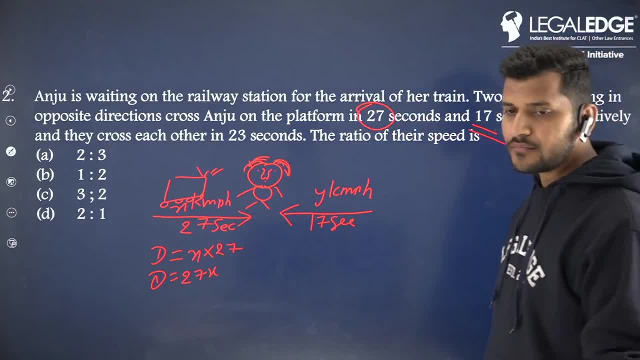 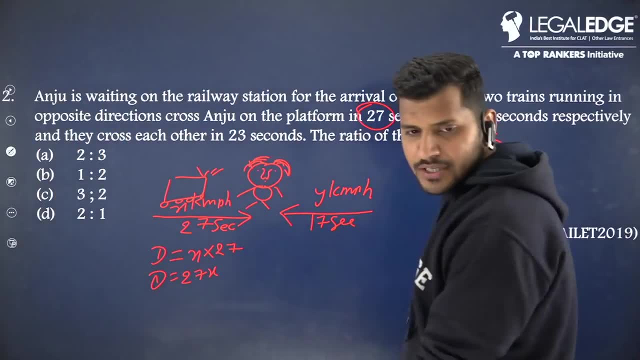 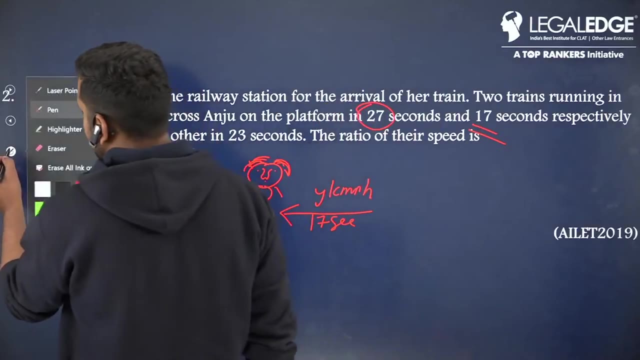 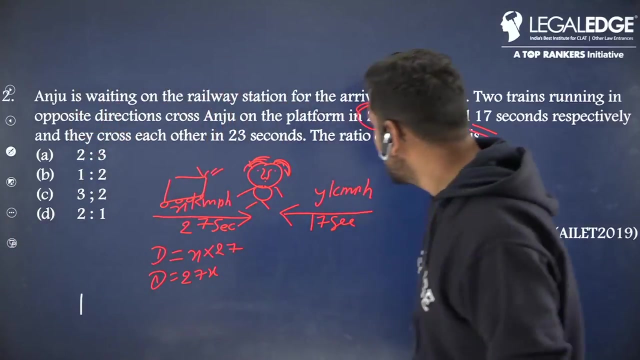 will this train also travel the same distance as his own length or not? absolutely, sir. use white line marker. use another marker. oh, we will have to use another marker. okay, I do understand this. I have a lot of color in my life, so we have to keep the color of the pen white if you want it. so now it is white, okay. so, guys, how much distance will be here? distance is equal to speed into time, speed is y, and how much time is it taking? 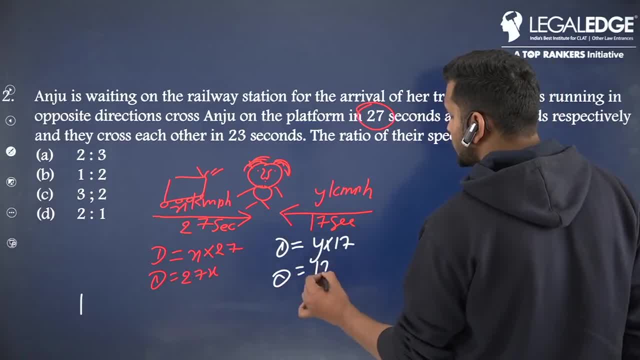 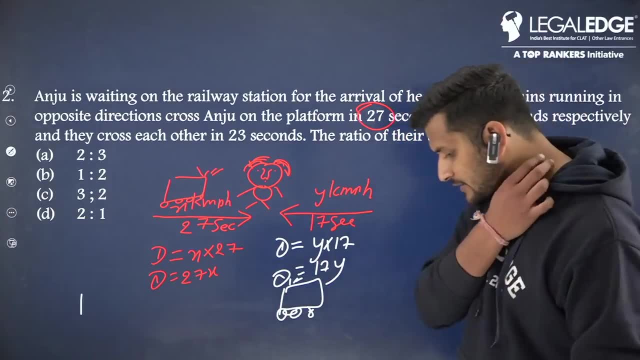 17,. then what will be the distance here? 17y. So what will be the length of this trend? guys, The length of this trend which is going in this direction, it will be 17y. Why, When the trend crosses a person, what is the distance? It is equal to its length, right? So its length. 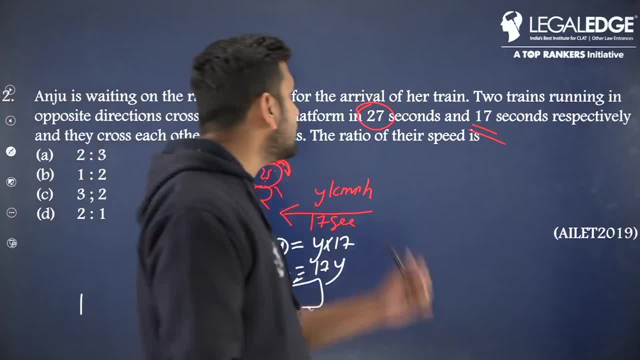 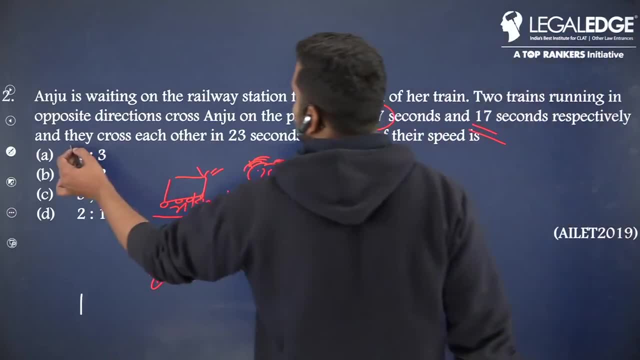 will be 17y, it will be 27x. Now, what is the question saying When these two trends? what is it saying When these two trends? what is it saying These two trends will cross each other and they cross each other. They cross each other in 23 seconds. This means. 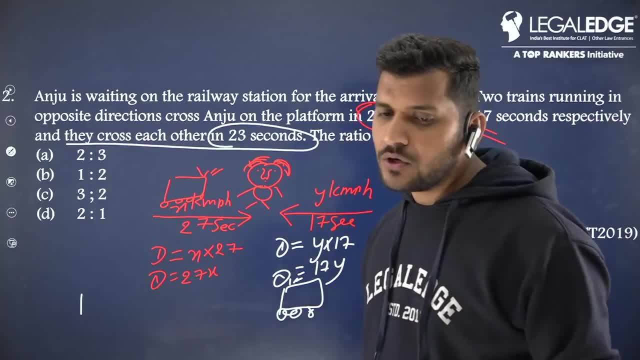 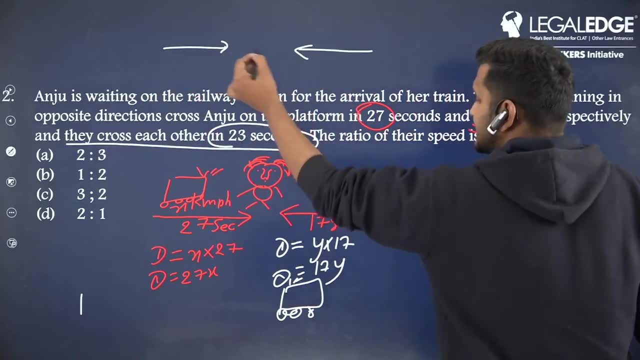 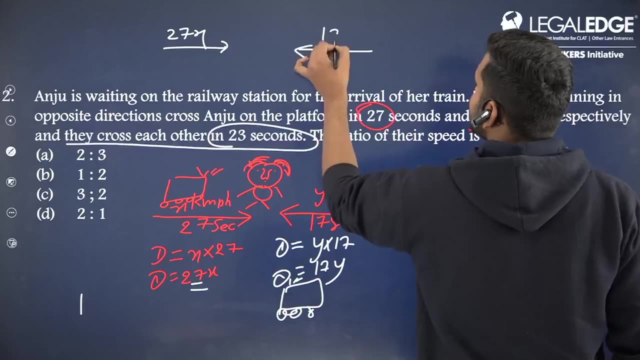 that both the trends cross each other in 23 seconds. A trend was coming from this side and a trend was coming from this side, right? How much is the distance of this trend? 27x. this is the length. And how much is its length coming from this side? It is 17y, These two. 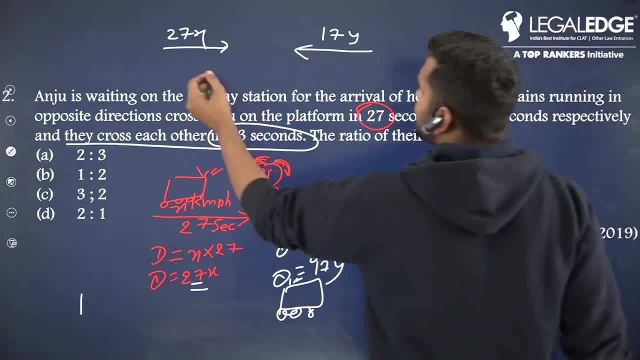 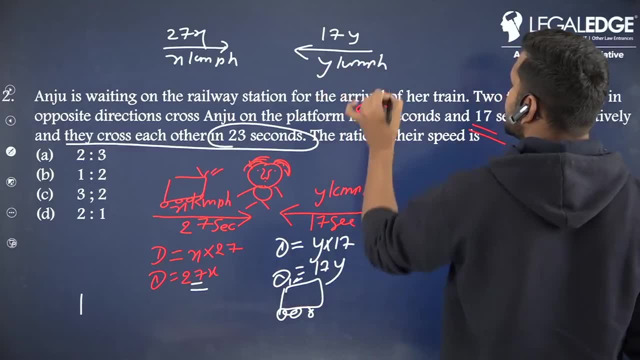 will cross each other in the opposite direction, And we know its speed: it is x km per hour. We also know its speed: it is y km per hour. Understand this carefully. We know its speed is y km per hour. Both are coming in the opposite direction. If they cross each other, then 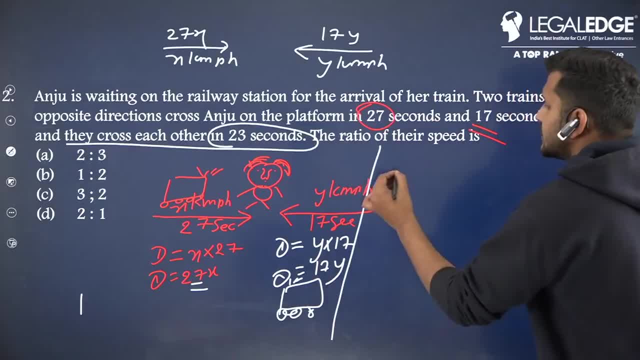 what will be the crossing time? So, sir, we know the time. Time is equal to what? Distance upon speed, What happens? Distance upon speed, And guys, both are crossing each other in 23 seconds. So time will be 23 seconds. How much will be the distance When two trends? 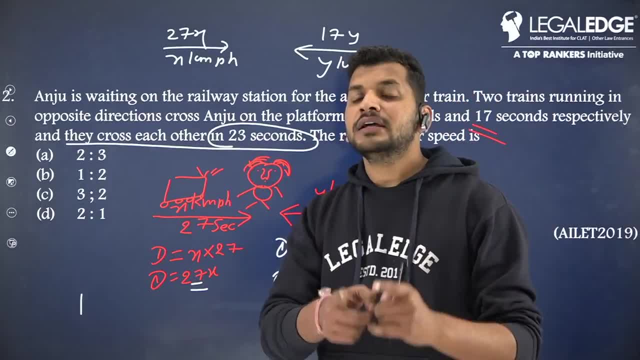 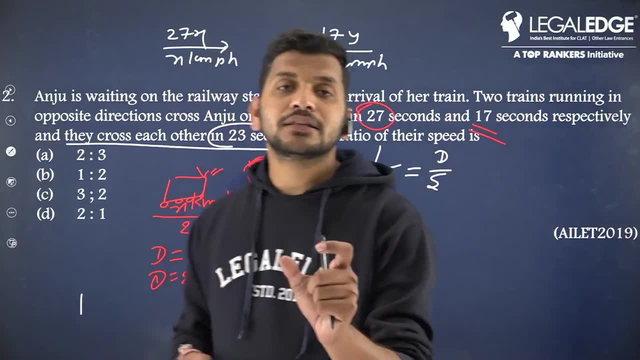 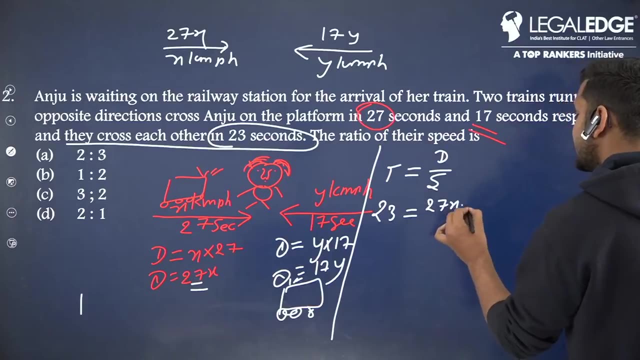 cross in the opposite direction or in the same direction, distance will always be added right. When two trends cross in the opposite direction or in the same direction, distance will always be added. Distance will be 27x plus 17y. So distance will be 27x plus 17y, And guys, but 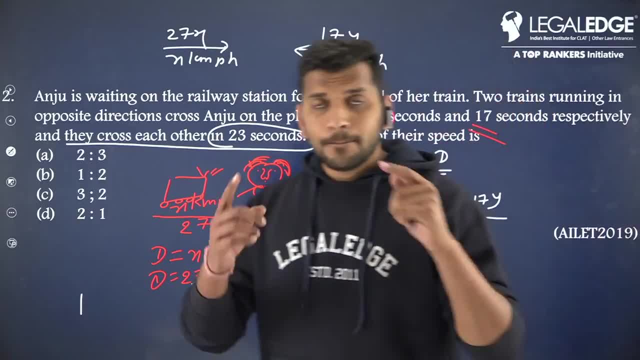 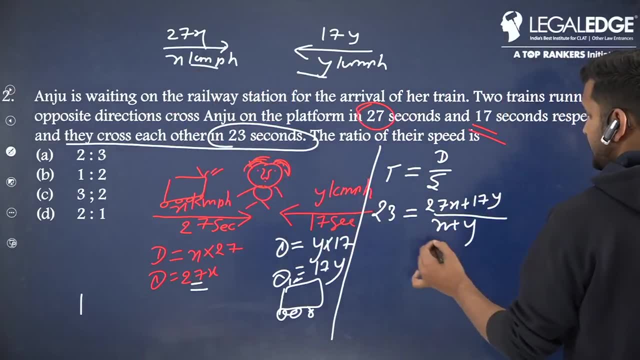 speed, remember, is minus in the same direction and is added in the opposite direction. So what will be the speed? It is in the opposite direction, So the speed will be x plus y. We will just cross, multiply x and y here, so it will become 23x plus 23y is equal to 27x plus. 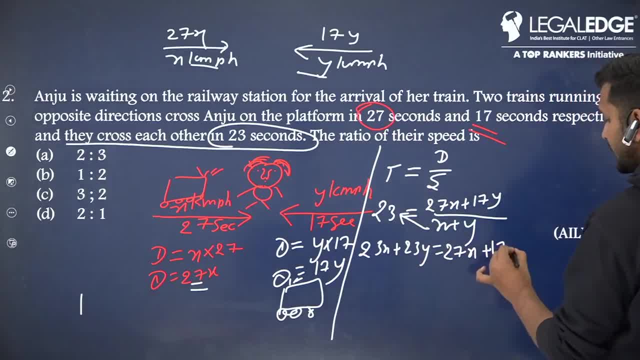 17y, x and x will be did to the side of y, y, X and x will become minus. in this way, Then how much will remain? 23 to 3 will flow. 4x will be left. This is equal to 7 in this direction. 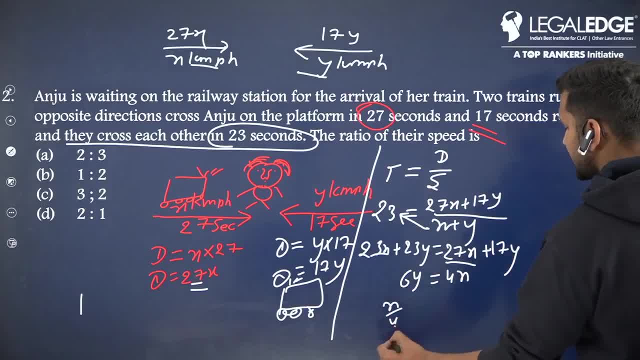 Then 6y will be saved right Here. x to y ratio will be 2, 2.. 2, three. So how much did we get Here? I had done x upon y, So 3wise 2.. So 3wise, 2 is the ratio. There is an option: 3wise 2.. 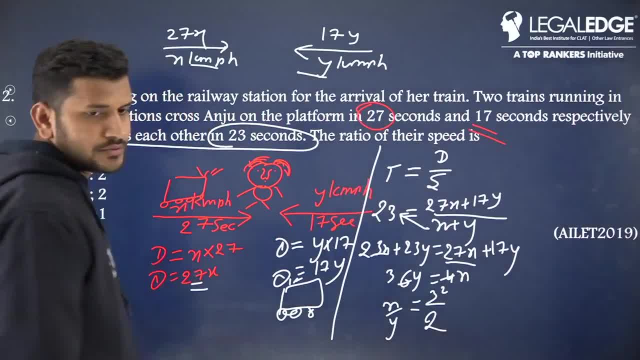 All right, Thenbere're getting it Simple. plus simple is therapist's habit, But I, you Kob, cái Option number C will be correct. C option will be correct. Okay, Vanshi's C is correct. Right, guys, in this way. 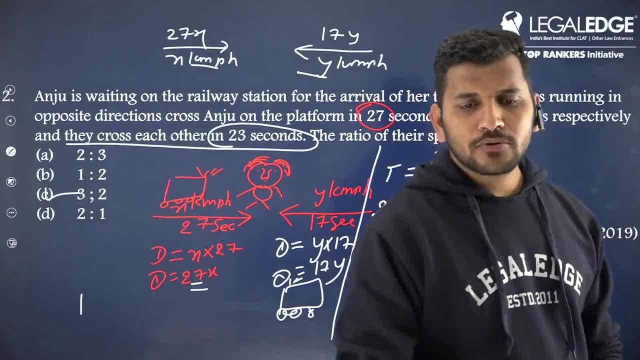 I had to do this question. You have to understand the whole concept. That's why you must be thinking: Sir, this question takes so much time, How do we do it in exam? So to explain you, I have to explain this whole concept. That's why. 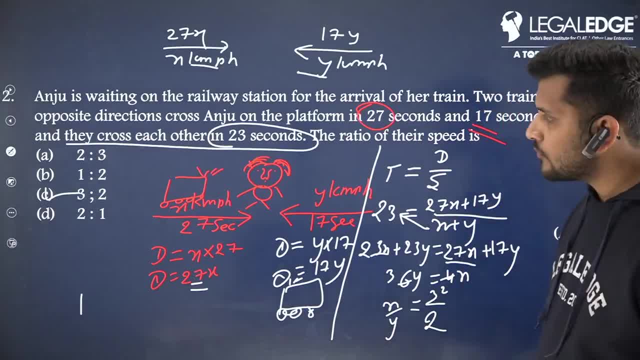 I am not taking time. I don't take much time, Okay, So I think you must have taken a tip. Yes, Anupama C is the answer. Shivan C is the answer. Absolutely So, guys, you have taken a tip. 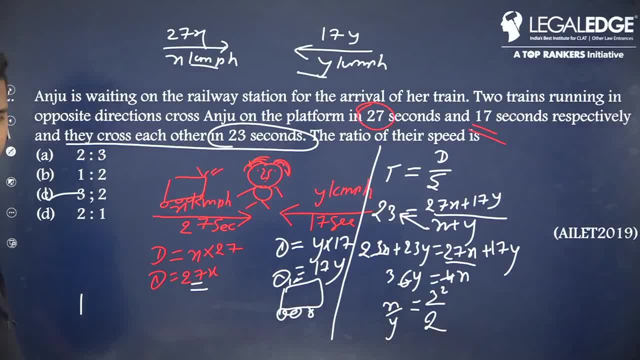 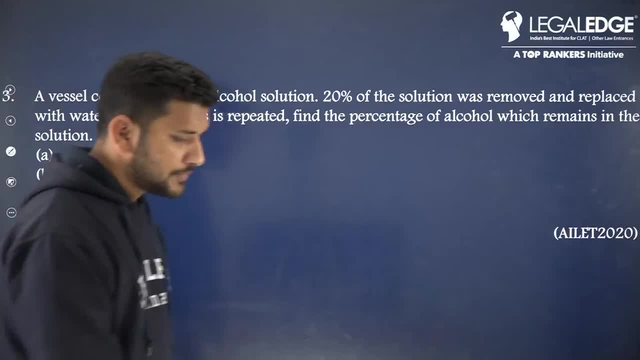 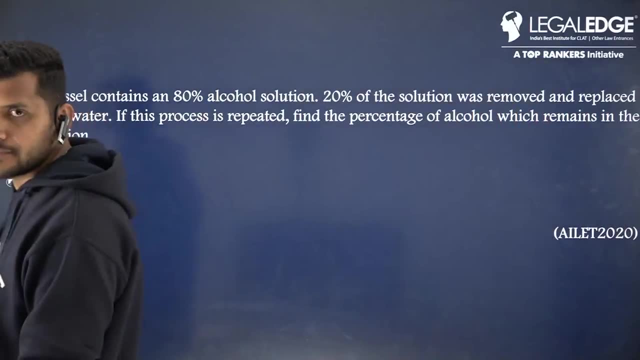 Let's go to the next part, Okay, Because we have a lot of questions in your life. This is the third question. Third question: is this Good question? This is also Elite 2020.. This question has come in Elite 2020.. 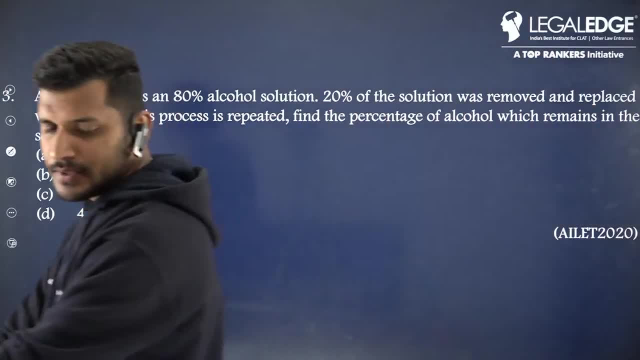 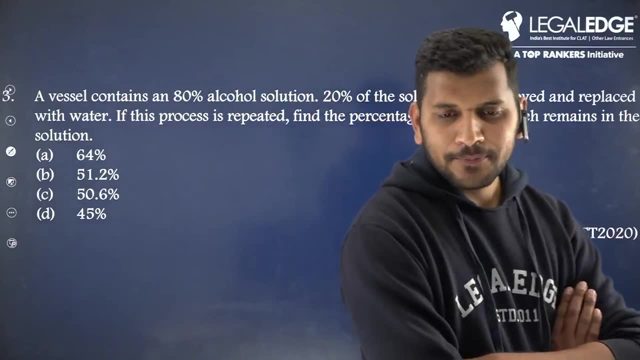 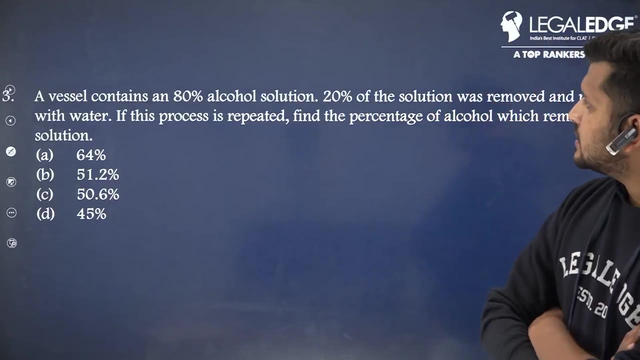 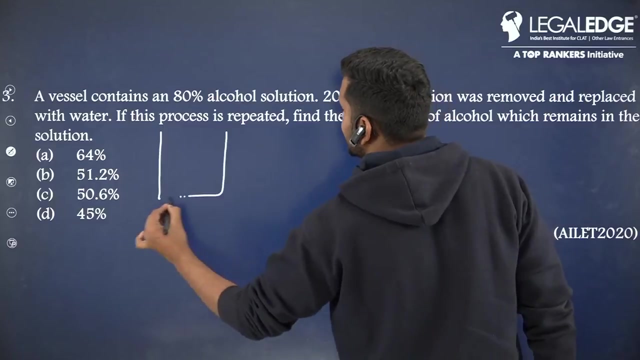 Hmm, Mr Comrade, Use another marker. Now the marker is correct. Now the marker is correct. guys, So a vessel contains an 80% alcohol solution. Bro, there is a vessel which has 80% alcohol solution. There is a vessel, How much is the solution in it? 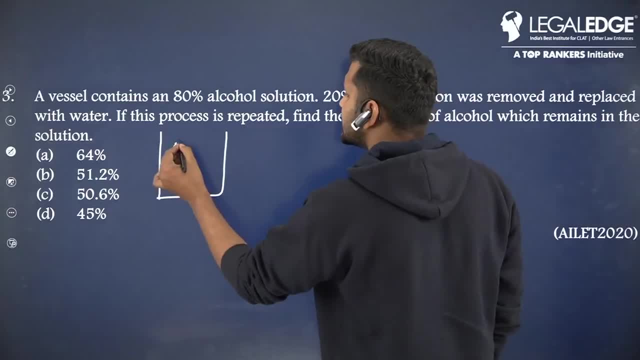 How much is the alcohol? I don't know anything else, But how much is the alcohol? 80%, 20%, something else I don't know? Suppose the quantity of this container is x liter. Suppose the quantity of this container, guys. how much is it? 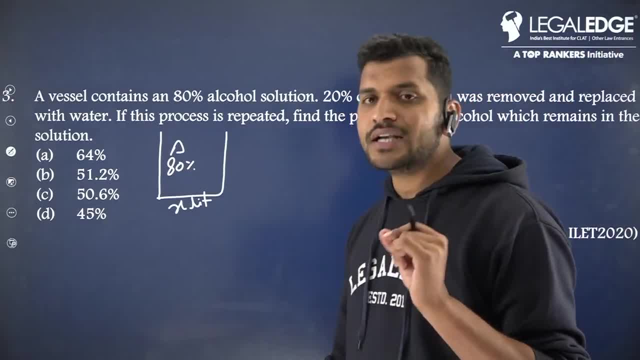 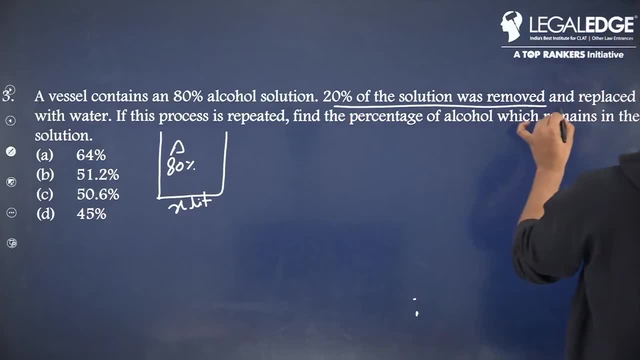 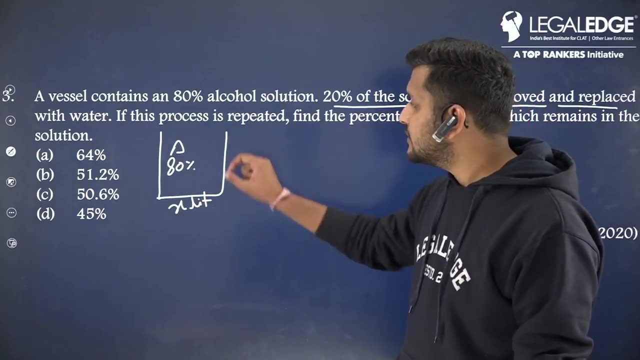 It is x liter. Do you understand? The quantity of this container is x liter. A vessel contains 80% alcohol. 20% of the solution was removed and replaced by water Means in this. whatever x liter is in this, the total solution is x liter. 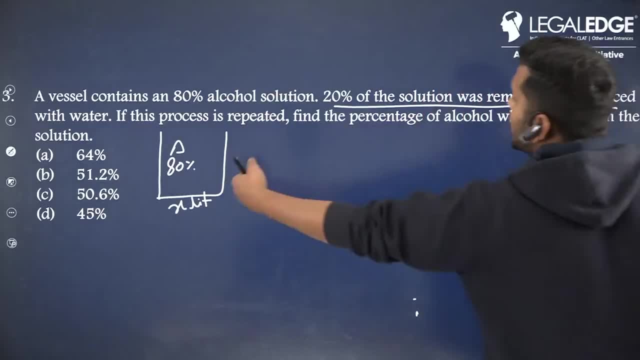 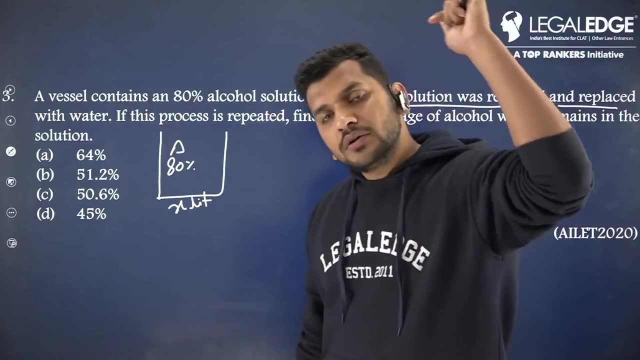 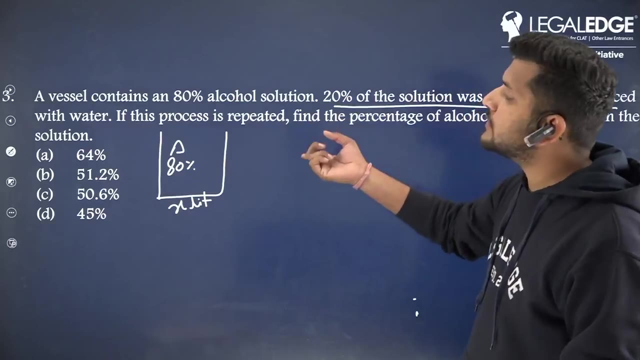 Out of which 80% is alcohol. The quantity of x liter: 20% of the solution has been removed And after removing 20%, in that whatever is removed, that much water has been added And with water replaced with water. If this process is repeated, 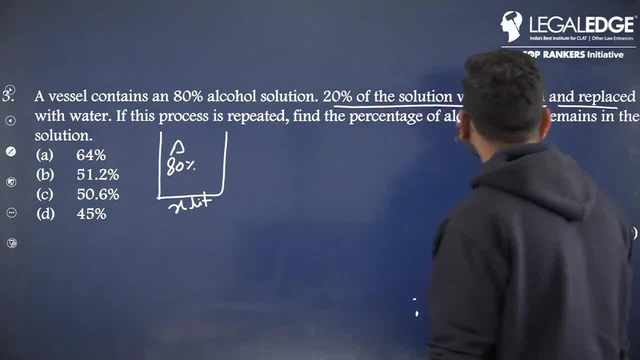 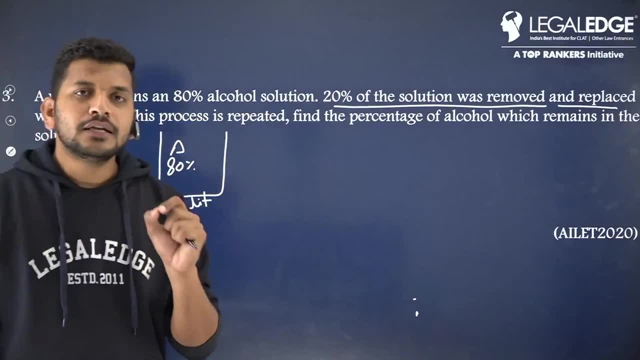 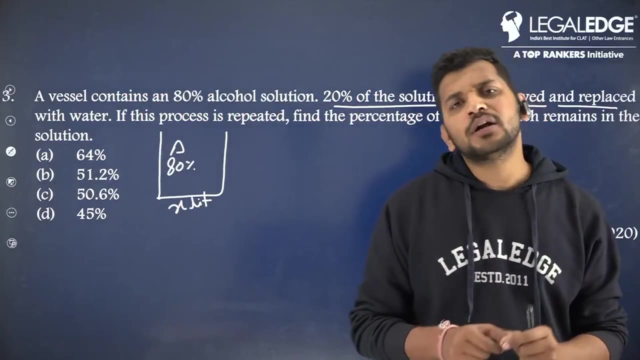 this process is repeated once. then find the percentage of alcohol which remains in the solution. He is saying: once there was a container, the quantity of that container was not told. The quantity of that container was x. Right, There was a container and the quantity of that container. 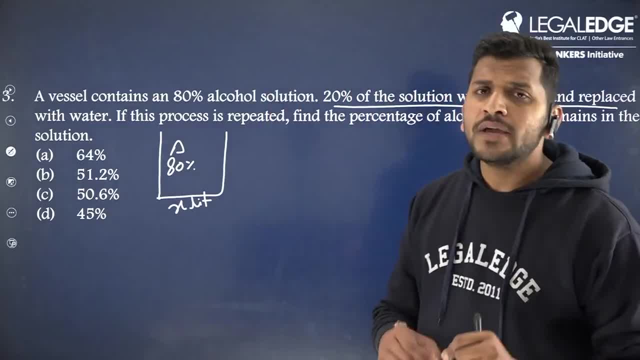 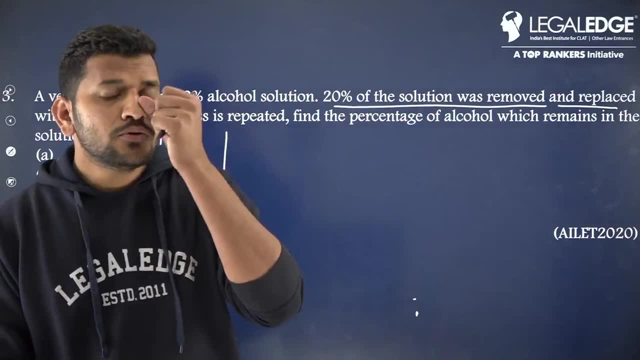 was not told, guys. The quantity of that container was x And in that alcohol was 80%, Right Or 20%. Anything can happen. But when he removed 20% in that, when he removed 20%, then the mixture will come out 20%. 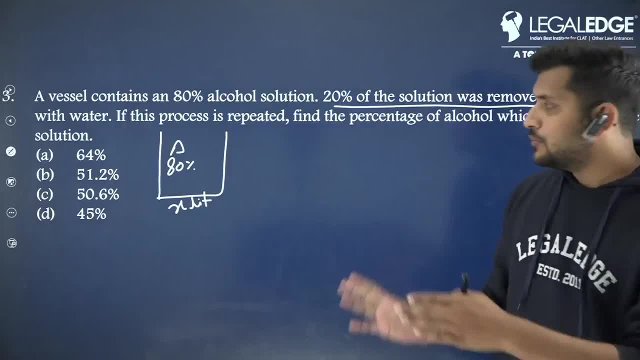 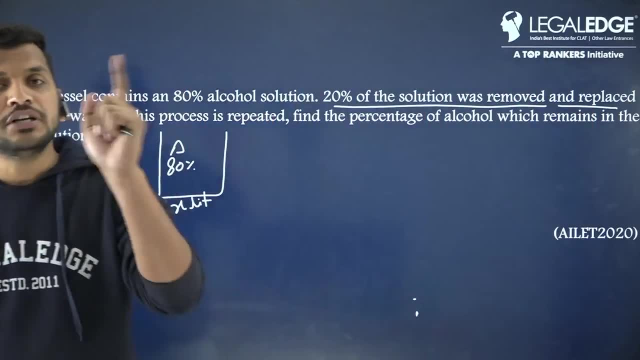 And in place of that 20% he added water. And then he said that whatever quantity has been added, this process has been repeated once again. That means next time he must have removed 20% of the mixture And he must have added water. 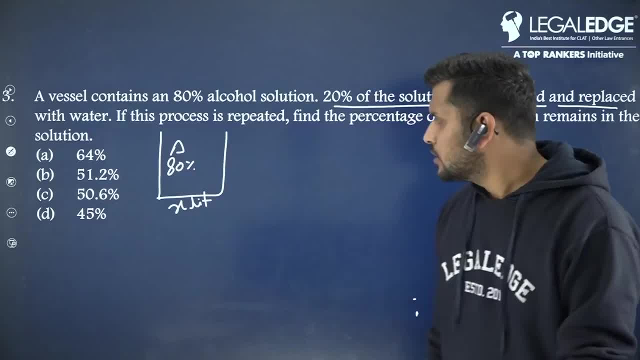 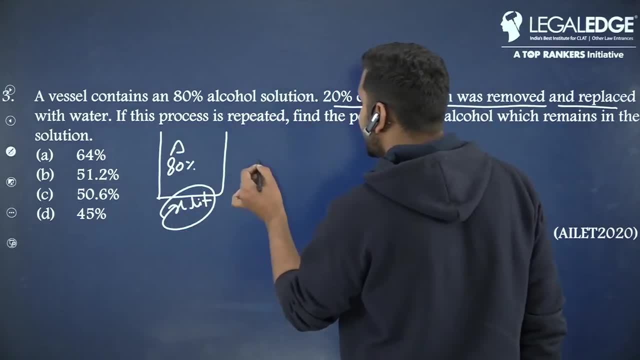 Then he is asking how much alcohol is left. So how much percentage is left? Understand the way to do this question. First of all, we know what is the total. It is x liter. It is x liter. How much is the alcohol in it? 80%. 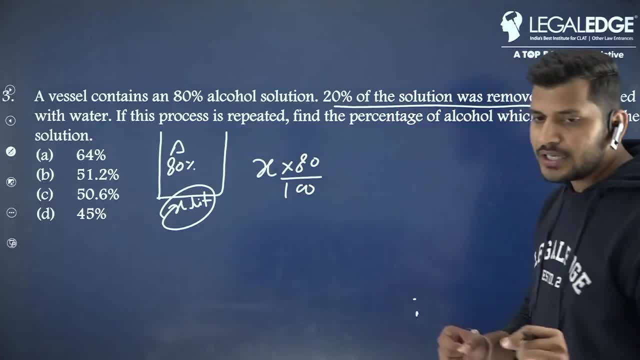 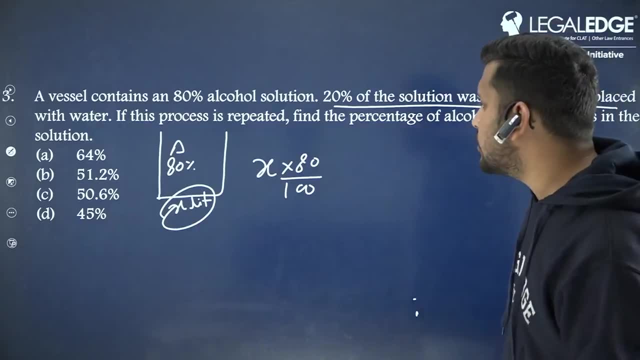 So is the alcohol this much in the initial container? Initially the quantity of the container is x liter. If we remove 80% of it then I got to know that how much is the quantity of the initial container x into in the initial container? 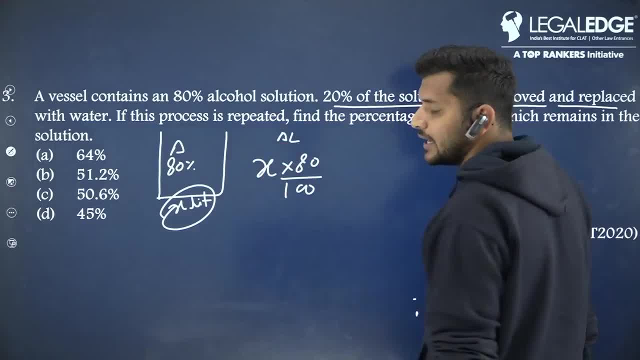 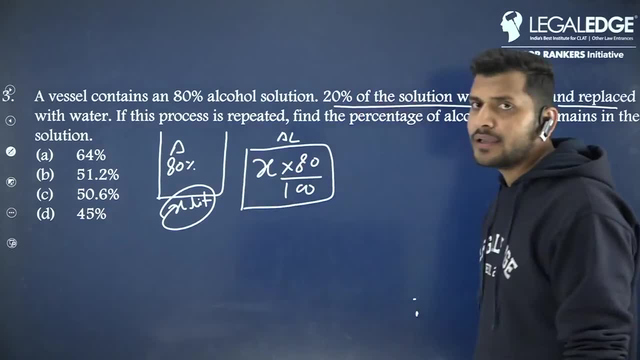 how much is the quantity of alcohol? This is the initial quantity of alcohol. 80 upon 100 is the initial quantity. But now he is saying that the initial quantity is this much. How much has been removed from it, Guys, if he is saying that? 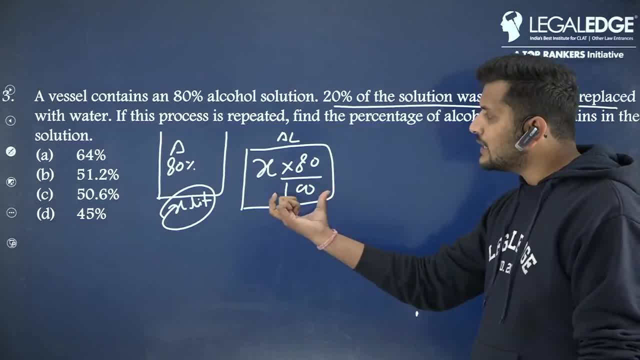 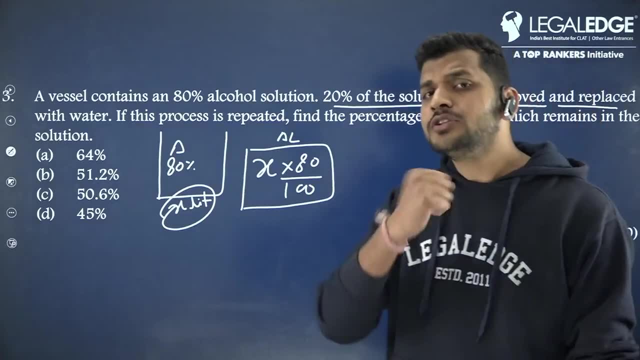 20% solution was removed. this total quantity of alcohol out of this 20% alcohol will be removed. Now it is alcohol. The quantity of alcohol is this much: out of this, 20% alcohol will also be removed. So 20% alcohol was removed once. 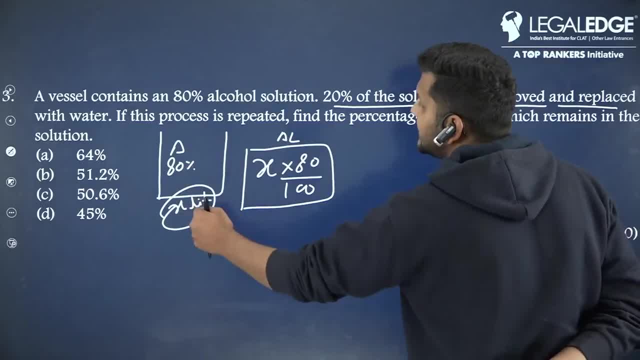 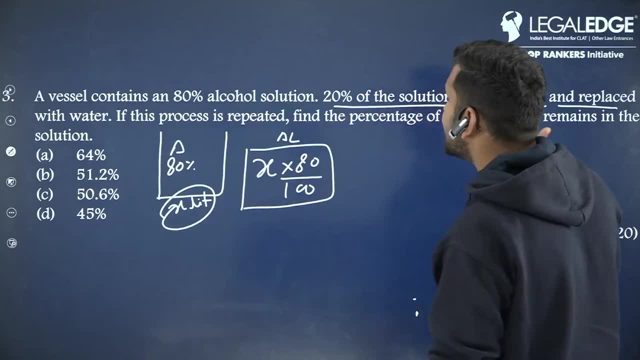 This is alcohol. This was the x liter quantity of this container in which I first found alcohol. This is the total amount of alcohol in it. Now, if 20% is removed, then 20% alcohol will also be removed and the other mixture will also be removed. 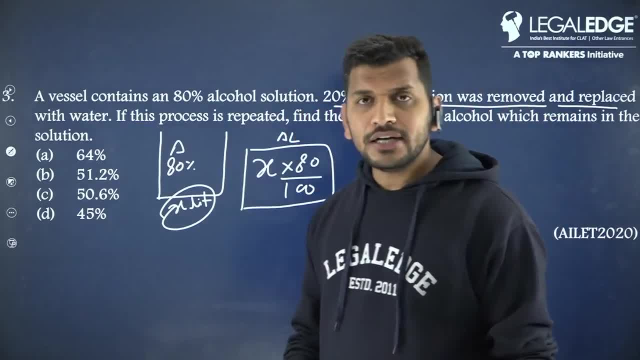 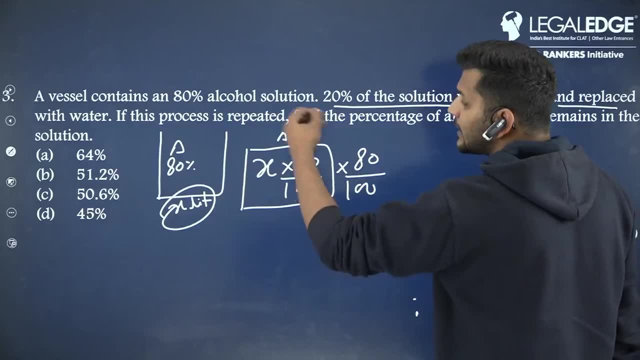 But I have to keep the meaning of alcohol. So how much alcohol will be removed? 20% of it will be removed. Then how much will be left? 80% will be left. This data is calculated and whatever value comes, 20% of it is removed. 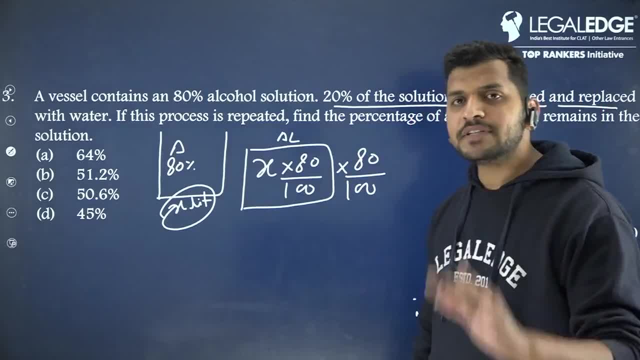 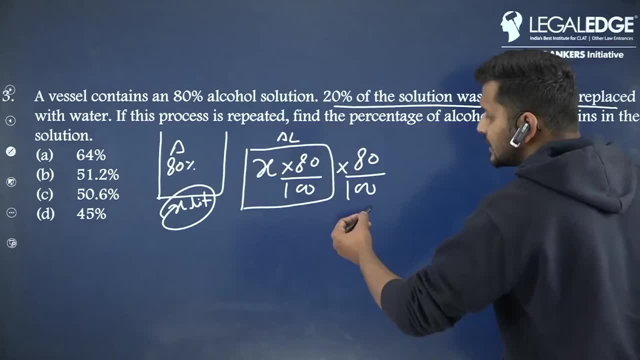 So only 80% will be left. Exactly, sir, 80% will be left. Now, what happened after this? After this? what did they do again, They repeated this process. Now, this much alcohol is left. This much alcohol is left. 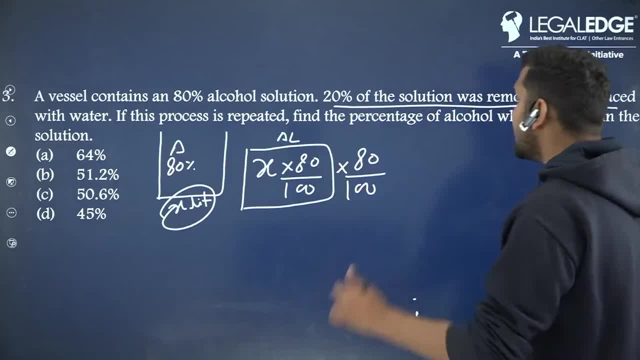 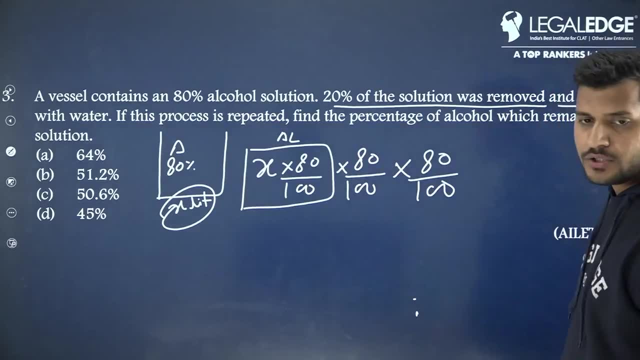 The total amount of alcohol is left. But again, they have repeated this process and again 20% has been removed. Now, again, 80% is left after removing 20%. Now, finally, this much alcohol is left. We will solve these three. So, after solving these three, 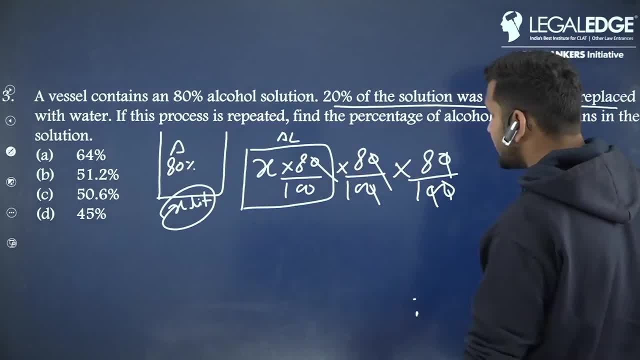 1, 2, 0, 2, 0, 2, 0 are cancelled 4 into 5, 512.. This multiplied by 512x upon 1000.. This is the final alcohol. What is this quantity? 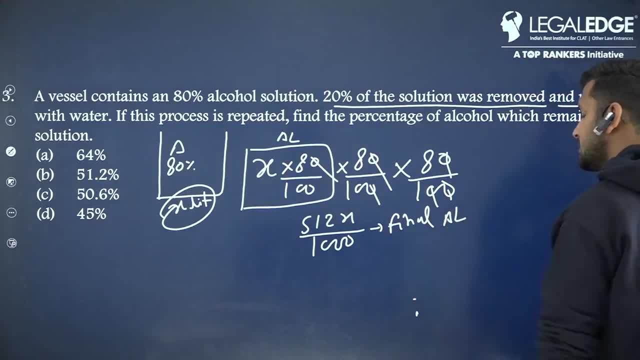 Final alcohol after two operations. Final alcohol is left in that container after two operations. So they asked if this process is repeated. Then they asked: find the percentage of alcohol which remains in the solution, Sir, 512 is left 512, how much is this? 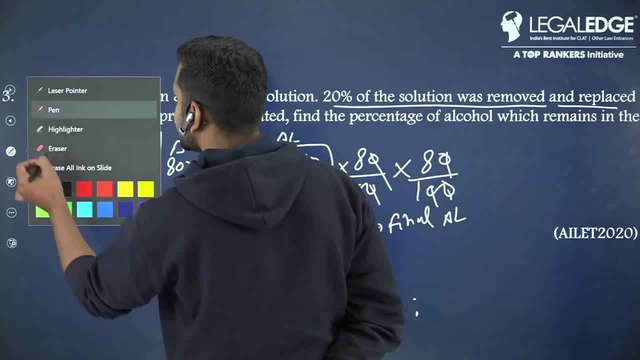 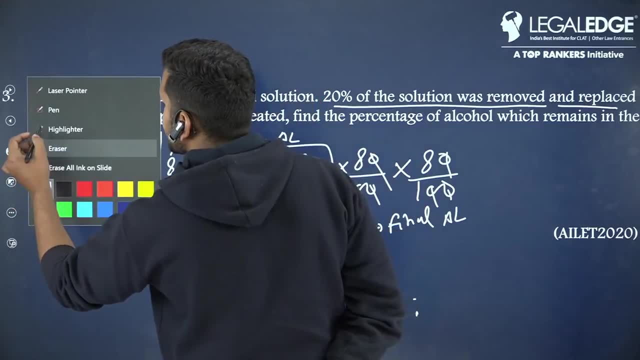 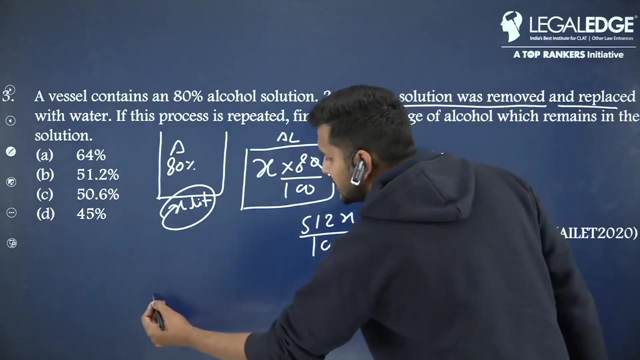 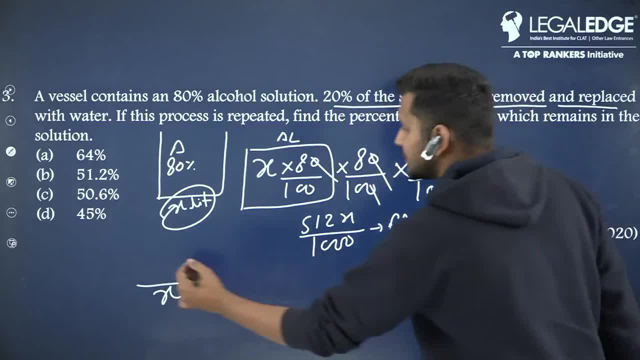 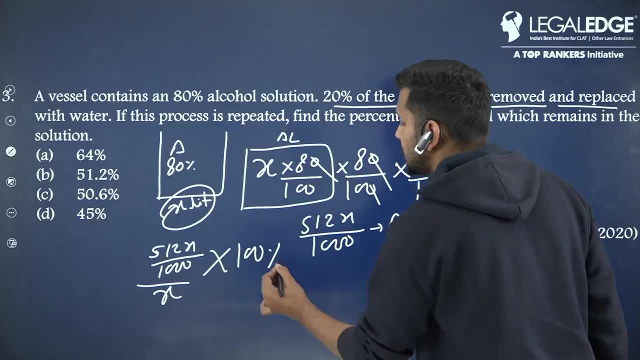 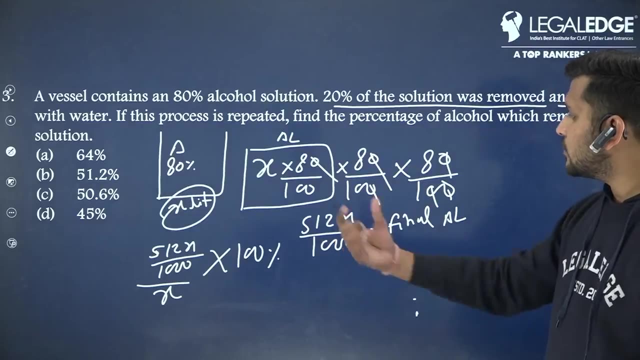 Total quantity. We take out the percentage And how much is left- 512x upon 1000. And how much is left 100%. This is what we have to take out. We have to calculate from the total quantity. The total quantity was x and there is so much alcohol left. 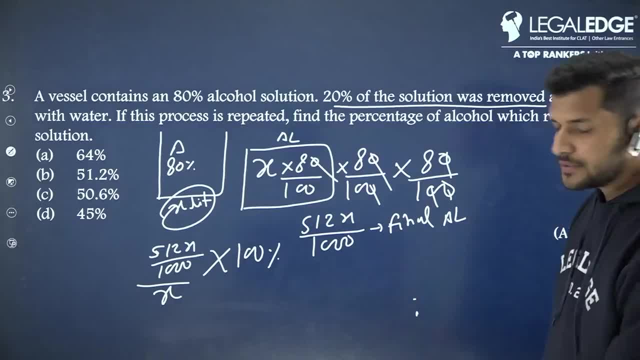 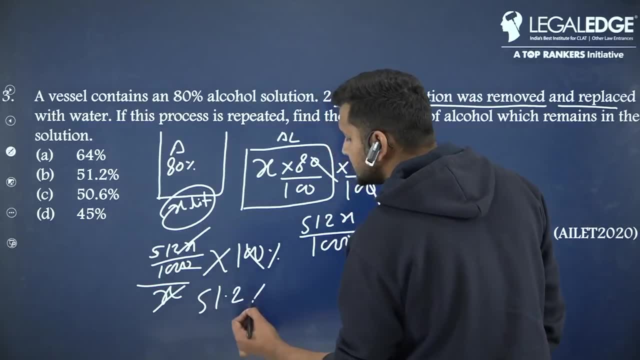 That's why I asked: find the percentage of alcohol which remains in the solution. x will cancel x. 2 zeros will go away from 2 zeros. If it will go away from 10, then it will become 51.2%, Which means this option will be correct now. 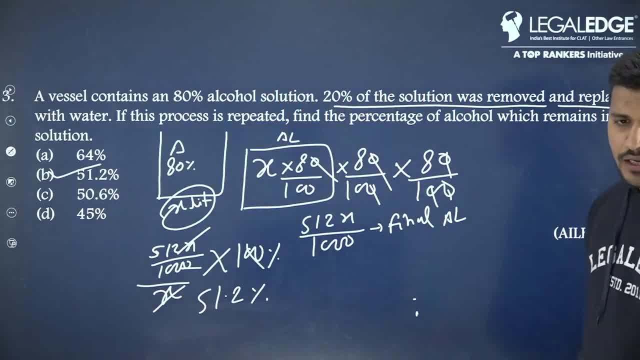 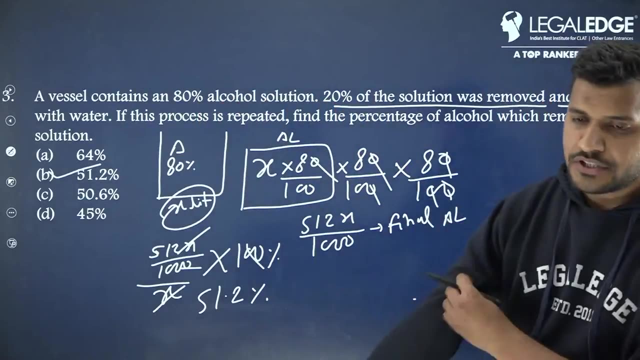 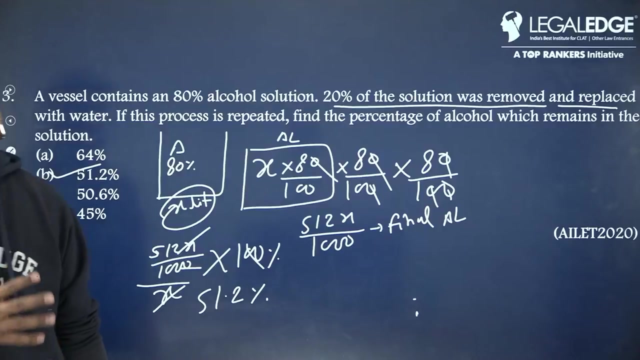 Okay, guys, it was easy, It won't take time. It won't take time, You just have to calculate. The questions that I am asking from the previous chapter are important. Arif, The whole chapter is important, Like ratio, proportion, percentage mensuration, time-speed, distance, time in work. 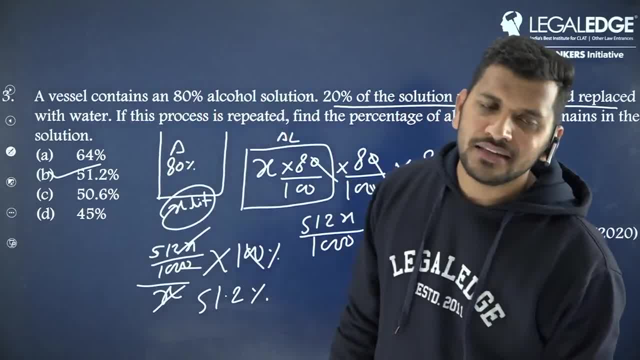 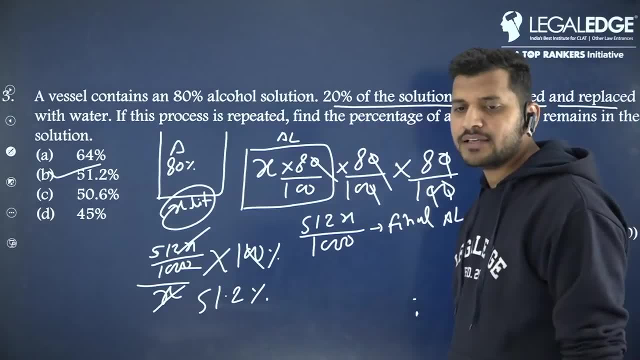 simple intest compound intest number system, LCM, SCM, permutation, combination probability. all are important for CLAT- Sorry, ELITE. And important for the basis of CLAT. Okay guys, 51.2%. You must have taken the tip. 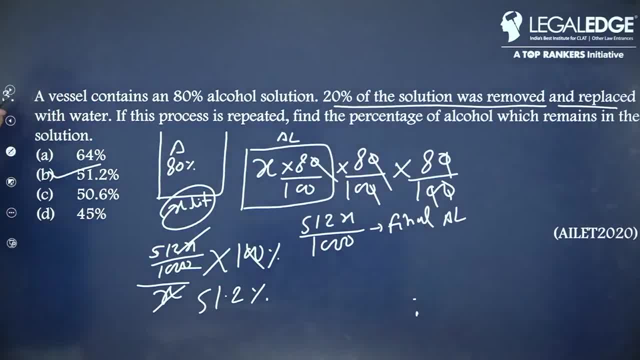 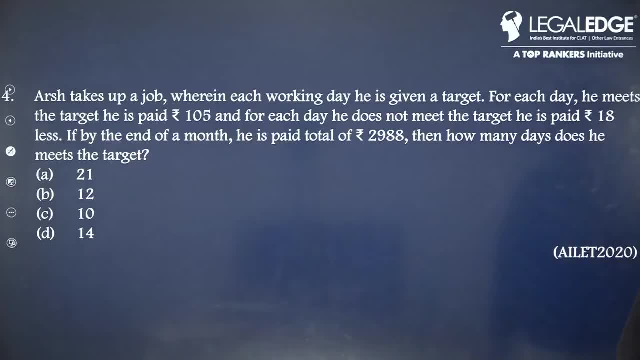 I have so much trust on you guys, Right? So let's do the next fourth question. This also came in ELITE 2020-2020.. This question also came in 2020-2020.. Tell me the answer to this. 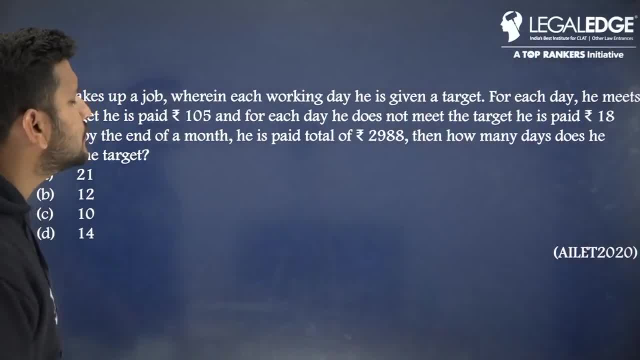 Hours takes of the job when each working day he is given a target. He is given a target every day. What are you saying? Hours takes of a job Right. Hours takes of a job wherein each working day he is given a target. 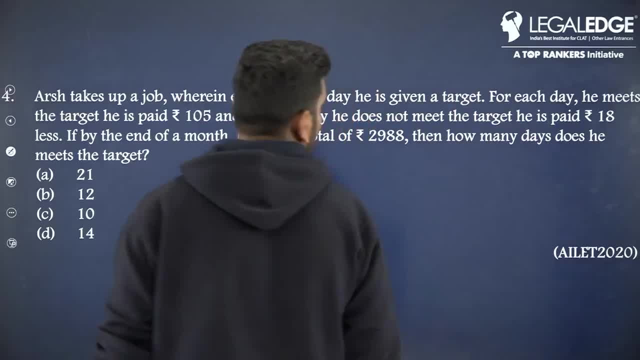 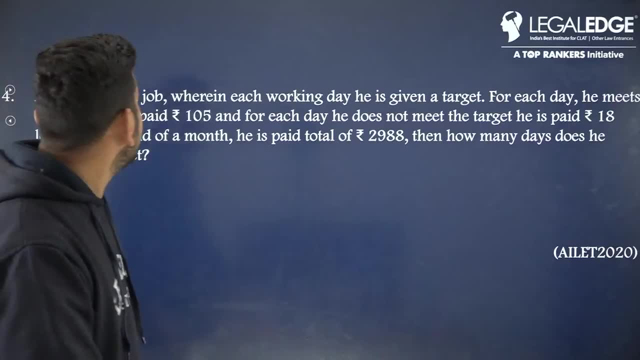 Each working day he is given a target. For each day he meets the target, He is paid 105.. Let's talk about one month Takes of the job where each working day he is given a target. He is given a target in every working day. 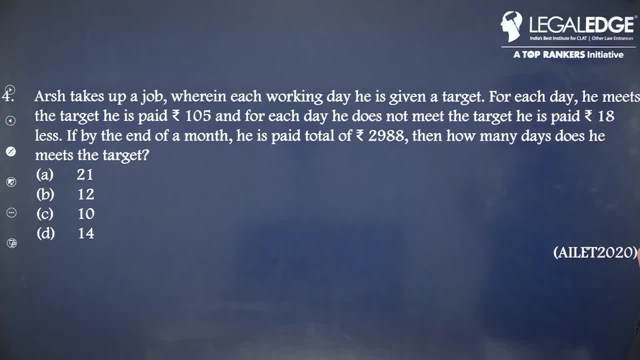 For each day He is talking about. every day He meets the target. If he gets a target every day, he will get 105 rupees. If he gets a target in one day, he will get 105 rupees, And for each day he does not meet the target. 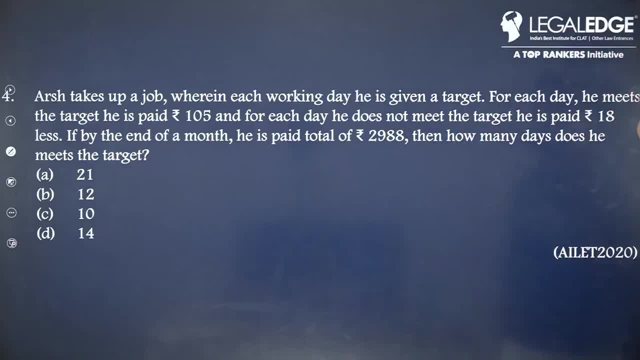 If he does not get the target on the day he is given the target, he will get 18 rupees less And by the end of the month he is paid total 2988 rupees. And how many days does he meet the target? 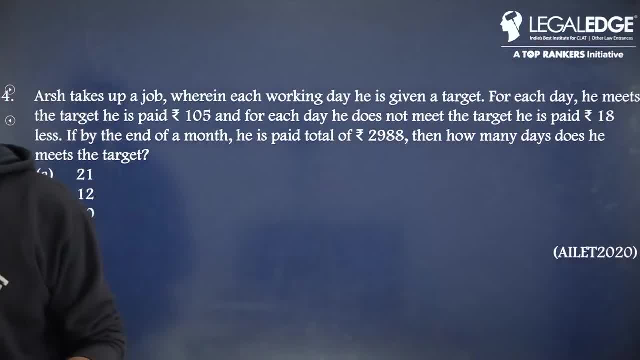 So guys, keep in mind that we are talking about one month And in one month we are talking about 30 days and not 31 days, Because he said that if it is a matter of one month, then some days he got the target and some days he did not get the target. 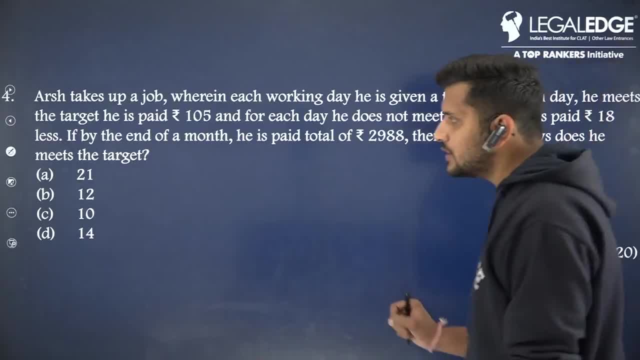 One month means you have to consider 30 days in this question. There was a problem in this question. People were worried that you have to take 31 days and 30 days, So you have to take 30 days of one month here. 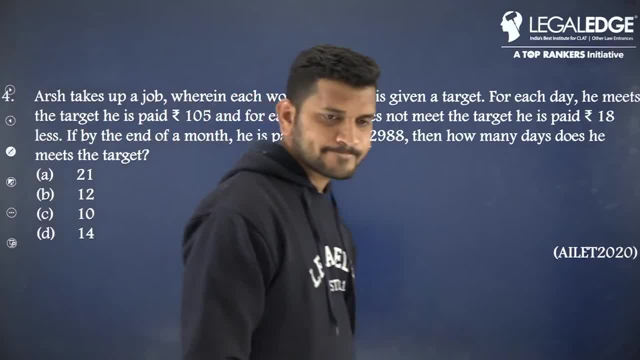 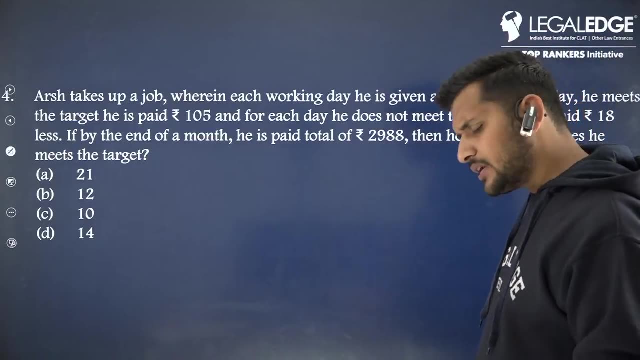 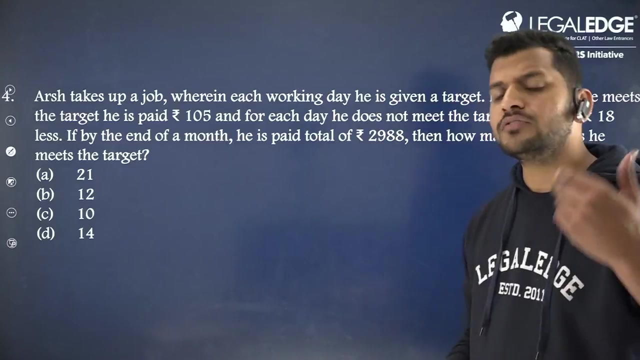 Right. So let's see: Arsh takes up a job wherein each working day he is given a target, But he is saying that for each day he meets the target He is paid 105.. As soon as he gets the target, he gets 105 rupees. 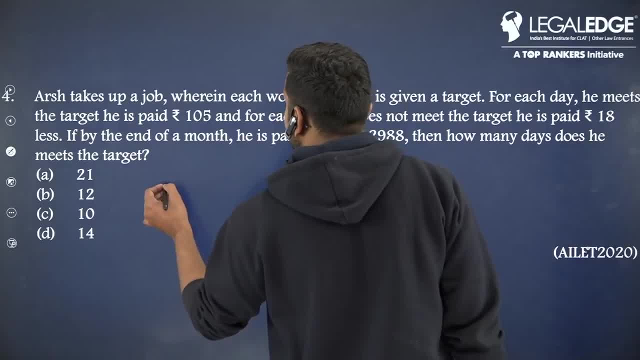 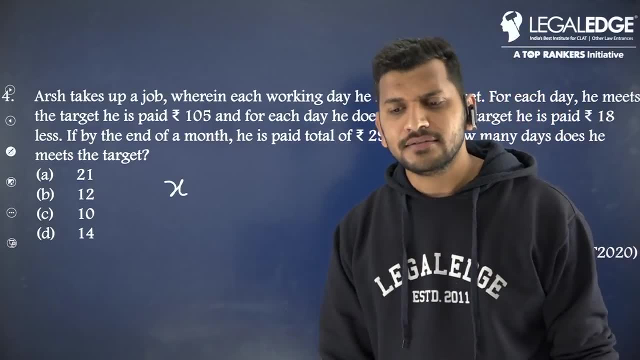 So I said that let's take a value x. x is such a value. x is such a value for how many days he got the target. Guys, we are talking about one month of one month, Right? Please make the supervisor, do the supervise. 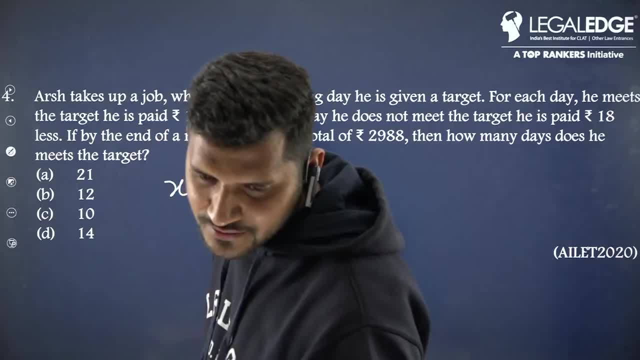 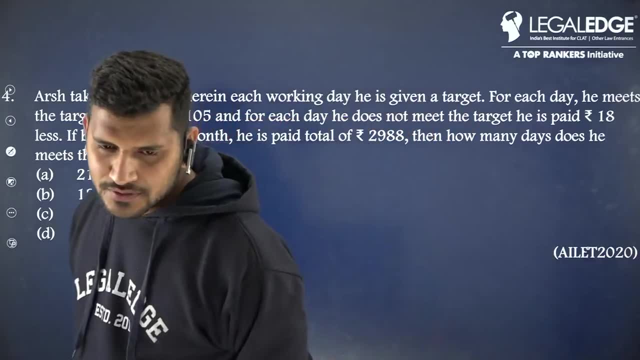 Okay, please make the supervisor do the supervise. Aayush Sharma is saying: Yes, Sir, please up Chattervise. previous year, Questions were about those who also did: Who comes in the class of advanced level, Who does not come in the class of advanced level. 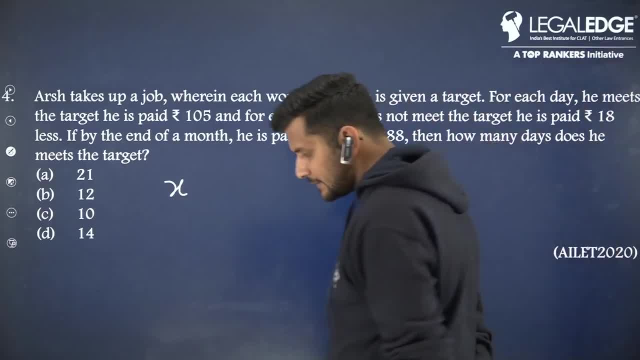 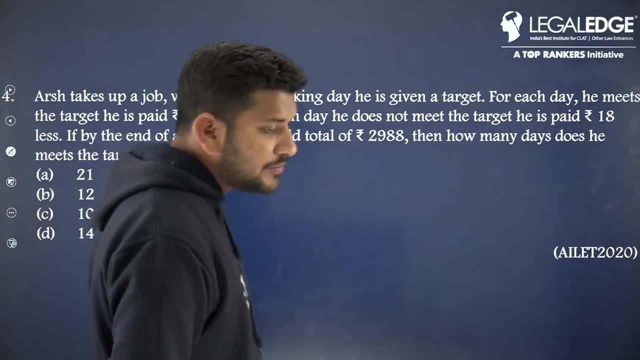 Now look here. So what I am saying is that there were 30 days in total In which he will get the target for some days and some days he will not get it. You cannot say this from your mind. You cannot become a scientist. 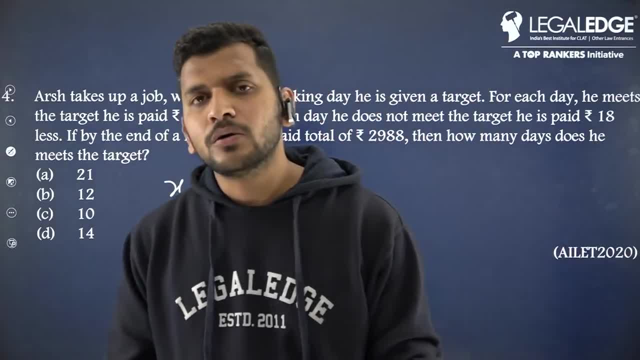 Sir, you must have got the target for 15 days And you must not have got the target for 15 days. How can this happen? It cannot happen. So you said Sir X has such a value for how many days he has got the target? 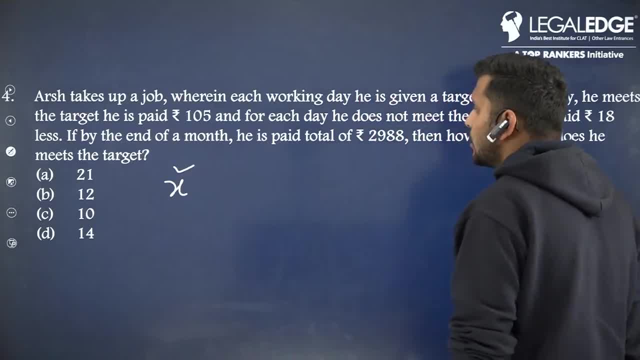 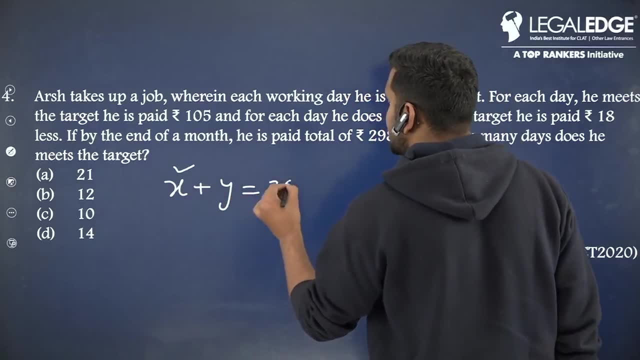 Right. X has such a value for how many days he has got the target And Y has such a value for how many days he has not got the target In this way. what are the total days? 30 days. One month means 30 days. 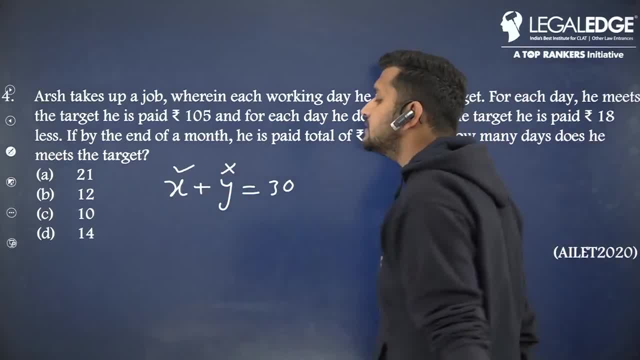 X has such a value for how many days he has got the target And Y has such a value for how many days he has not got the target. You understood the thing. So this is it: 30 days. Can I do this? 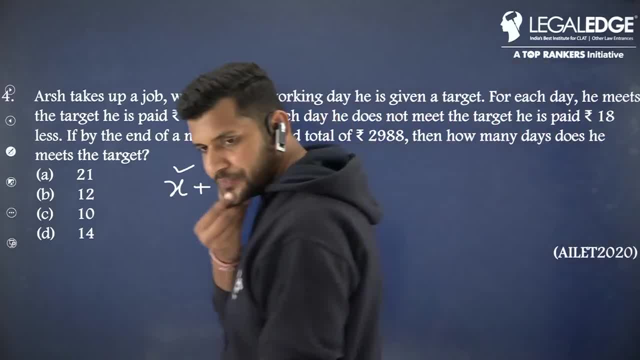 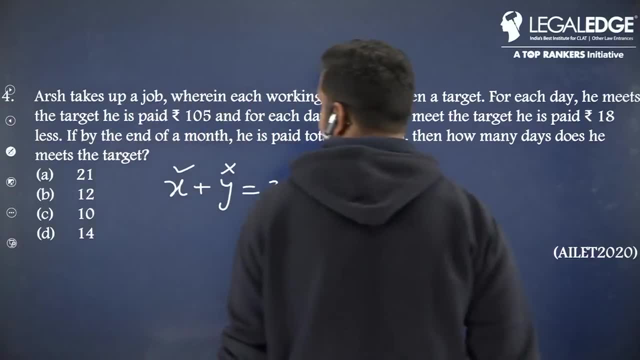 Is there any problem in this, Sir? please do it. We will do it. We will do it. Don't worry, Everything will be fine. Hmm, Now see what happens after this. He said when he gets the target, he gets 105 rupees. 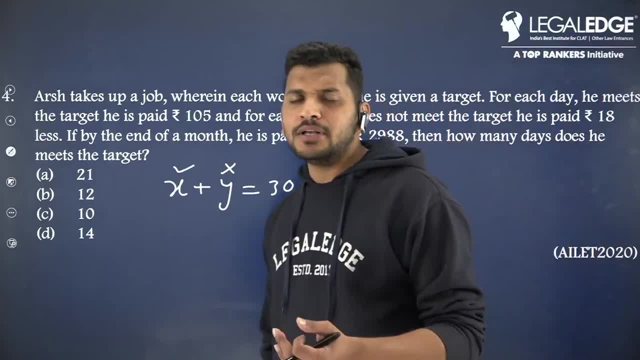 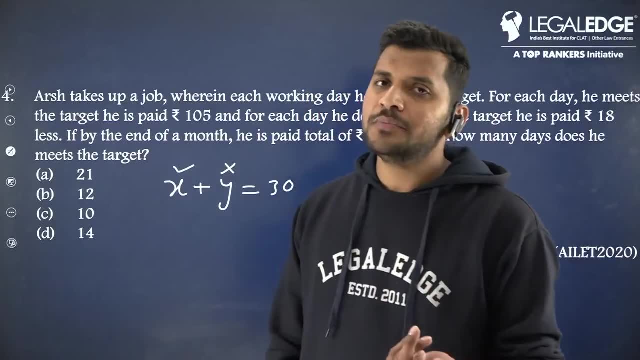 Means today I worked, Today I got the target, So for today I will get 105 rupees. Hmm, Today I worked, So for today I will get 105 rupees. And if today I did not work, I did not get the target, then my work did not happen. 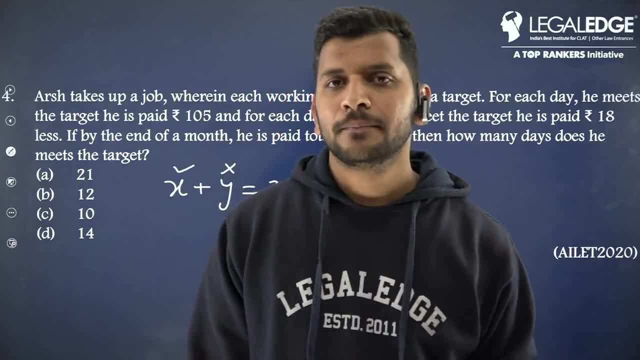 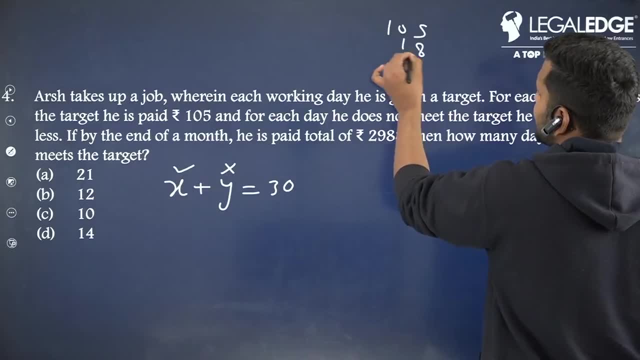 That means I will get less than 105 rupees. So today I understood. So if I do minus 18 rupees from 105,, 105 will be this: You do like this, You do like this. If 15 goes like this, then how much is 7?? 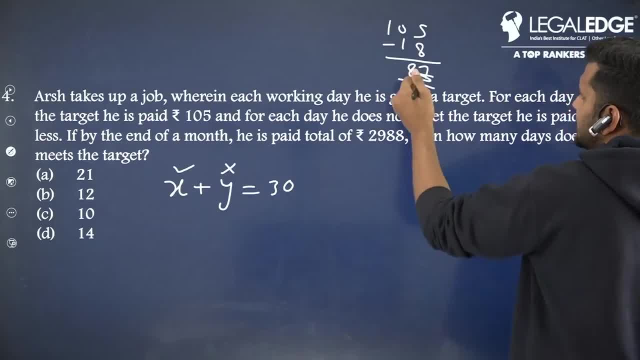 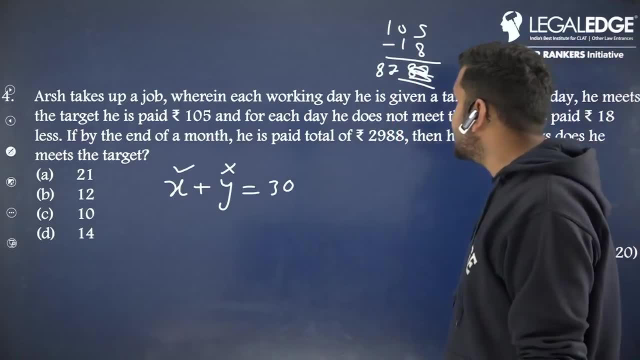 Minus 1 becomes 87.. You do like this, Guys. it is 87.. Cut this. This is 87. Right? Okay, So you said: Is there any answer? Is there 21 answer coming? 21 is correct. 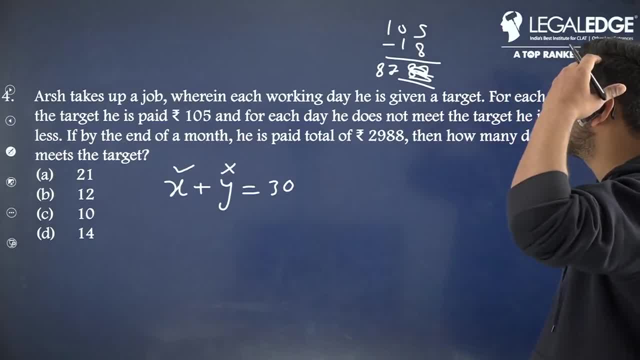 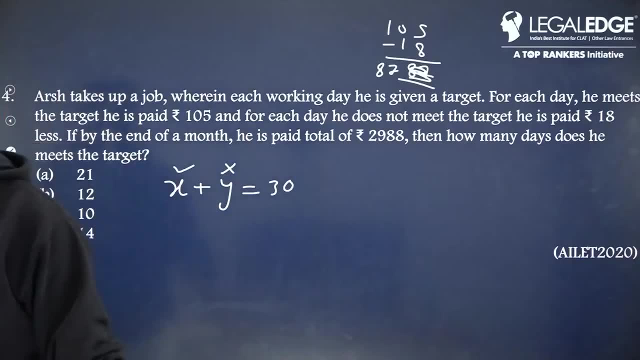 21 is correct. Tell me quickly Once more. Look, I am saying what is the need for once more. It is a matter of one month. There were 30 days. I got a job. I was told. if you achieve the target, if you get a target every day, then you will get. 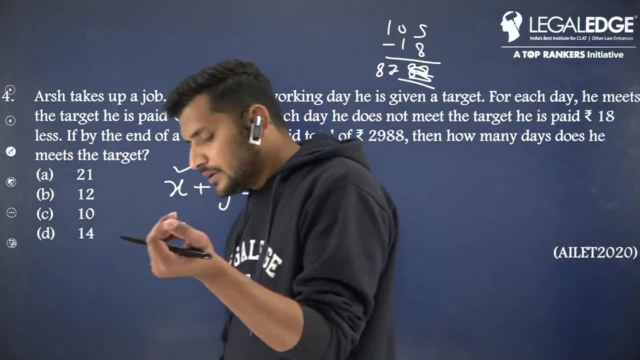 1: 0.. How much will you get? How much would you get? How much would you get? 105 rupees will be given And if you don't bring the target, how much will you get? Less than 105 means you will get 87 rupees. 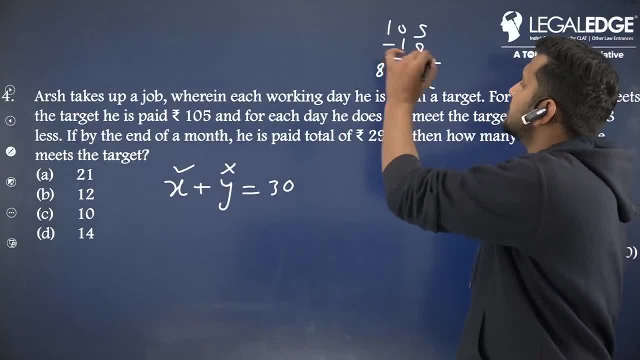 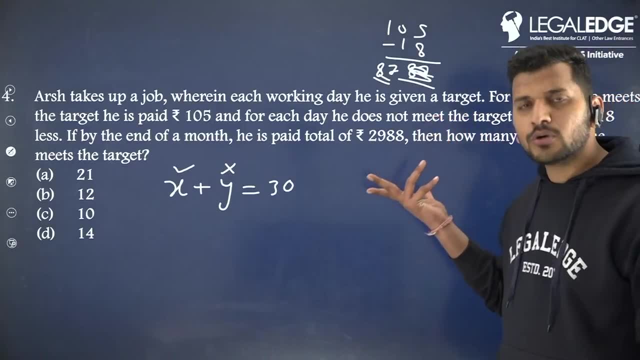 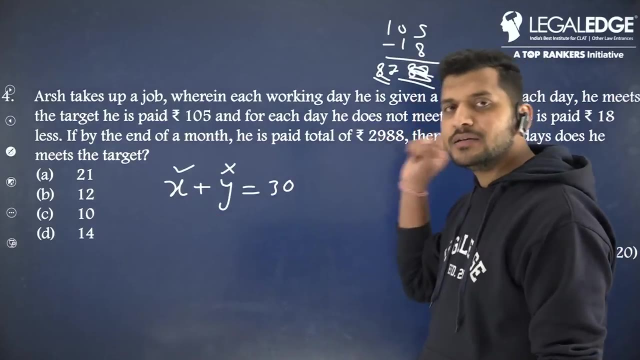 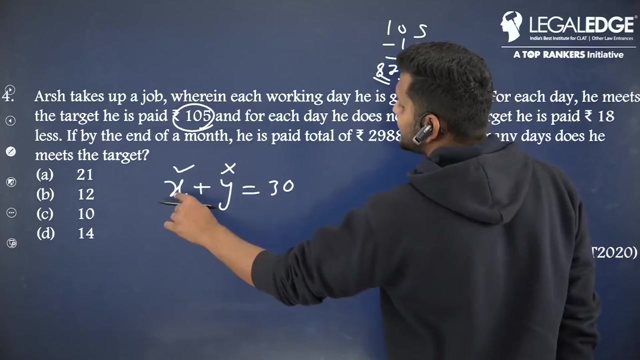 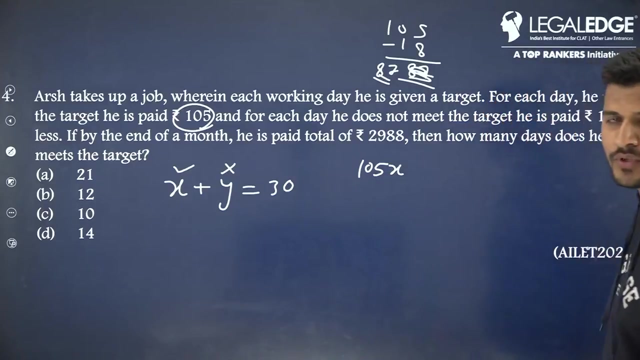 And if you don't bring the target, how much will you get? 105 means less than 18, means you will get 87 rupees. I said, okay, let's do the job. it is the time of lockdown, there is nothing, so let's do the job. so in this way the total days became 30, but when I got the target, then I got 105 per day. I got 105 per day and I said: I got the target for X days, so how much will be the target for X days? then 105 into X will be done. I got the target for X days. 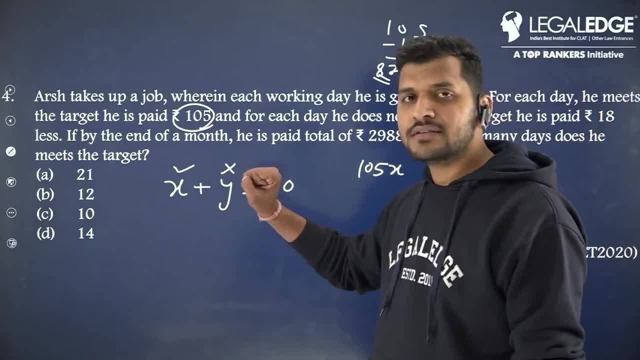 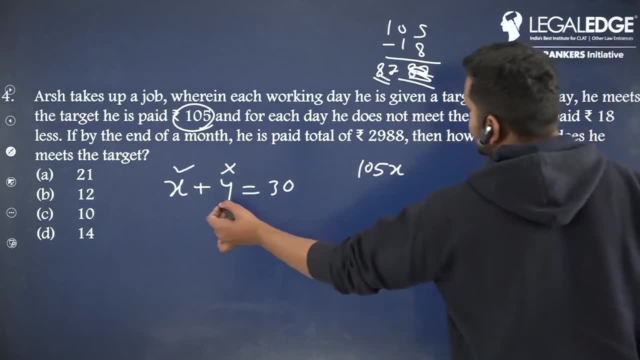 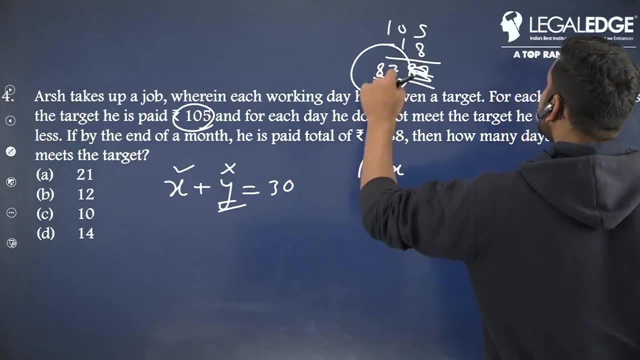 so how much will be the target for X days? then I got the target for X days and the day I got 105, then it will be 105X. for the day I got it and the day I did not get it it is Y days and for the day I did not get it I am being paid only 87 rupees. so in one day I did not get it, for Y days and the day I did not get it I am being paid 87 rupees. so it will be 87 into Y. it will be Y. in this way, the total value is 2988,. 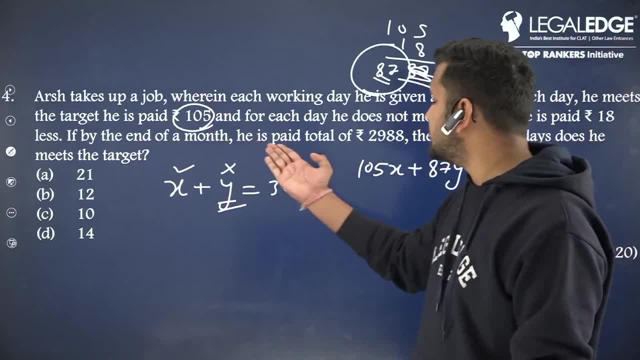 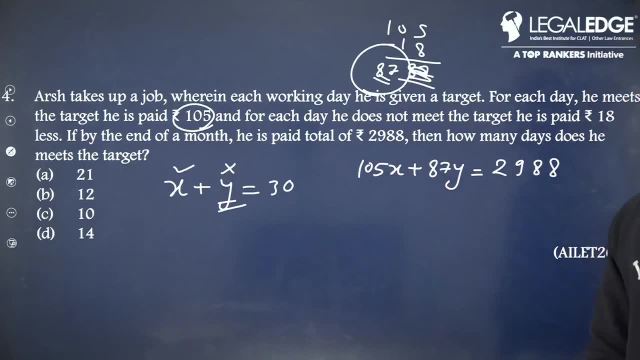 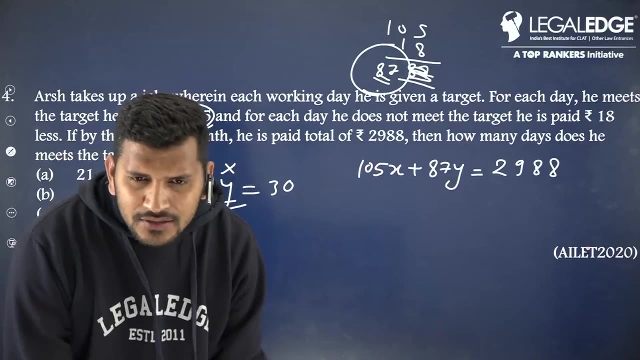 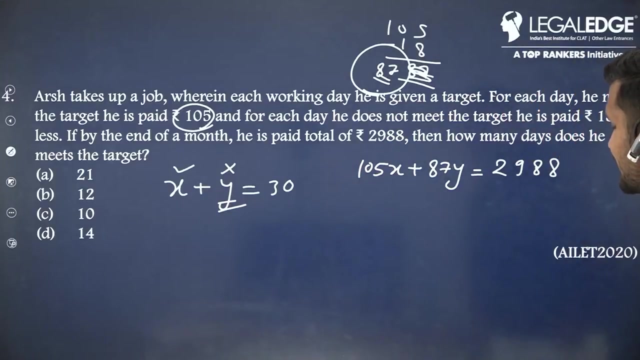 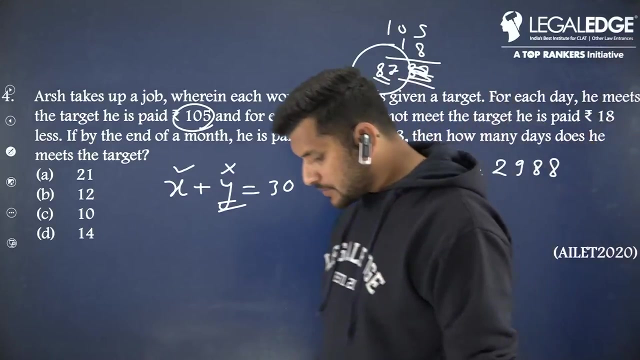 in this way, the total value is 2988, here here, here I am correct. I have to see it at least. okay, I have to see it at least okay. So now, here we know, the elimination method. how will we do it? 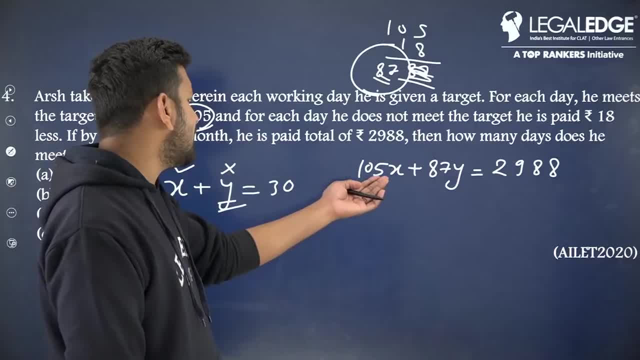 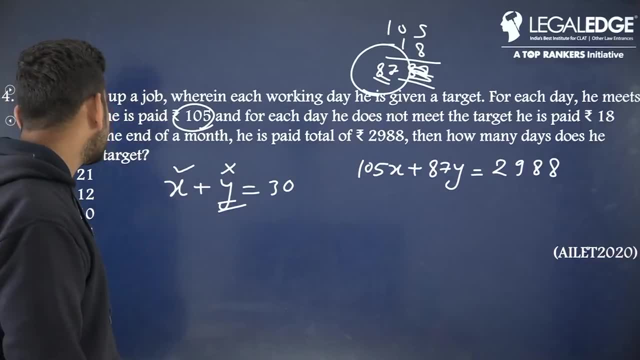 Sir, here we have to make y easy. 105 is here, so in 105 we have to multiply by x 2 equations, 2 unknowns. we can solve it Right. you can do it with an option, but it will be a little long. we will have to put it in that also. 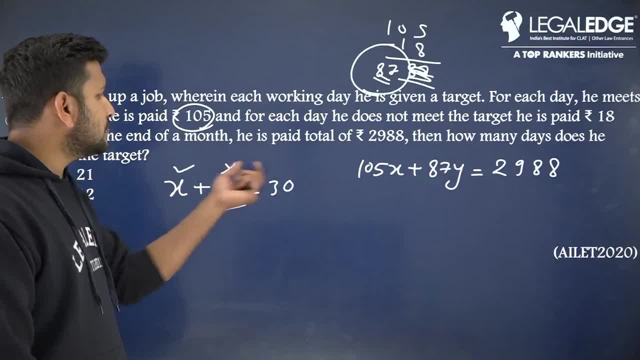 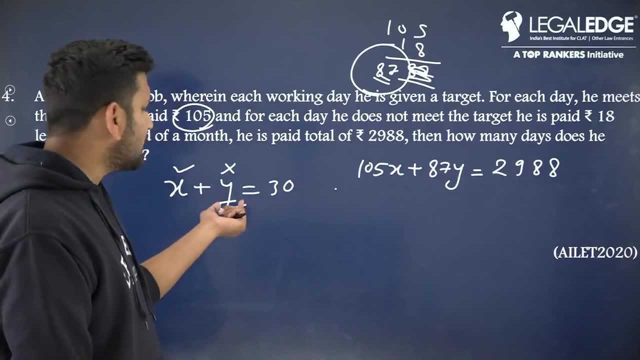 That's why what you do is straight, sir, here if we make x then we will have to bring 105 with it. it will be a big deal. That's why we made y. so 87y is here. so make y. 87 here means we have to multiply 87 in this. 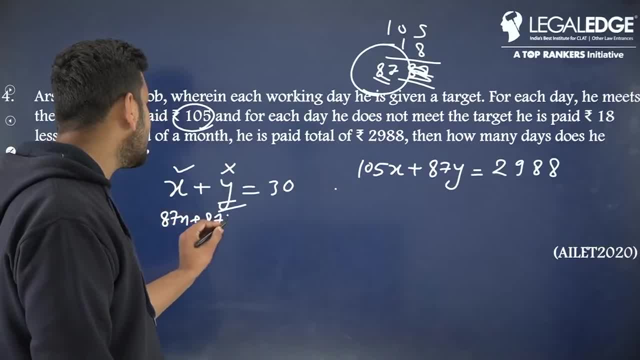 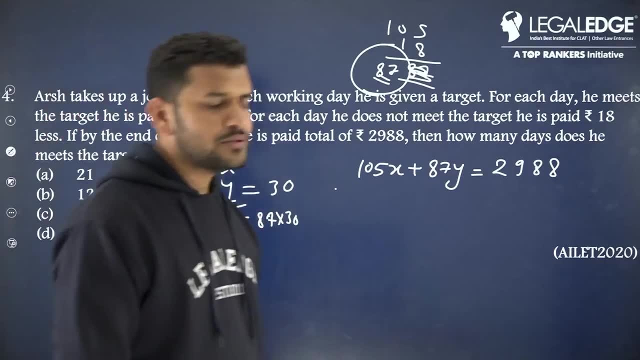 So it will be 87x. it will be 87y right. and how much will it become? It will become 87 into 30,. are you understanding? How much will it become 87 into? It will become 30,. and they solve the equation. 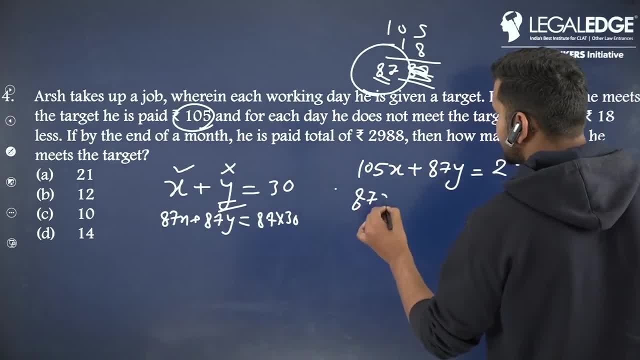 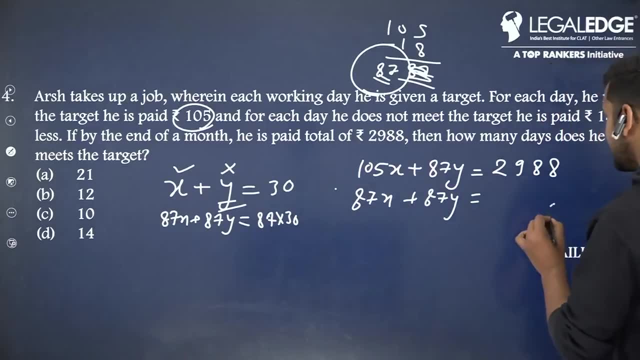 So guys write x here, it is 87x. and how much is y? It is 87y, no problem. and how much is their multiply? 20.. It will be 0,, 7,, 3 is up, 20, 1, right, 2 will be left, 24 and 2, 26 will be left. 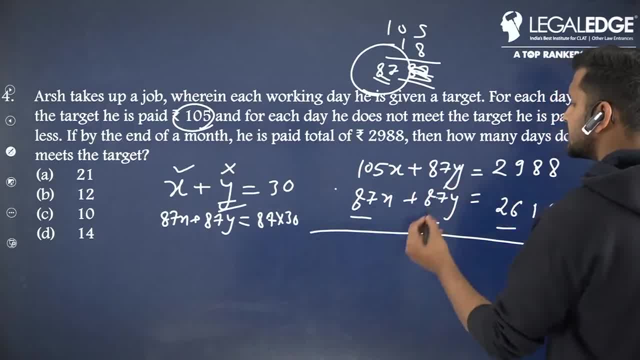 We will subtract them. you can subtract LHS and LHS. both of them will get cancelled. LHS can be subtracted from LHS, RHS can be subtracted from RHS, so how much will be left? 378 is equal to right. are you understanding what I am doing? 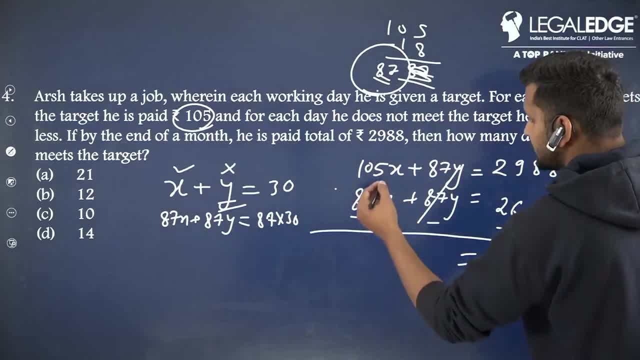 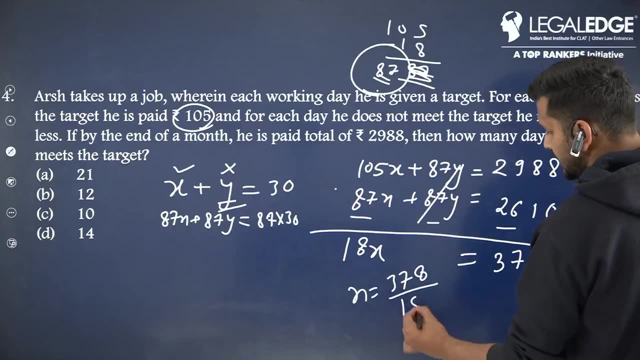 And how much is this? their difference will not be 18,. we know that 7 is in 15, 8, 18x. so how much will be the value of x from here? 378 divided by 18, 18 into 36,, 18 becomes so x equal to 21.. 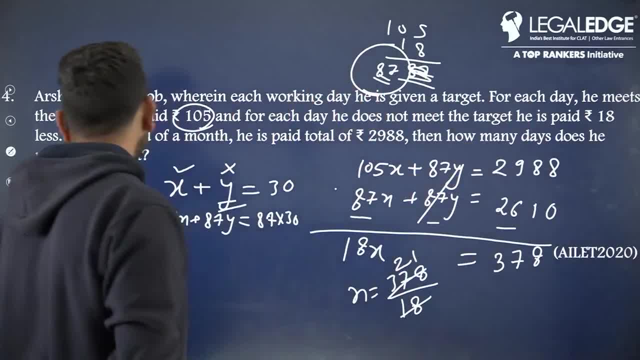 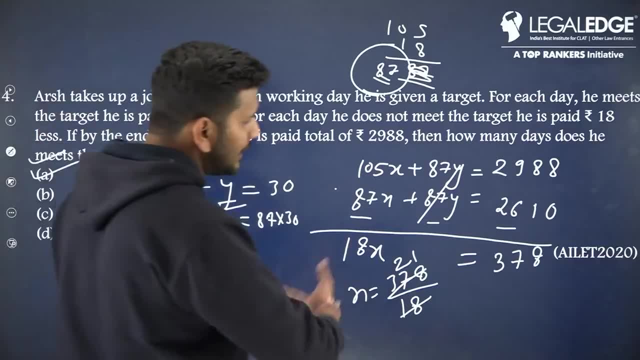 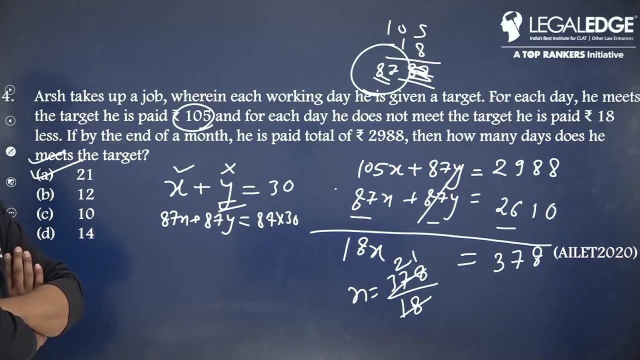 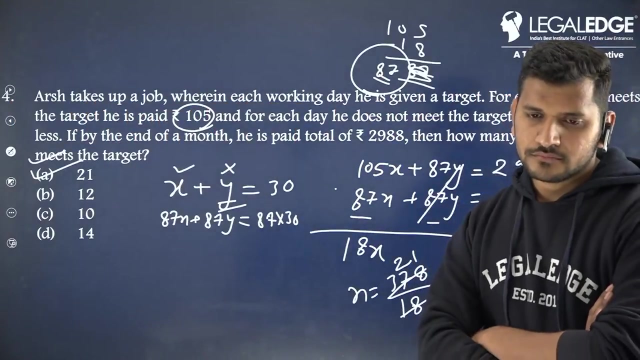 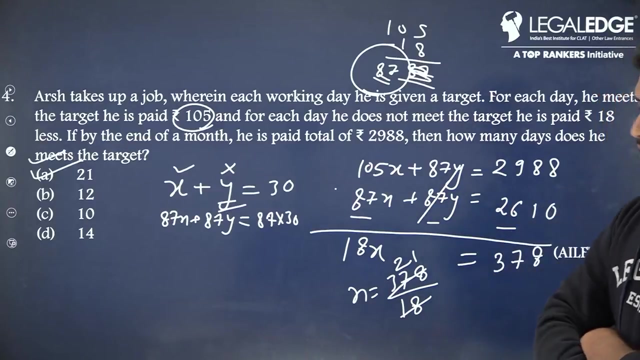 So the question is asking then: how many days does the meat the target? so for 21 days it will get the target. Jyoti, don't make it so long. the elimination method is being solved. Okay, guys, Price Done. 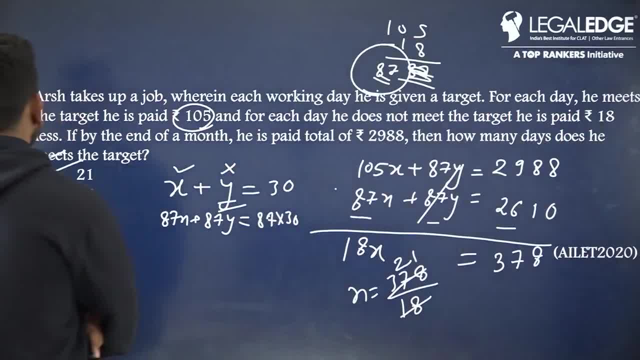 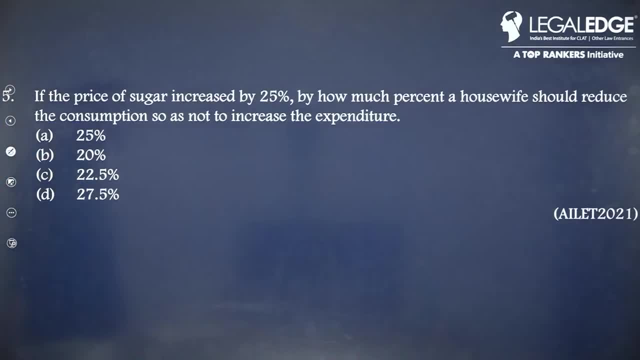 This way you could solve this question Next. Solve this question. Fifth, If the price of this sugar increased by 21 cents, how much per cent? how much per cent house value should reduce the consumption so as not to increase the expenditure? 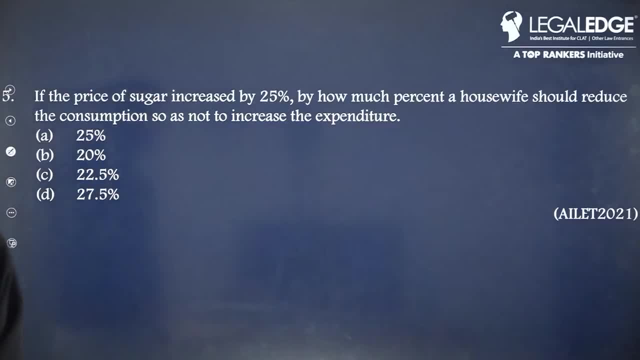 So as not to increase the. this is all based on LH and LH has only come in 2021. Currently, Absolutely. Tell me, from where should I tell this? 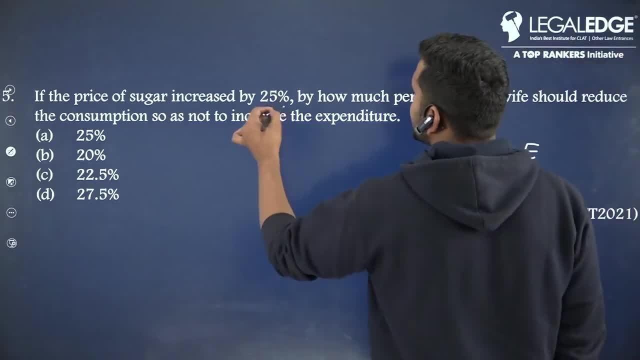 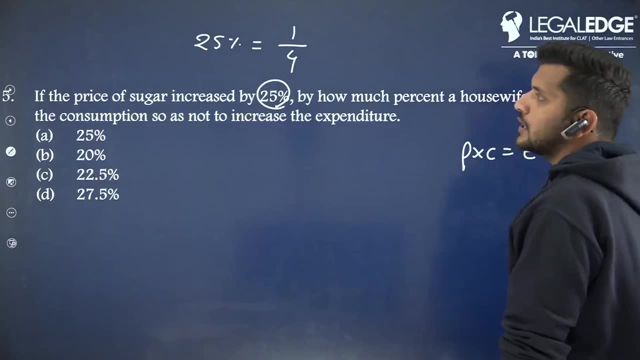 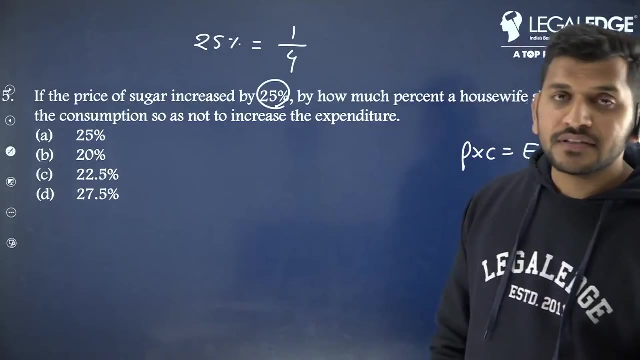 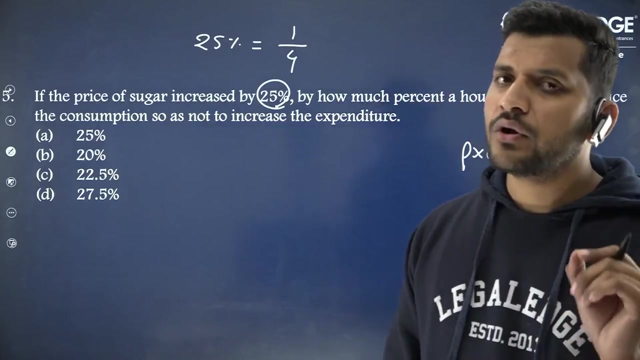 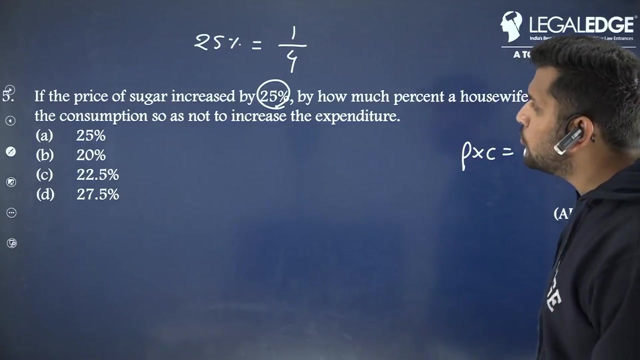 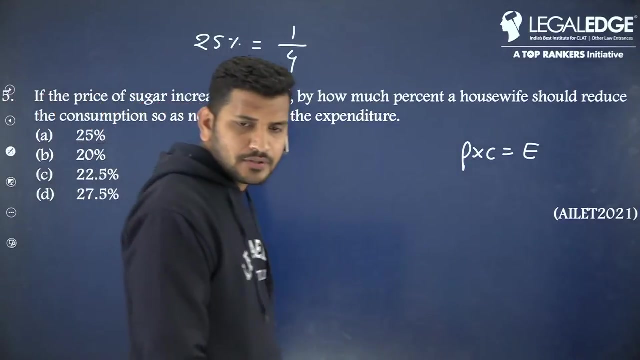 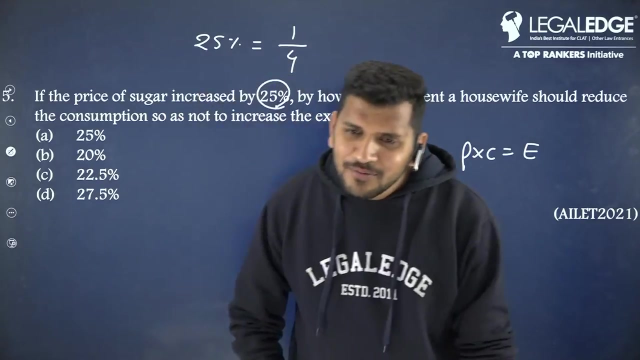 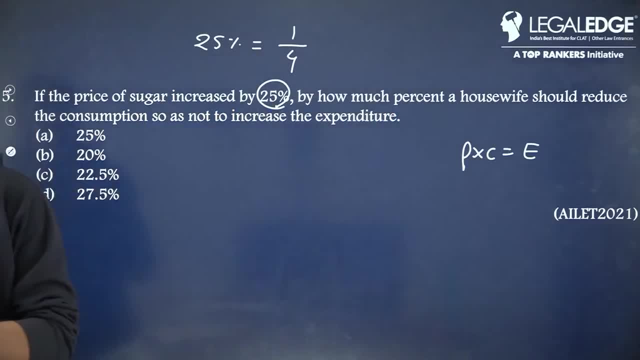 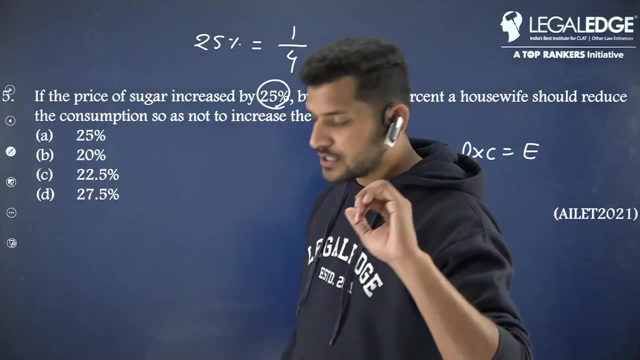 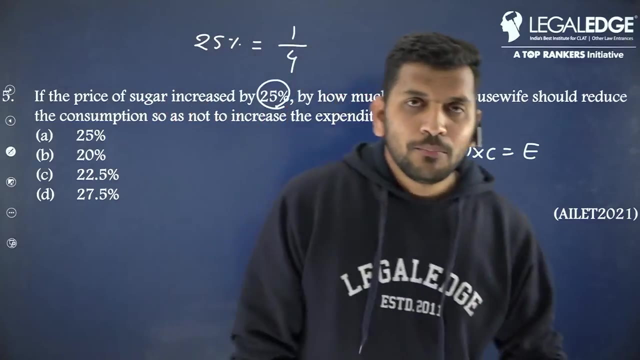 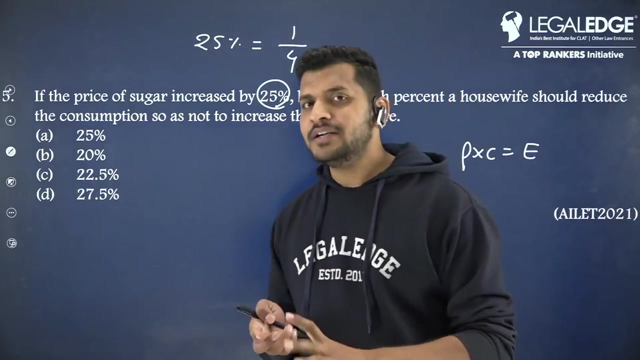 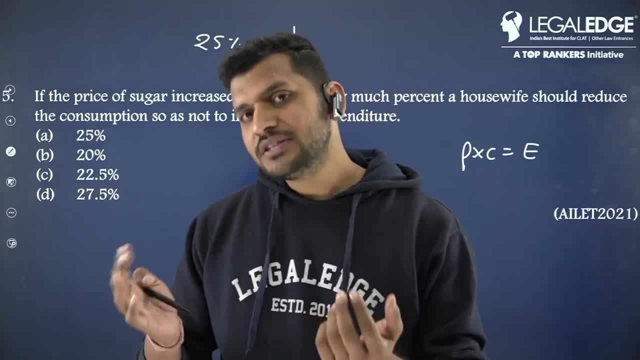 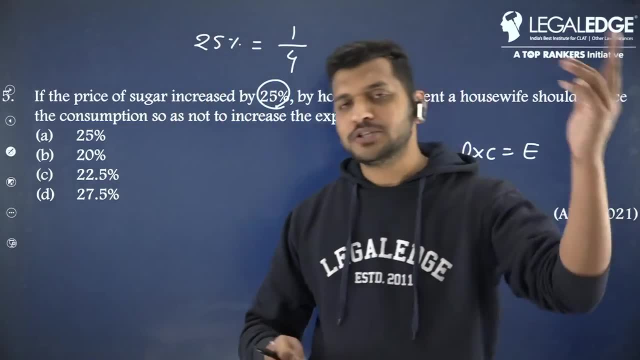 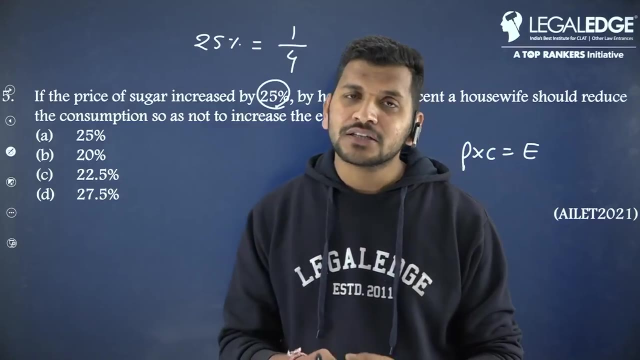 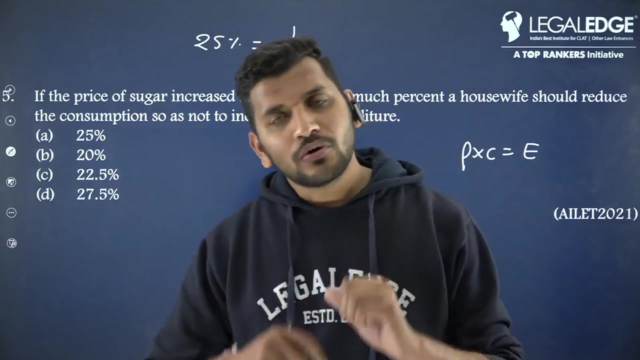 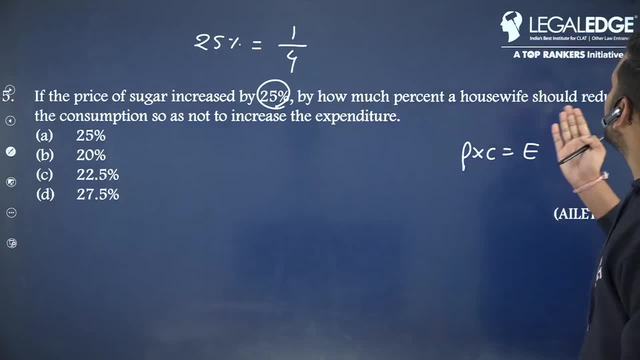 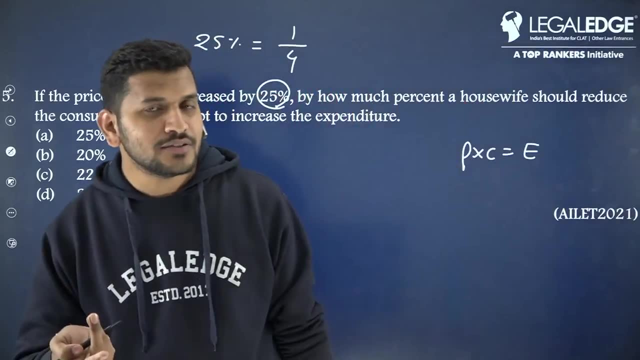 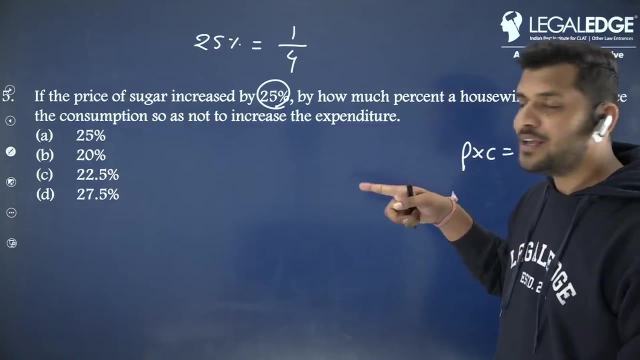 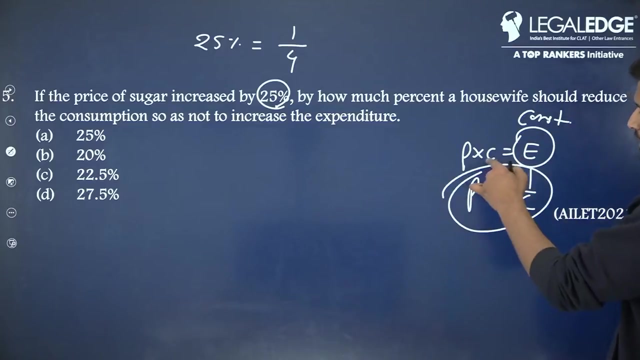 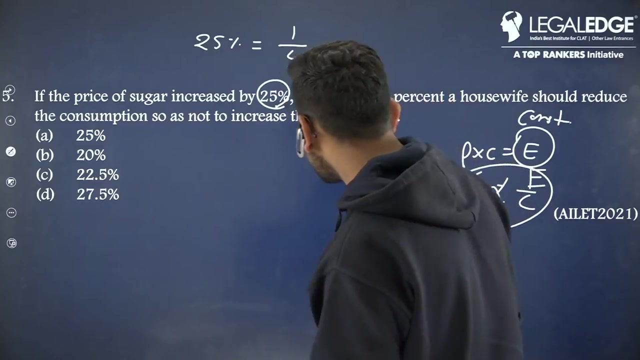 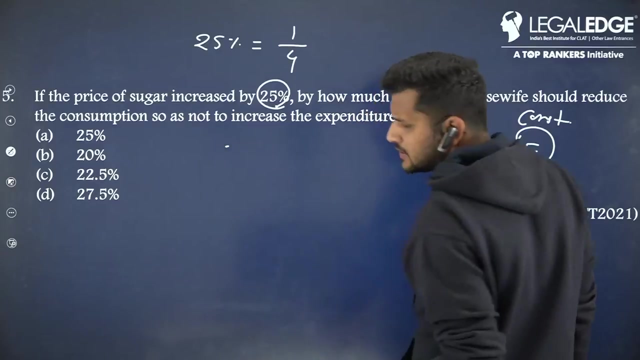 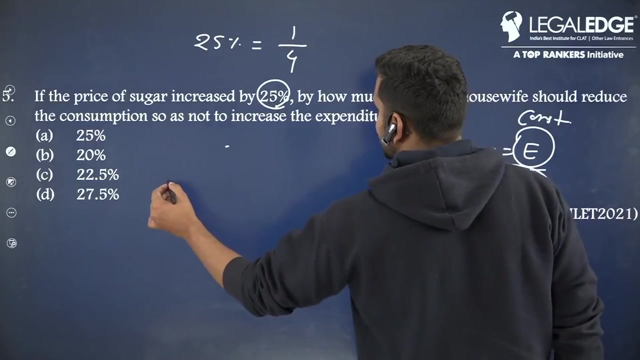 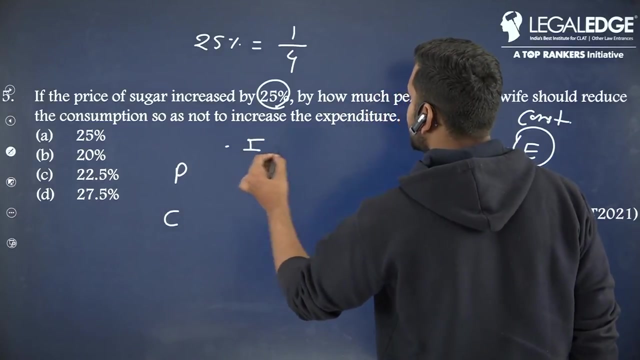 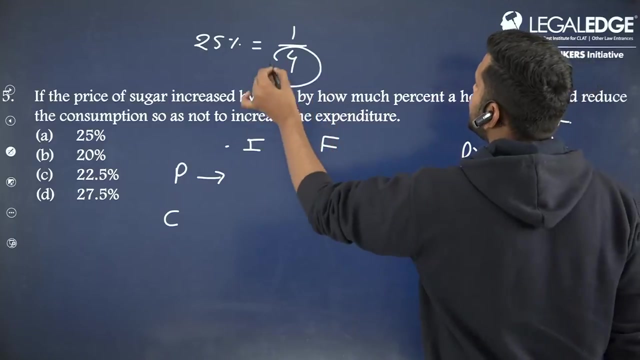 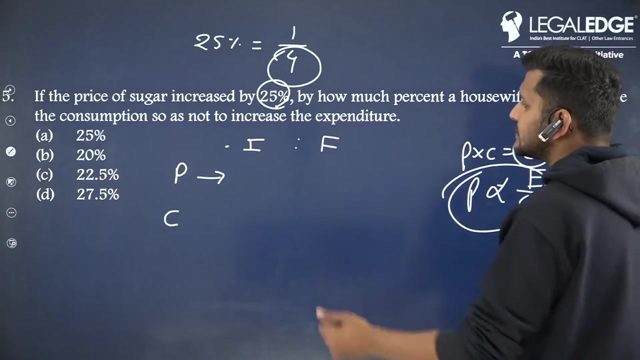 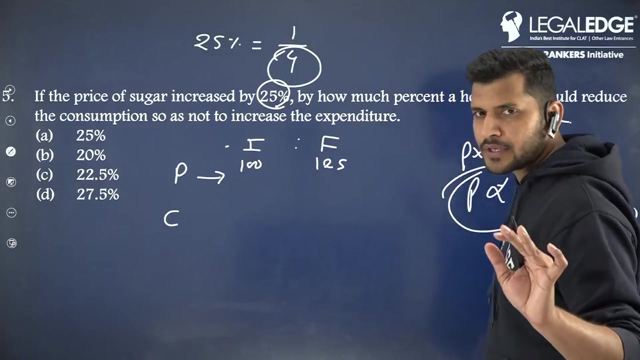 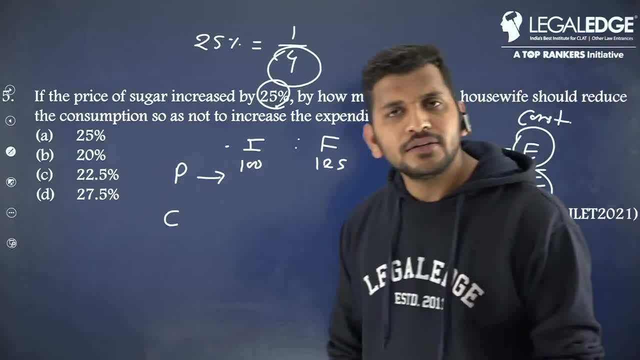 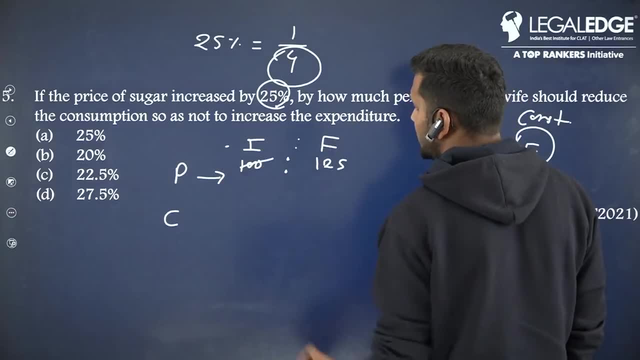 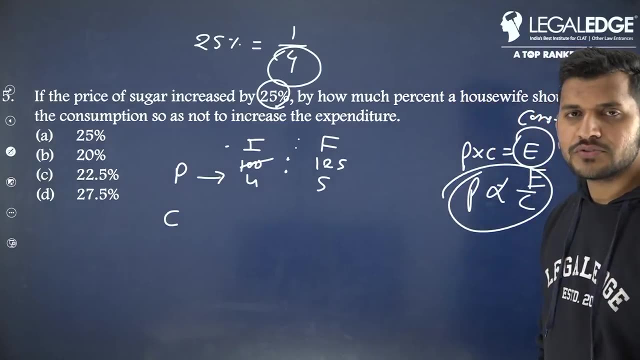 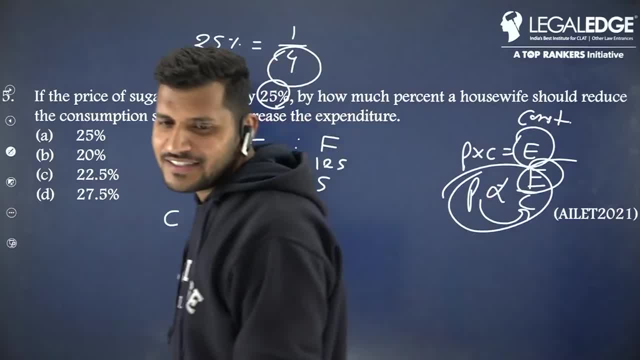 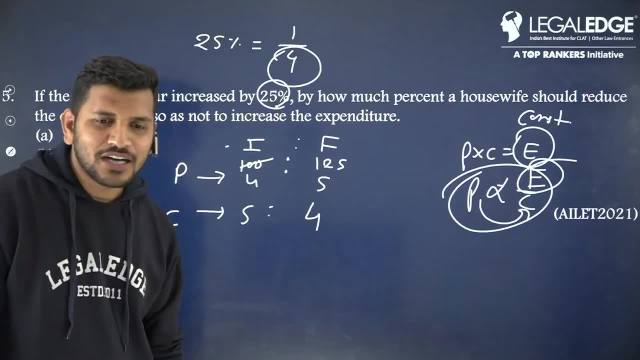 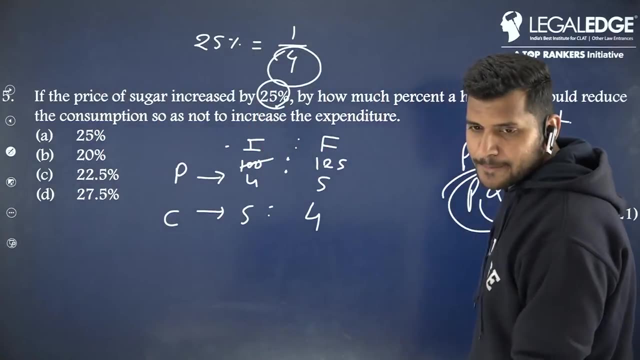 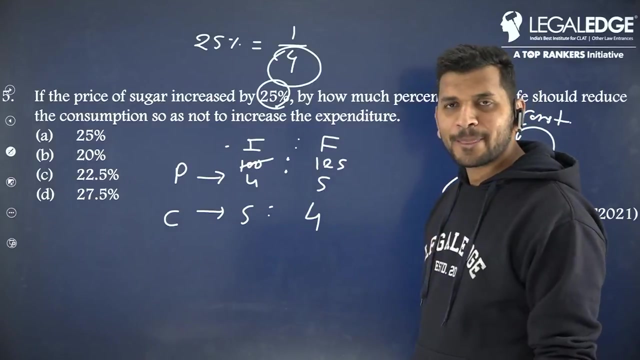 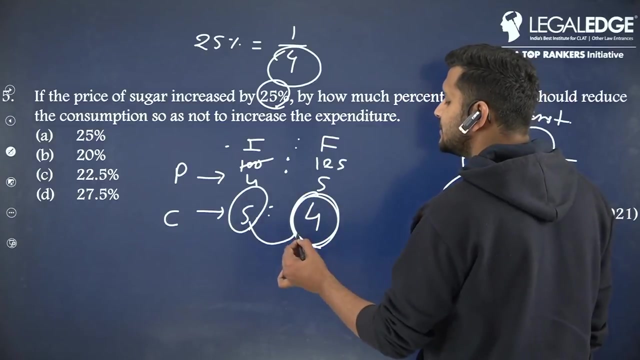 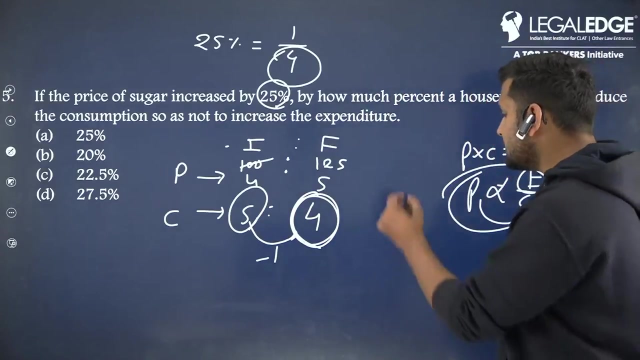 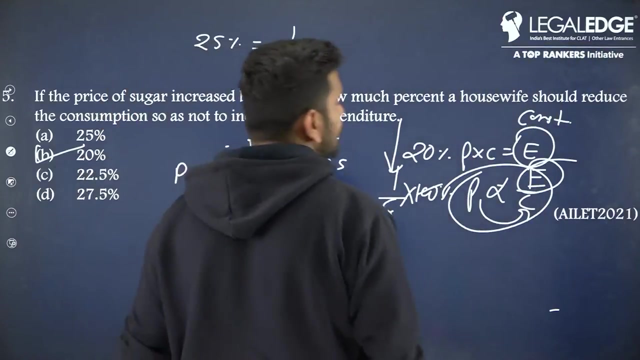 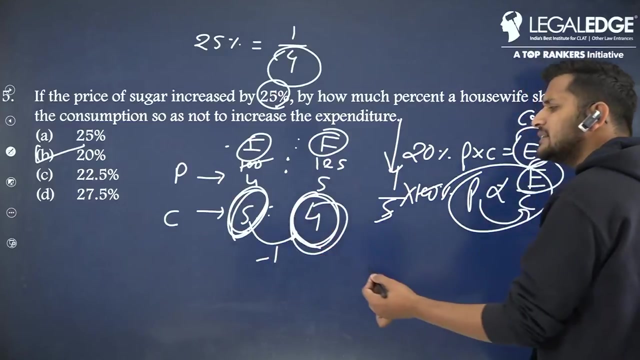 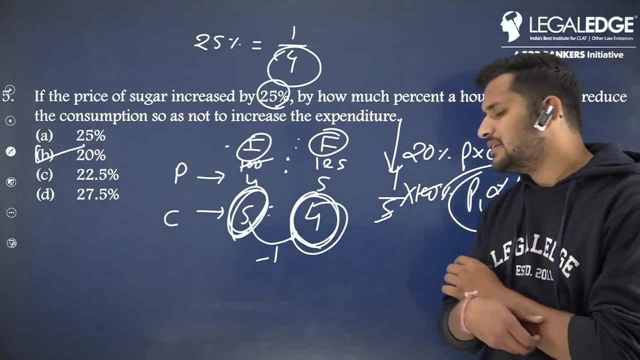 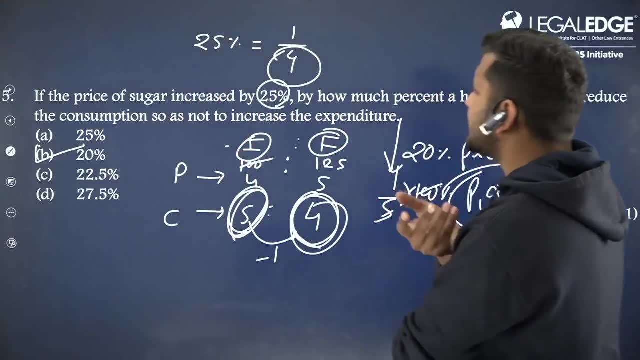 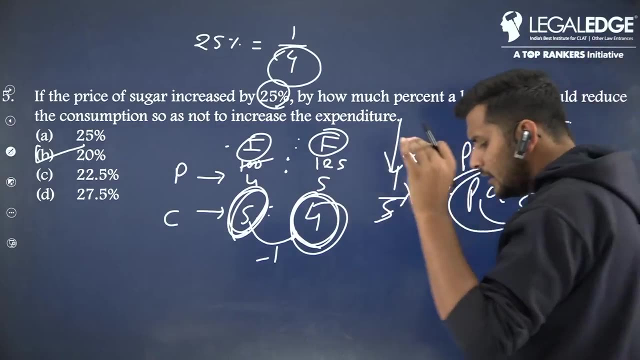 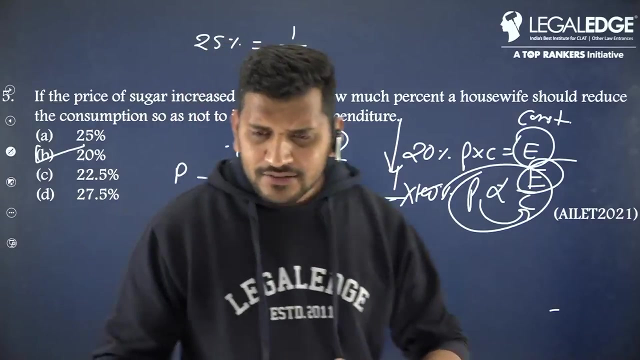 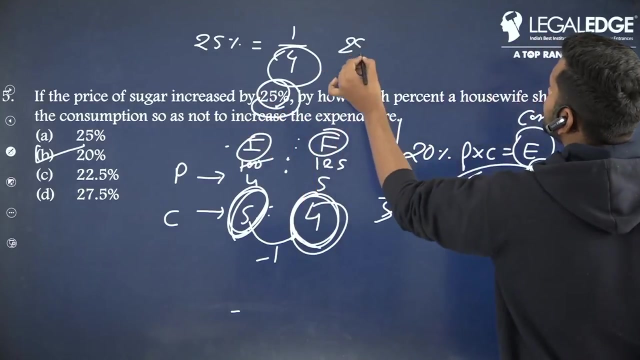 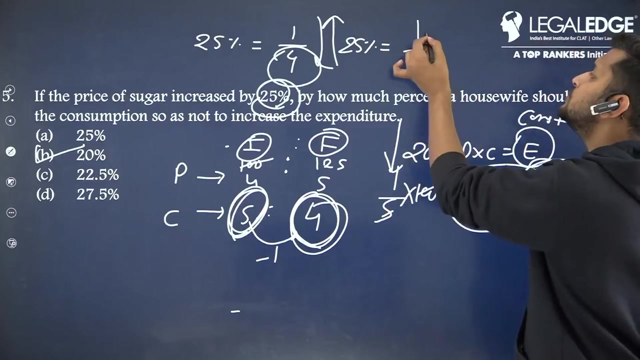 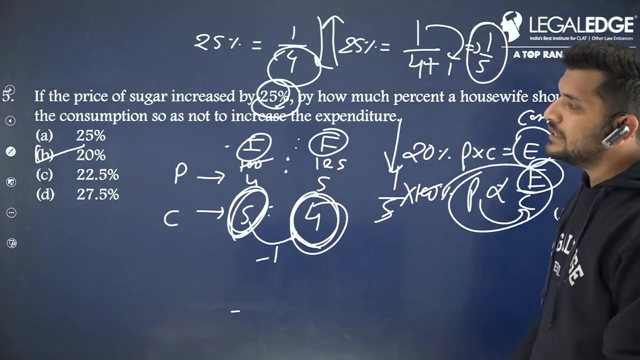 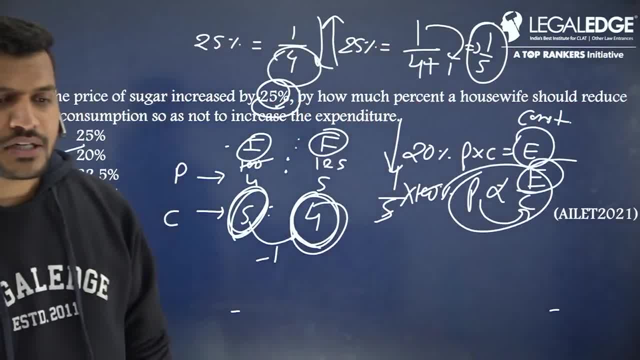 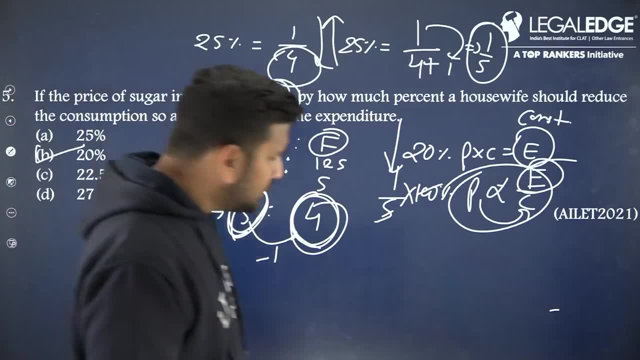 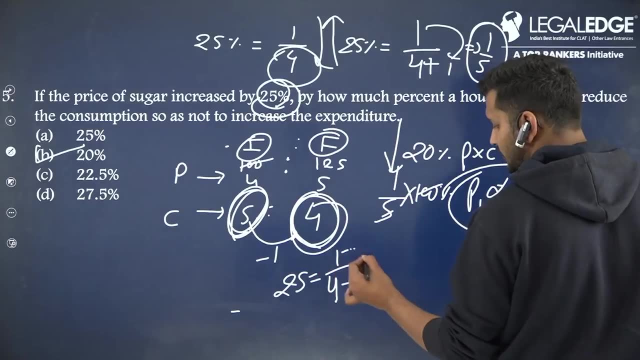 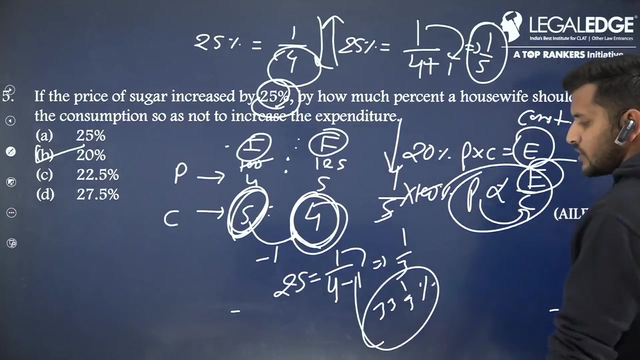 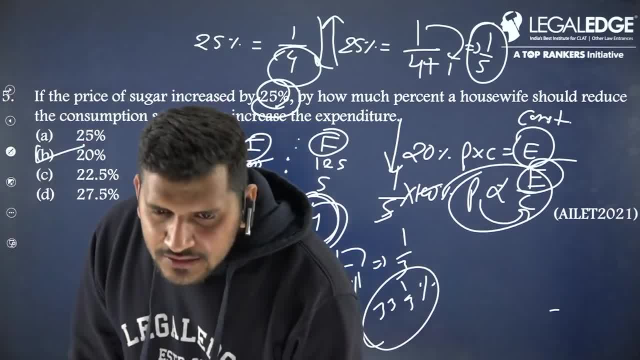 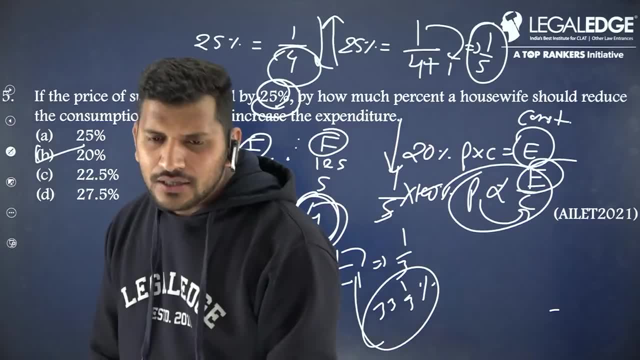 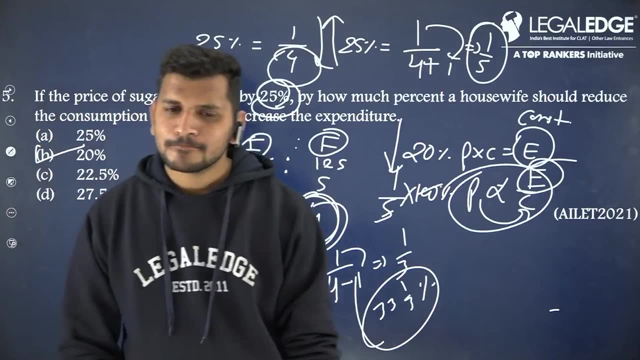 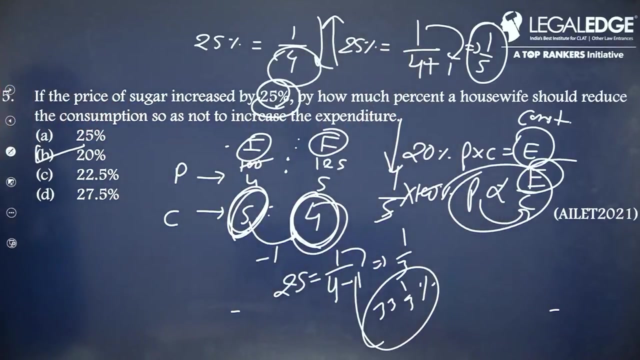 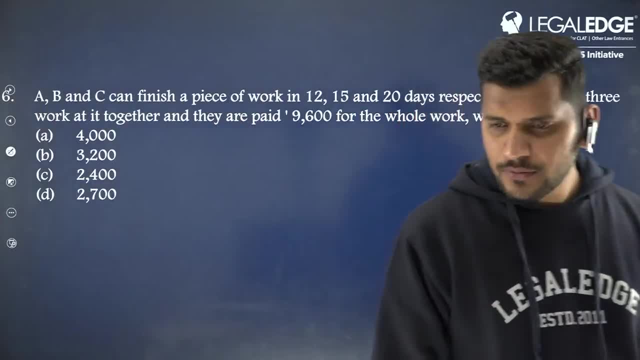 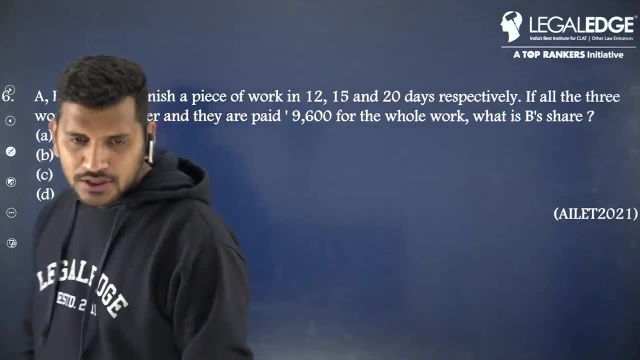 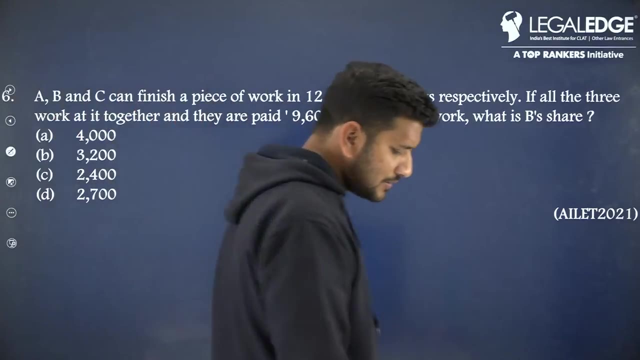 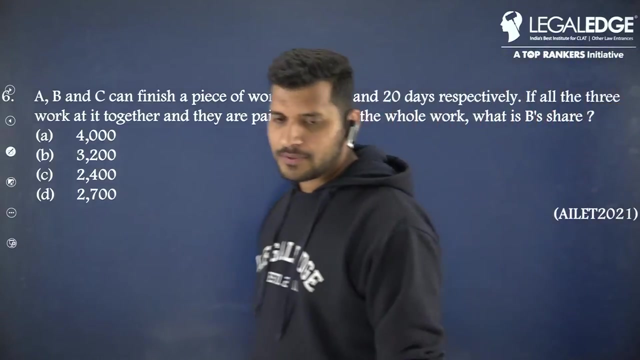 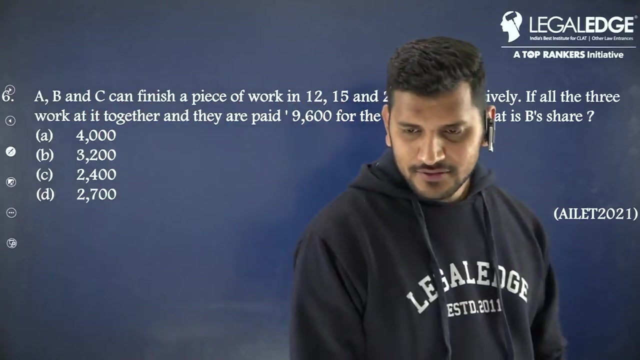 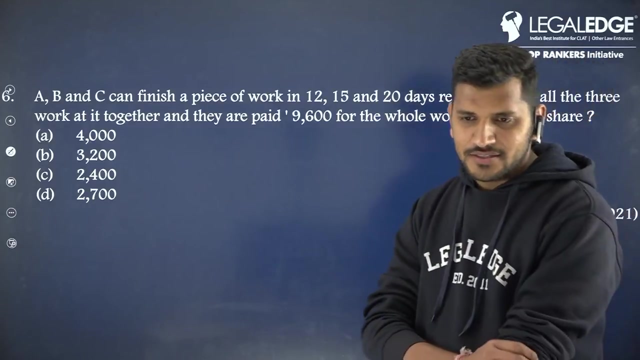 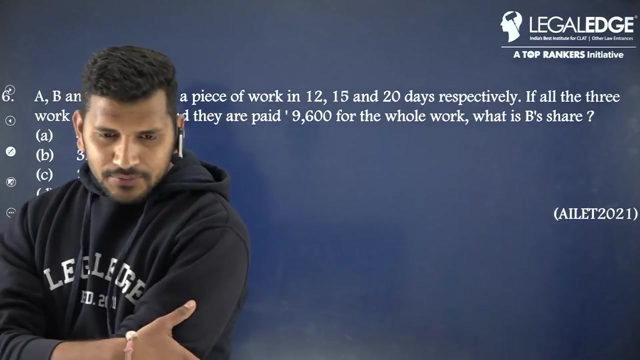 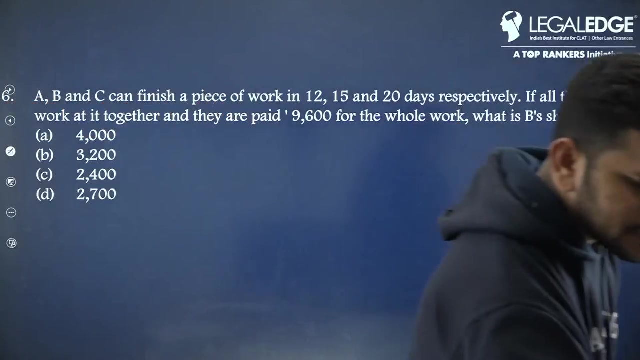 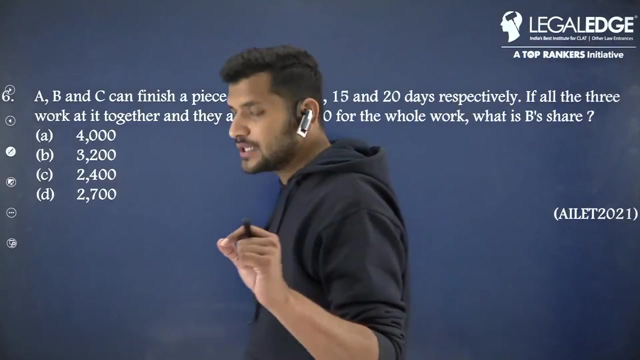 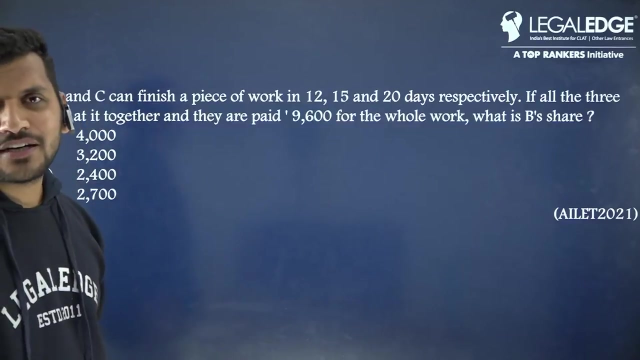 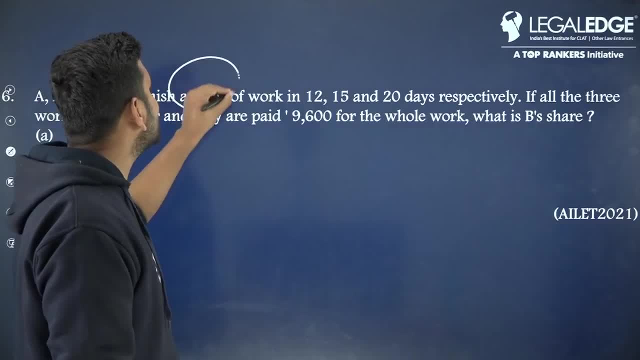 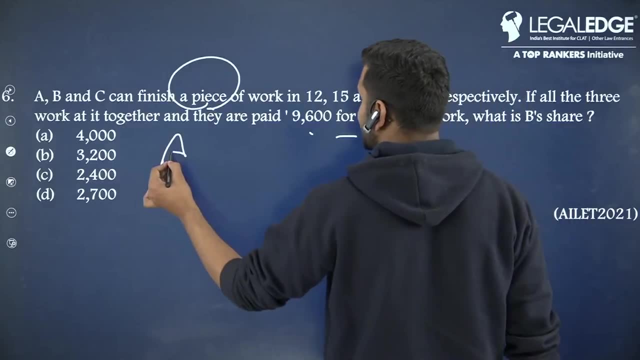 In this question. it is very easy to attach a piece of work In 12 days, 15 days and 20 days respectively. The ABC person If there is a piece of work Means if I am eating bread, So A can eat bread in 12 days. 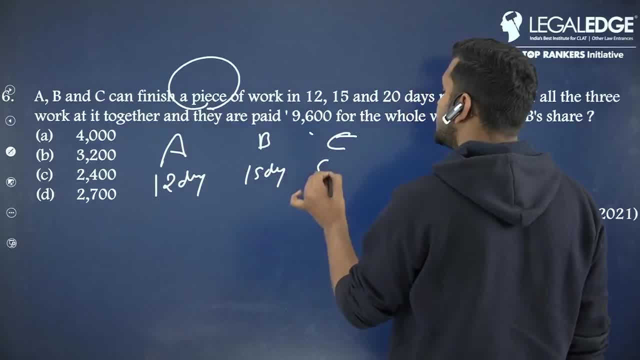 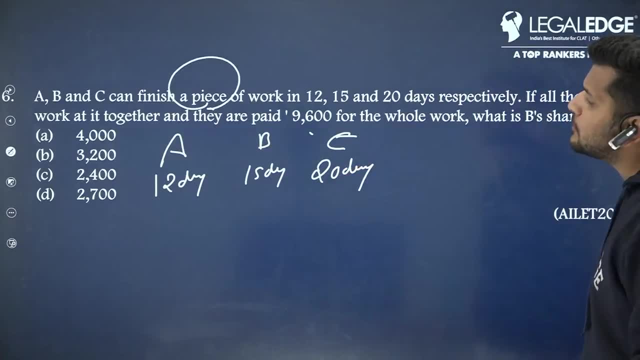 B can eat bread in 15 days And C can eat the same bread in 20 days. This is what is happening If all three work together And they are paid 9600 rupees for the whole work. 26: What is being said in this question? 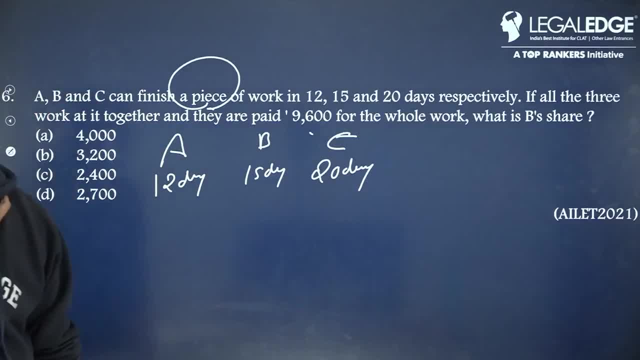 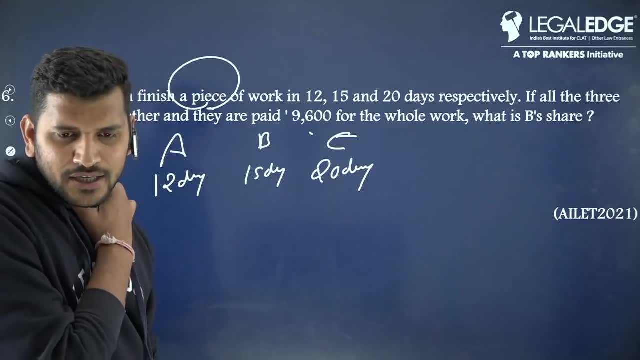 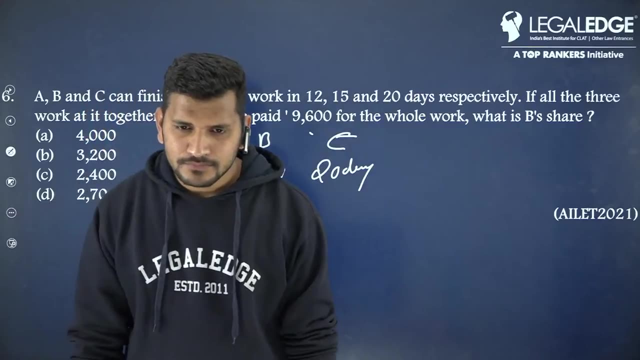 Your class runs daily on YouTube. This class runs daily on YouTube. My class does not run daily. Where do you take the question of circulate? I take legalist Aayushi. Where are you from Legalist top rankers Dharmendra Kumar? This class runs daily on YouTube. 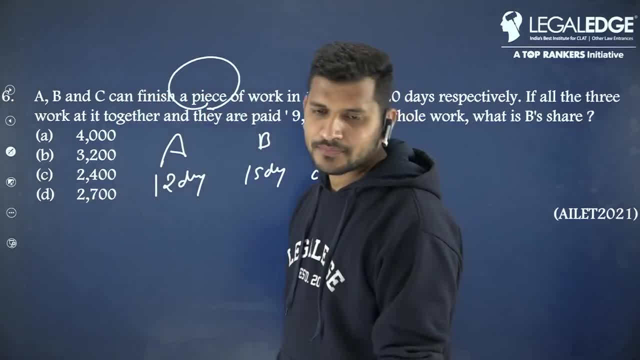 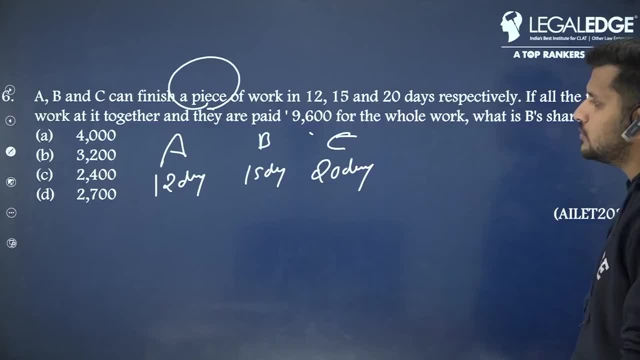 No, no, no, no, no. Sometimes, Listen, listen What is being said. ABC finance a piece of work in 12,, 15,, 20 days. Okay, fine, Someone was going to do some work. They were doing labor A, B, B, C, B. 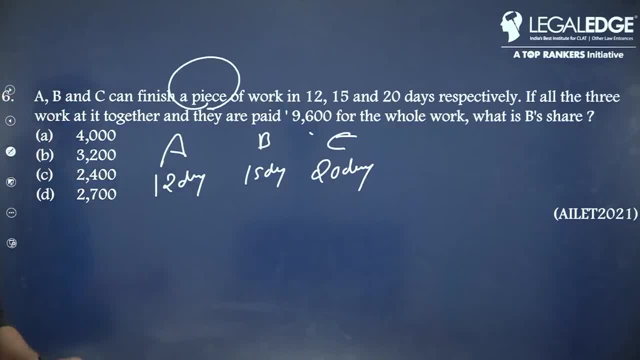 A did the same labor in 12 days. Did the same work. B also finished the same work in 15 days And C finished the same work in 20 days. Got it? Guys, whenever you have to question time in work, So take their LCM in whatever days. 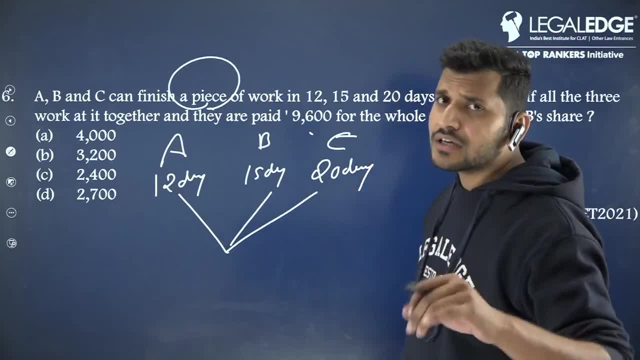 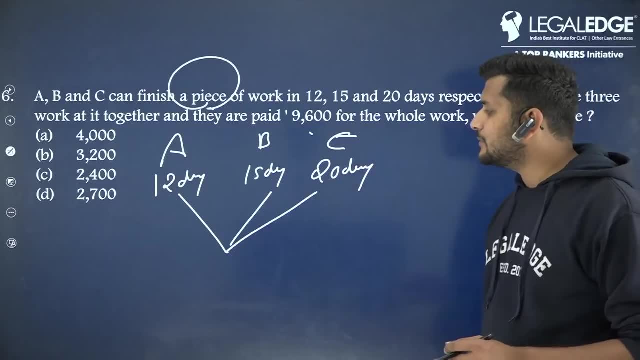 Because same work, A is also doing the same work, B is also doing the same work, C is also doing the same work. When the work of A is done from A, It completes in 12 days, And guys, it is done from B, It completes in 15 days. 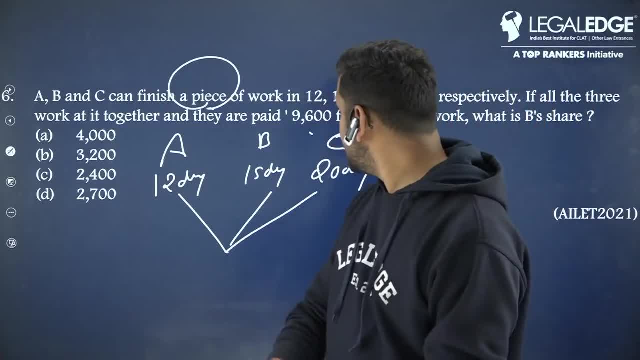 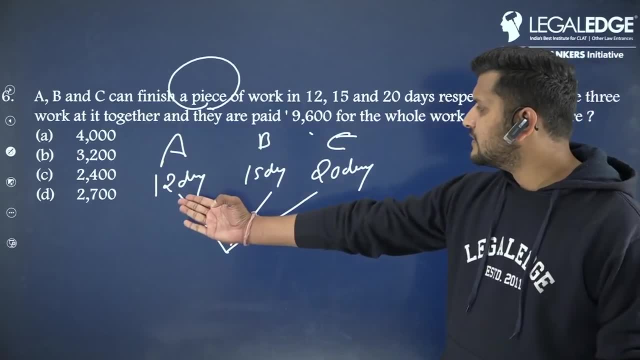 It is done from C, It completes in 20 days. So in how many days Their efficiency is less somewhere He is doing it. in less days Means his efficiency is more. This is a little more than him. Means this is the most efficiency of his. Then less than him. 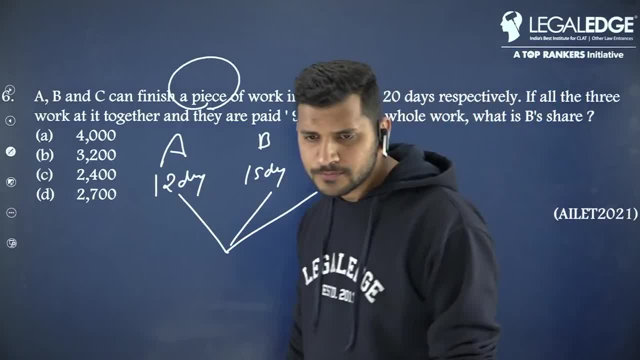 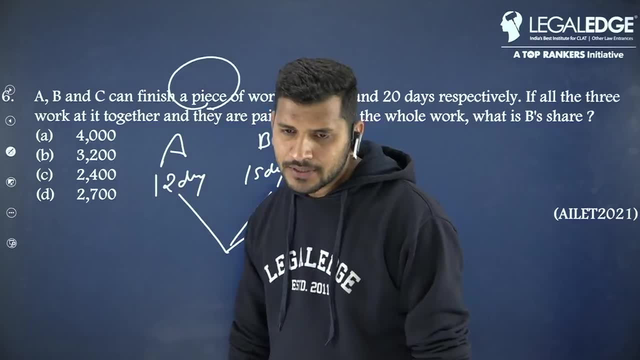 Then less than him. Do you understand my feelings, Sir? which LCM, Which book do you take? for CLAT, For CLAT, there is a CLAT list here And there is RSM Enough. So your class runs in Lucknow. No, not in Lucknow. 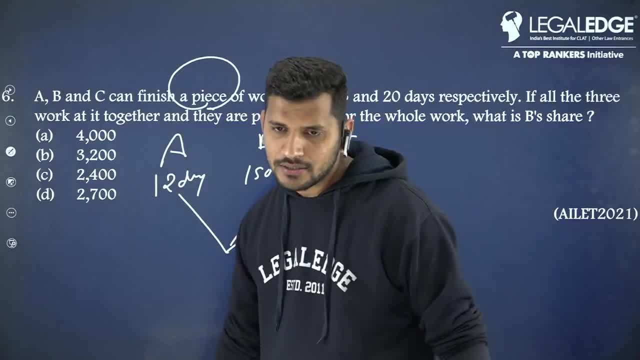 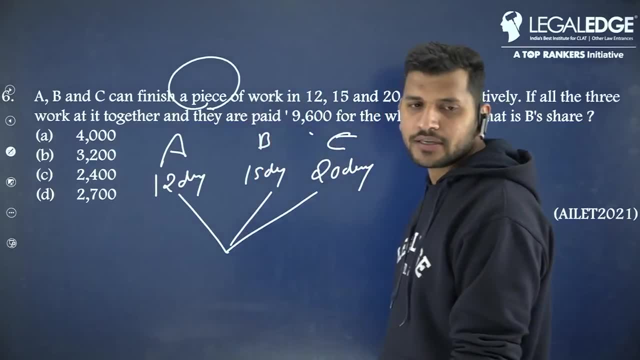 Deepak is in Bhopal. I am from Bhopal, NIL Taking class in Bhopal, Right, Okay, okay, okay, See you. So, guys, A completes in 12 days, B completes in 15 days, C completes in 20 days, Whenever you have to complete this type of question. 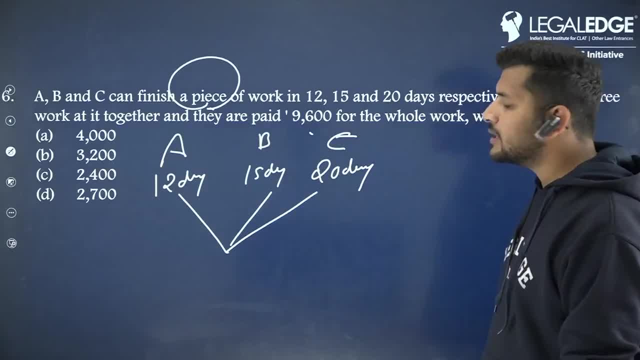 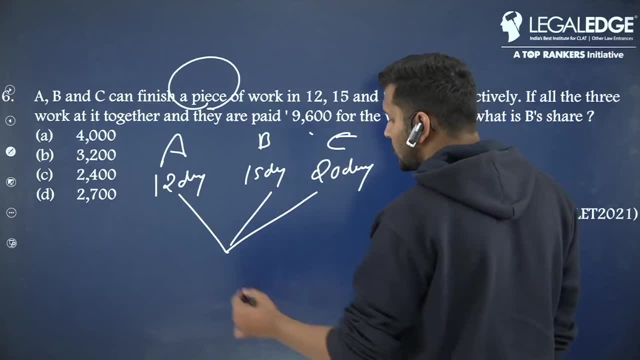 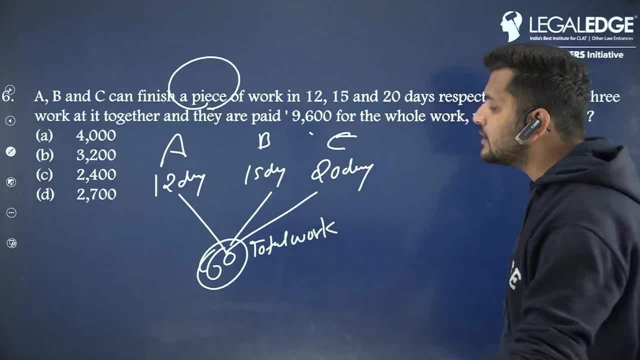 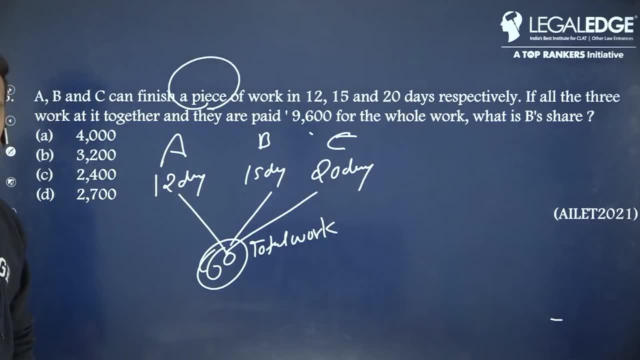 Their LCM. What do we always have to take? We have to take their LCM That A completes that work in 12 days, B completes in 15 days And guys C completes that work in 20 days. Have you understood the thing? Absolutely, sir. 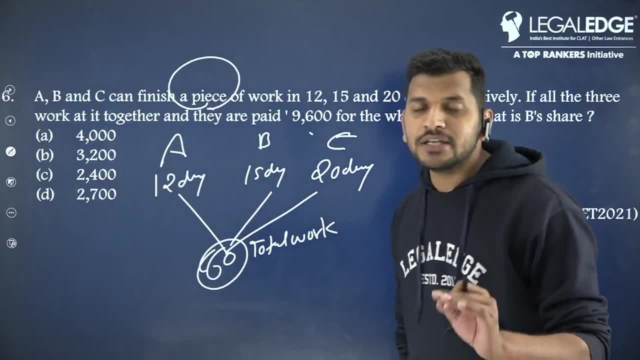 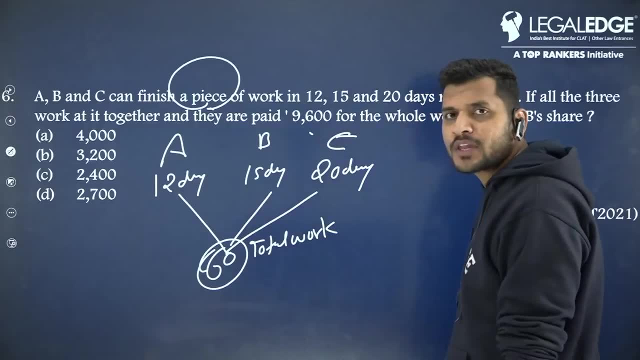 So, guys, what do we have to do? Take the LCM of these days, And the LCM is called total work, Means total work was 60 units, 60 parts. Now let's see what is the work per day. You tell me this. Do you want me to answer the question? 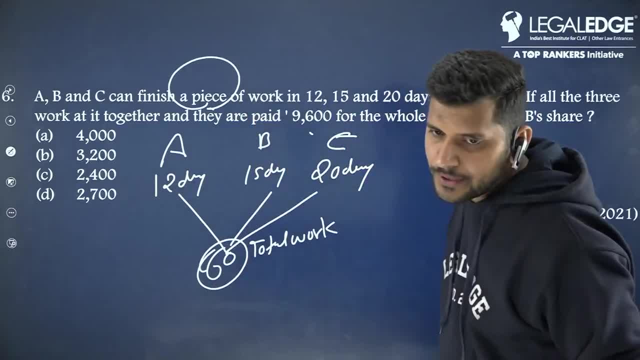 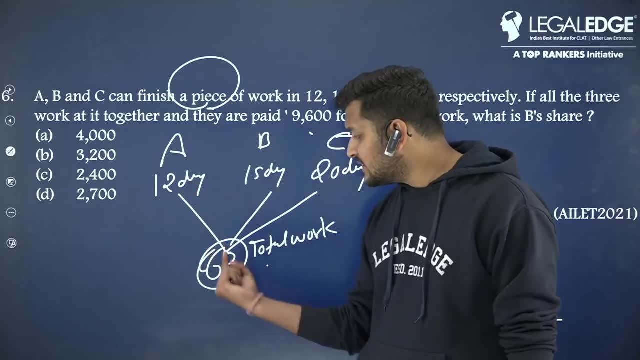 I don't know. So the answer is 31. Okay, So, guys, you tell me this That this 60 units total work, 60 units total work, A has to do 60, B has to do 60, C has to do 60. Now don't say in your mind: 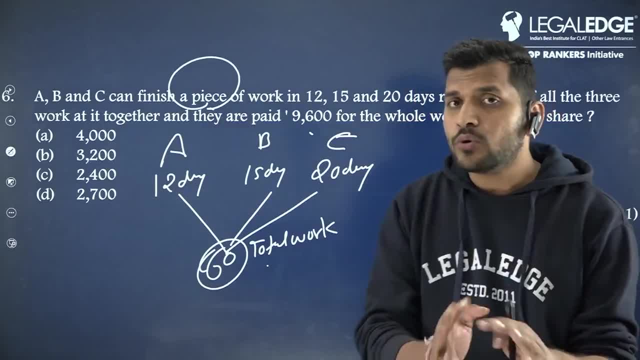 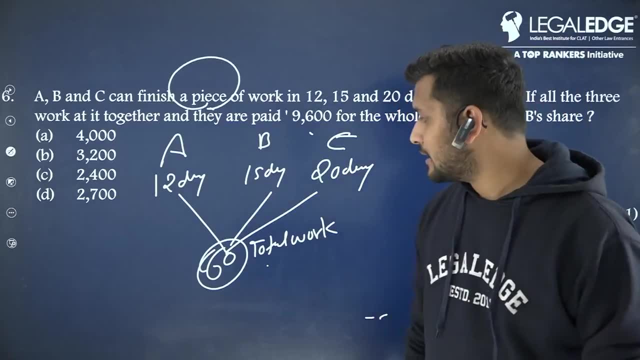 Sir, will it be 60?? You can take 120, You can take anyone, No problem. You can take 1, You can take 2, No problem. The answer will be same. But why did you do this? You will understand now. Okay, He does 60 units in 12 days. 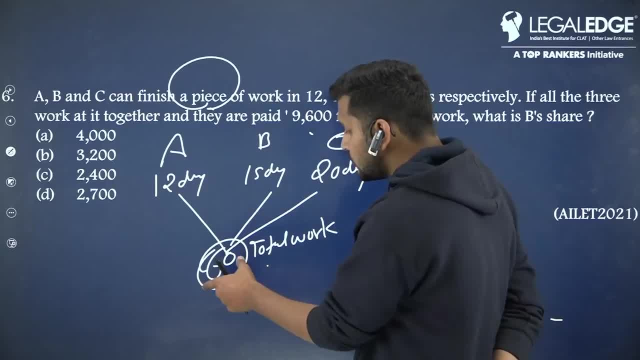 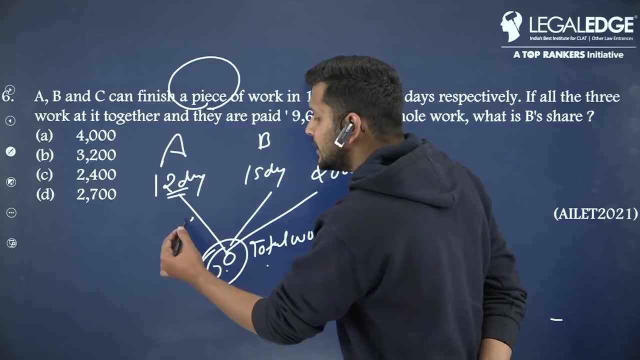 So how much will he do in one day, guys? A person completes 60 units in 12 days, So how much will he do in one day? If we divide 60 by 12, So will he do 5 in one day. He will do 5 units in one day. 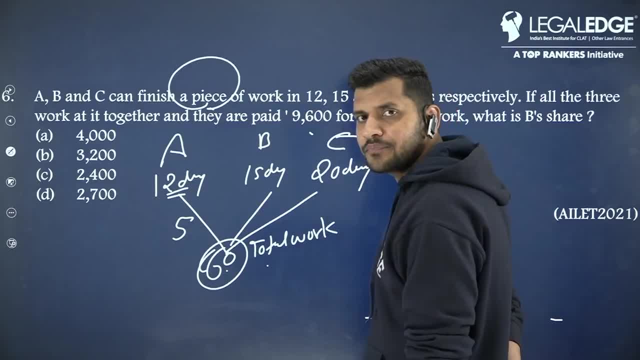 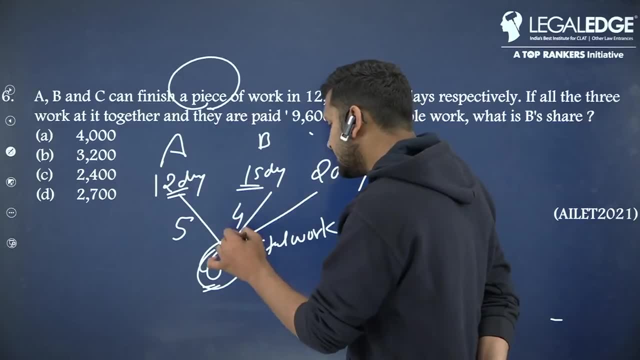 Now see here What is B doing. What is B doing, guys? He is completing 60 units in 15 days. So how much will he do in one day, Sir? he will do 4. He divided 60 by 15, Sir. see the LCM. 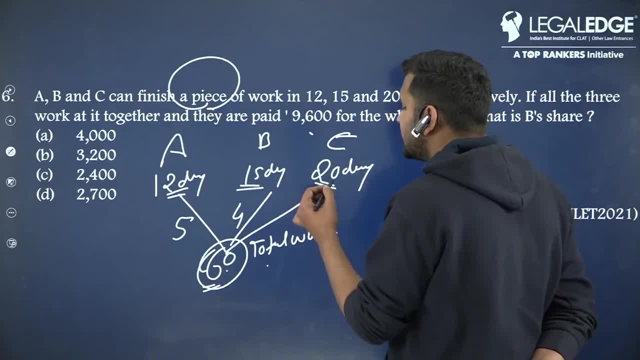 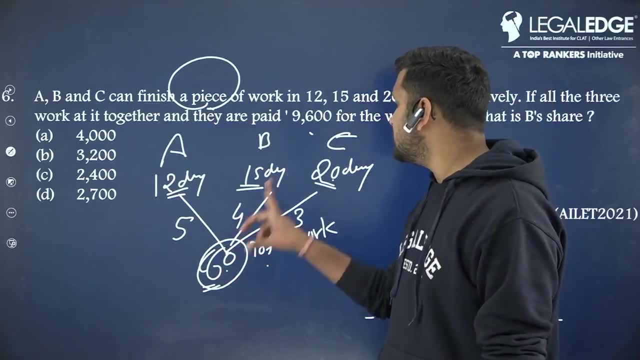 How many days is C doing Sir? he is doing this work in 20 days. How much will he do in one day? 60 by 20, He will do 3 units in one day. A works 5 units in one day. B works 4 units in one day. 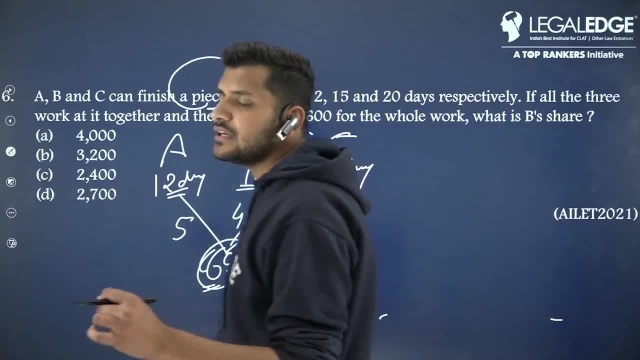 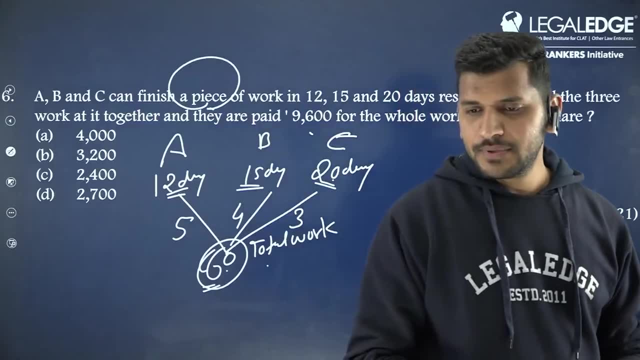 C works 3 units in one day. So their efficiency is the work done in one day. What is being worked in one day is only their efficiency, guys. What is the matter, sir, Amit, Sir, works 5 units in one day, 4 units in 1 day. 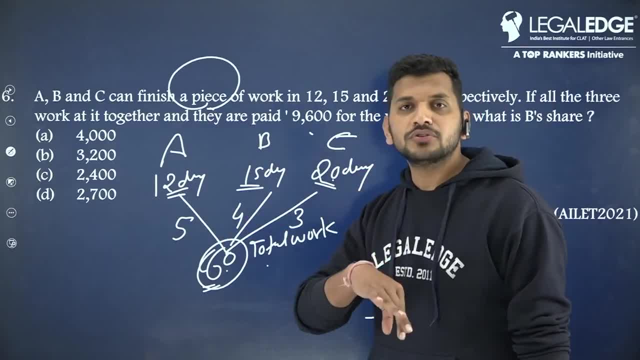 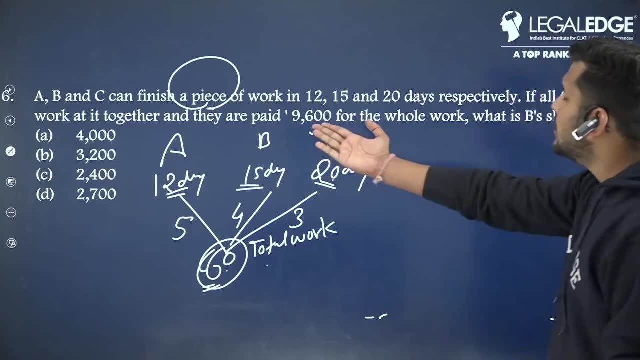 3 units in 1 day. So the work done in one day is only their efficiency. That is their efficiency. Absolutely correct, sir, it is their efficiency. So now the money that has to be divided according to their efficiency, you don't have to do anything. 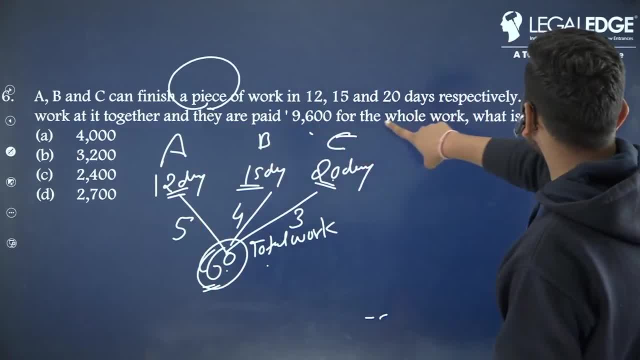 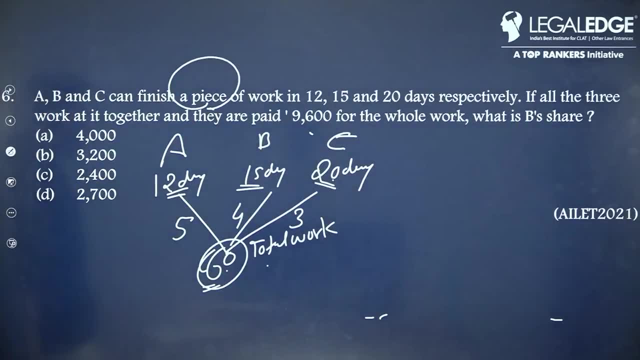 Your answer will come directly. What is he saying? And they are paid 9600 for the whole work. What is the wish here? So what will you always do? Divide the money according to their efficiency. So A will get 5 parts, B will get 4 parts. 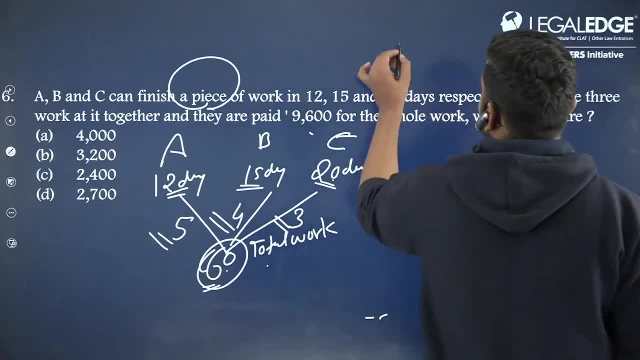 C will get 3 parts. So how much money has to be divided in total? So 9600 has to be divided in all three. So how much in all three? Sir, 5 parts this, 4 parts this, 3 parts this. 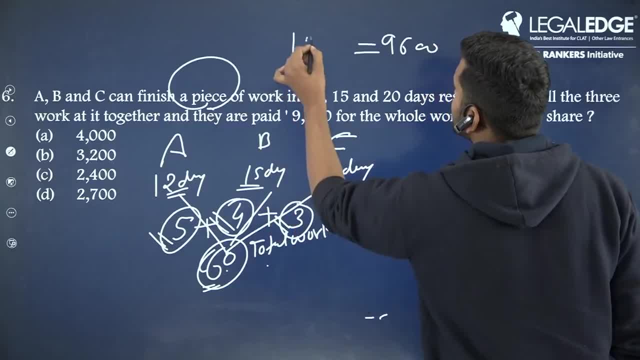 5 plus 4,, 9 plus 3, 12.. Sir, 12 parts equal to this much has to be in all three. All three, 12 parts is equal to 9600.. So, guys, how will the value of one part come out? 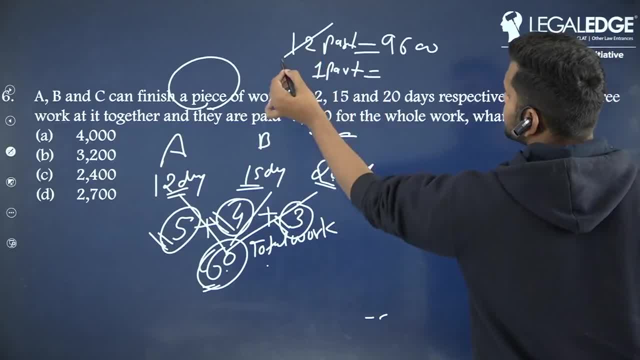 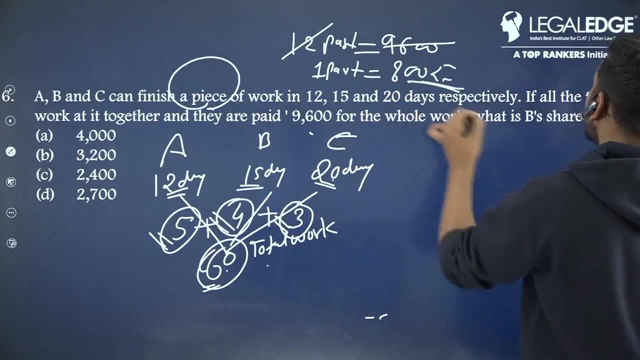 Sir, we know how to get it out. Okay, 12 is 8000.. We will divide it by 12.. 800 rupees is the value of one part. But the question is, how much did B get, Brother, these 3 parts? 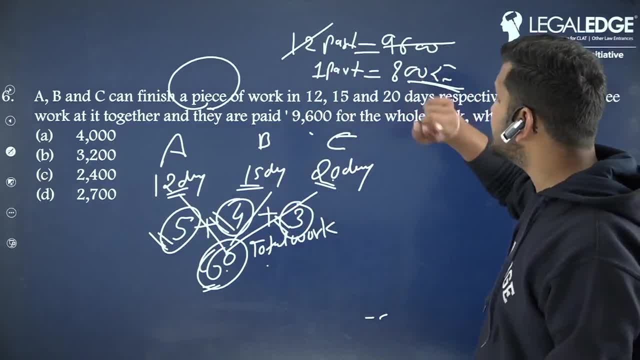 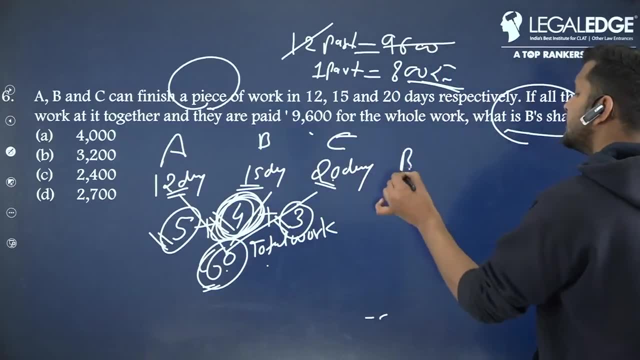 5,, 4, 3.. If we divide all three by 12, then it will be 9600.. One part will be 800.. I just have to find out B's value, And how many parts does B have? 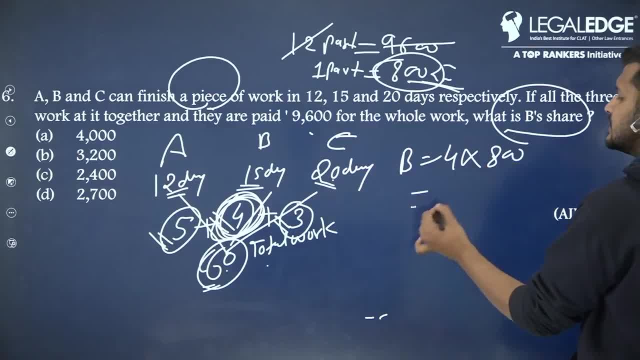 Sir, B has only 4 parts And you have found out the value of one part, 800, which we could not find out. So 8, 4, 3, 200.. The answer will be B. Is it clear or not? 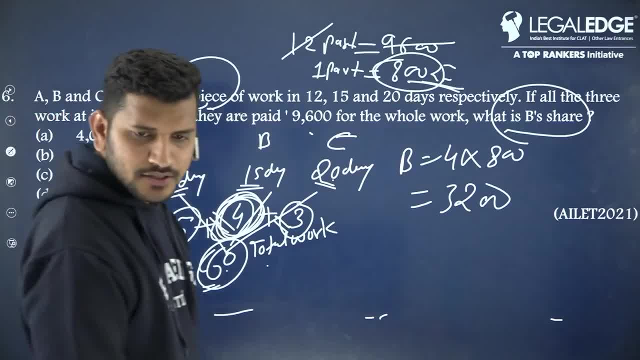 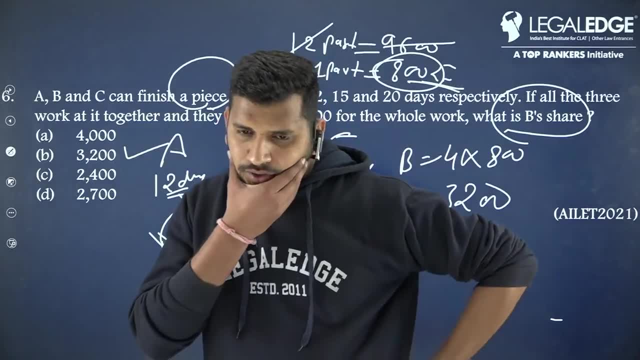 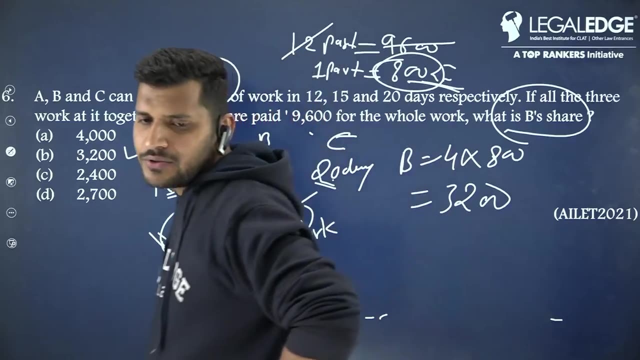 Efficiency ratio. yeah, What's the matter, sir? Sir, for math, the book is legal. Where can I get it from other than the course? Please say: Hey guys, who is Pranay? Are you only talking about CLAT? 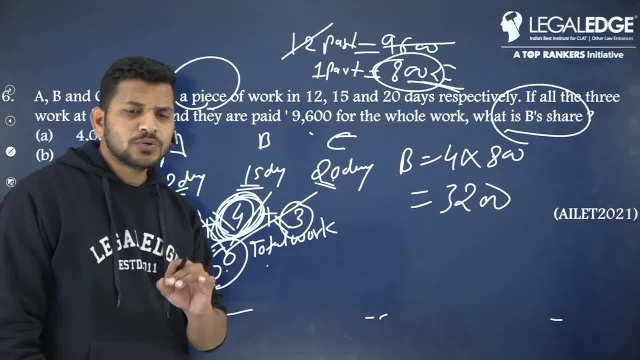 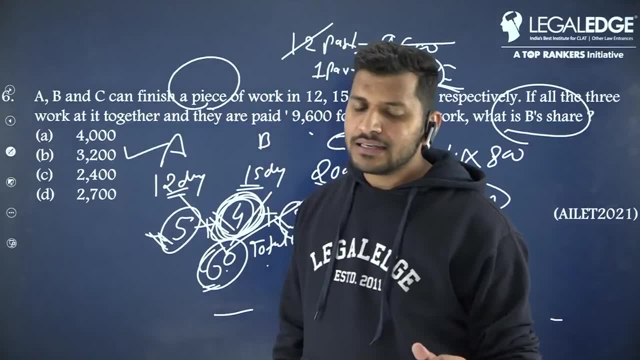 Is it clear, sir? Okay, Do you want to talk about CLAT or ELIT? Is RS Agwal best? for ELIT, Is RS Agwal best, But if I talk about CLAT, because legalists have a lot of DI questions- 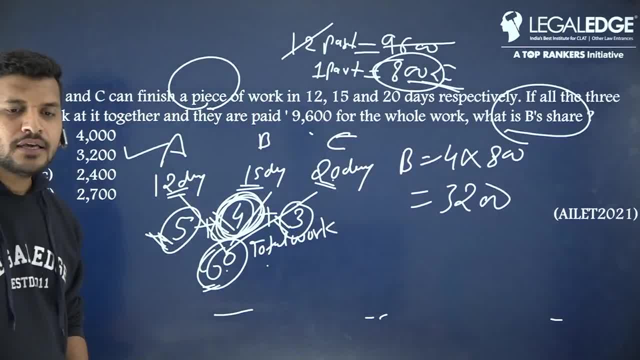 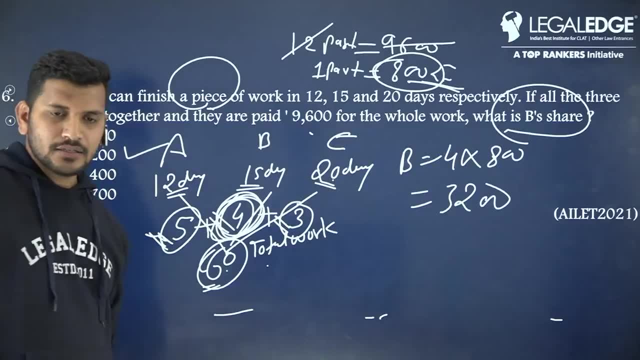 Case lead. DI comes more in your CLAT. That's why I am saying that you should at least take a CLAT list from here. A CLAT list comes with a book and an RSM comes- RSM 4 and CLAT list. 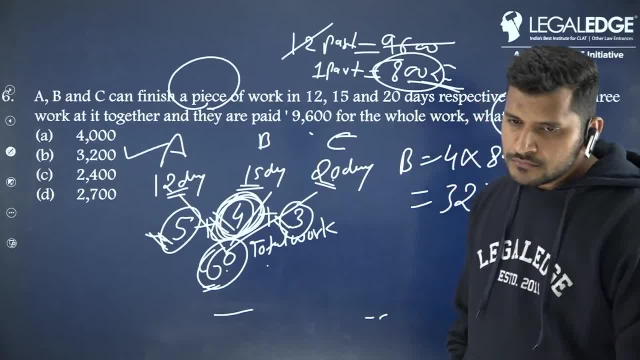 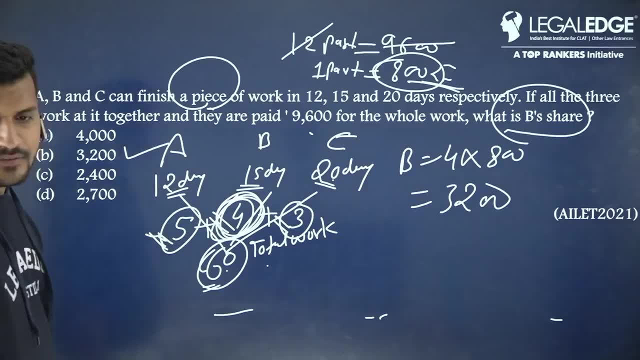 The DI in RSM 4 and a CLAT list. those two books are enough. Okay, So this was about ELIT, Now let's talk about CLAT. Let's talk about CLAT too. Okay, okay, okay, okay. 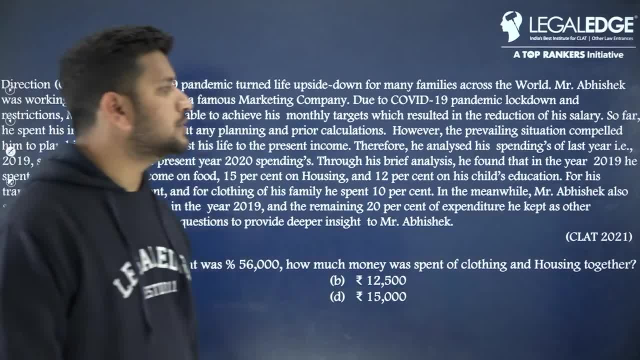 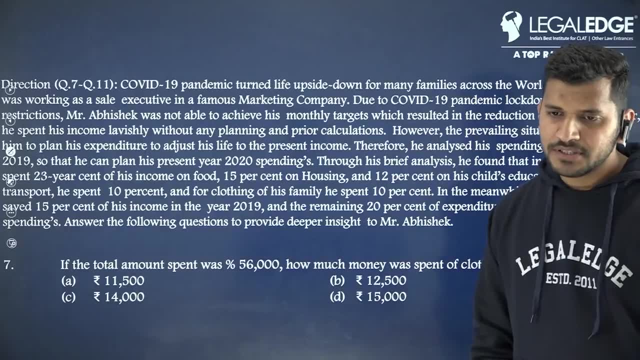 Next, This is a CLAT question. This is a good question. This was a good question in CLAT 2021.. This is a good question. Life will change. Anuj Maheshwari, you are also here, Very good. 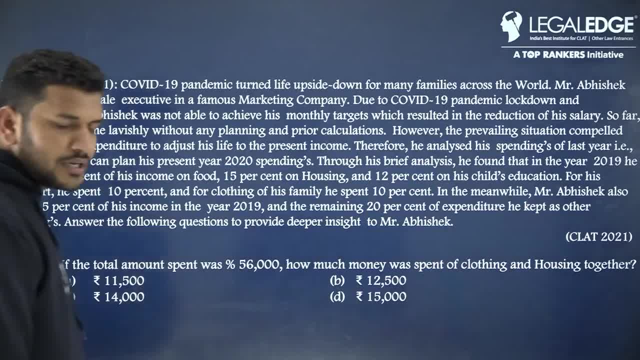 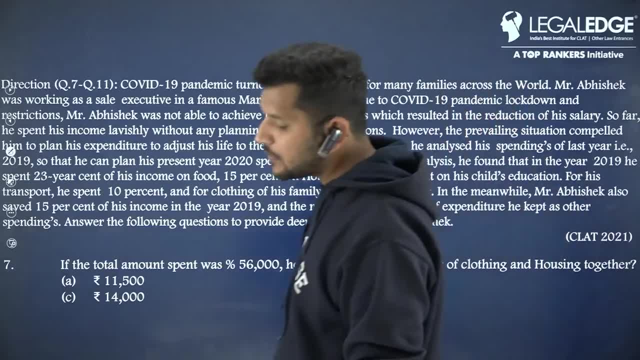 Take it for ELIT. Your work will be done with RS Agwal And if you want to talk about CLAT, you will have to apply a case lead DI. For CLAT, you will have to apply a case lead DI For CLAT. you will have to apply a case lead DI. 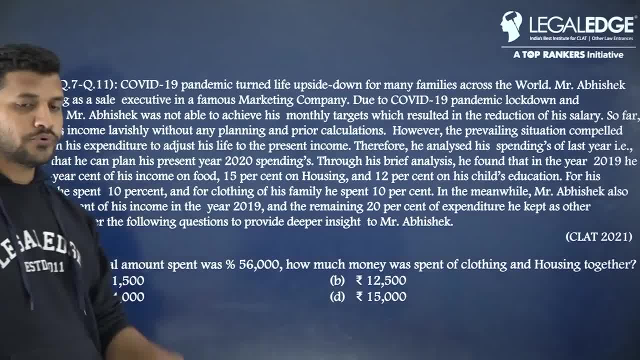 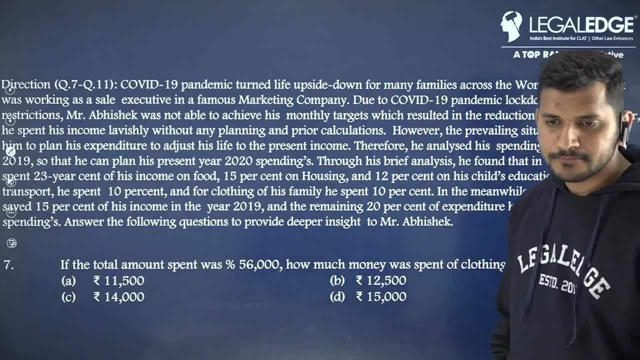 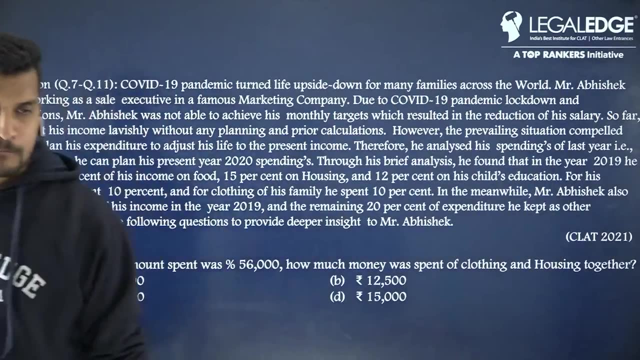 You will have to apply a case lead DI Here. CLAT list and RSM 4 are used for MASS. Clat list and RSM 4 are used for MASS. Take that book, You are being a fool. Solve the question. 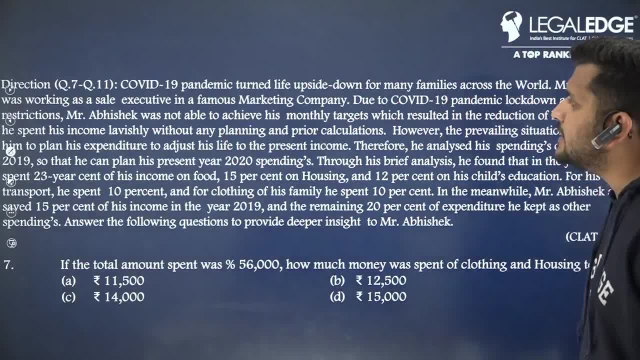 What does it say? COVID 19 pandemic turned life upside down down for many families across the world. mr abhishek was working as a cell executive in a famous marketing company by mr abhishek, a famous marketing company due to the covid 19 pandemic lockdown. 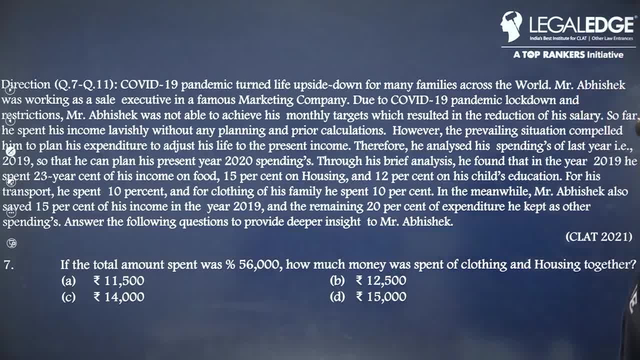 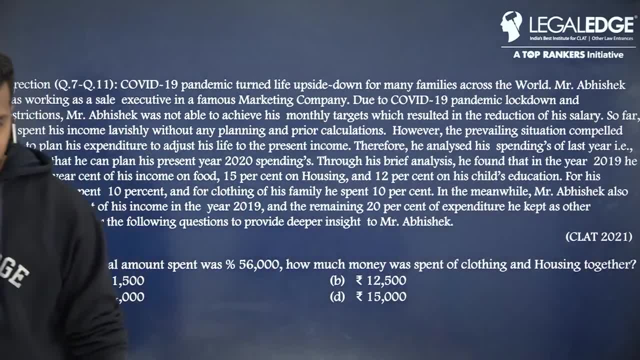 and the restrictions, mr abhishek was not able to achieve his monthly target, which resulted in the reduction of his salary. what happened when covid came? and due to covid, what happened in his life? he suffered. a lot of people suffered in his life. this is his sorrow and on that he asked a question. 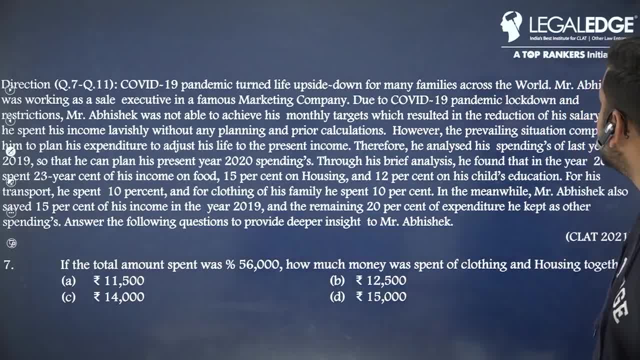 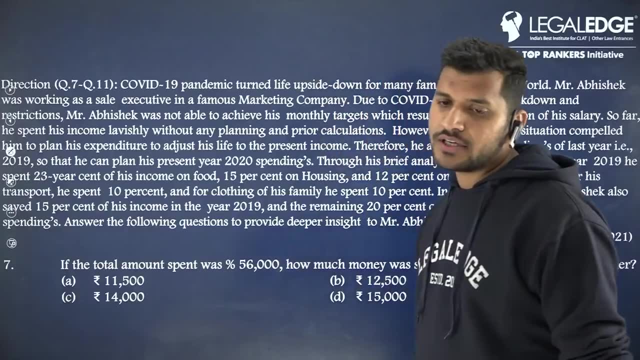 that mr abhishek, who could not achieve his target, could not achieve his target, due to which his salary was reduced somewhere because he was doing a job in a marketing company. he was working as a sales executive. so sales executive is the same: until your product will not be sold, you will not get money. according to how much it will be sold, you will get money. 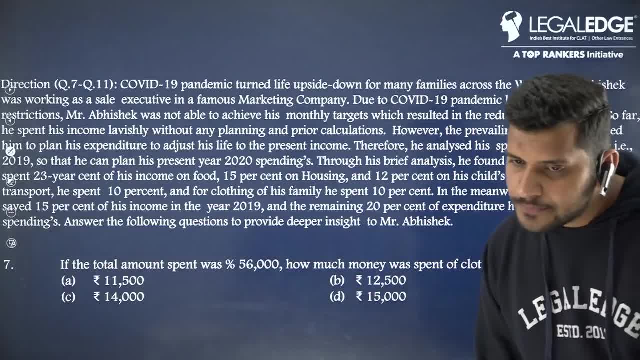 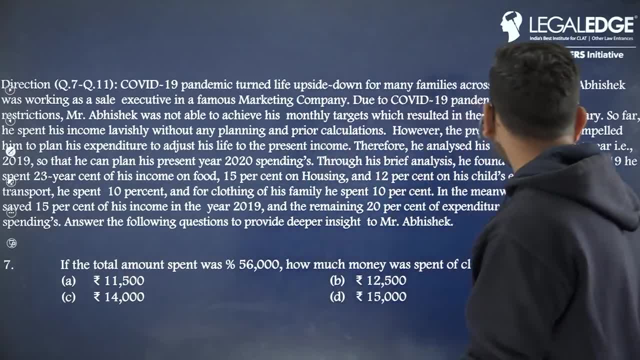 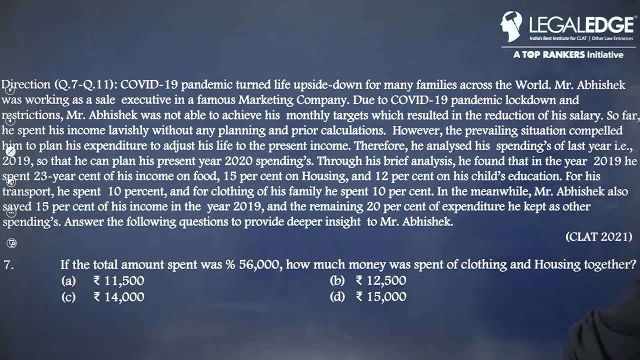 so for all its, for all its aarsagwal, lavitha lavithra. okay, you are enough. for all its aarsagwal, okay, or how was the align situation compelled him to plan his expenditure to adjust his life to the darling come. therefore, he analyzed his spending. 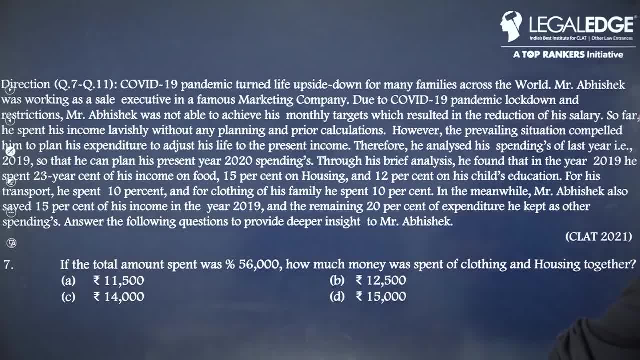 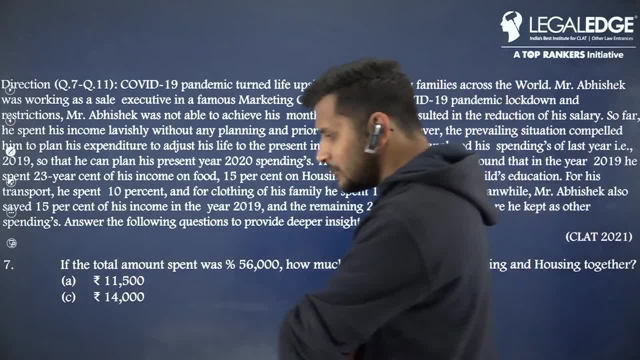 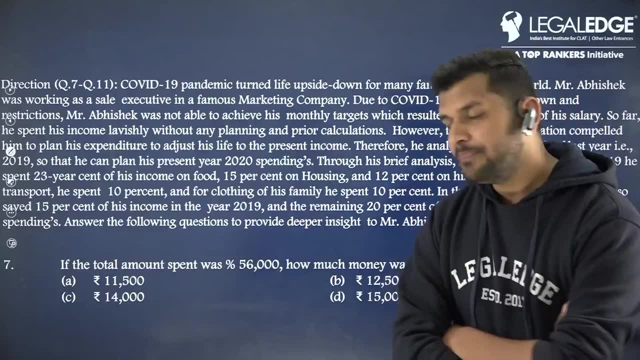 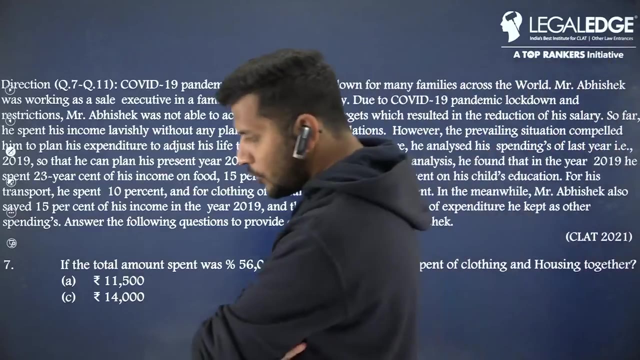 He analyzed his last year's spending in 2019 so that he can plan his present 2020.. So, whatever he spent in 2019, like he spent money on alcohol, he spent it for nothing. So to avoid that, he took out the data of the previous year and said that in 2020, I will spend everything. very well. 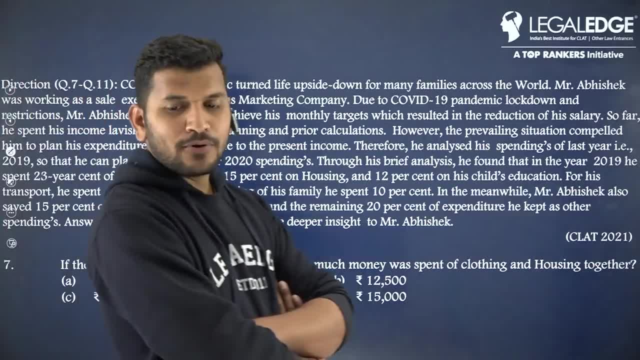 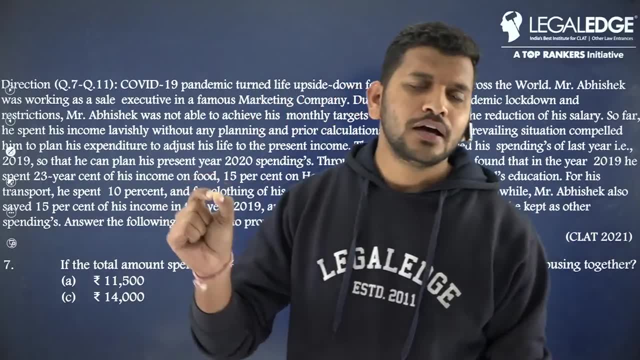 But what to do in 2020, the corona has come. Like you, people swear. when do you swear? When you swear on the 31st? On the 31st, say that I will do this from today, From 1st January 2022, I will study every day, or I will study every day. 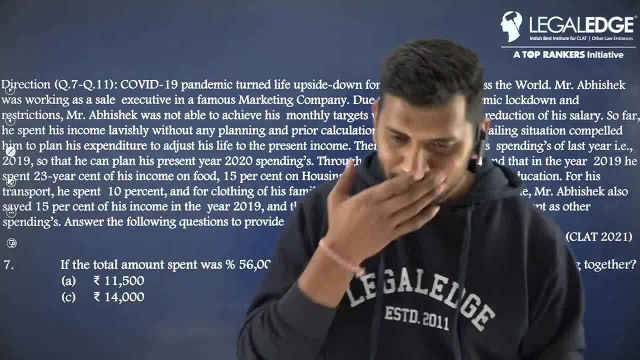 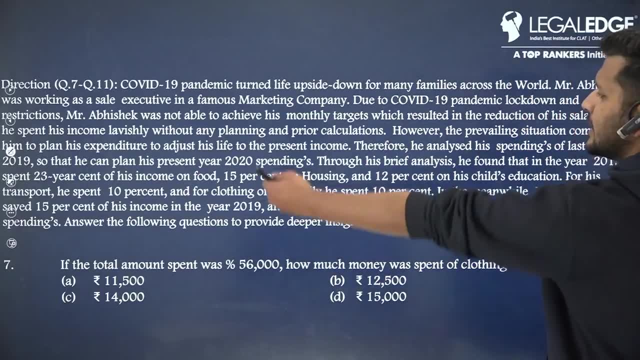 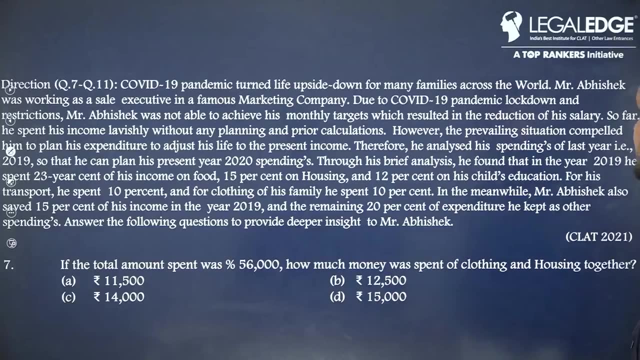 But you don't do that, You don't do that. Let's see what the answer is. Do you understand the point? So, therefore, what did he do in 2020?? So his brief analysis: he found that in the year 2019, he spent 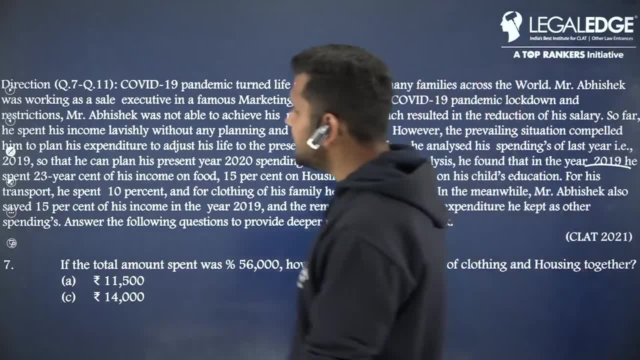 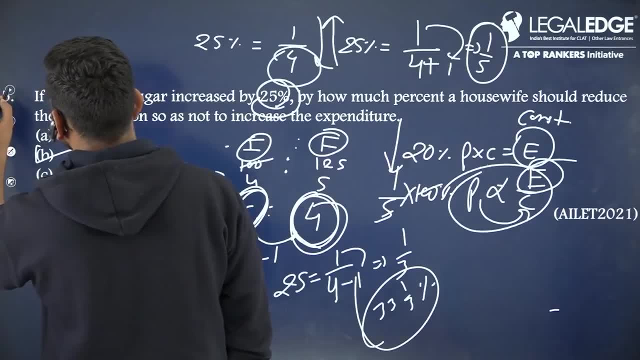 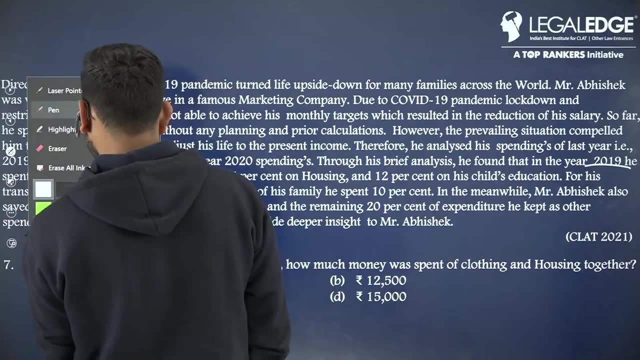 See in 2019, he spent 23%. Okay, should I take the green color on this pen? I will need a little here. I will need a different color of pen. guys. You will say, sir, what color did you take? 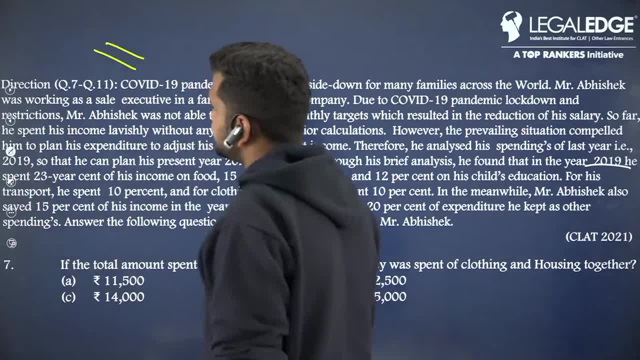 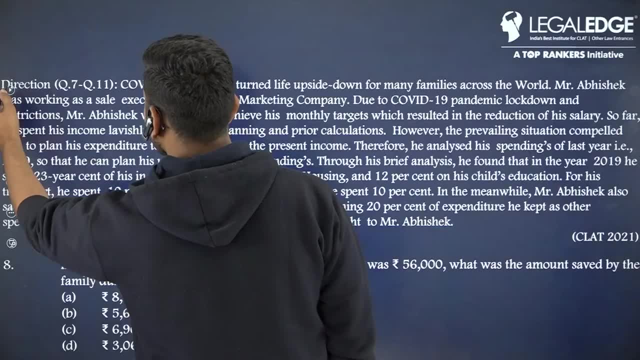 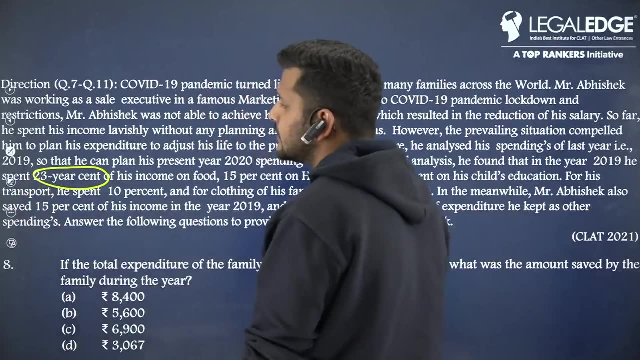 Will yellow color work? Will yellow work? Okay, He spent 23 years. He didn't write 23 years. One second, what happened? Listen, this is 23%, Right, 23%- of his income on food. Guys, how much did he spend on food? 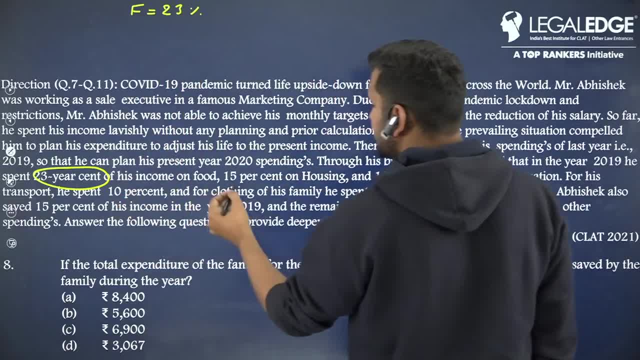 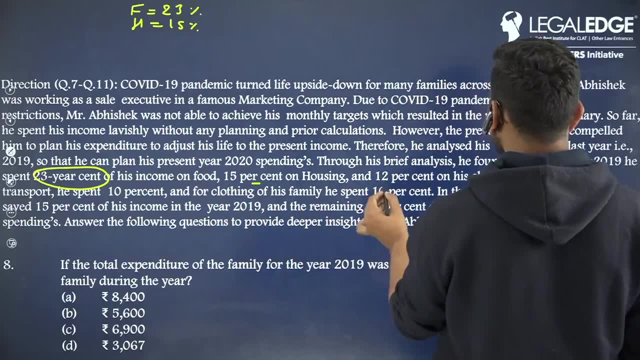 I will write it here: 23% Right, 23% on food, 15% on housing. So how much did he spend on housing? 15%, Let's keep writing- And 12% on his child education. On child education. 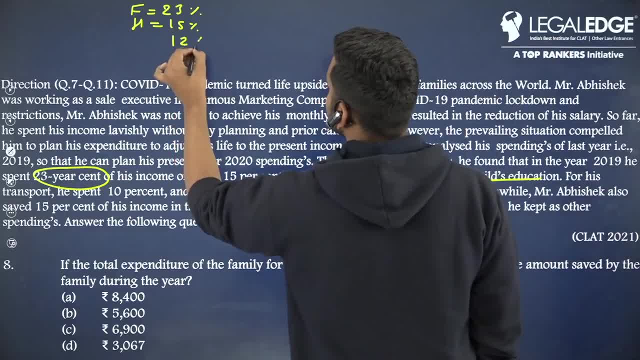 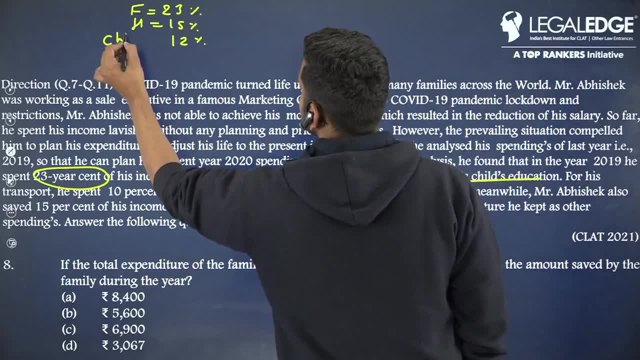 How much did he spend on child education? 12%. He spent 12% on his income. He took out the data of 2019.. That he could do, planning for 2020.. So how much on child education, guys? 12% on child education. 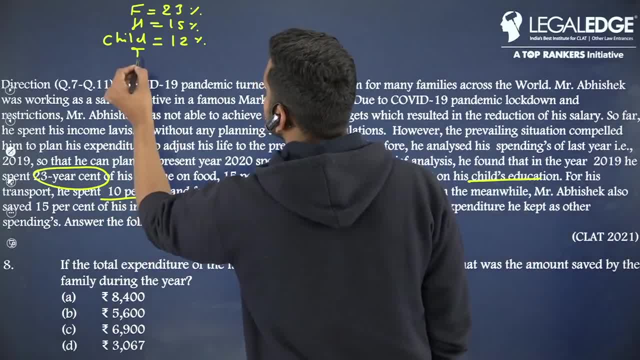 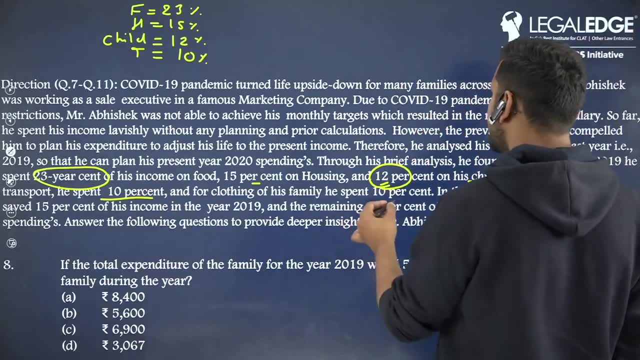 And for his transport: 10% on transport, 10% on his transport. Keep writing. Whatever you will say, I will keep writing. And for clothing family: His family spent 10%. What did he do for clothing 10%. 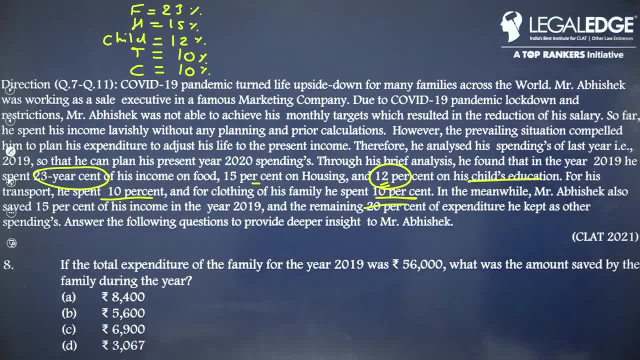 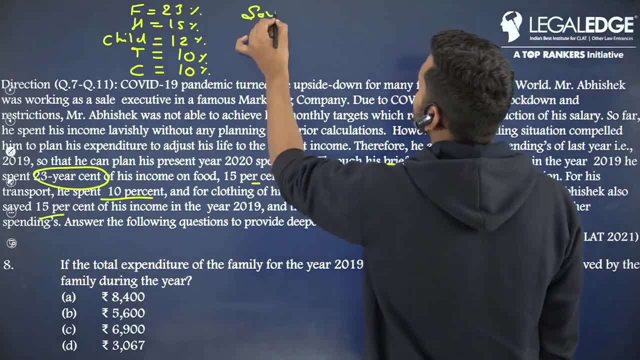 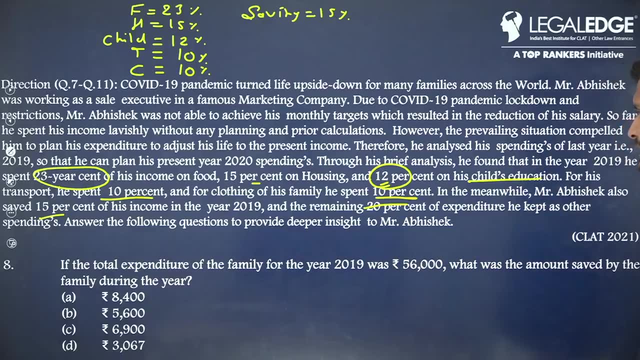 Right, Okay. Meanwhile, Mr Abhishek also saved 15% income And he also saved 15%. So let's write the saving as well, guys. 15%, Okay, And the remaining 20% expenditure he kept as other spending. 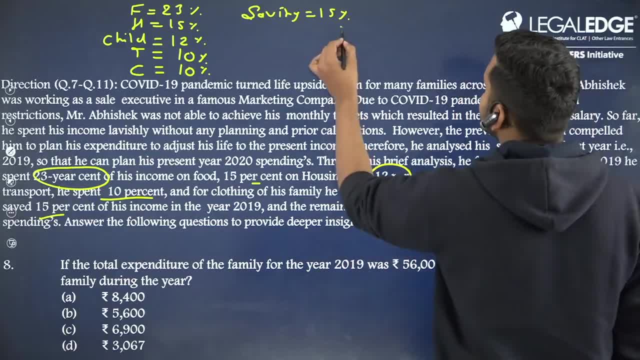 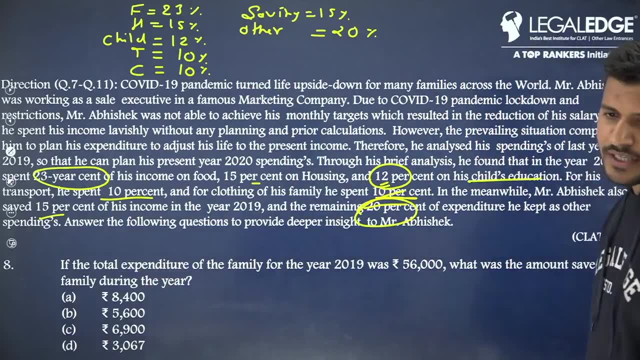 20% on other spending. He also spent 20%, But on what On other? This is how it is, Is it clear? The question is very easy. All the answers must have come Scientists. everything will be fine Okay. 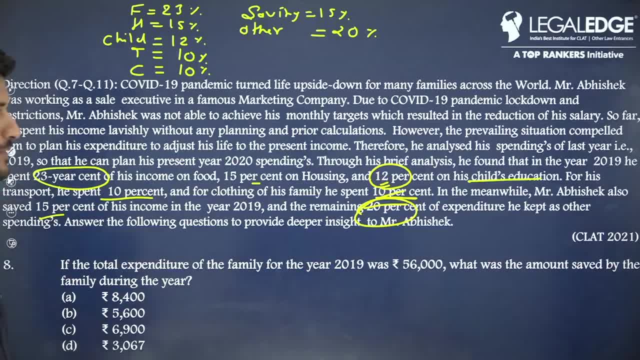 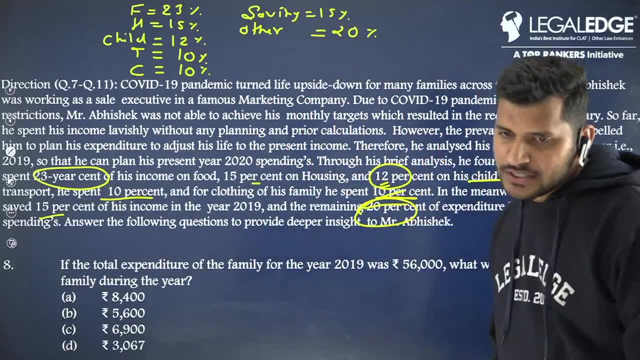 No problem, This has come in 2021.. This is called Casualty DI Paragraph based Right FYI. What do you write? What happened to you? I don't understand anything. M W U H S F. 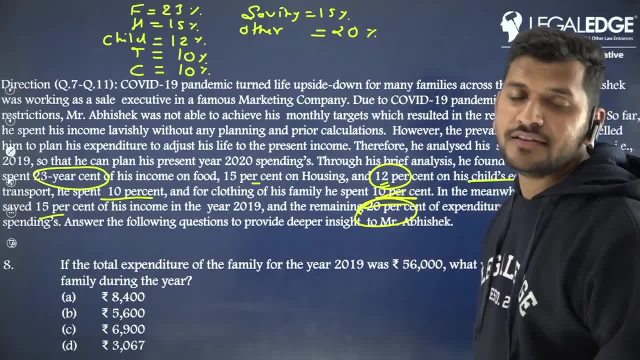 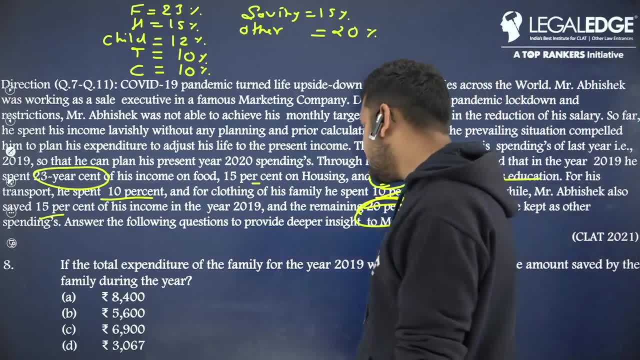 I don't know what. Write the name correctly So that we can read. We don't know Chinese language, So how can we read? So guys try to understand here. Question says: If the total expenditure of the family for the year 2019.. 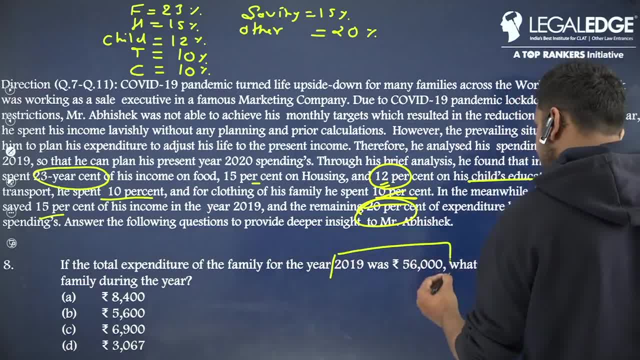 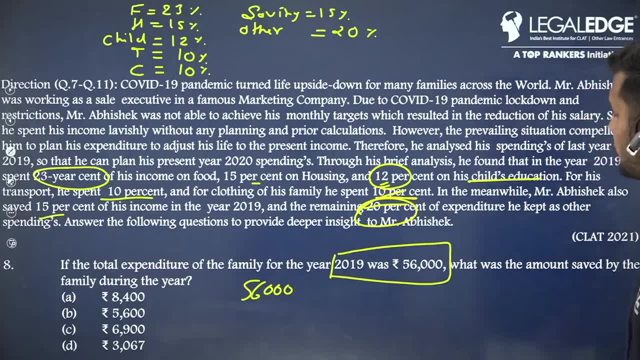 The question says: What was the total expenditure for 2019?? It was 56,000.. Means the total expenditure which he added in 2019, it was 56,000.. Then he asked What was the amount saved by family during that year? 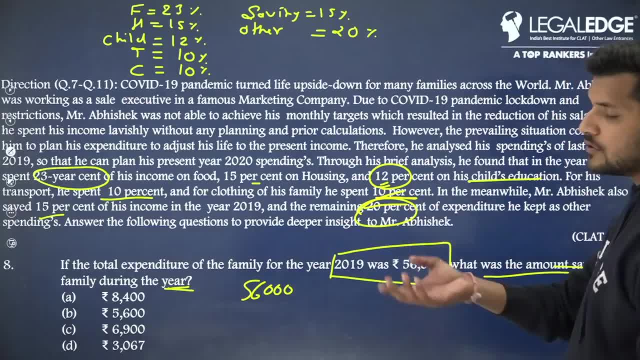 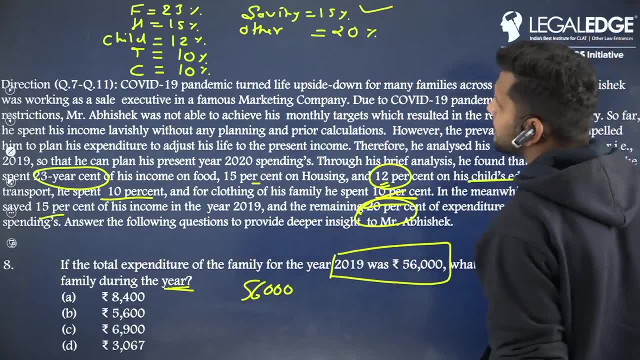 How much saving was there in that year? In total, he spent 56,000 in 2019.. And how much was the saving? Saving is only written here: 15%. How much is the saving? 15%? So just take out 15% of the saving. 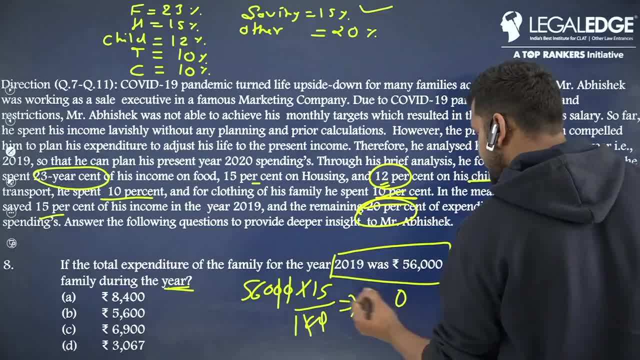 So 2 zeros will go from 2 zeros. This will be zero. Okay, 15,, 6,, 0,, 90.. 9 will be left. 75, 70.. 75,, 84 will be left. 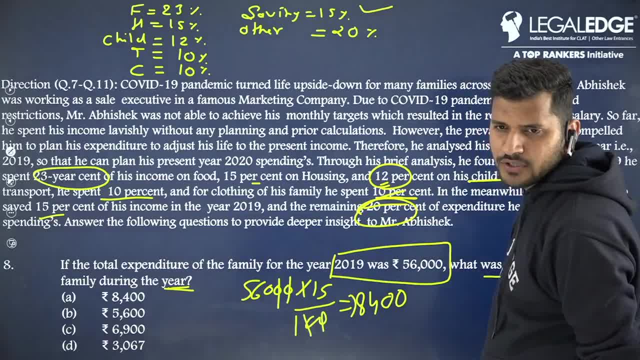 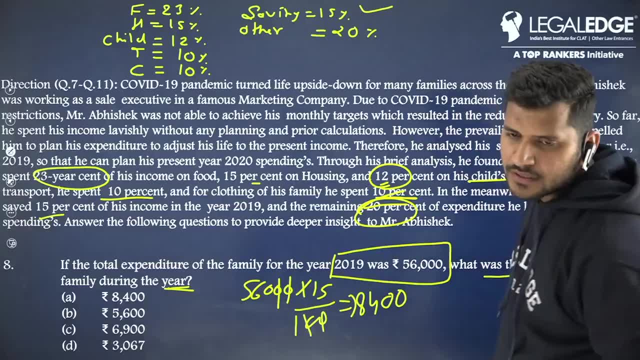 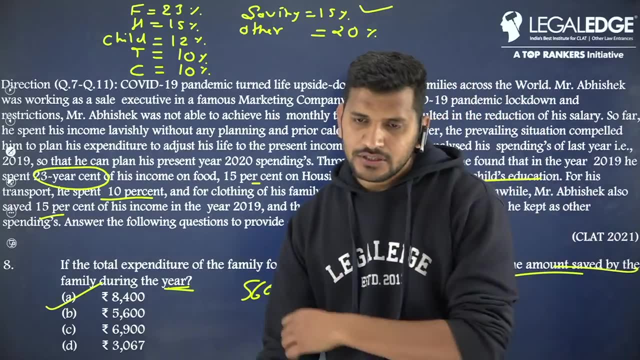 This is the answer of the whole world: 8,400.. Right, So the answer is coming from here. He made it like this and gave the answer, And the answer is not 505.. He said the remaining. Pay attention here. 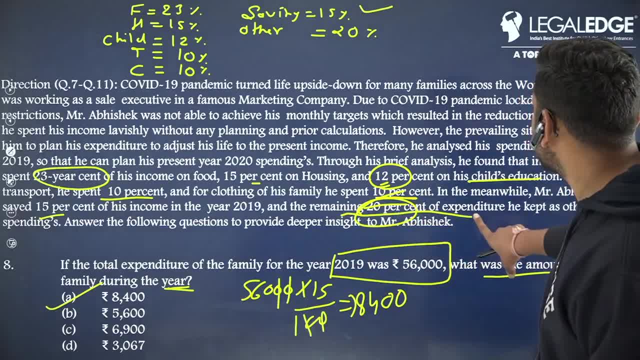 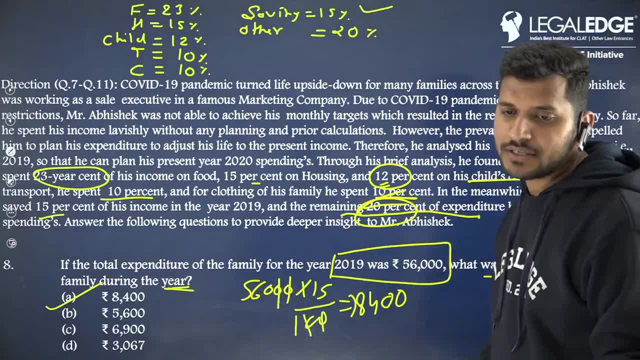 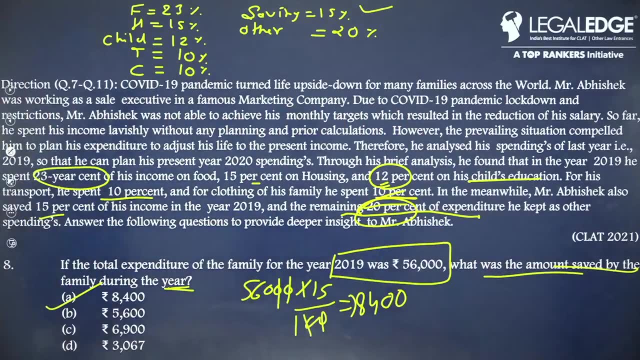 What he said And remaining 20%, Right, So the remaining 20% after taking out all the remaining. That's why you can't say like this: Yes, Okay, Okay, Okay. Let's go to the next question, guys. 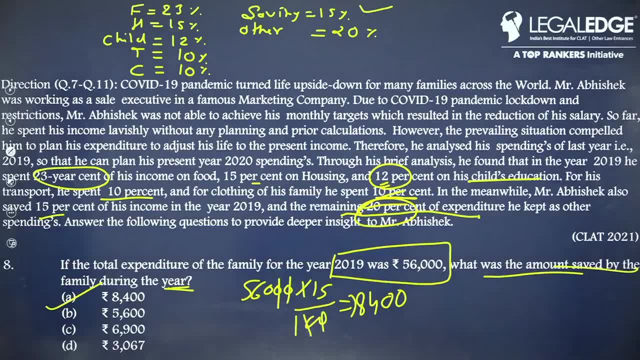 Let's go to the next question. Has one question been skipped? No, Where See, this is 6 and this is 7. And 8.. Okay, one question has been skipped, No problem, No problem, One question has been skipped. 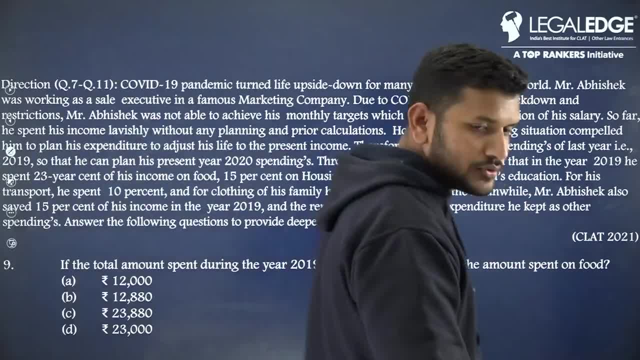 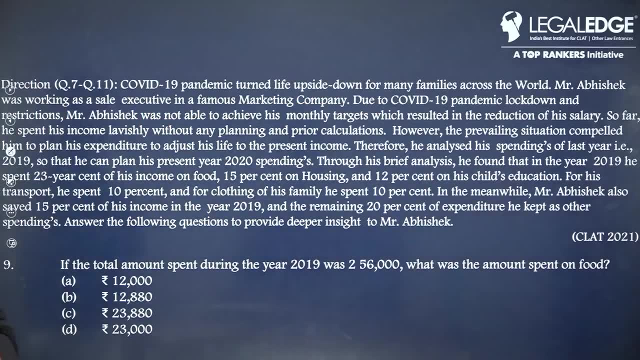 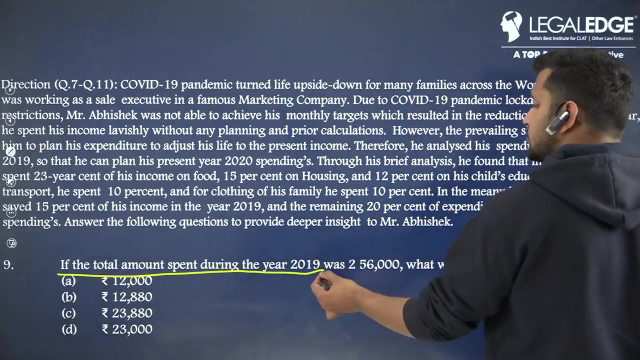 Now you can solve it. This has been skipped. Solve this question Right now. Now, Solve this question straight away. This has been skipped. Can you solve it yourself? Okay, If the total amount spent during the 2019 was 2,56,000,, what was the amount spent on? 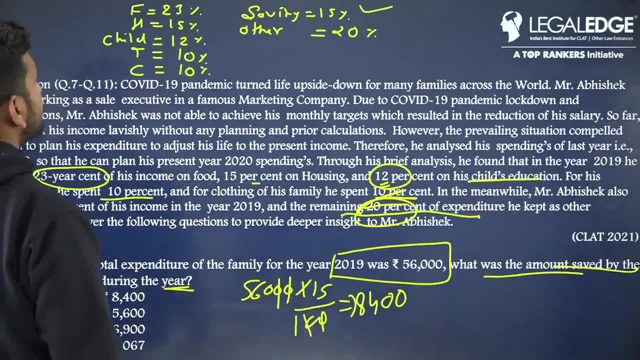 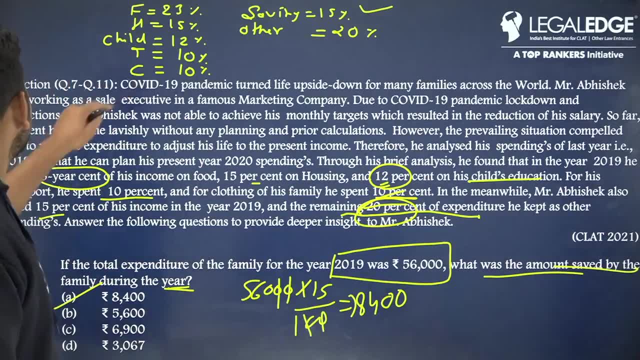 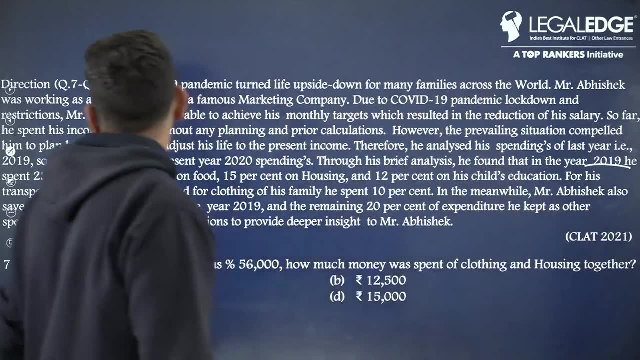 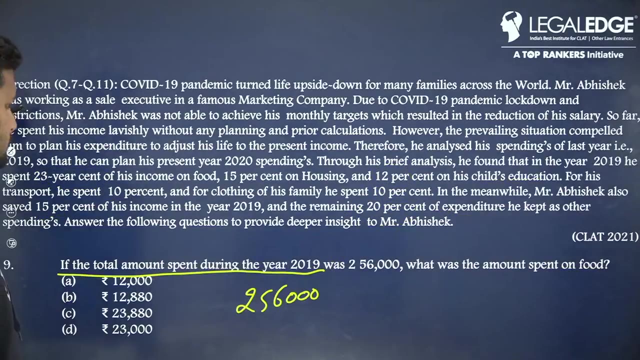 food. How much is the total amount spent on food? It is 23%, right. How much is the total amount spent on food? It is 23%, right. So just do it One minute. where did it go? We will take that question tomorrow. that is also easy. 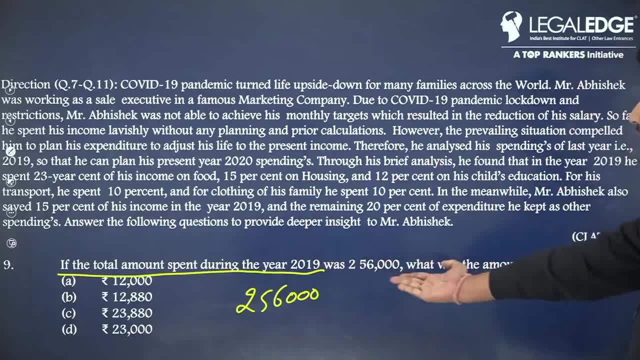 How much is the total amount spent on food? It is 23%, right. How much is the total amount spent on food? It is 23%, right. How much is the total amount spent on food? It is 23%, right. 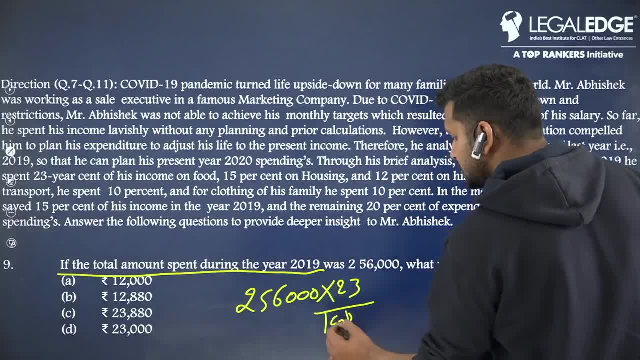 So what is the answer? Let's take out 23%. 23 upon 100 will be 0 to 0,. 0 to 0 will be cancelled. We will multiply 23 by 0.. So if we multiply 23 six times, 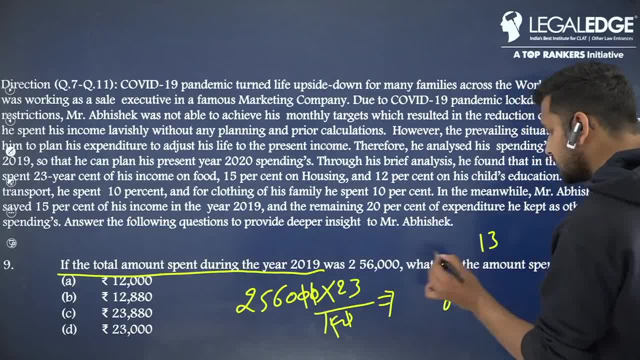 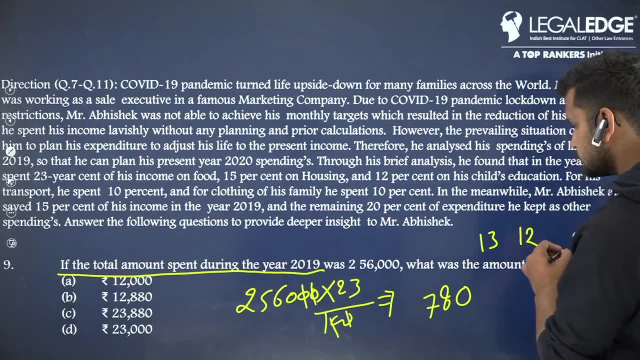 then it will be 138.. 8 will come, 13 will be carry forward, 123 will be 115.. 125,, 120,, 7.. 7 will come, 12 will be left. No, it will be 128, right. 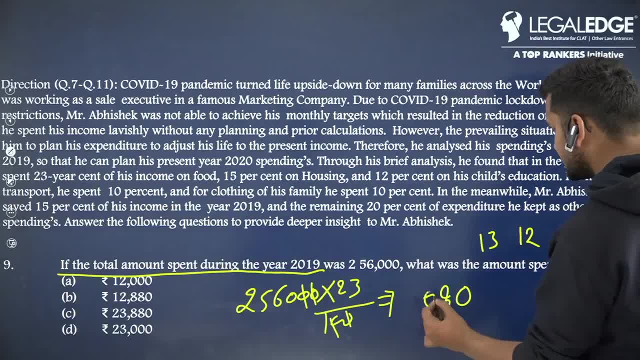 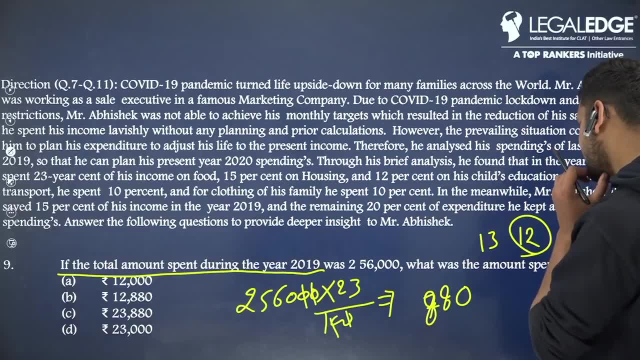 No, it will be 128,. right, It will be 128,. 13 will come. So 12 will be left right, 23 to the 40,, 6,, 46, or 12,, 48,, 58,, 5.. 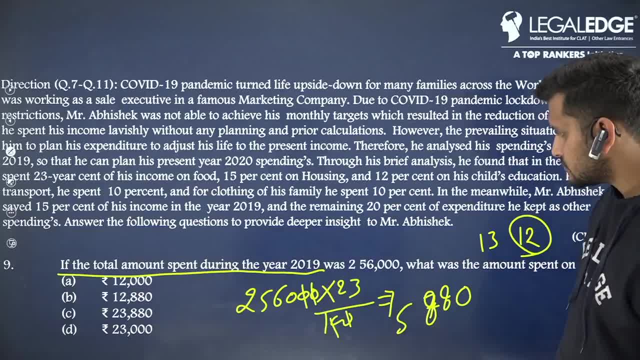 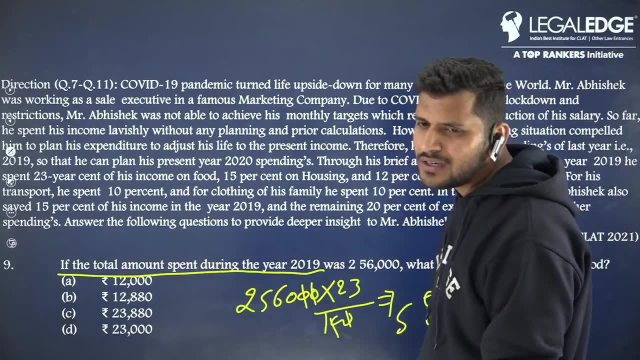 Did something go wrong. What was the amount spent on food? It is 23%, right, Sorry? 9. Question 9.. Yes, okay, we will do it back and forth. Let's see its multiplier once. did something go wrong? 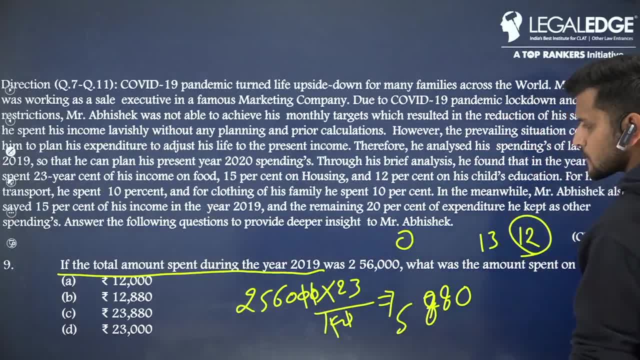 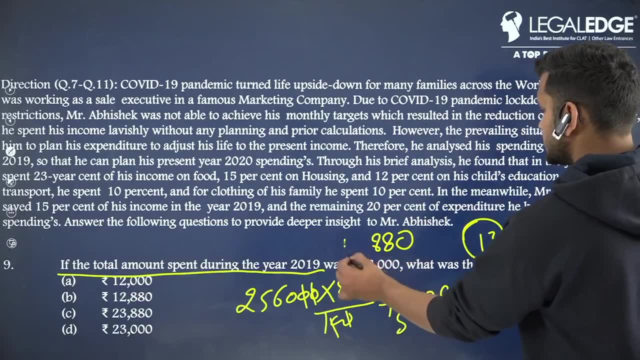 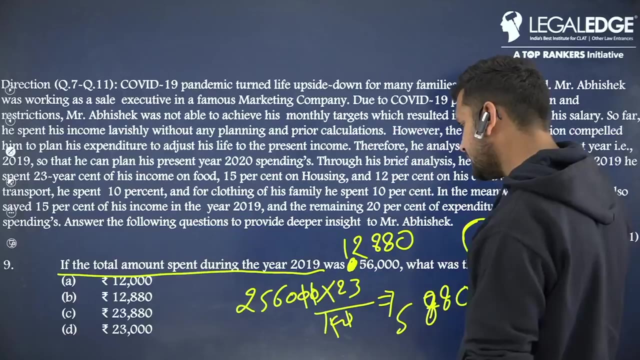 0 will be 0,. okay, 13 will be left. okay, Listen, it is written 2, it is not 2.. If you cut 2, it will be 56,000.. Sir, total, yes, it will be 56,000.. 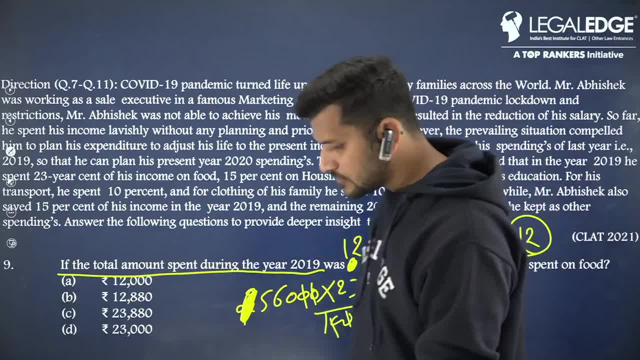 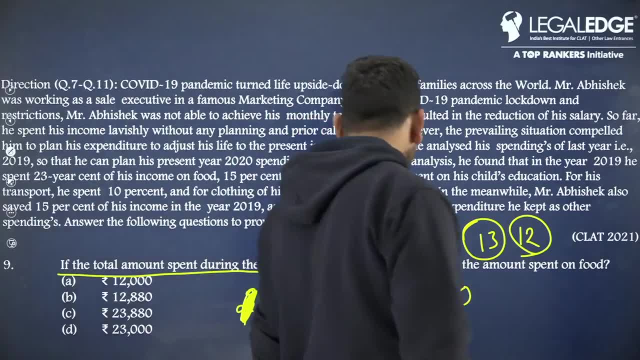 2 will not be left in this question. This is wrong. It will be 56,000,. 2 is wrong, Sir, data is wrong. Yes, yes, I told you It was 56,000 in 2019.. 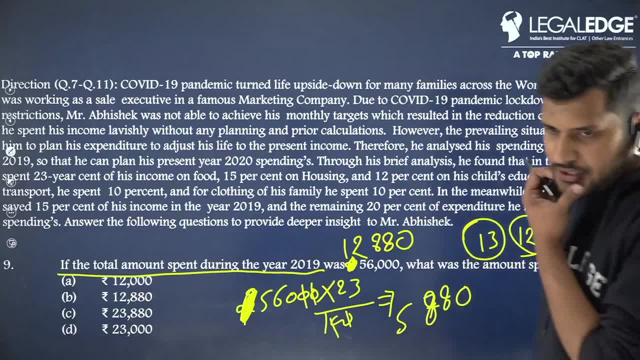 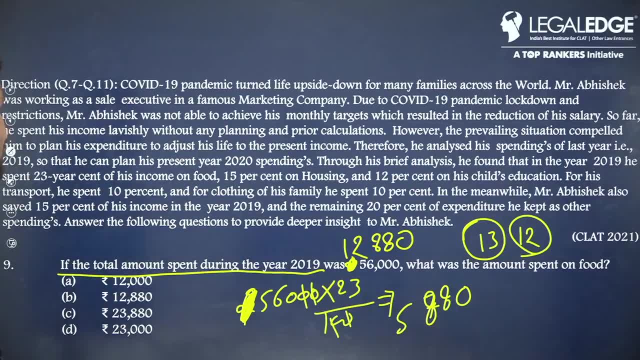 Remove this 2.. 2 was not 56,000,, it was 56,000.. Correct it, it is 56,000.. Right, So option number 12,000.. How much 880 is coming? B option is correct. 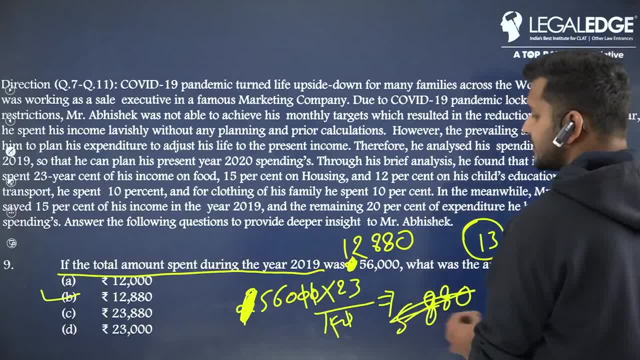 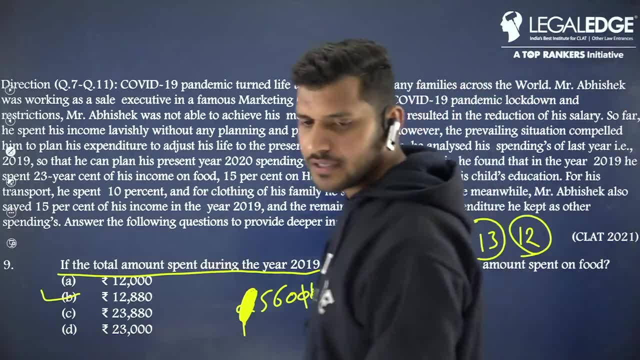 No, no, 588 will not come. This is wrong, Because I have taken it out according to this: 2,56,000.. Now it will come out according to 56,000.. It will come out according to 56,000.. 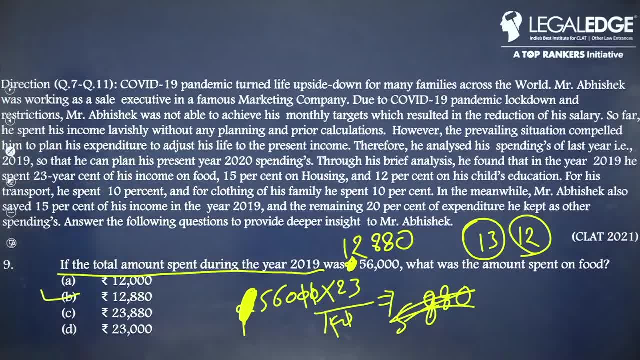 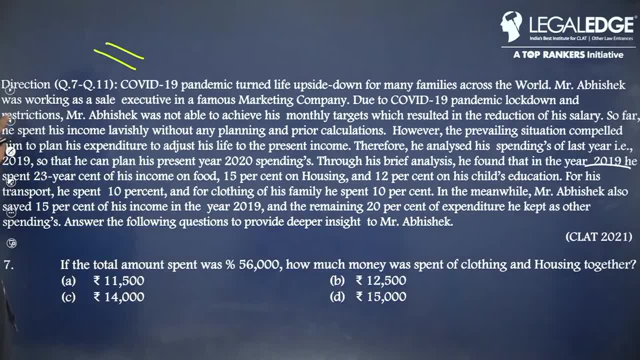 Sir, it is wrong. Yes, yes, yes, B answer came. Ok, we left one question behind This. This was 7.. Was this left? Do this If the total amount spent was 56,000.. How much money was spent? 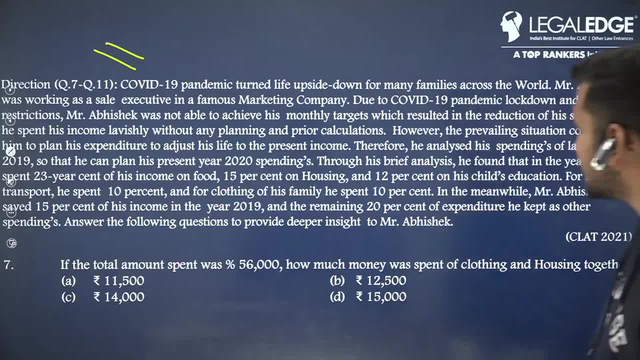 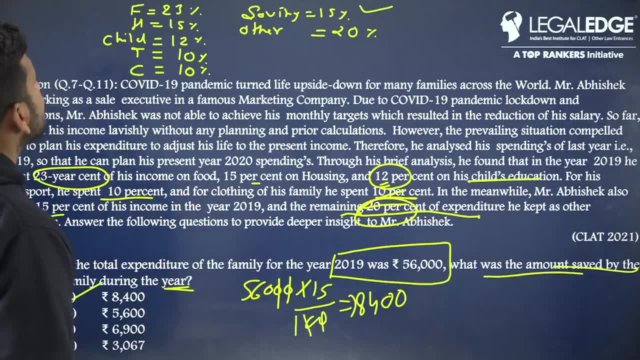 clothing and housing together, Clothing and housing together. Let's see how much. It was 56,000.. Guys, we have to check on clothing. How much is there on housing and clothing? 15% on housing And 10% on clothing. 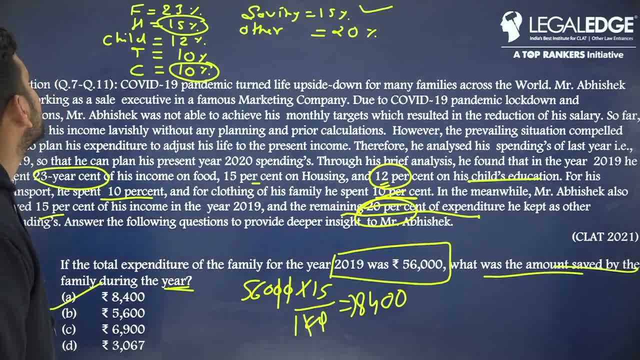 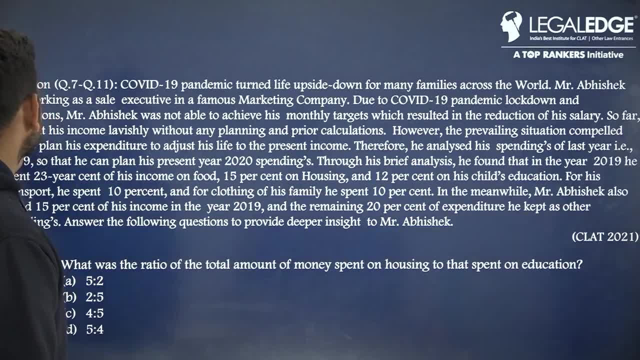 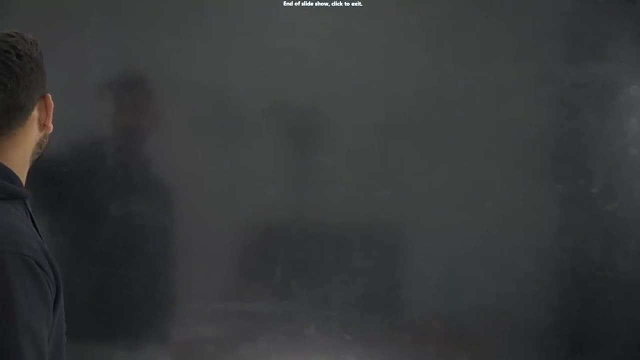 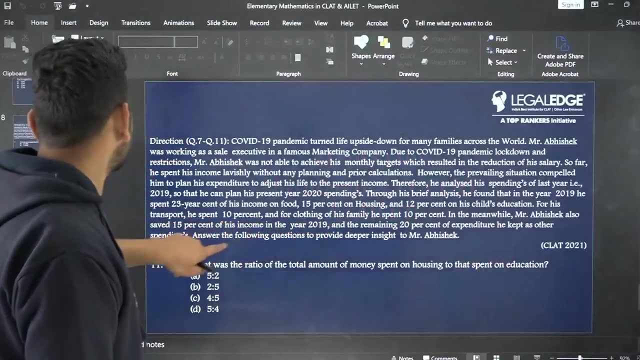 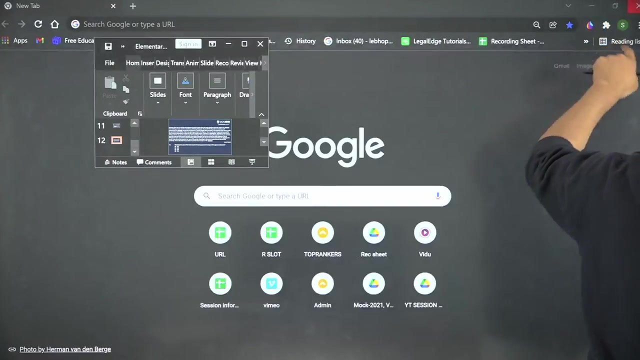 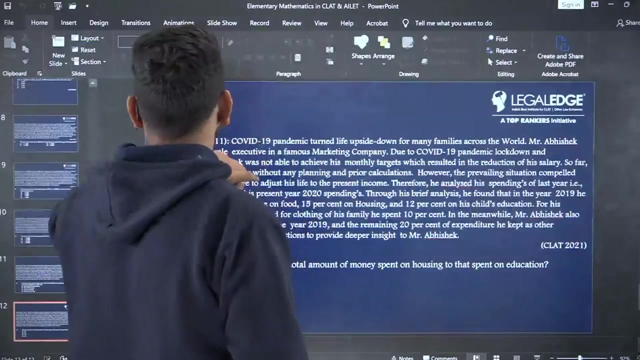 Right, 15% on housing And 10% on clothing. So Housing and clothing, What was the ratio of total amount 11. What is happening? I don't know. What is happening? I don't know, Come on tell it. 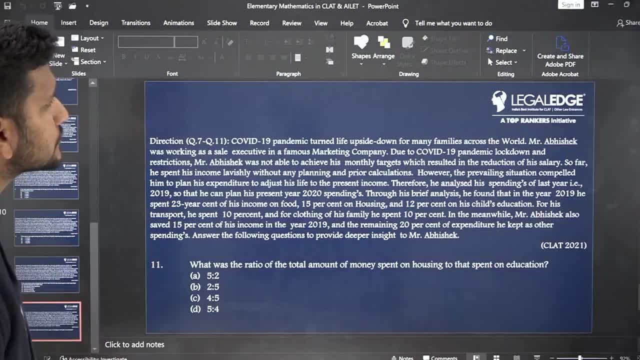 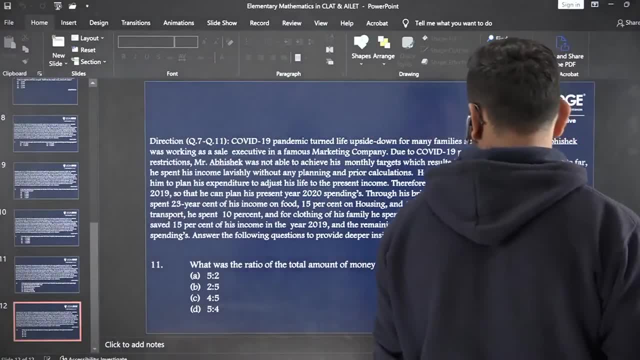 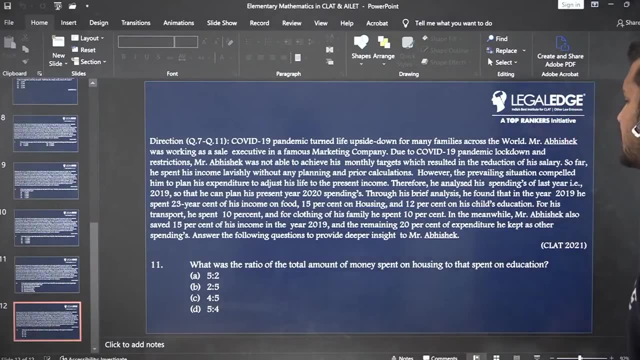 Tell it. Tell it from this Housing and clothing Housing to that. What is he saying? Spent on housing to that of Spent on education. Tell anything from 11.. Tell the answer from 11.. Because what data did we do here? 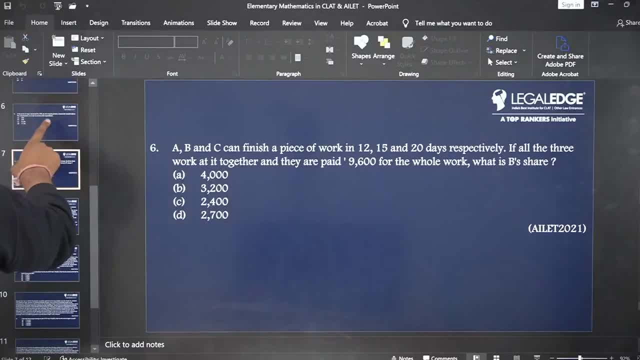 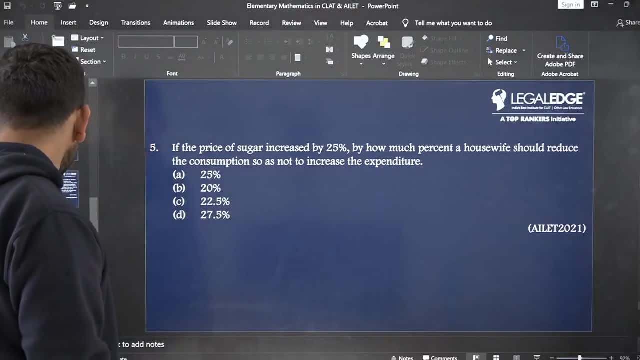 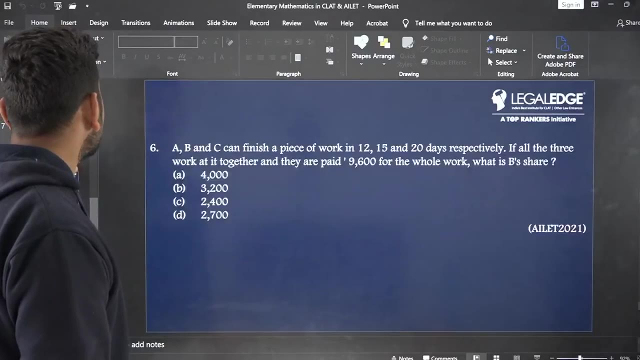 We have written everything on this question, But here everything is rough. The PPT that we made. Hold it for a second. You will do it right. Give the question. Come on, I will tell you every question. 6 is done. Was it 7th? 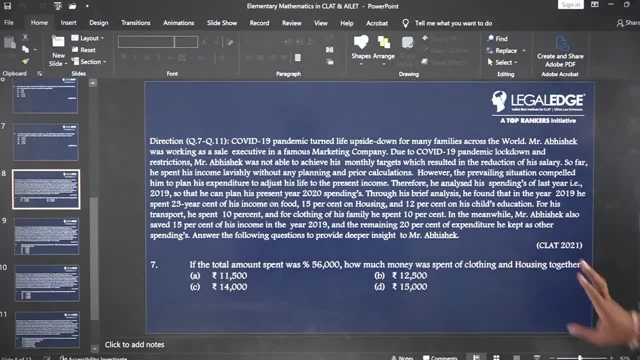 See how much on clothing and housing. See from here How much on clothing and housing. 7th answer: How much on clothing and housing. See here How much on clothing and housing. 25% was happening. Clothing and housing was. 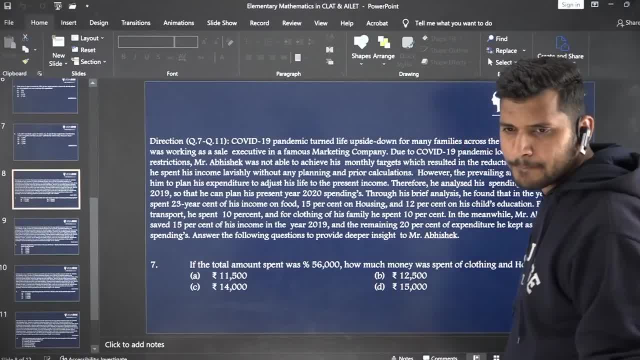 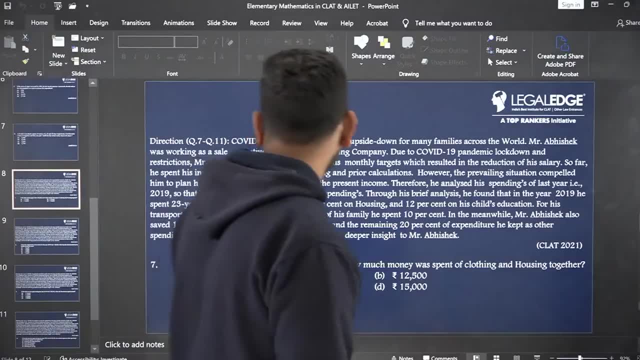 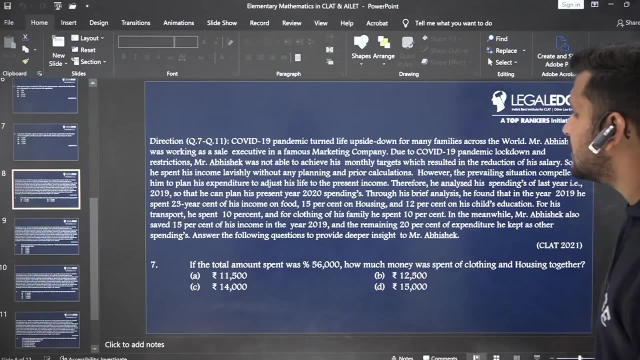 25% of 56,000.. Okay, Lawyer, Yes, yes, Absolutely. Tell me how much on clothing and housing is happening. Tell me quickly. So let's see Where is it written: on clothing and housing: 15% on housing. 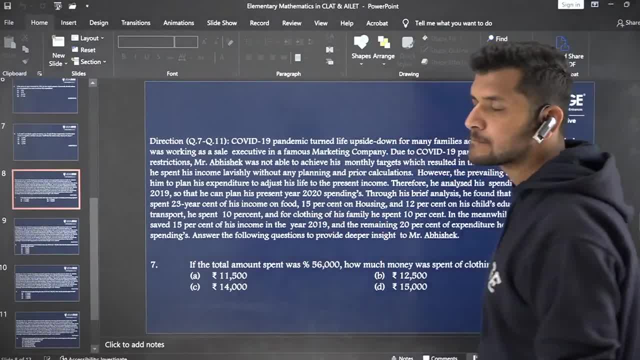 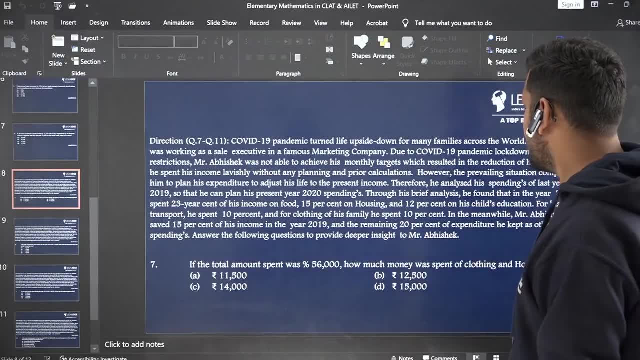 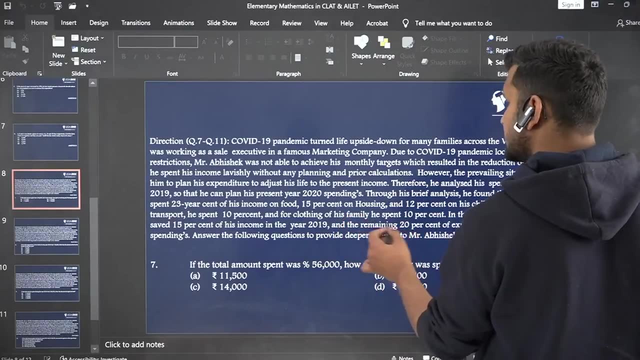 This is it. How is it not coming on total 15%? I will tell you directly: 15% on housing And how much on clothing Spent, Spent at 10%. So you have to subtract 25% from 56000.. 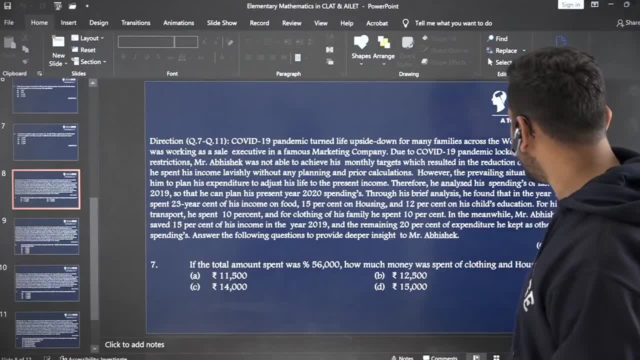 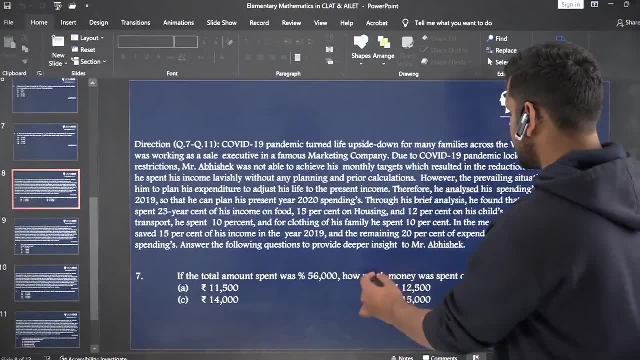 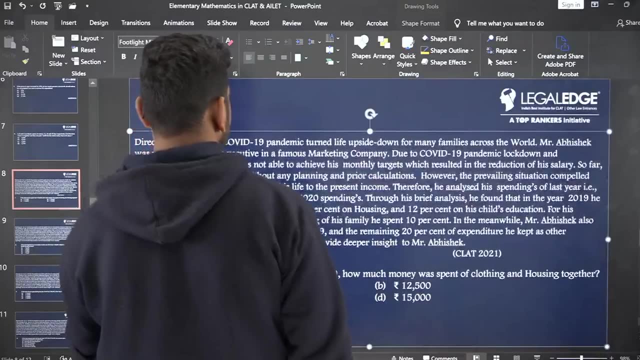 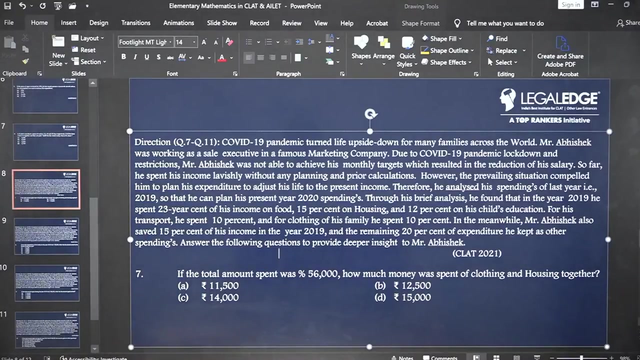 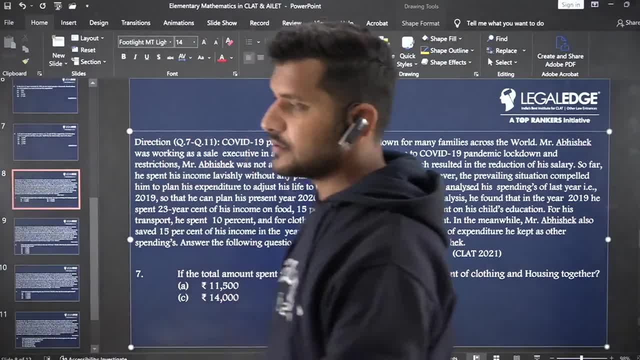 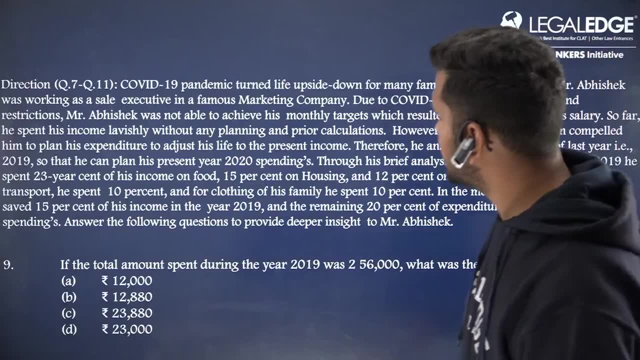 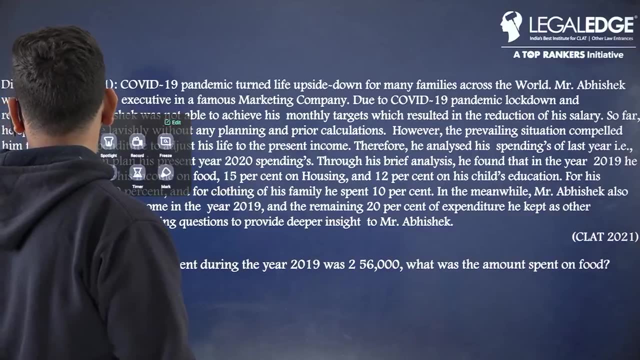 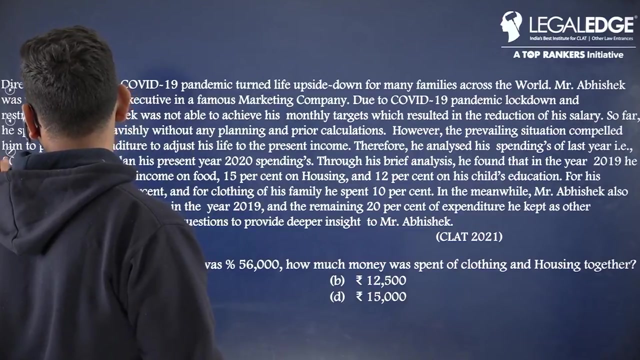 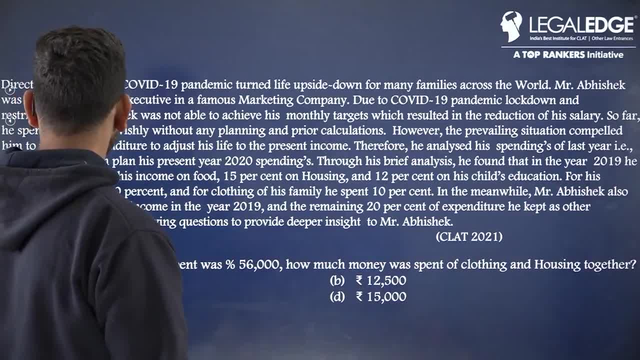 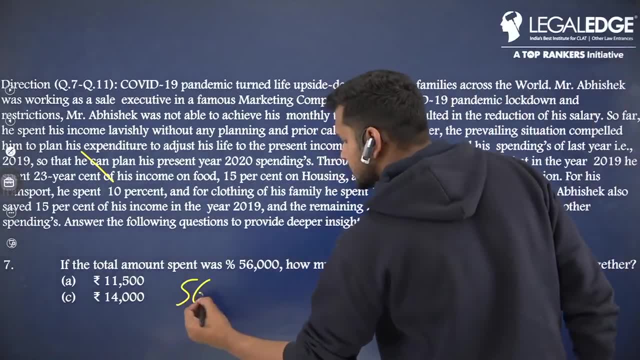 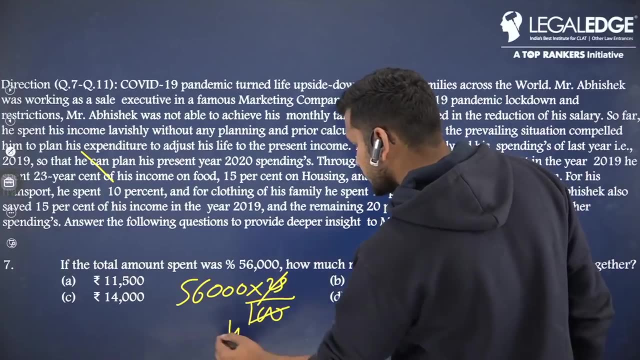 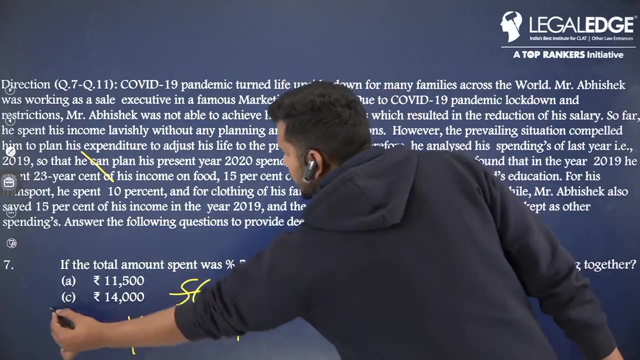 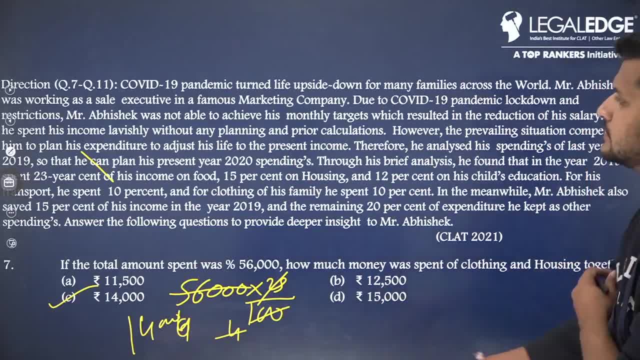 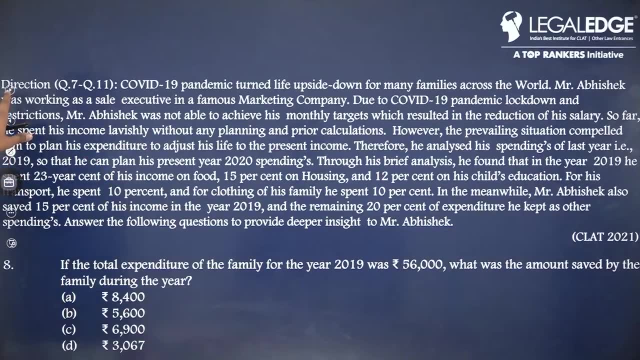 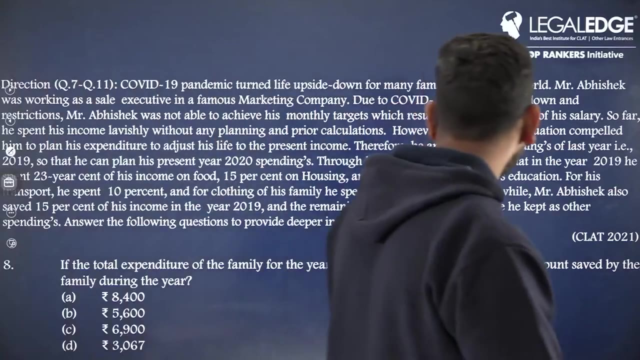 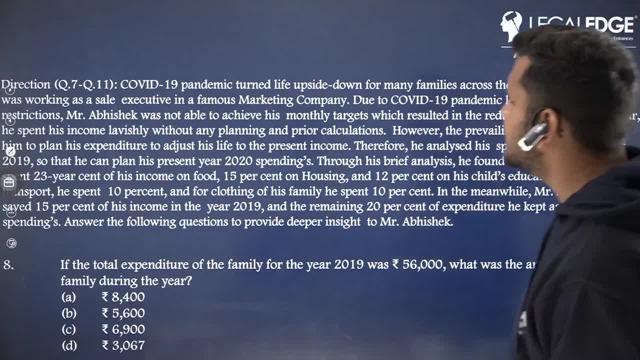 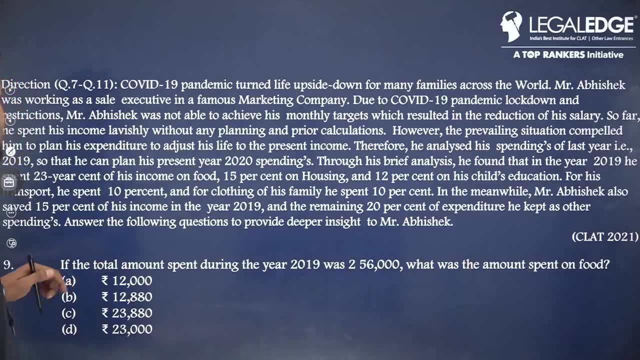 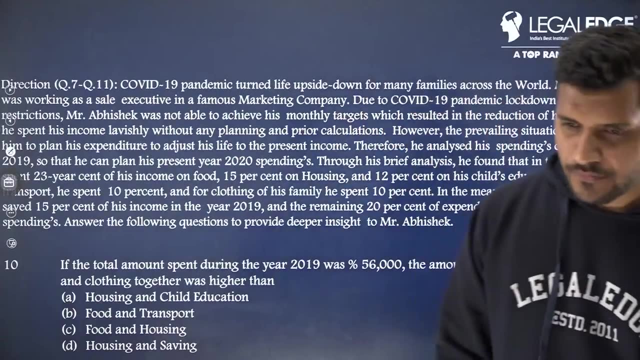 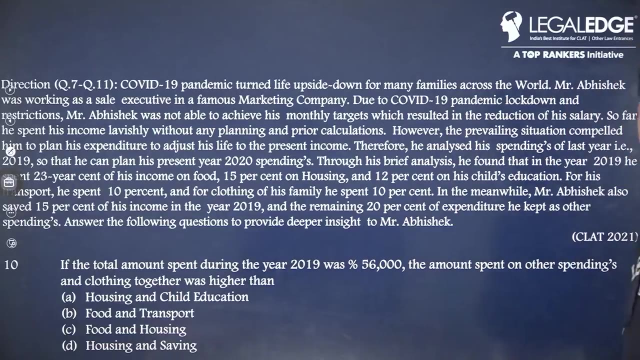 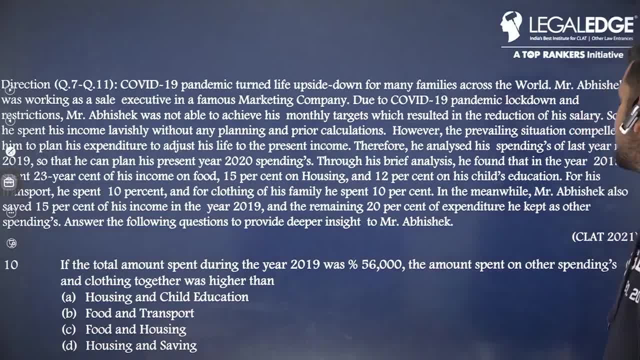 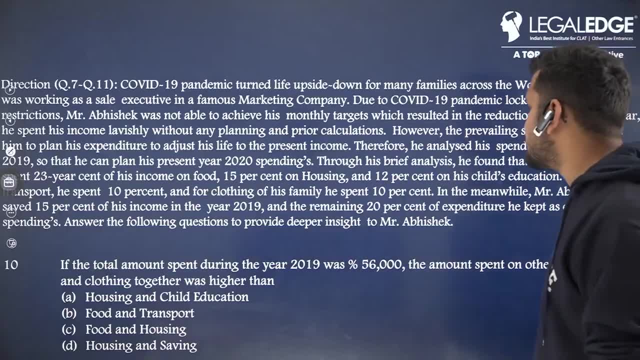 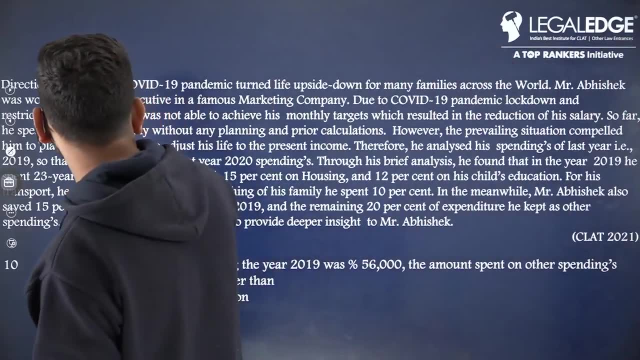 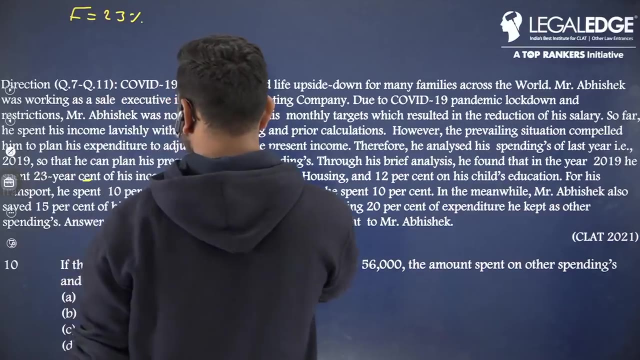 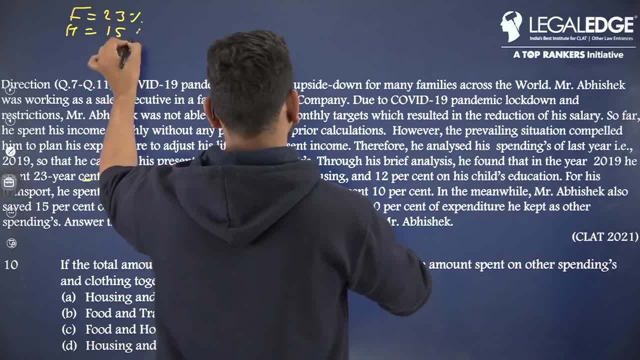 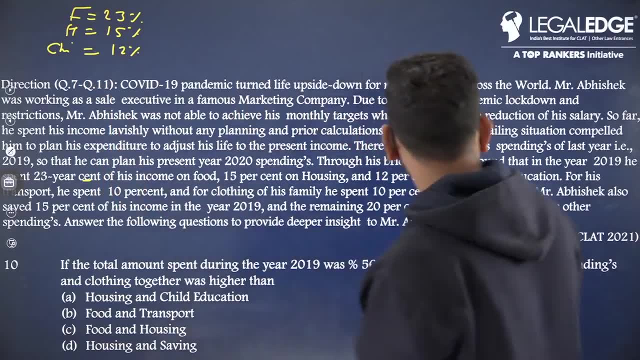 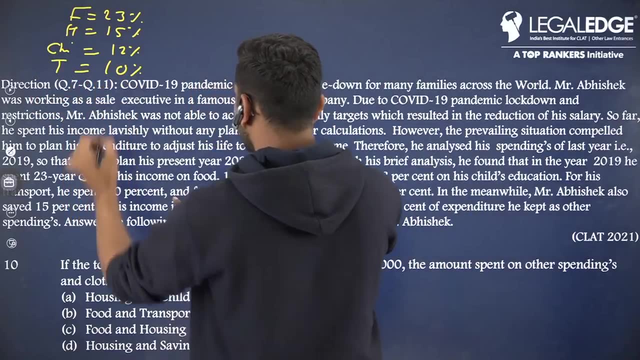 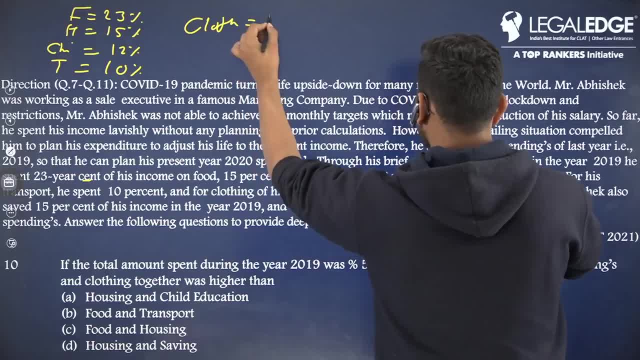 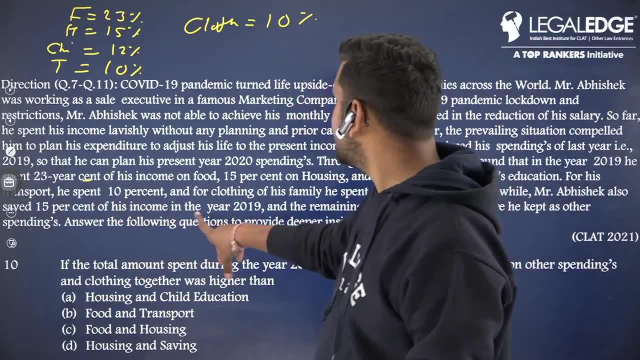 he spent clothing ke liye. dekh lete hain clothing ke liye. kitna tha 10 percent tha clothing of his 10 percent in meanwhile, mr abhishek also served 15 percent of his income in the year, saving pe 15 percent hai uski. ye sab data tha and the remaining 20 percent other per. 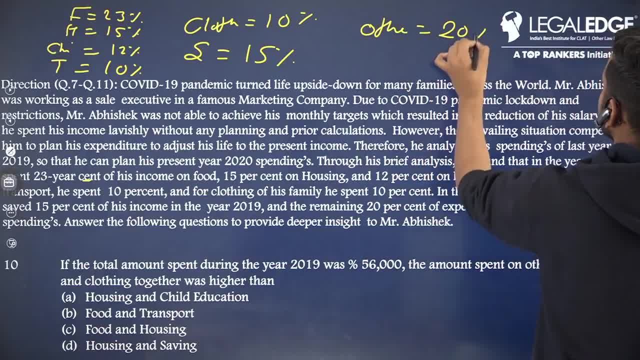 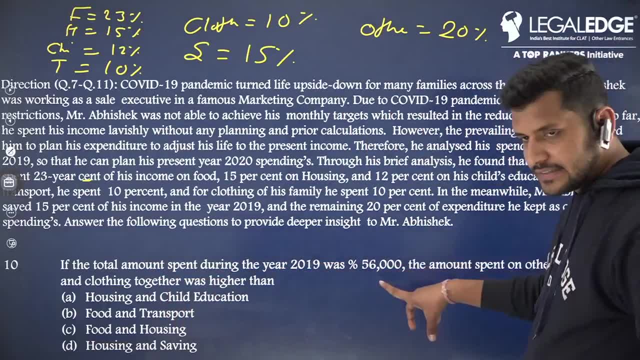 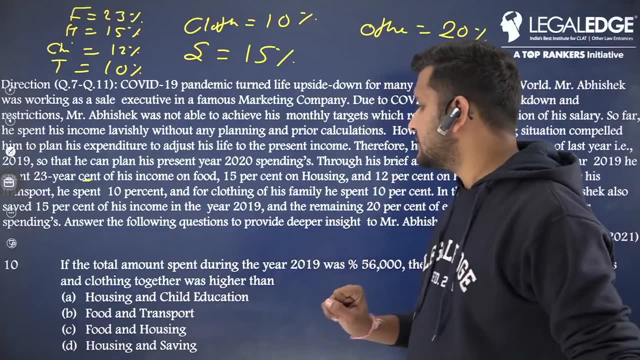 tha other kitna tha right 20 percent tha to dekho is question ko solve karne ke liye. kya karna padega if the total amount spent during the year 2019 was this: ye to tha the amount spent on on other spendings and clothed together was higher than higher than kisme other other. 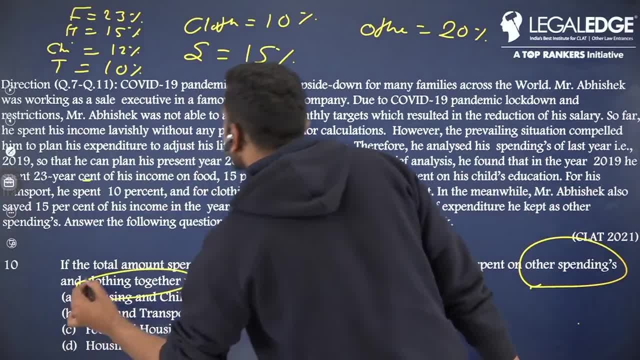 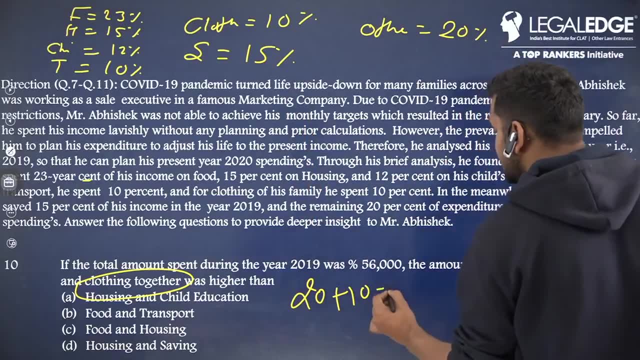 ki baat kar raha hai other spending per or clothing together, other or clothed together other per 20 hai right, 20 percent, plus clothing per kitna hai 10 percent, marlo 30 percent. hora direct aap percent. se hi solve kar sakto iska data mat nikalna jabardisti ka time. 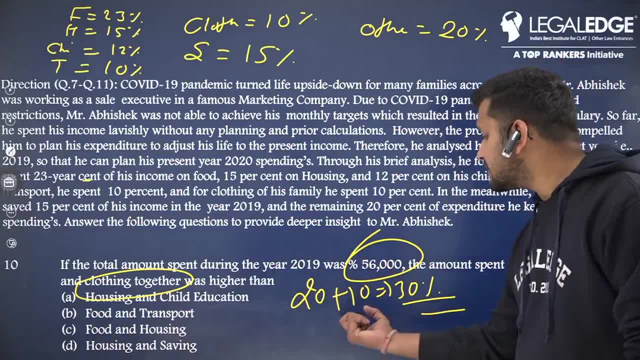 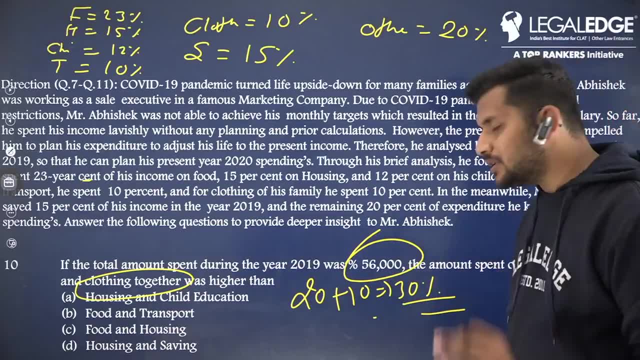 miss karoge kyunki aap 56 ka 20 percent nikalogu, 56 ka 10 nikalogu, 56 ka 30 nikalogu. all are same thing. koi jaroobat nahi aapko nikalne. ki right, koi jaroobat nahi aapko nikalne. 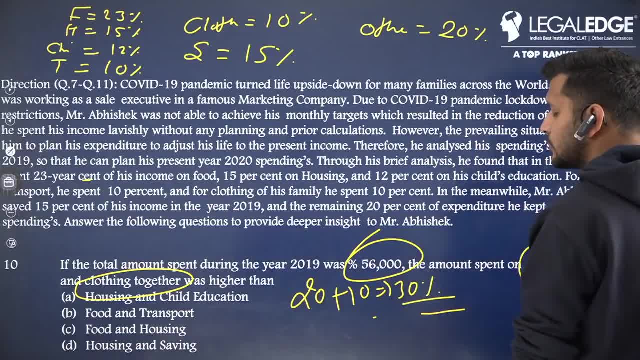 ki guys, toh main yaha par seedi baat aapko ye bolo ki ye toh 30 percent ho gaya. ab bo bol raha hai ki in jo hai amount on other spending ke liye, ke liye ki aapko nikalne ki. 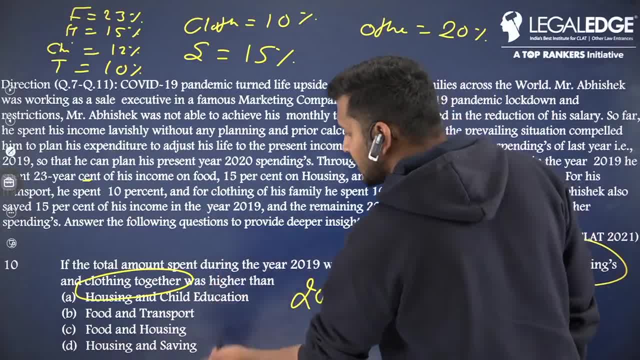 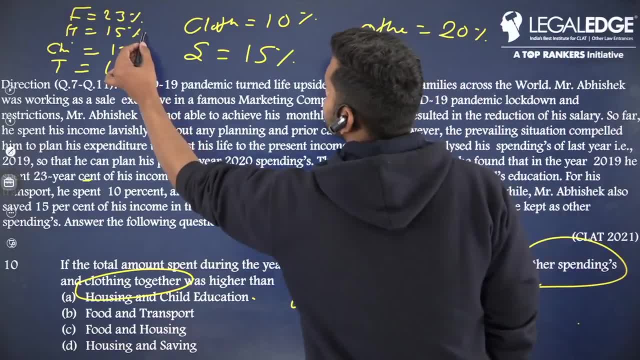 ke liye, ke liye ki ye toh 30 percent ho gaya. ab bo bol raha hai ki in jo hai amount on the other, spending per or clothing was higher than kis. se higher hai housing and child education se higher hai kya housing and child education ka. dekhte hai, housing ka 15 hai, right, 15 hai. 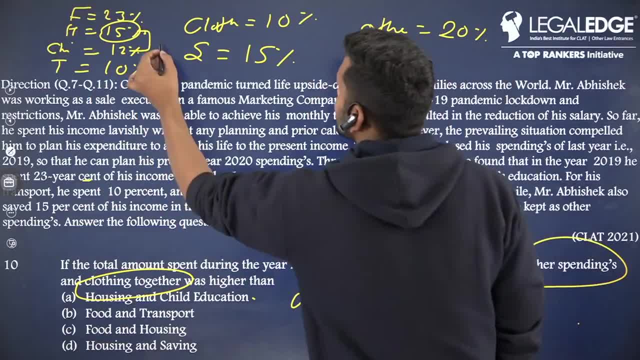 aur child ka kitna hai? 12 hai, toh 15 aur 12 kitna ho jayega 27? haa, sir, iss se toh abhi jada aara hai. iss se toh jada aara hai, lekin abhi tick nahi kar sakte. ki answer hai ki. 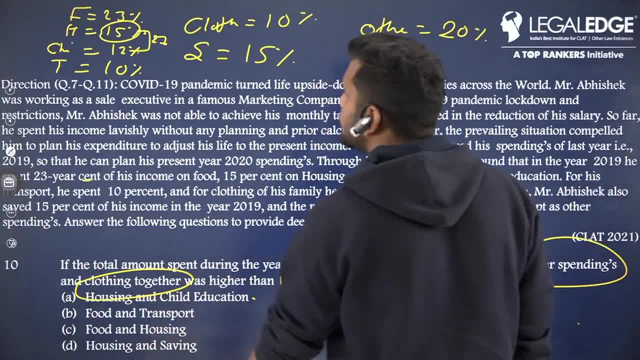 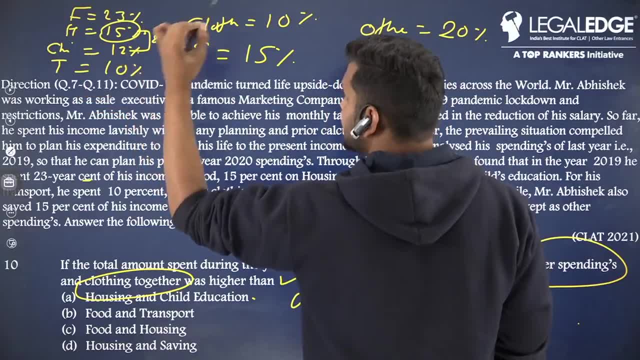 nahi. aur dusre pe bhi dekne padega housing and child education. housing and child education ka dekne padega child education ka kitna bhi. First is housing and second is food and transport. Food is 23% and transport is 10%. 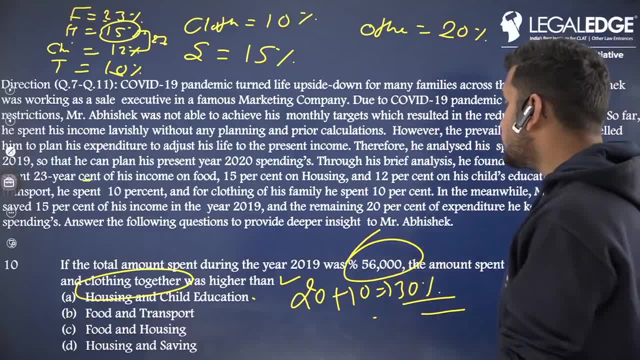 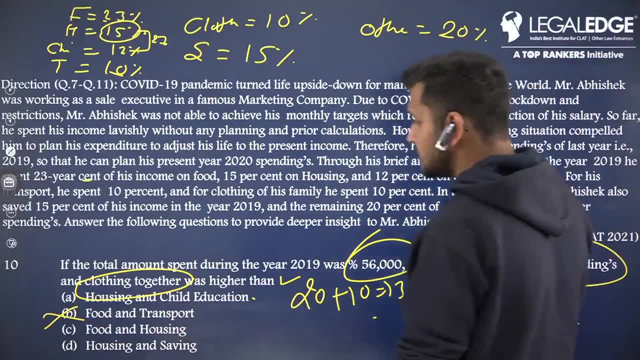 So 23% plus 10% will be 33%. This is exceeding Means. this answer is not possible. He is saying that 30% is more than what Let's see. food and housing. Food is 23% and housing is 15%. 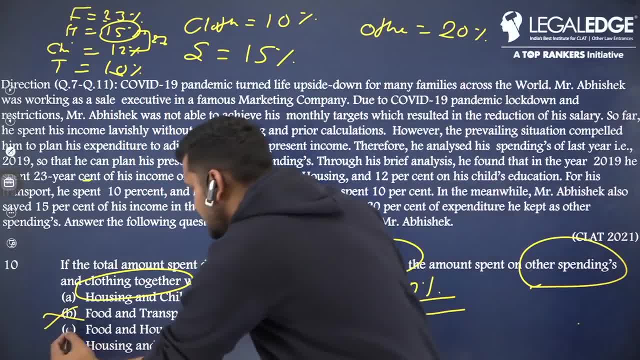 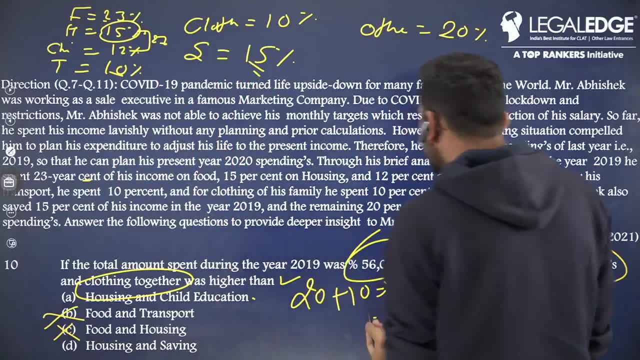 23% and 15% is still exceeding 30%, So there will be no option Talking about housing and savings. Housing is 15% and savings is 15%. Sir, this is 30%. Equal is there? So this will also not be an answer. 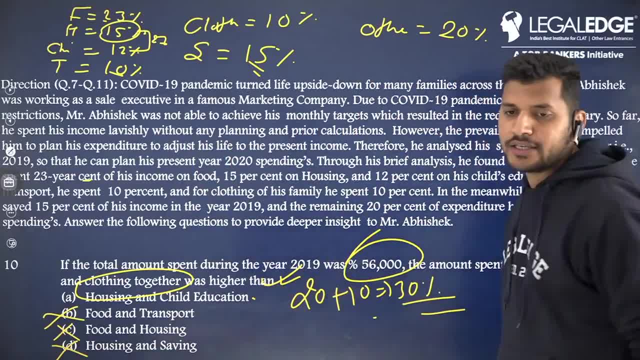 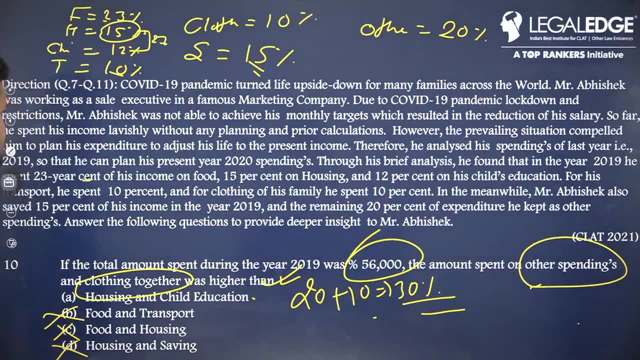 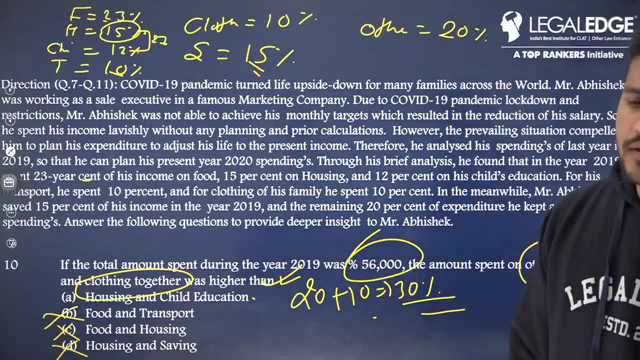 Because he is saying higher. So option number A will be correct. A will be correct. Okay, This question came last year. Now you tell me How many easy questions come. You say that math is tough. I am making you practice. 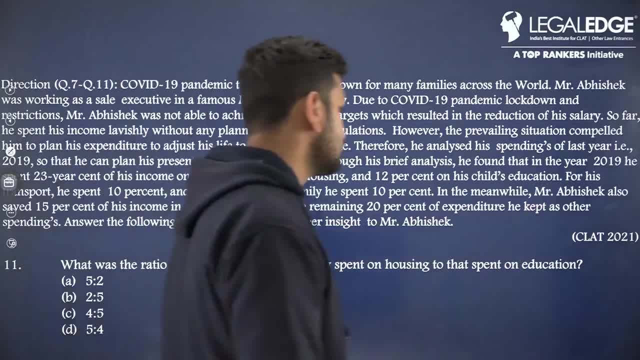 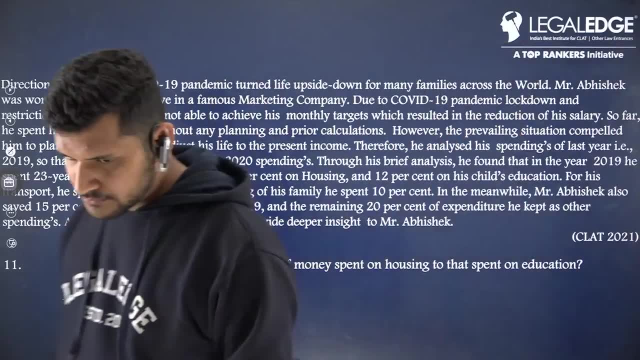 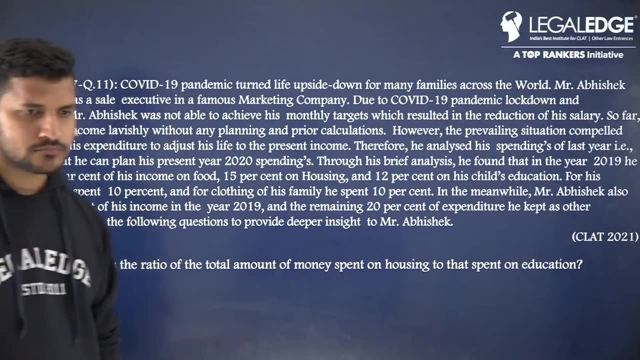 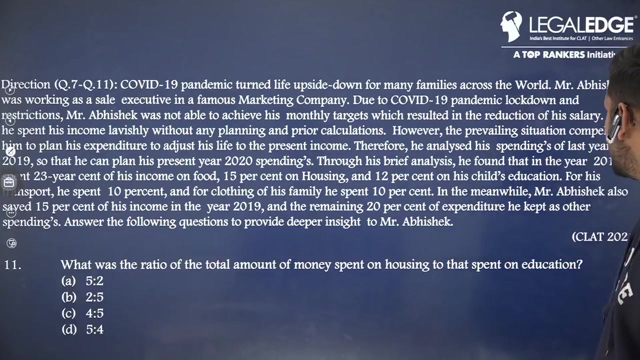 At least practice once. Tell me another answer of this quickly. No answer will come. What was the ratio of total amount of money spent on housing To that Spent on housing or education? Write the percentage directly. You can take out only the percentage. 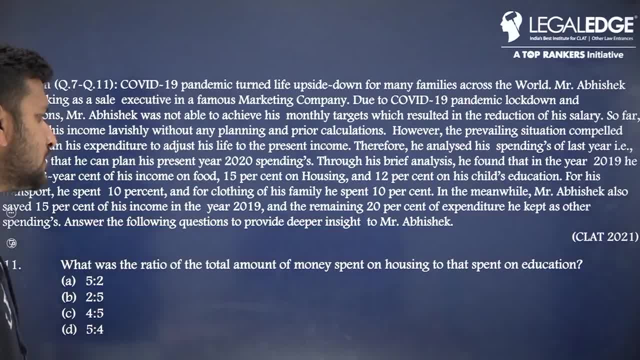 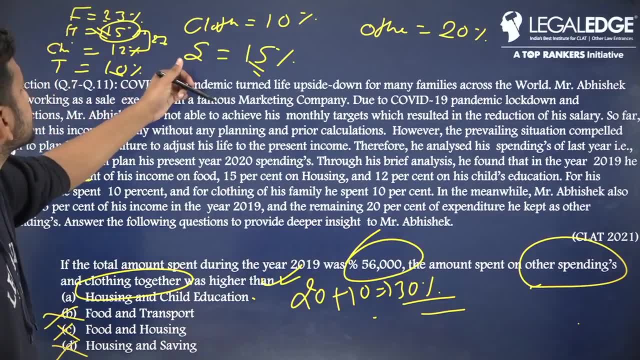 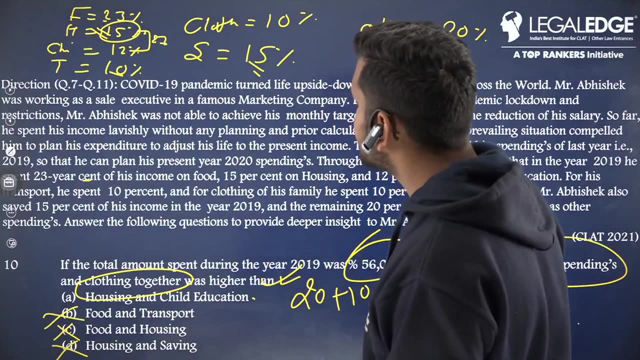 There is no need to do anything Right. Which one you want to see Housing to that education? See housing and education Housing is 15%. How much is education Housing is 15%. Child education is 12%, 15 and 12.. 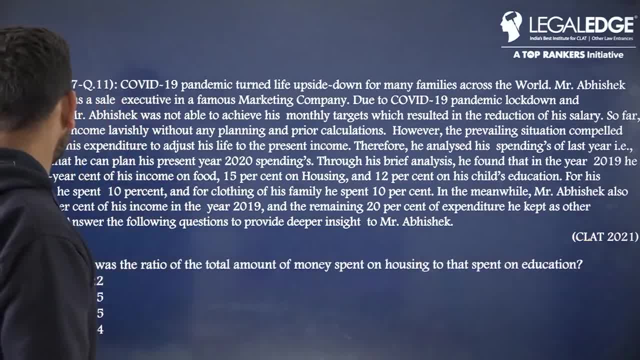 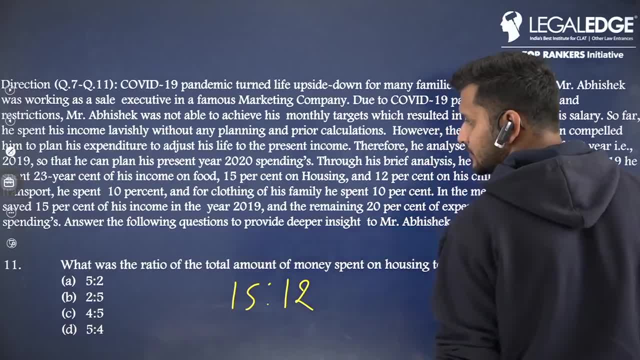 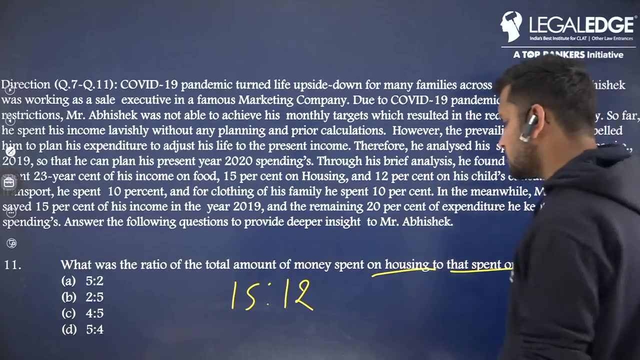 Right, 15 and 12.. 15 is housing And education means child education. Okay, So keep in mind Housing to that Spent on education. So 3 goes to 4.. 3 goes to 5.. 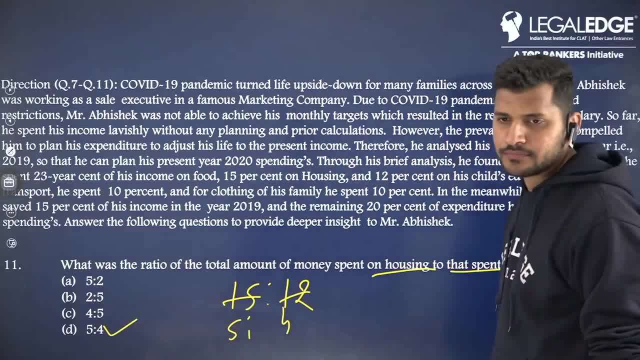 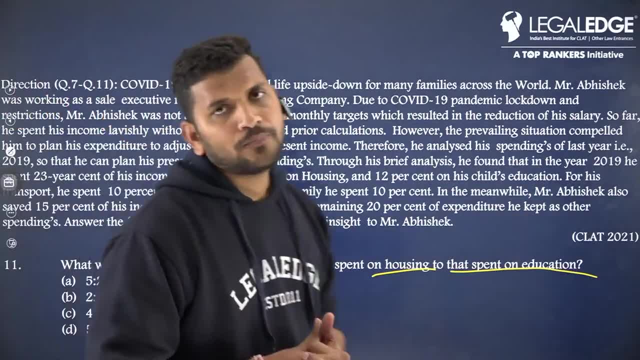 So 5 to 4 will be the answer. D will be the answer Right. This is how you have to solve these questions. These questions are not difficult. If you start doing it, Then math will also be easy. We just have to practice. 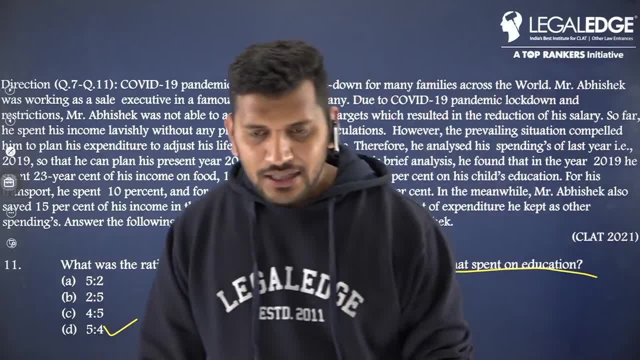 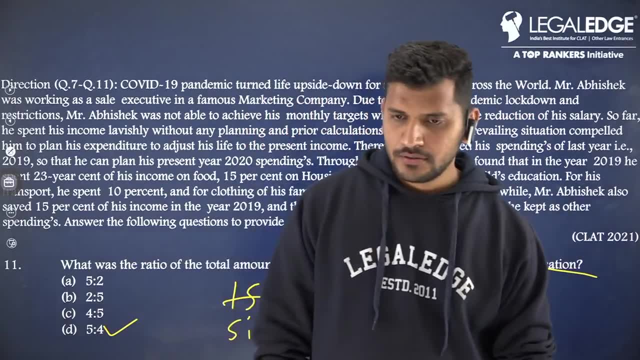 Right. So guys Like Subscribe, Share, Comment, Do everything And thank you so much for today. Okay, Then we will meet in the next session With a good video like this. Yes, 5 is to 4 answer. 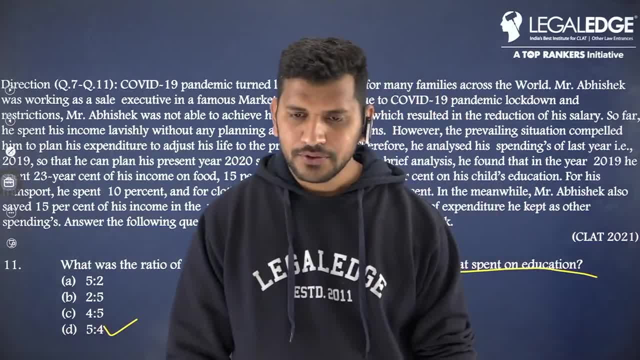 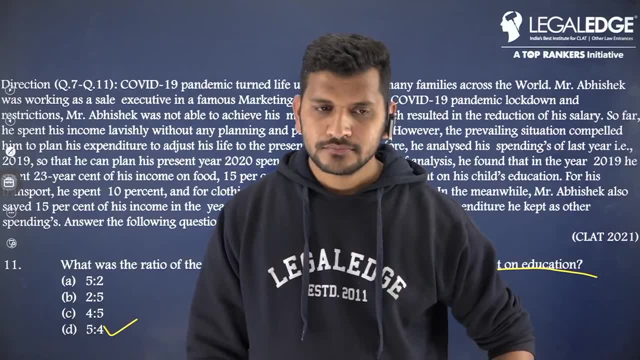 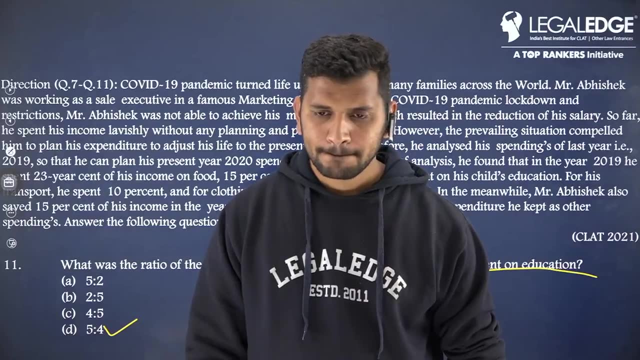 All are correct, Right, Then we will bring the next video, Whenever it happens. Then finish today's class, If you have permission. Bye, Bye, Bye, Bye, Bye. Thanks for watching. Love you all And stay in good health. 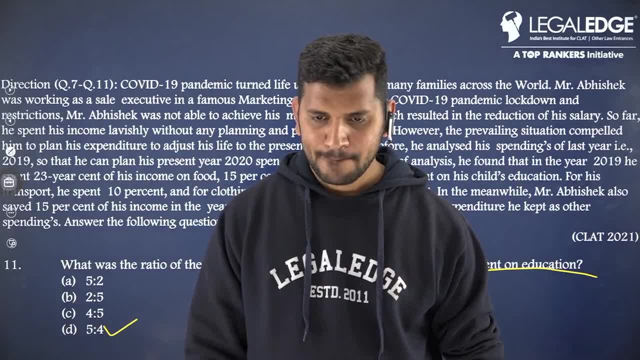 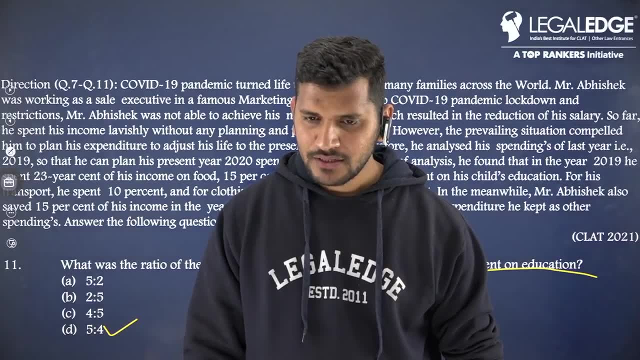 Sayonara. Bye, bye, All right, I'm going to get this done. Many have not played in the last couple weeks This kind of Oil Islamic Welcome to all. Look, he is ready. We will start at 8 paus, but 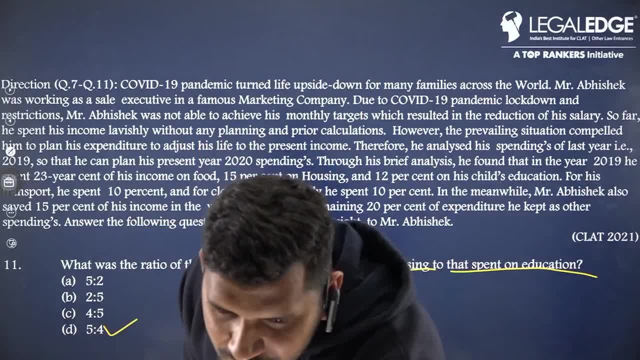 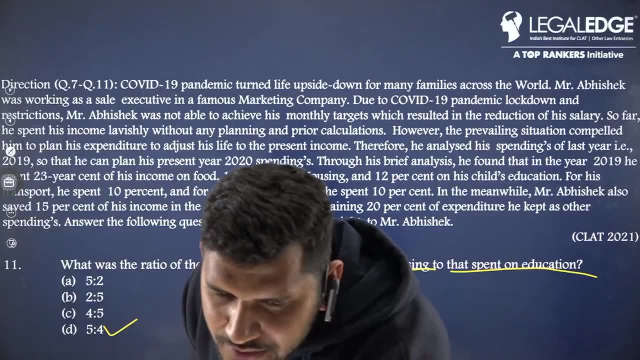 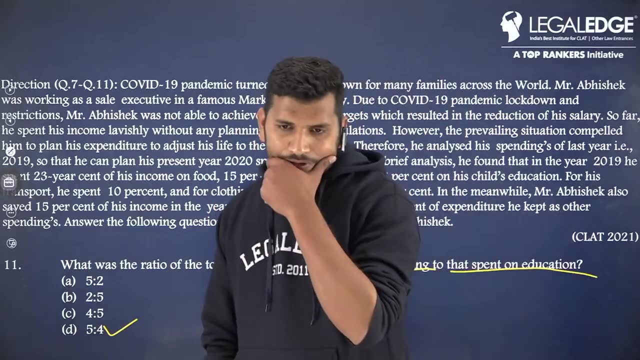 He got me ready for this class. CYeah, Ok, And I will take the class. No exam is required for investment. I don't understand, Pranay. Good night, Pranay. Pranay, you do one thing: You can take any friend from him. 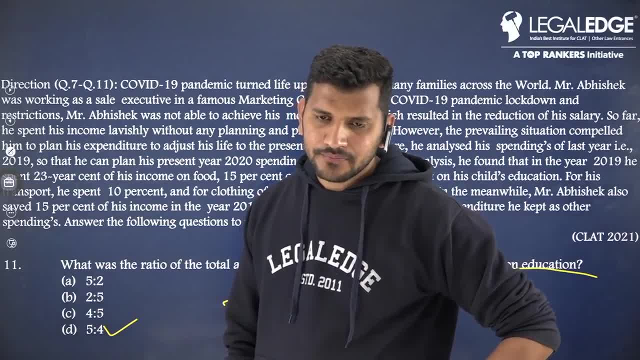 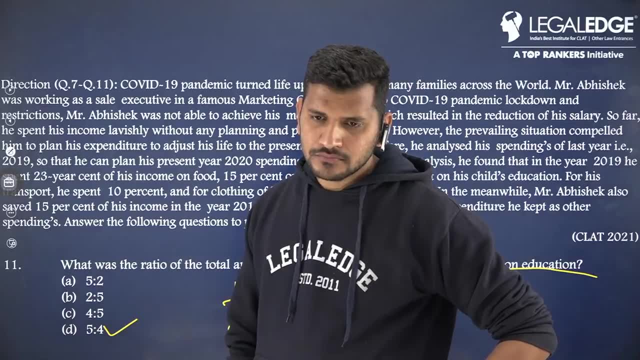 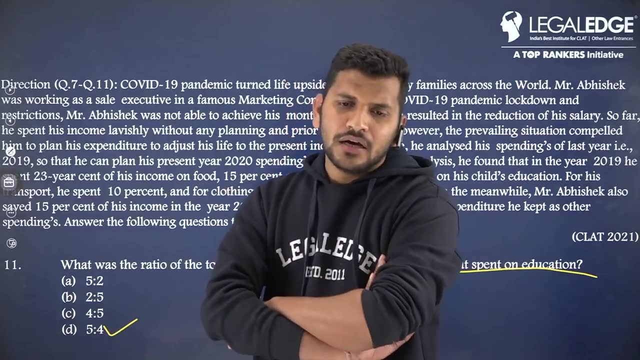 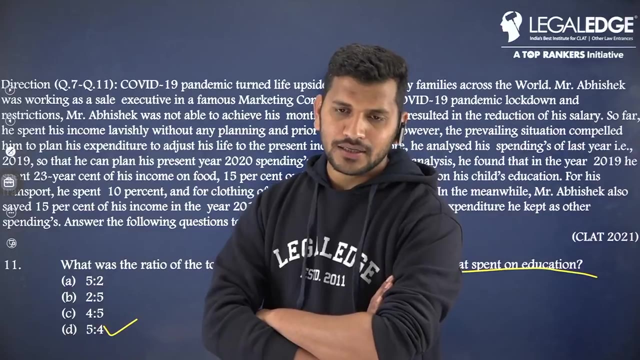 You will get some material. Thank you so much For that. I am telling you that you will get RSM4 from anywhere. You can put DI Data Interpretation. You can put Caselet DI On Google, Caselet DI for bank- You don't need book. You don't need book. 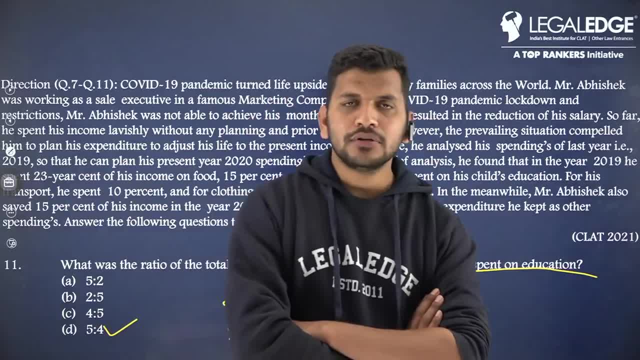 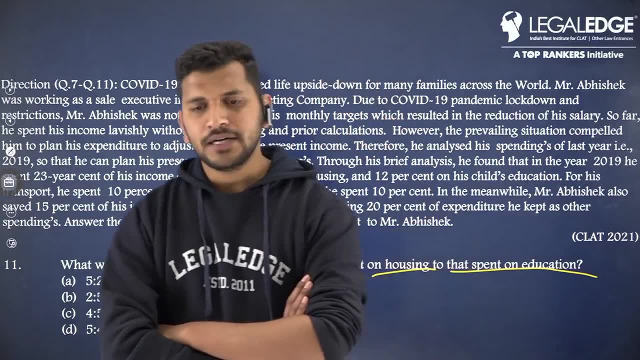 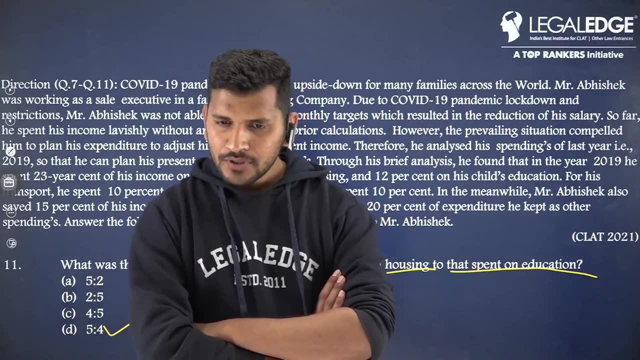 Put Caselet DI for bank. Put some tabular DI. Tabular line graph, bar graph, pie chart, Mix graph. Put Caselet DI. Put it on net. You can do this much. Thanks for your wonderful session. Thank you Login. Thank you. Thank you so much everyone. 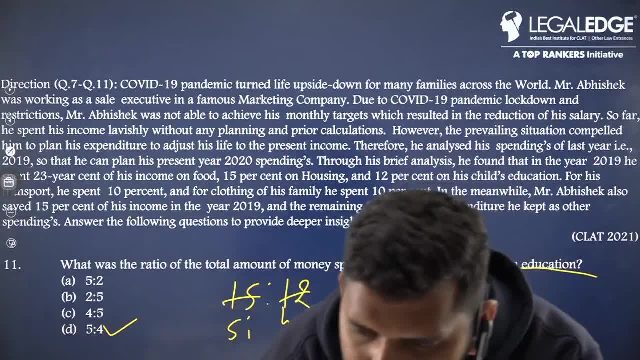 Let's end Good night, Thank you.